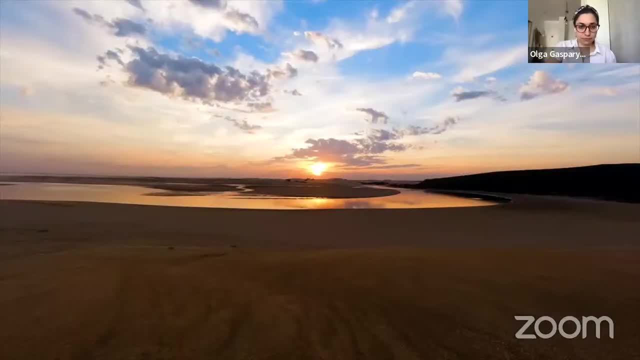 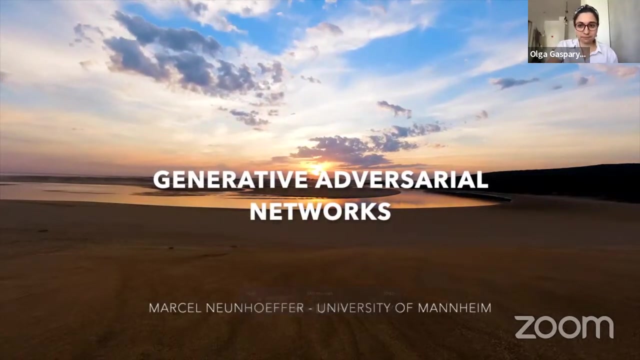 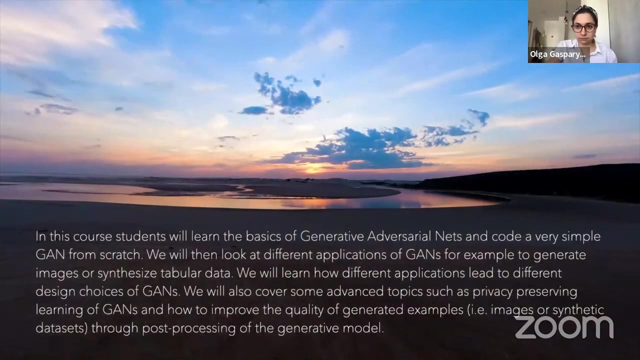 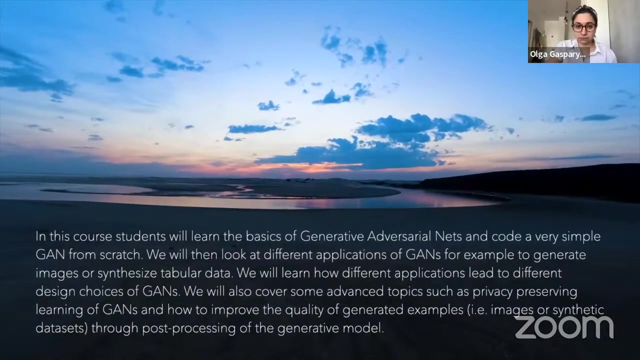 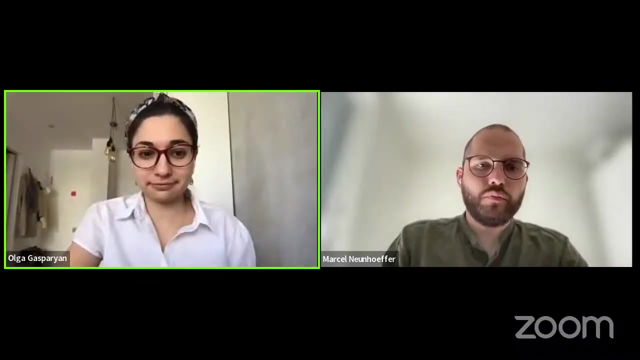 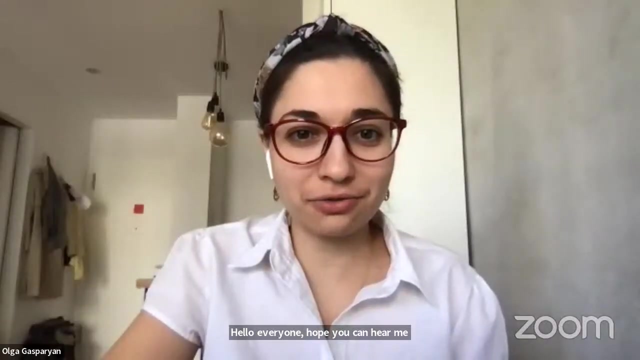 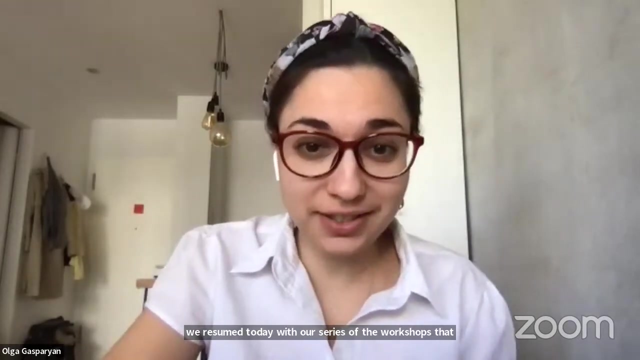 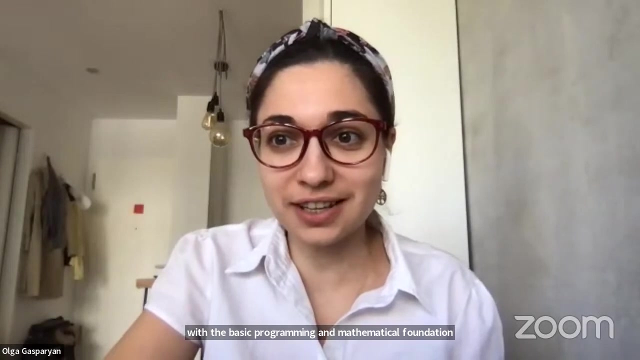 We can start now. Sound blank, but it's okay, right? Hello everyone, Hope you can hear me Well, welcome back. We resume today with our series of the workshops that are that are having advanced topics. So we are done with the basic programming and mathematical foundations necessary for data science scientists. 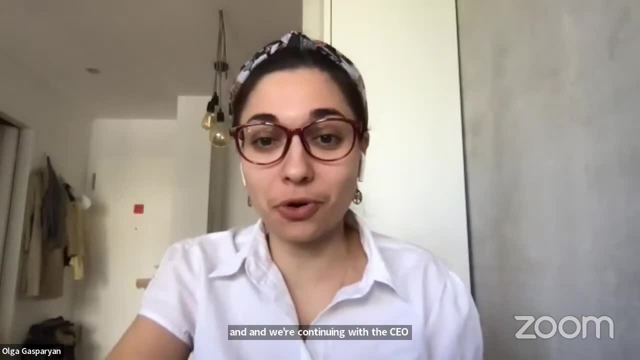 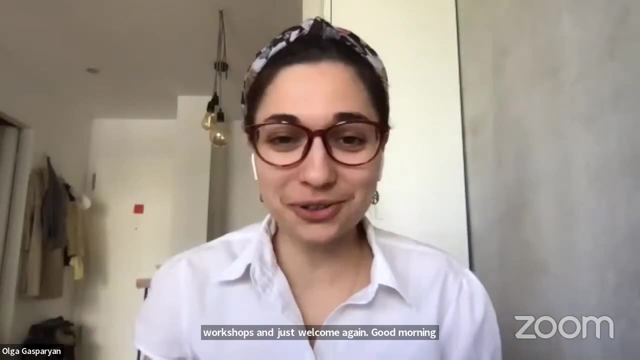 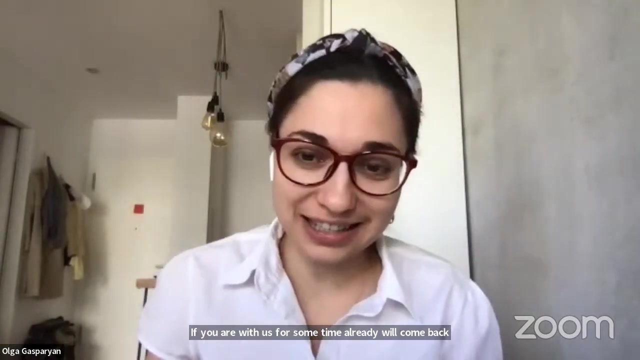 And and we're continuing with a series of more advanced workshops. And just welcome again. Good morning, Good afternoon or good evening, depending where you're located. If you're with us for some time already, welcome back. If you're new, welcome to the second data science summer school organized by the Hardy School Data Science Lab. 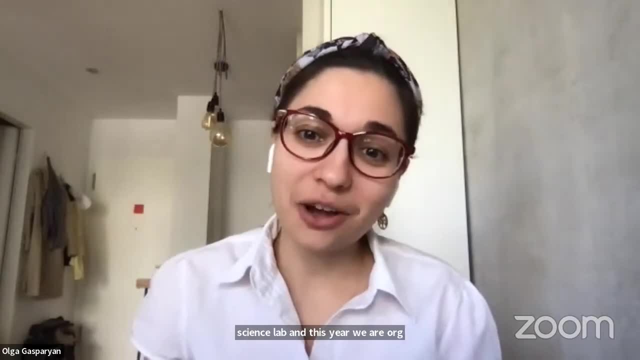 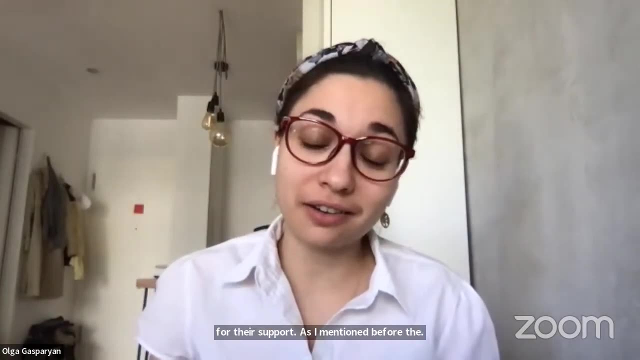 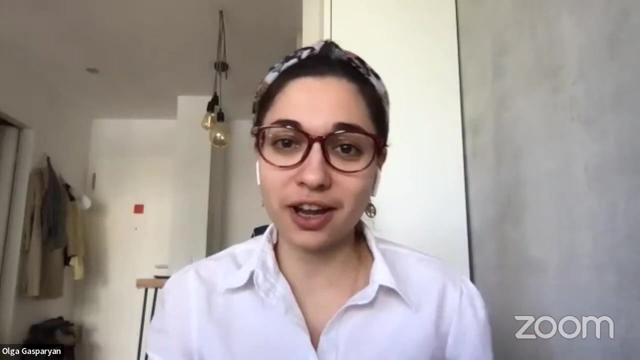 And this year we are organized and funded by Hardy School, which we're really grateful for their support. As I mentioned before, the, the, the, the school kind of is split on the introductory workshops that we're done with, But you can find all the materials of this workshops on our Web page. 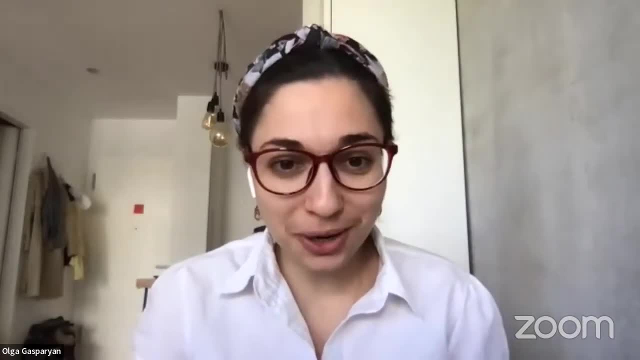 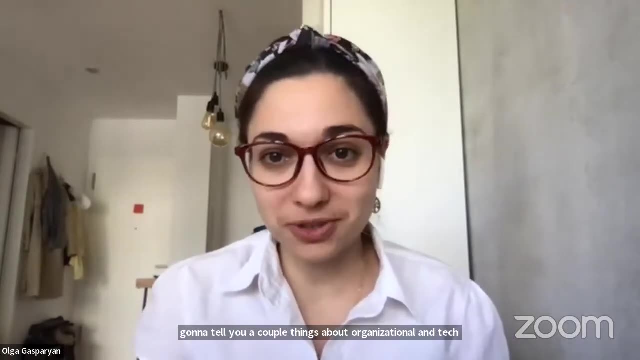 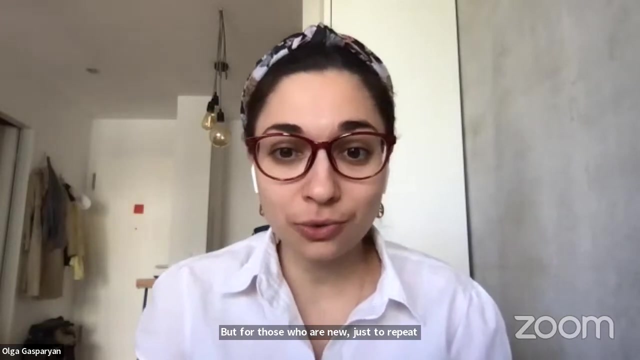 And now we're continuing with advanced workshops. I'm going to tell you a couple of things about organizational and technical details. Sorry for repetition if you're with us for some time already, But for those who are new, just to repeat that if you are on Zoom you, you probably are muted and your cameras are off upon entry. 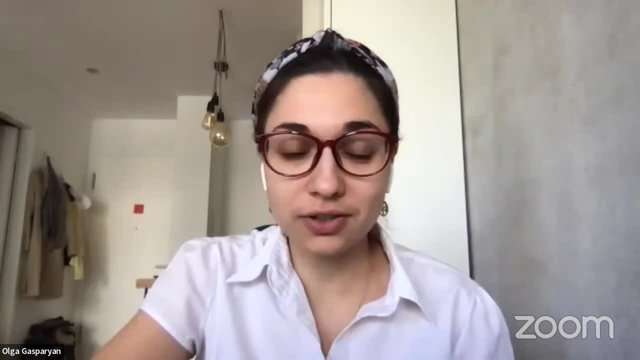 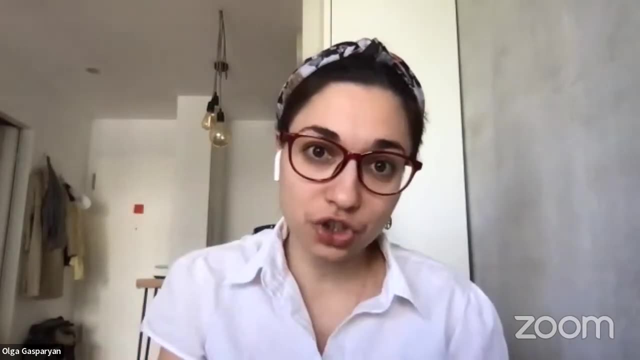 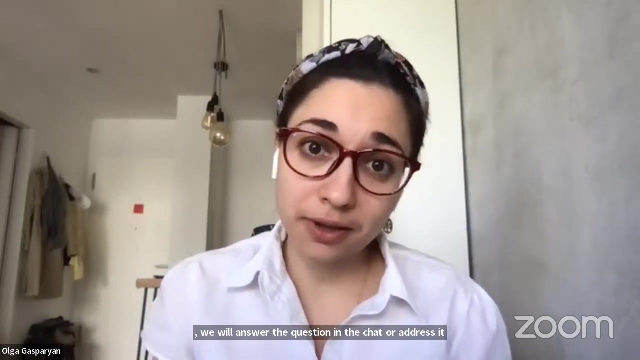 Please do not unmute yourself or turn your videos on unless you do have a question. If you want to ask a question, you can put it in the chat. We will answer the question in the chat or address it To the instructor. Or, if you do want to speak up and, you know, actually ask the question out loud. 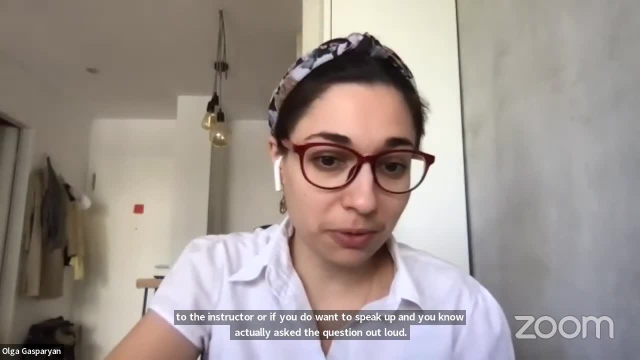 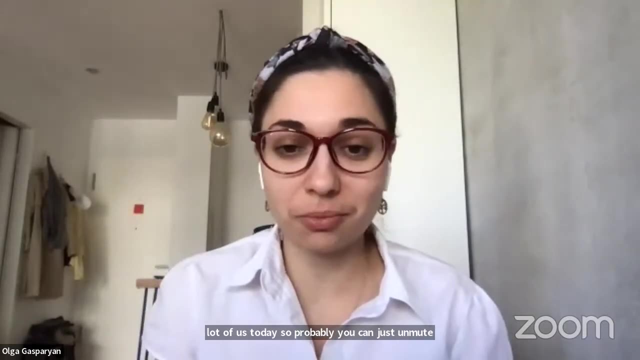 You can raise your hand, or, judging by the amount of people here- Actually it's not a lot of us today, so probably you can just unmute yourself and just ask a question, And actually Marcel said that it's. it's okay with him if you just like jump in and ask the question. 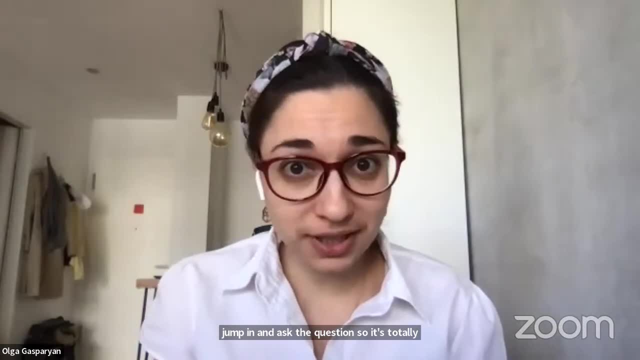 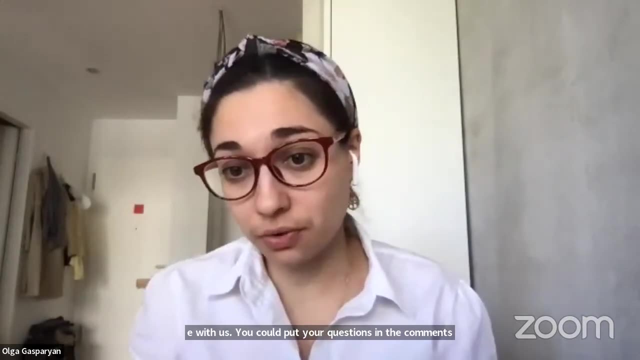 So it's totally fine. if you are in the parallel stream session on YouTube with us, You could put your questions in the chat. You can put your questions in the comments box And we will try to answer the question there or address your question to the instructor. 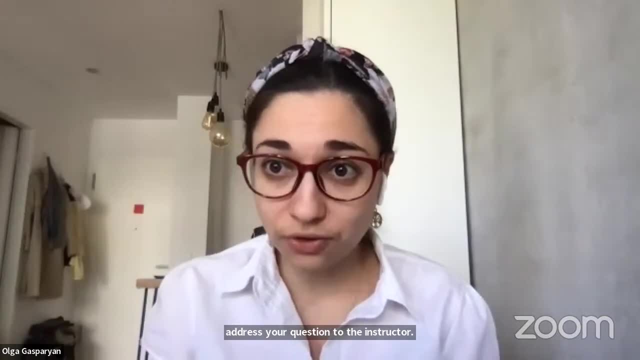 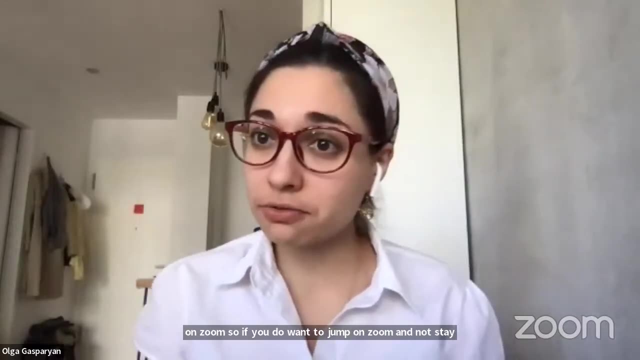 Also just just a quick note. We do still have a room on Zoom, So if you do want to jump on Zoom and not stay on YouTube, please, you're more than welcome to do that. I also want to remind everyone that the Zoom session is being recorded. 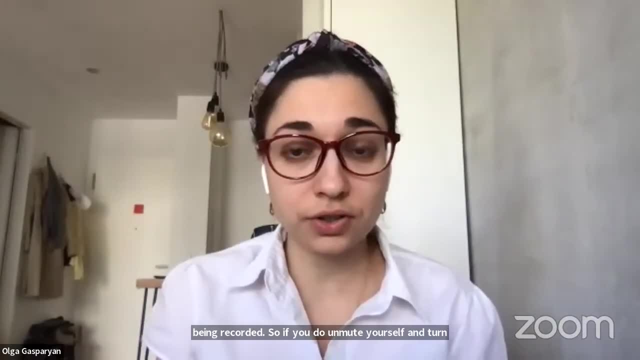 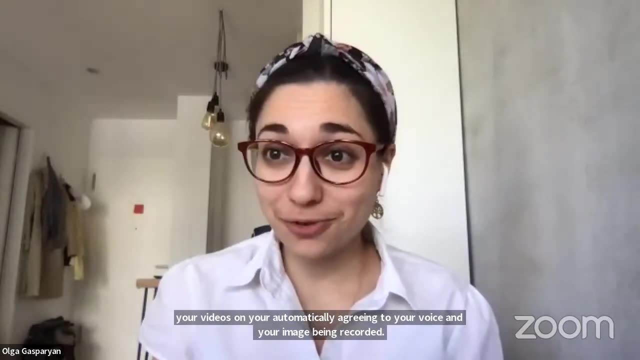 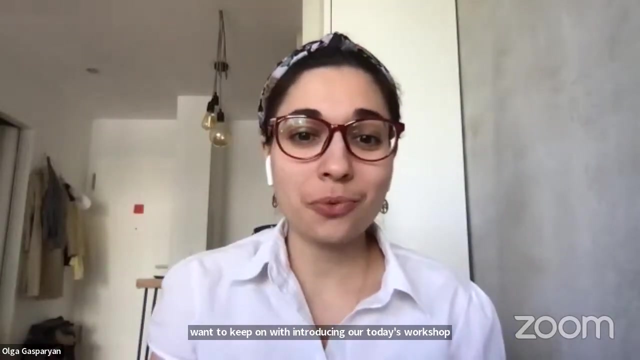 So if you do unmute yourself and turn your videos on, you're automatically agreeing to your voice And your image being recorded. Thanks in advance for following these rules, And I just want to keep on with introducing our today's workshop. We're continuing with the with the, as I said, the first workshop in the advanced series. 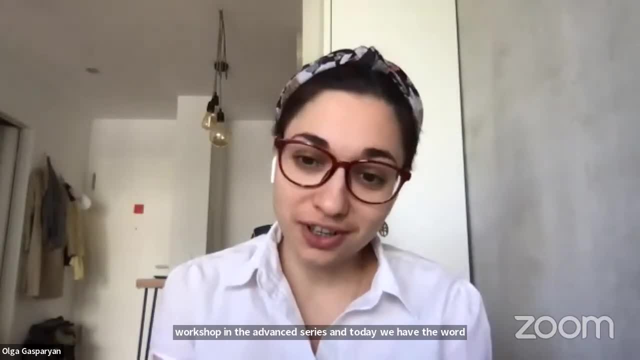 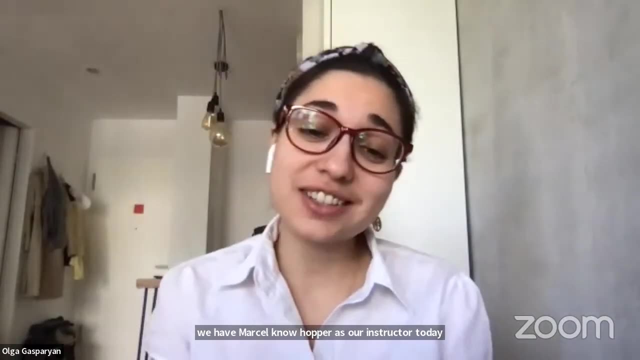 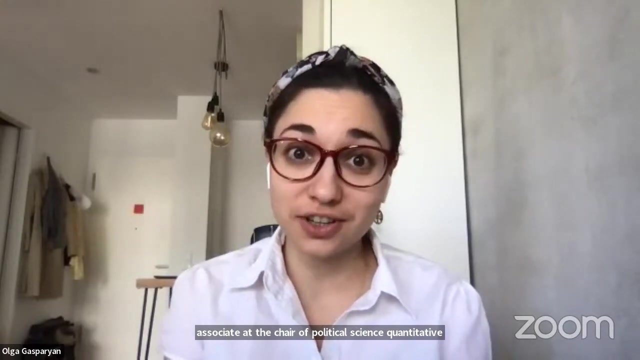 And today we have the workshop on generative adversarial networks- GANs, And we have Marcel Neuhofer as our instructor today. Marcel is a PhD candidate and research associate At the Chair of Political Science- Quantitative Methods in the Social Sciences at the University of Mannheim. 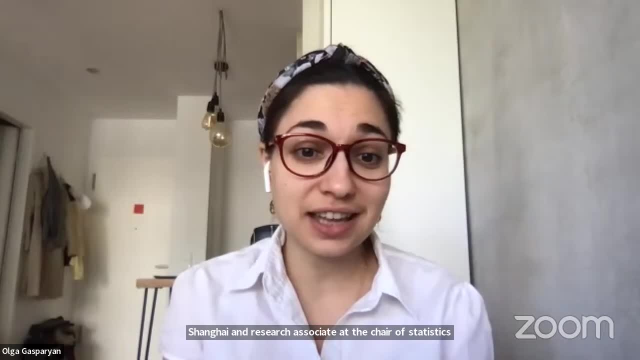 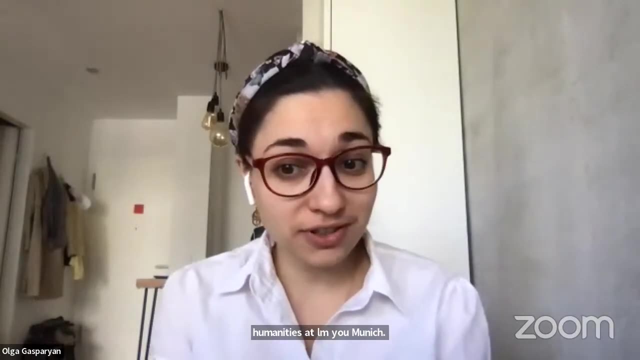 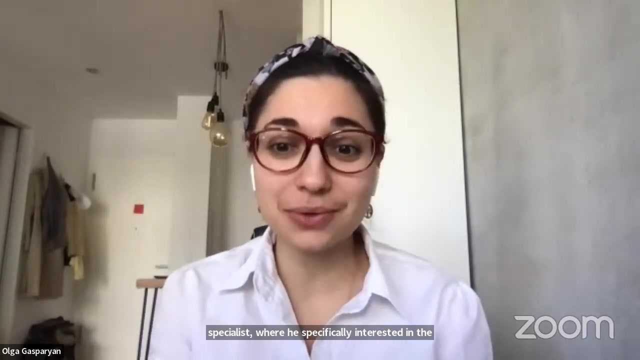 And research associate at the Chair of Statistics and Data Science for Social Sciences and Humanities at LMU Munich. His research focuses on quantitative methodology, where he's specialist, where he is specifically interested in the application of deep learning algorithms to social science problems, And he's also a co-founder and contributor. 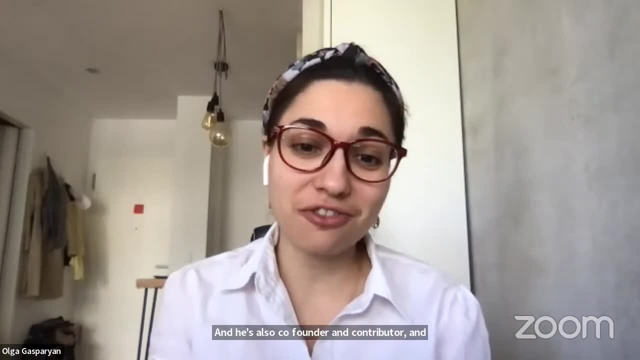 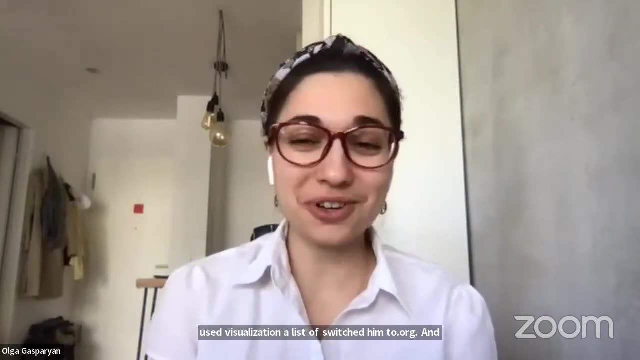 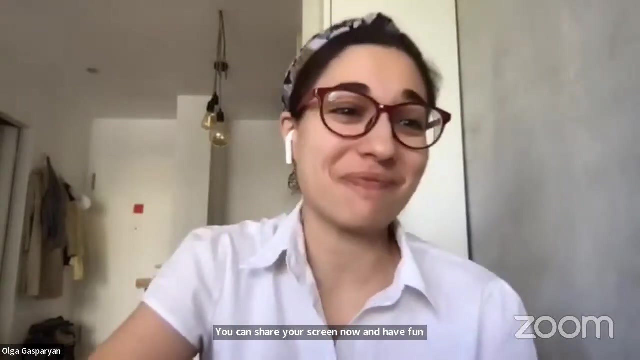 And they've used visualizationalists, And, without further ado, I just want to give the words and then the place to Marcel. Marcel, the floor is yours. You can share your screen now and have fun and welcome everyone. Good luck, Thank you, Olga. 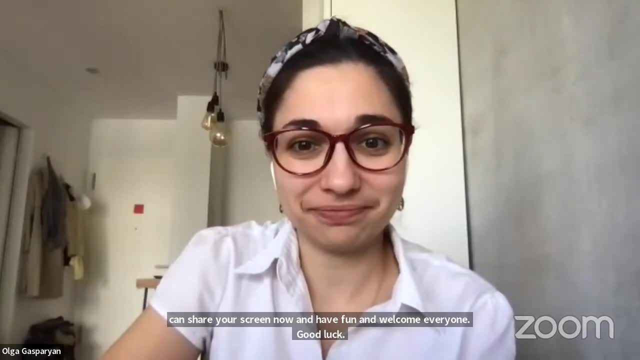 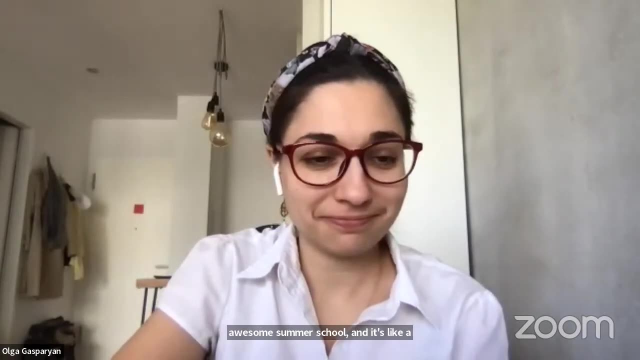 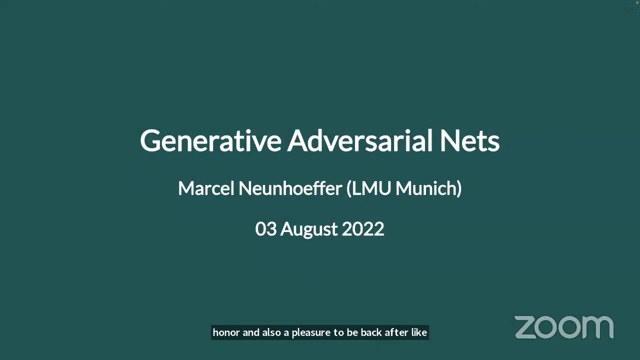 And thank you for organizing this awesome summer school And it's like a great honor and also a pleasure to be here. Thank you, And it's also a pleasure to be back after like instructing a course in machine learning last year. 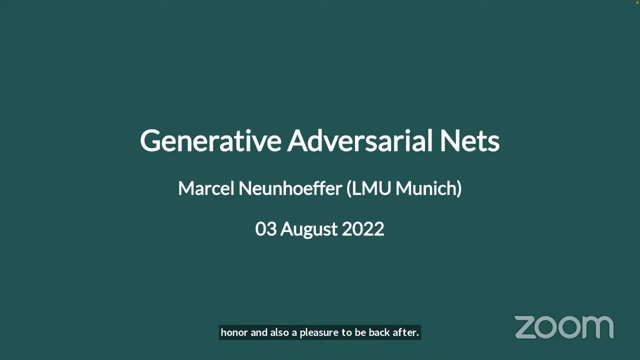 And this year like one of the advanced topics on generative adversarial nets. And also I'm excited that so many participants are here in Zoom And I hope, like in the first, like 10, 15 minutes to get to know you and your interests. 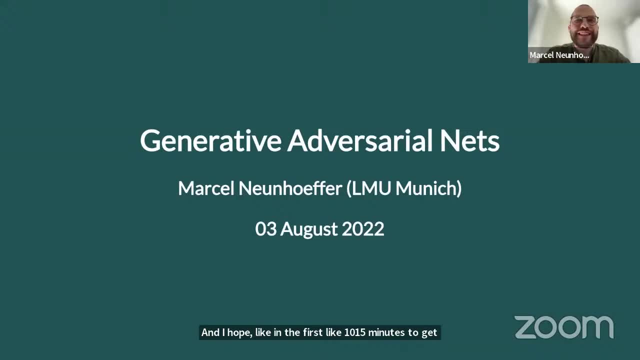 And what you want to get out of this course, a bit like, even though it's so many, And then we will dive in right into the like class for today. I hope you can all see my screen right now And before we get started, some housekeeping. 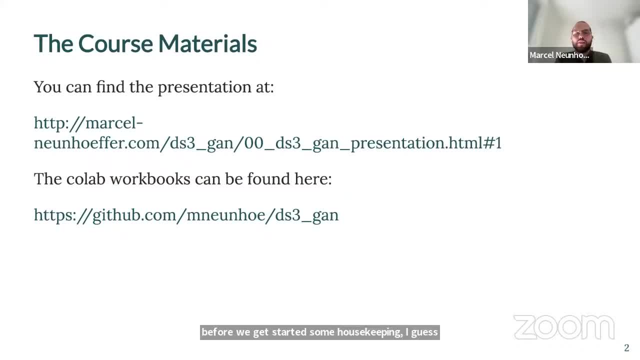 I guess you also found, like those links in the chat already, Like if you have any questions, Like if you want to follow along the presentation in your own pace or go back a few slides, you find that at the first link. 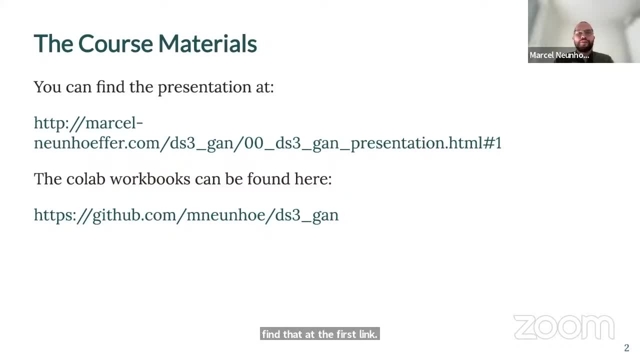 And or like look at the presentation after the course today, And we will have three Colab workbooks that we will walk through and work through along the way that you will find in that GitHub repo down here. Thank you, And also they will be up like after the course. 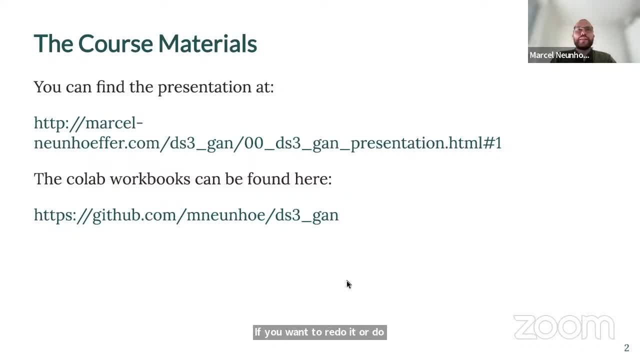 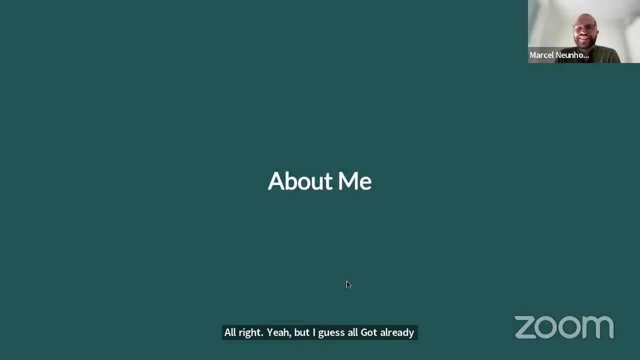 If you want to redo it or do it on a like on your own computer, All right. Yeah, like I guess Olga already said, like everything that can be said about me. But if you're interested, I'm happy to go to the next slide. 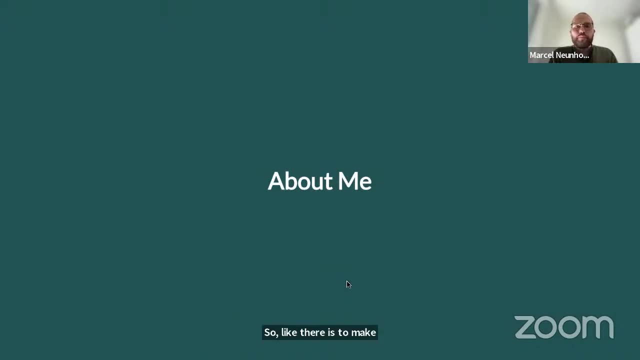 We will start with a little bit of text about generative industrial nets. That's actually a method and a technique that I used in my own research. So like there is two main directions there and the other big application, there is multiple invitation. 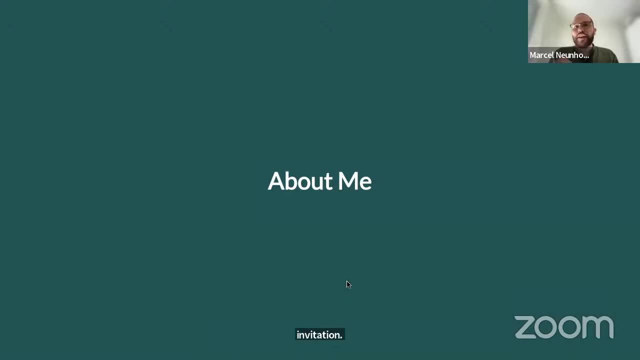 And so like it's. yeah, it was a great fit. I was very happy to be asked to play this course at the summer school And, as Olga also said- and please do that- interrupt me at any time, like if you have a question. 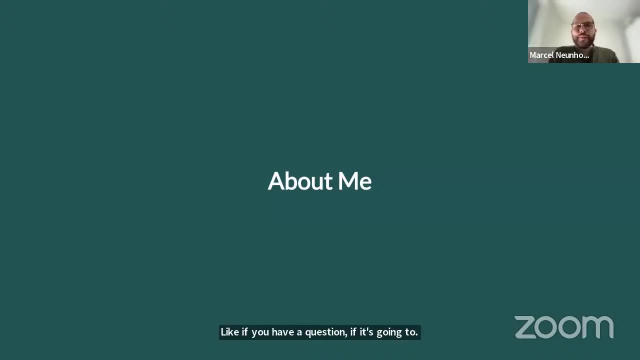 if it's going too fast, too slow, if something wasn't clear, let me know And I will answer your questions or try to answer them and like accommodate any other issues. All right, so let's get started with like learning a little bit about you and your interest. 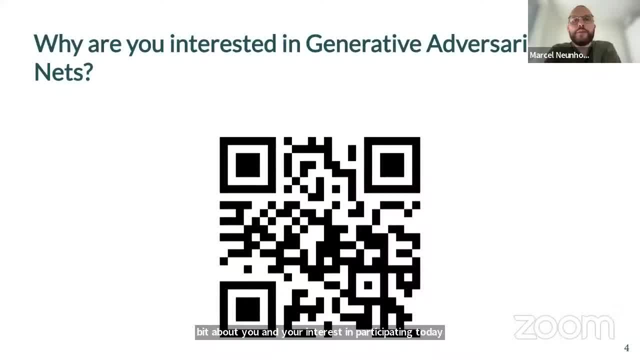 in pedagogy, So I'm really excited to be participating today. I set up a little mentee, So if you follow that QR code, you will get to an entry mask of where you can put in like five words or five phrases. 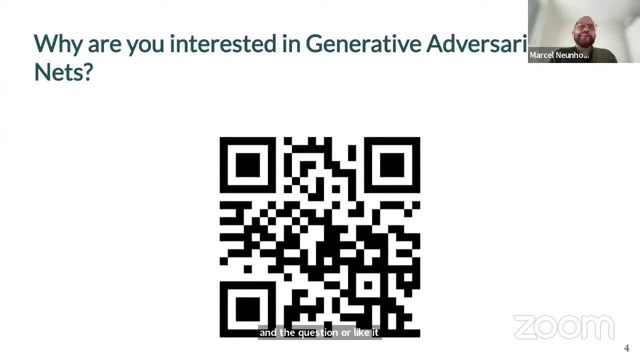 And the question- or like it's an open question- is: why are you interested in generative adversarial nets? And there's no right answers, There's no wrong answers. So I'm really honestly just curious about, like, what brought you to this class today. 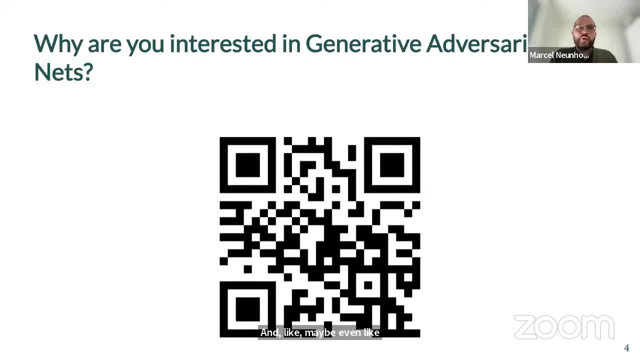 and like, maybe even like- what your goals are in your own research as data scientists, social scientists, with generative adversarial nets. So if you follow that QR code, just type in some words, it's all anonymous And it will generate a nice word cloud. 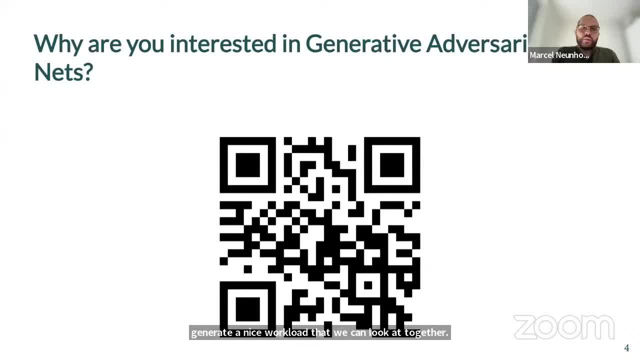 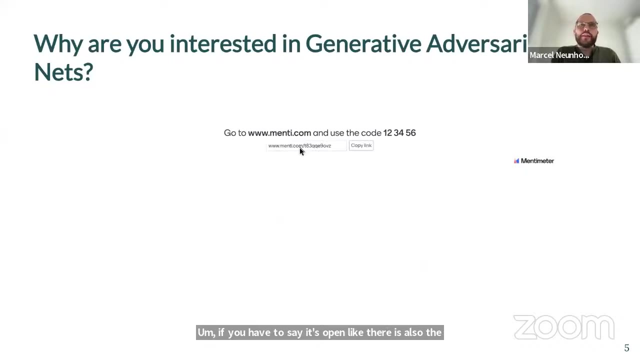 that we can look at together to learn about your interests today And then I hope like that this matches with what I have in mind for this class. If you have the slides open like, there is also the link in there, So therefore I can like here. 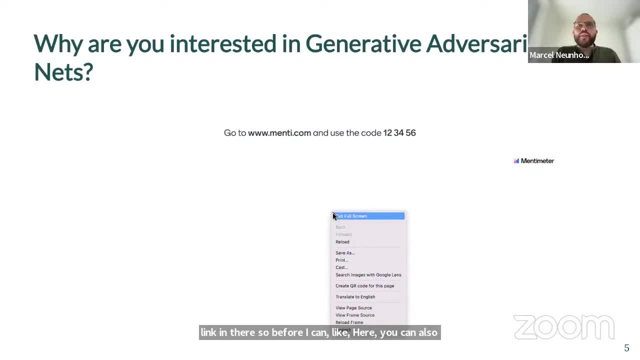 you can also just copy that link. So for some reason on the access code doesn't work. And we already have some first interests. We have machine learning knowledge, deepen knowledge, data-driven analysis job- That's interesting. Job preparation- I don't know them. That's a very valid interest in learning something. Reorientation, I guess. 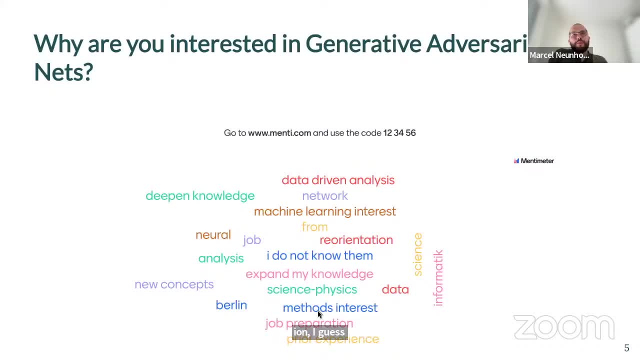 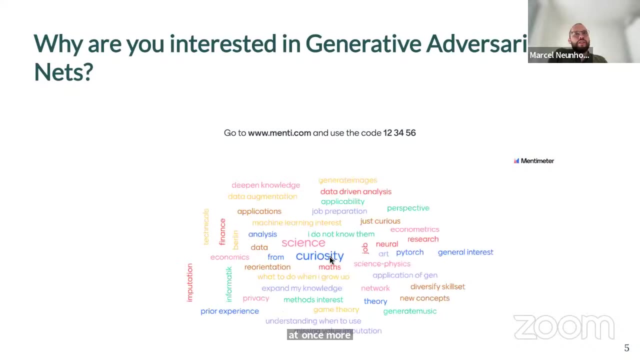 the yellow ones. they probably come from one person: Prior experience from science. Let's just reload once more to see if more Curiosity- That's always great for science and research. Diversify skill set PyTorch. We will work with Torch today, so that's a good match. 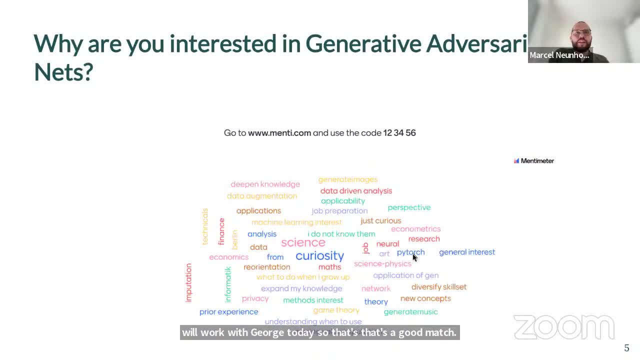 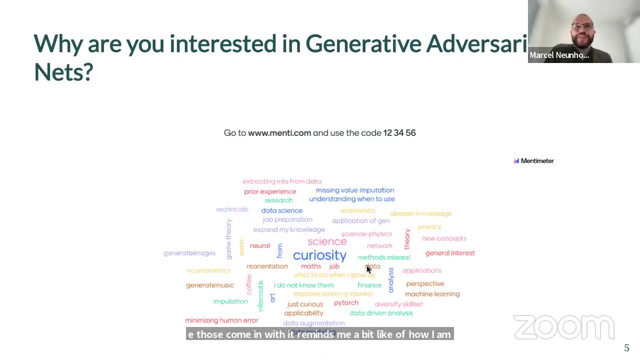 Although it will be from R, but it's very, very similar to what's going on in PyTorch And, while those come in, it reminds me a bit of how I also got started with generative adversarial nets a couple of years ago. Curiosity in the center here was really what started. 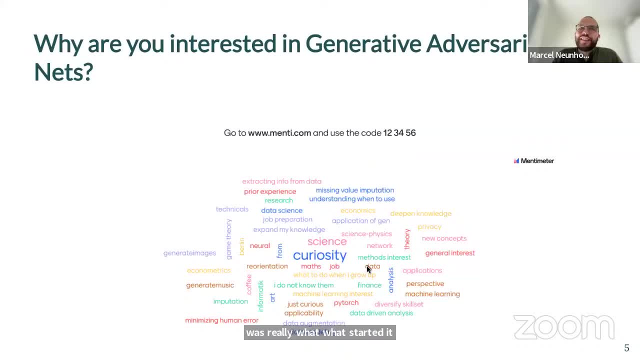 it, And a bit of hype about it as well, Because of all the cool or fancy applications, And I'm trying to think about how this could be useful as a political scientist or data scientist. So I hope to take you on that journey a bit. 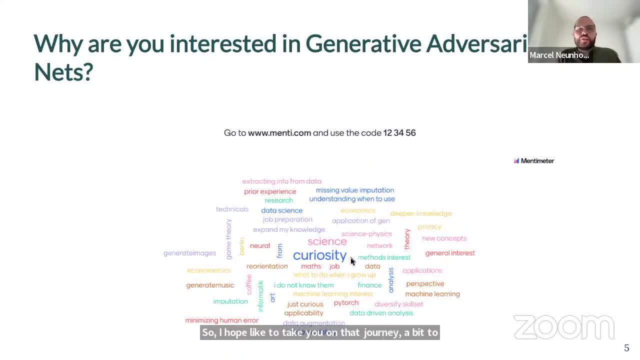 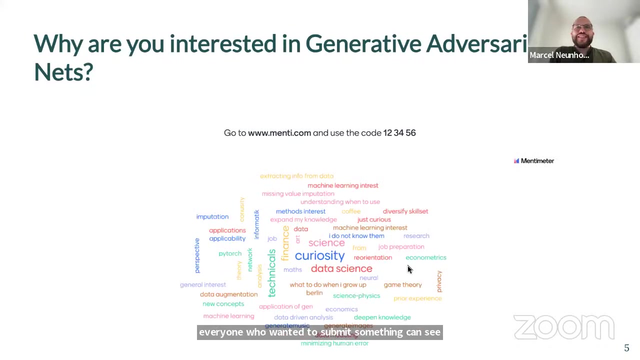 To show you why I think it's very relevant to understand the basics And then also get to like fancy, fancier things And really I think a little bit more about the kind of the tools and applications where we look at images And also privacy preserving synthetic data. 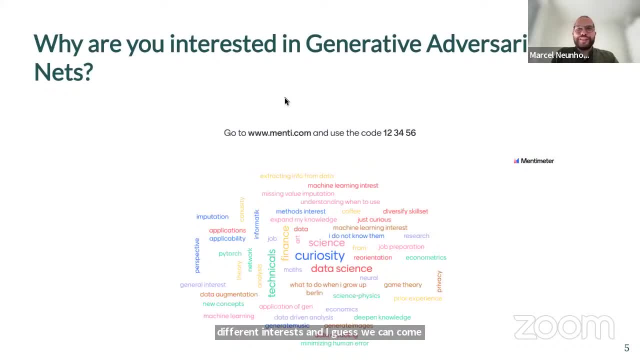 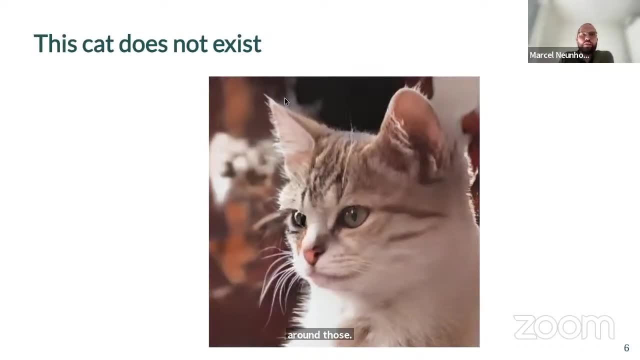 All right, Let's just reload once more. Then, like, everyone who wanted to submit something can see it here. Yeah, It's like a nice colorful basket of different interests And I guess we can try to work around those, All right. So I guess, if you heard the term like, even if it was just for the purpose of this course, and you maybe Google it, what you probably came across is like pages like: this cat does not exist. 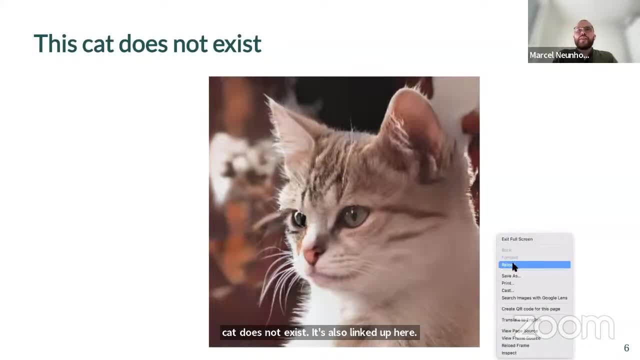 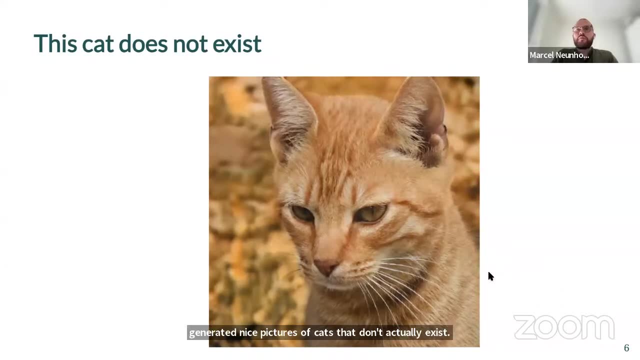 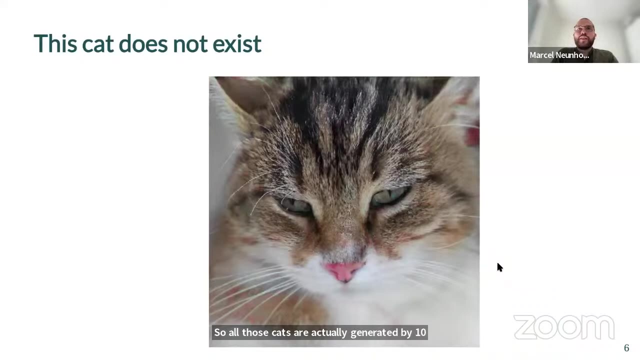 It's also linked up here That generates nice pictures of cats that don't actually exist. So all those cats are actually generated by generative adversarial network that learned to generate fake cats And they look pretty real. Sometimes you will get like this one, like if you have a cat. 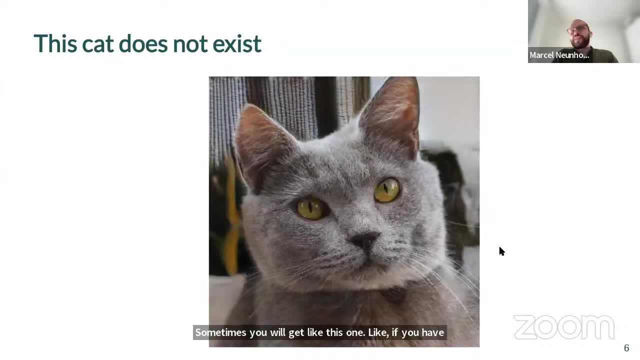 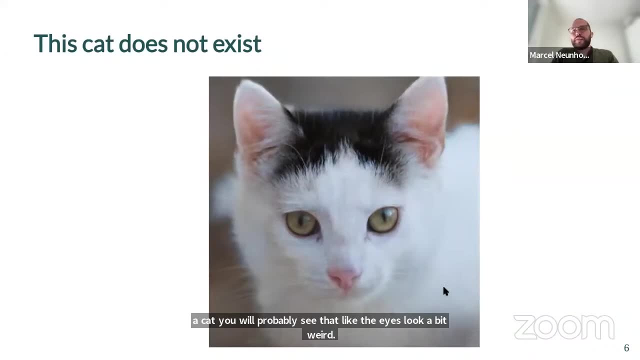 you will probably see that, like, the eyes look a bit weird, But overall they look pretty impressive And that's, I guess, a fun application, right, Like who doesn't like to have a machine that can generate, like, more images of a cat? 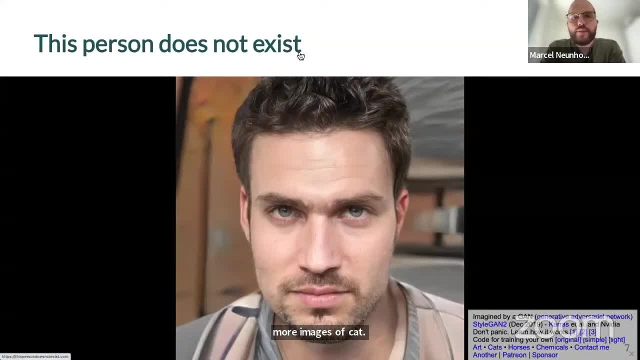 However, like, the same also works, of course, with persons right, And those are really really impressive And I think it's really interesting to see that you know from, like what is called the stygon implementation by people at NVIDIA. 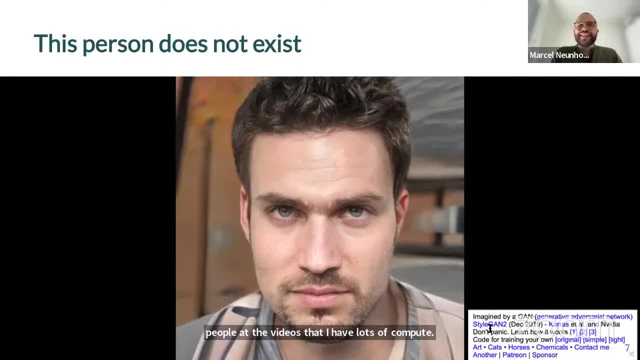 So they have lots of compute, lots of time and probably also lots of training data And they have very like high definition images of persons. And again, this is like a page. This person does not existcom. It's linked up here. 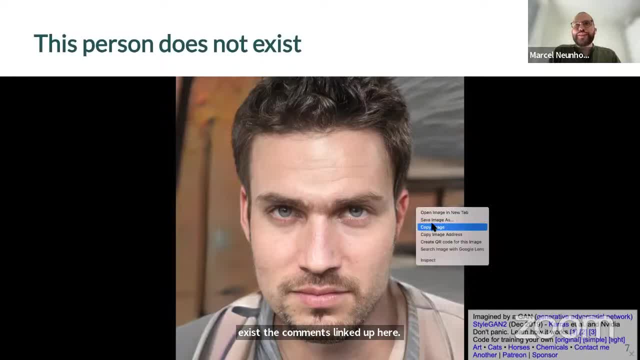 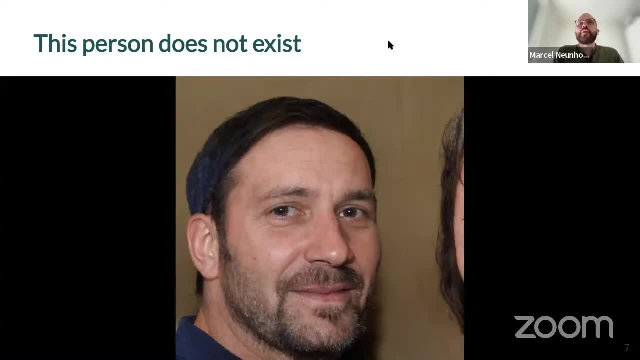 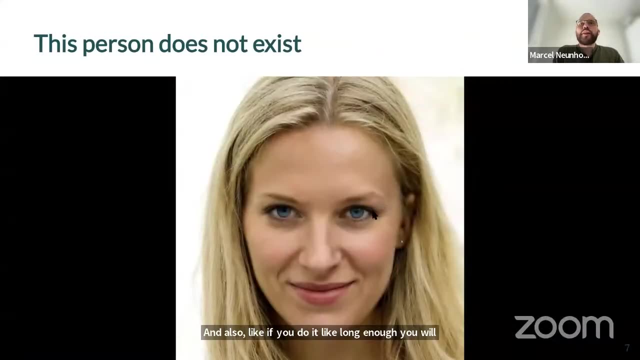 If you want to generate like fake persons by yourself as well, Let's just look at another person here And also like: if you do it like long enough, you will see sometimes weird artifacts that give away the fake person, But most of them are pretty, pretty good. 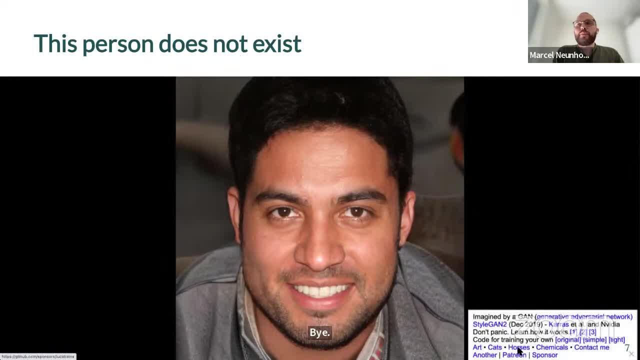 And, like what's also awesome about this page, This person does not exist, it's. it's a great, great resource, uh, to learn about guns as well. so, um, you get links to all those um like implementations that they actually use, um and and also um like they. 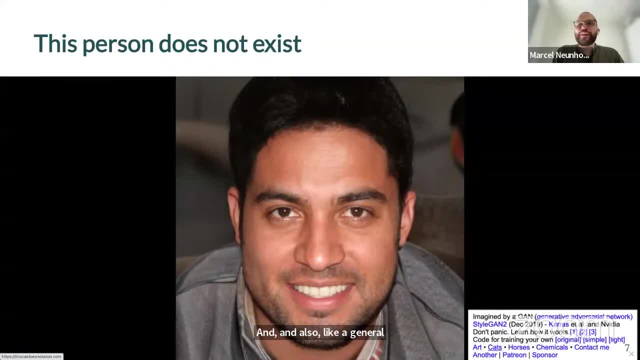 uh, generate other stuff than cats and persons as well, um, if, if you want to see, like horses or chemicals. um, so this is what drew me into into guns at first, like, uh, this amazing capability of, yeah, generating fake data, right, and, uh, images in particular, very hard, or seem to be very hard. 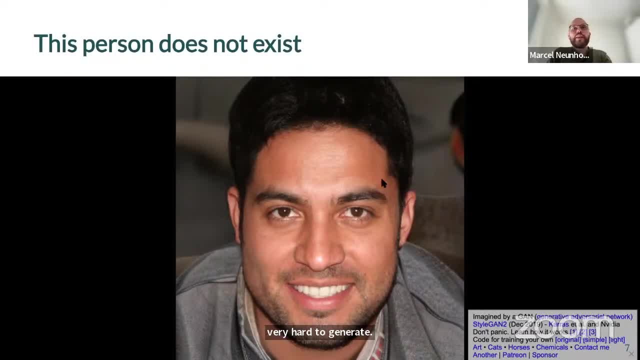 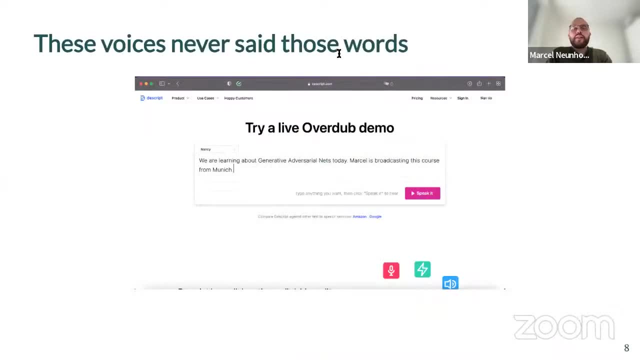 to generate um by machines, uh, pre-guns, um, and honestly, it doesn't stop there, um like. there is also guns for um video and uh, text-to-speech, where, like, you can basically have voices um say anything you want, um that those voices never said like in real life, um, and that's pretty awesome, like um as like this: 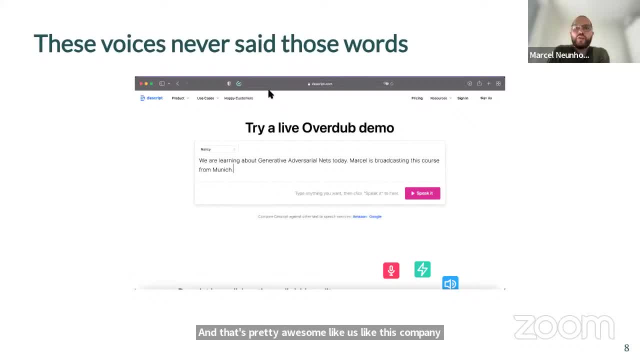 company d script, um offers this as like a tool to edit video or podcasts. um so basically transcribes what you say into a microphone and when you record it and then gives it as as a text, and then you could edit the text, and this would, in turn, um like. 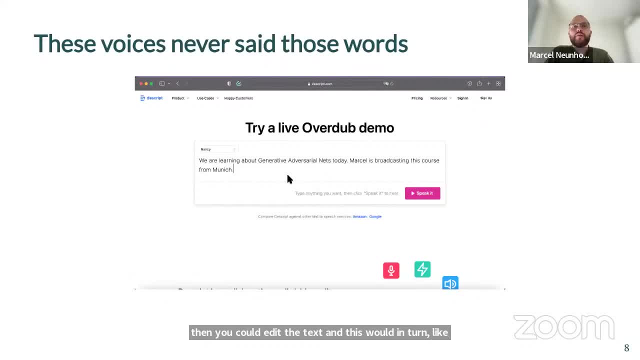 end up to be like edits in the actual voice recording or in the actual um video recording in your own voice or like this. this overdub, where you can try a demo on on their website, is like you need like a professional sounding voice um to talk over, um, like maybe a video um, and so you. 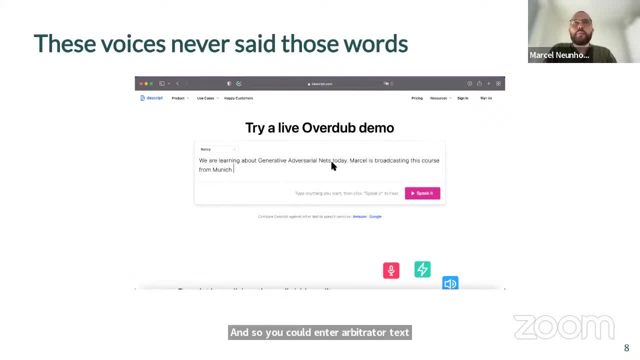 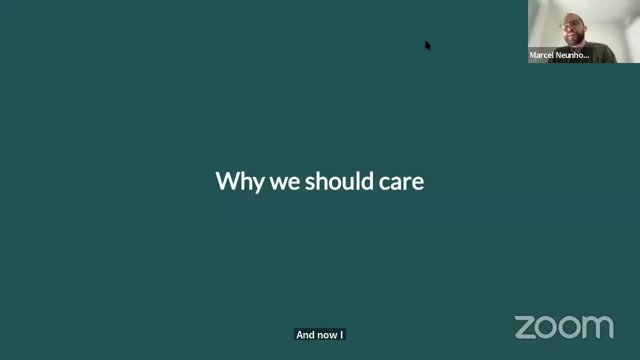 could enter arbitrary text and it will produce um very, very impressive um results. so this is all nice and shiny, um and uh. now i will put my social scientist hat on for for a little, uh, a little bit um why i think um, we should care as social scientists, as data scientists, um who also think. 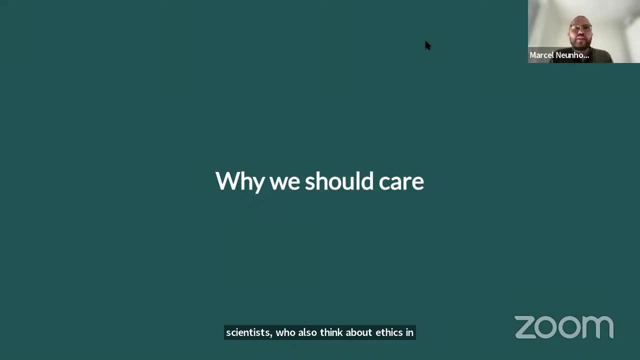 about ethics in research or in our applications and um, because we care uh, i think we should also know what's what's behind this like from the ground up and uh build an understanding of um how those uh like wonder machines um work um from scratch. um so, unfortunately, like that um. 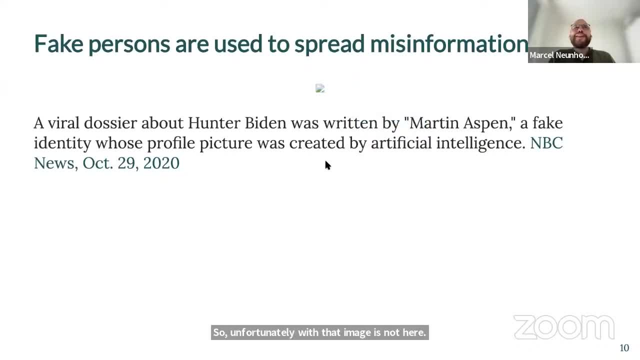 image is not here. okay, that's weird, um, but like for, for example, um, of course, like you saw those nice pictures um of people, you could start to um, create fake personas, like you can have a picture, but, um, no one is no one real, uh, so no one can sue you. 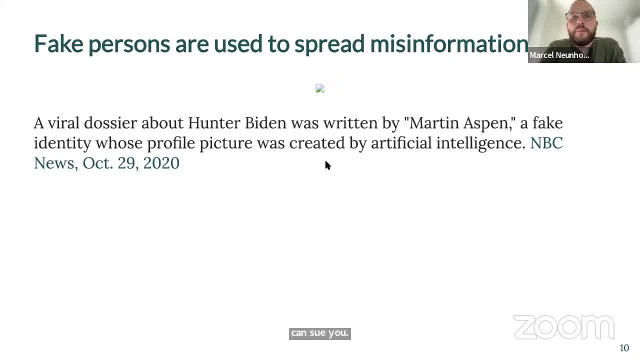 um and in the 2020 campaign in the us. uh, like a lot of the um rumors and- um- let's call it fake news around. hunter biden: uh was actually put out on twitter by a fake persona that had like a gun. generated um a profile picture and this was a big story like pre-elections uh. 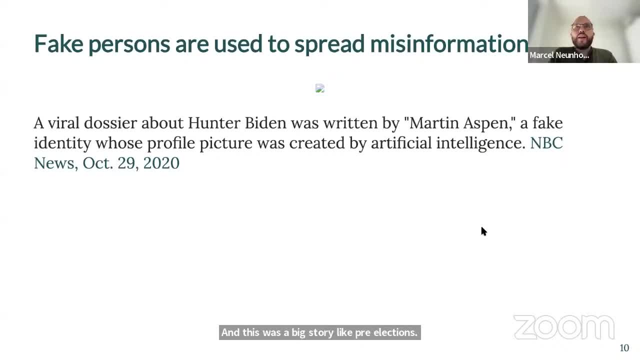 at nbc, like a big tv station in the us, um, how, where they tried to reconstruct, like who's behind that fake persona. so i guess that's like showing like the the um, no one um that has uh a fake persona. um, i mean the, the idea that the uh the fake for. 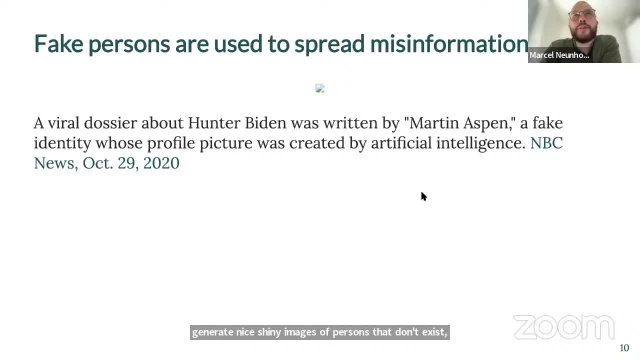 uh, there's always like two sides to a coin, right like, you can generate nice shiny um images of person that don't exist, uh, and that's that's really cool at first sight, but, like, at the same time, this technology can be used to mislead people, right? um? so people on twitter think they interact. 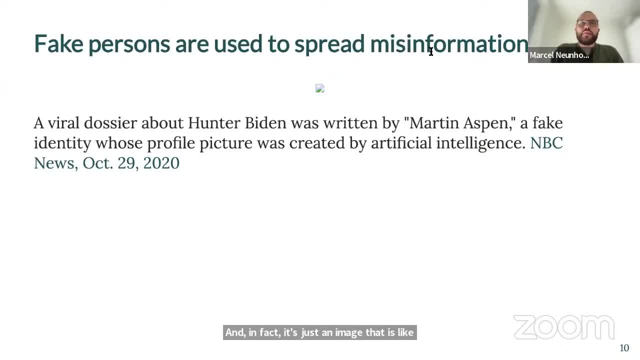 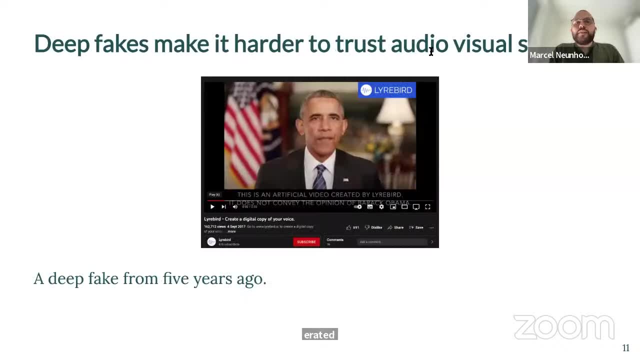 with someone real that they have never seen um and uh. in fact, it's just an image that is like, is like, generated by such a generative adversarial net. And it gets even worse, like if it's not just images but if it's videos and audio visual content. 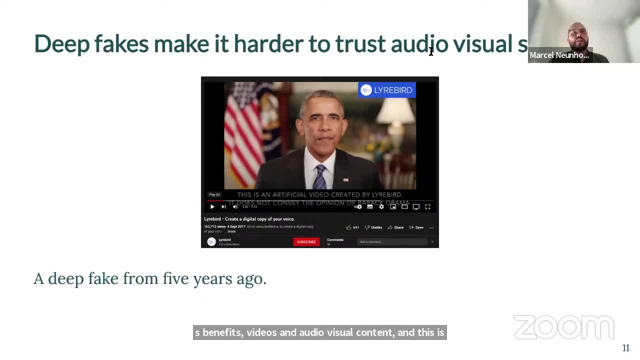 and this is an example from actually almost five years ago And it's still pretty impressive- where, like this company, Lyrebird that still exists- created a deep fake of Barack Obama saying like the words that the programmers at this company wanted to say him. 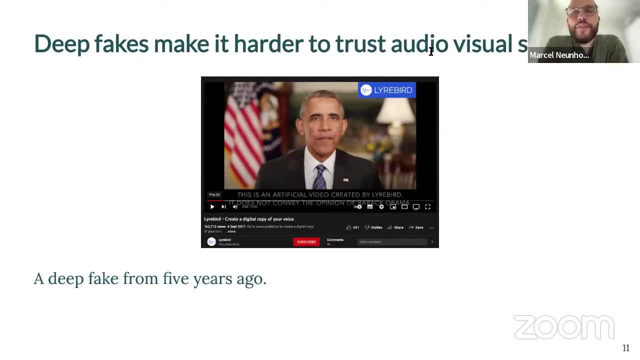 And they make it very clear that this is a fake and like. also. the message is such that it like is like: yeah, It's a warning for this technology And you could easily see how such deep fake videos could be used to influence opinions. 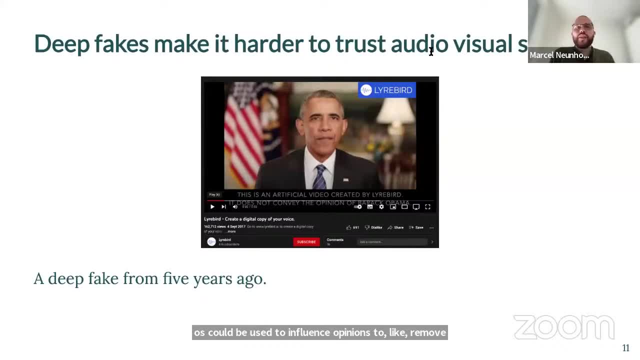 to like when people say something they never said, which, in turn, could lead to real life like outcomes, good or bad. And if you go and look at this YouTube video, it's pretty amazing, like what the technology could achieve five years ago. 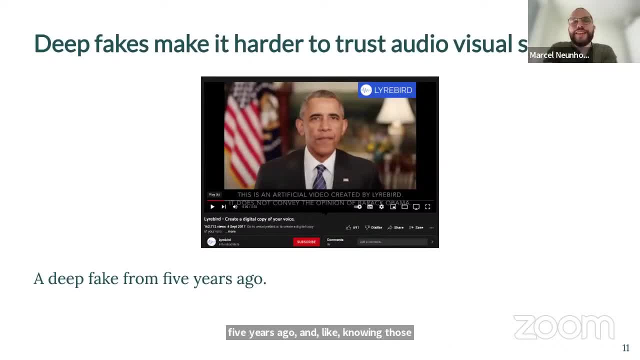 And like knowing those innovation cycles and like timelines and computer science and computer vision in particular, it's not too hard to see, like how much scarier or how much better deep fakes became in the meantime. So like, yeah, it makes it harder for us to trust all your visual sources. 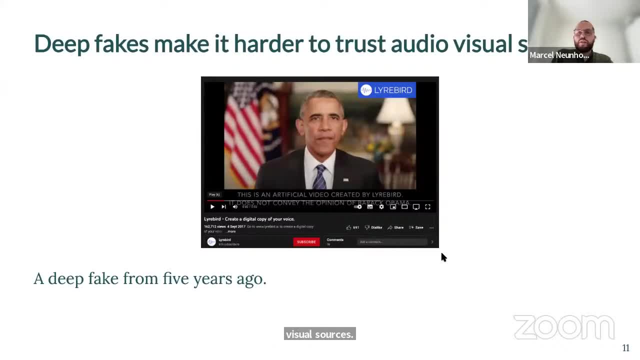 And there's also like a lot of research going on actually to make sure that Gantt generated content could be identified, like trying to figure out how to do that. So yeah, So yeah. it makes it harder for us to trust all your visual sources. 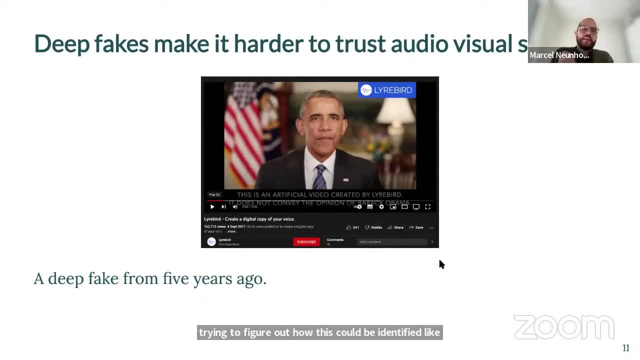 And there's also like a lot of research going on actually to make sure that Gantt generated content could be identified, like trying to figure out how this could be identified, like, think of it like this: Previously, like there was a lot of research. 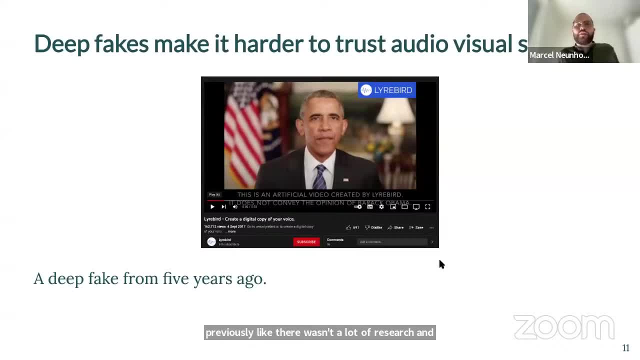 and basically data or image detectives trying to figure out if an image got tampered with, and they tried to develop techniques to like basically reverse engineer, to figure out, like, whether a Gantt was used, And to be able to do that, if that's your goal. 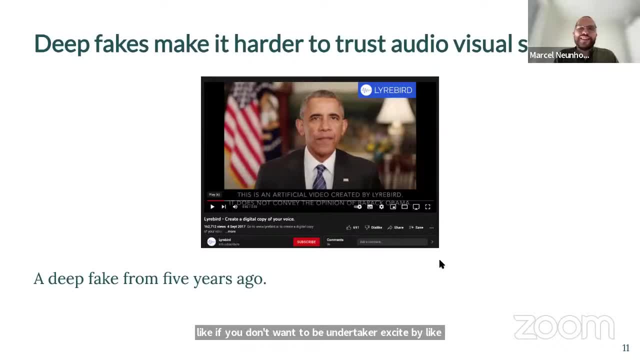 like if you don't want to be on the faker side, but like on the detective side and identifying, like Gantt generated content. I think it is also necessary, or like a very, very good idea, to actually learn how Gantt's work. Oh, by the way, I probably never introduced like this. 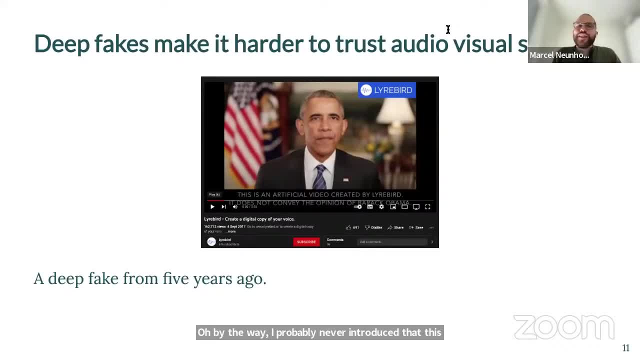 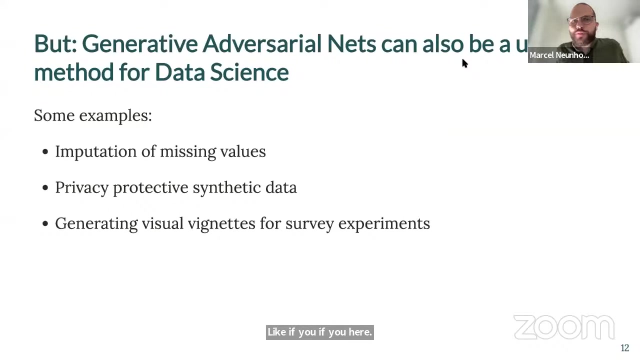 but Gantt is a big acronym, So Generative Adversarial Nets or Generative Adversarial Networks are typically just abbreviated with G-A-M and like it's called Gantt, like if you hear it So that's like the bad or maybe also like interesting examples. 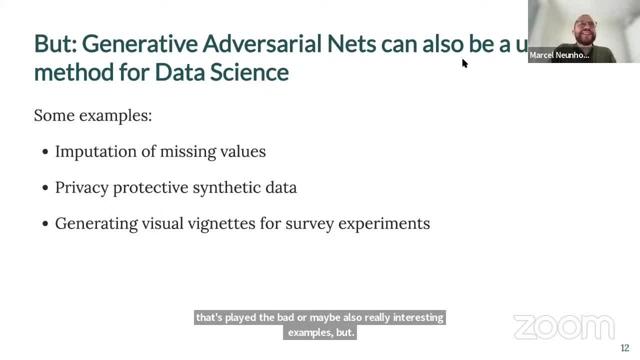 but- and this is why I stayed- Generative Adversarial Nets can also be a very useful method for data sciences. So some examples of applications that have actually been published is, for example, the imputation of missing values, Like, if you have like, the system of neural networks. 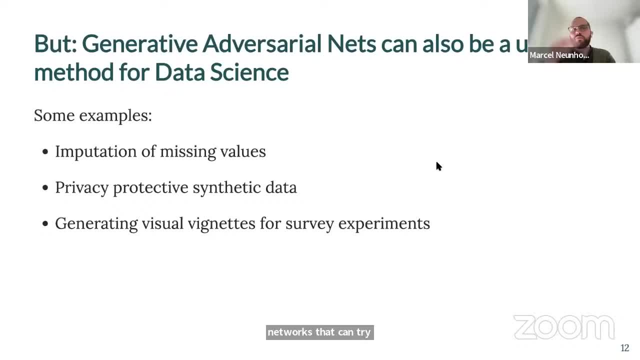 that can draw new observations, new values from like some underlying distribution. it makes sense to like think about how this could be used to impute missing values. So if you have like a data collection and some values in your spreadsheet or in your data set in your database are missing, 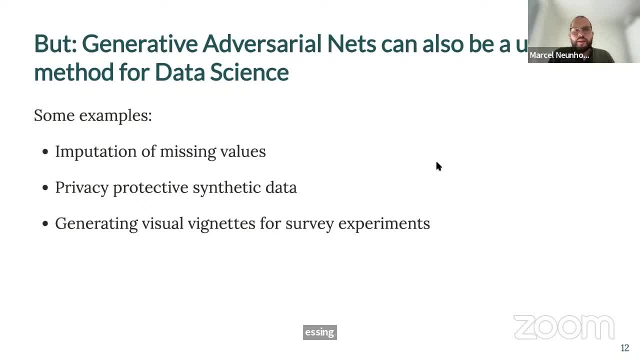 you typically don't want to throw away like the whole case, because you still have useful information in there And this, of course, would bias results And you want to use like a good way of like figuring out what the values could have been like if they were observed. 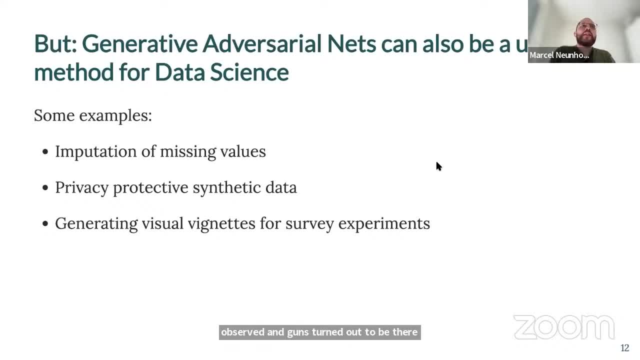 And Gantt's turned out to be very useful for that. Then another very cool idea is like that you could use those Generative Adversarial Nets to make a copy of some original data set, like if you have a survey that you collect. 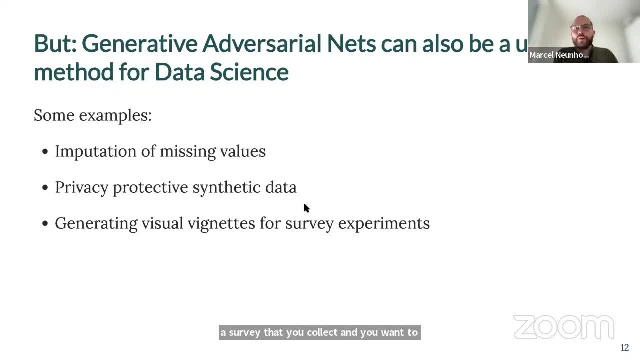 and you want to upload it to a replication archive, or you want to share it with a business partner but, like privacy laws prevent you to actually share the original data, You could come up with a Gantt that creates a copy of that original data that is very close and like. 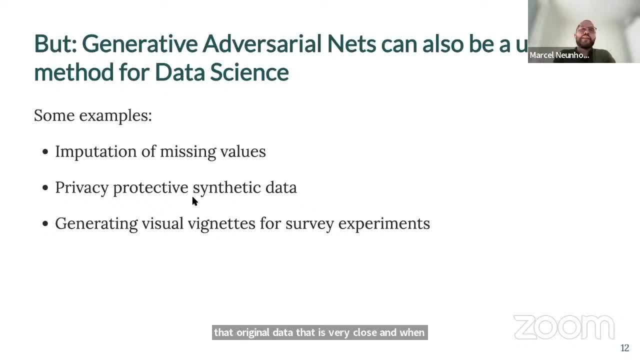 the statistical like properties of that copy should be very similar to the or like, in the best case, should be very similar to the original data And then you could pass on like this synthetic copy And if you build in some form of privacy guarantees, 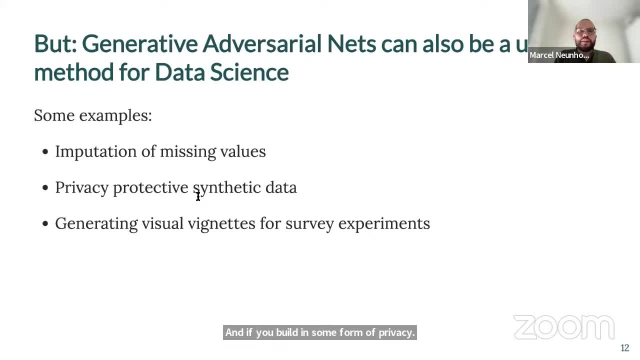 like your like, the problem of sharing the data could be solved. You can actually share it freely without harming anyone in the data collection and without going against any privacy laws that you might have to comply with, And more in the original line of the like. 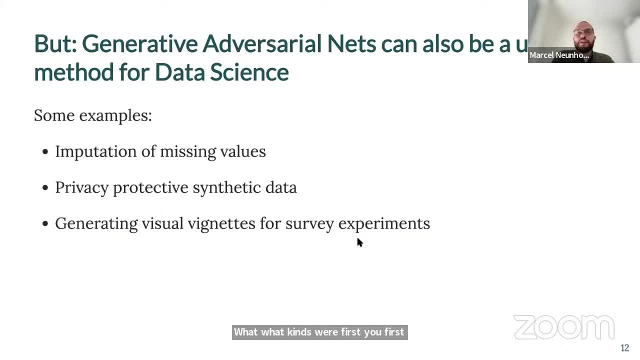 what Gantt's were first used with like image data. There is some research out there where they use Gantt's to generate faces of, like visual features of persons and use those faces, or those persons- personas, in vignette studies, like in survey experiments. 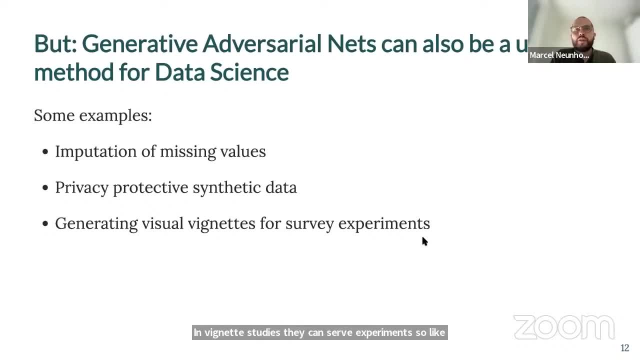 So like they want to. for example, if you wanted to figure out like, if some trait like helps to get to be voted for in some country, or if some other traits are discriminated against, And it's very hard to actually use real people for that. 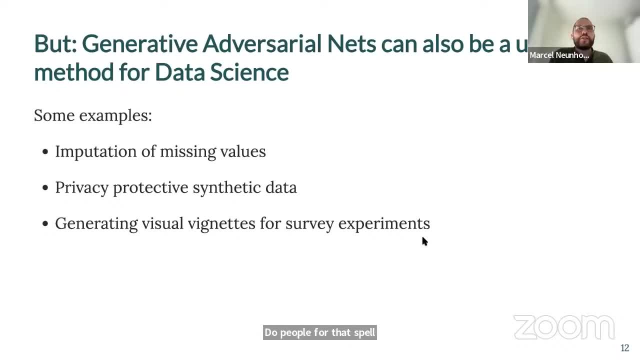 Especially if those people maybe don't even know that they are part of such a survey experiment. So, coming up with like you know, like, if you want to, coming up with generated images that then allow you to tune it to the way that you need it for 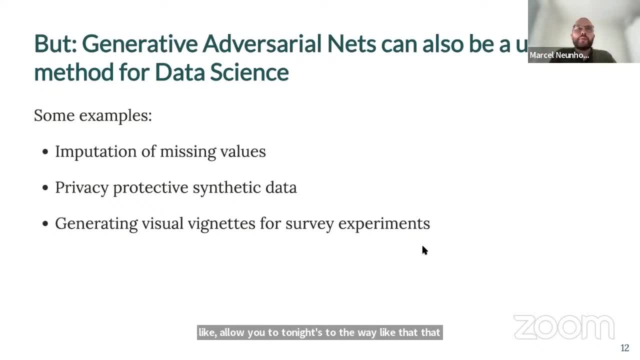 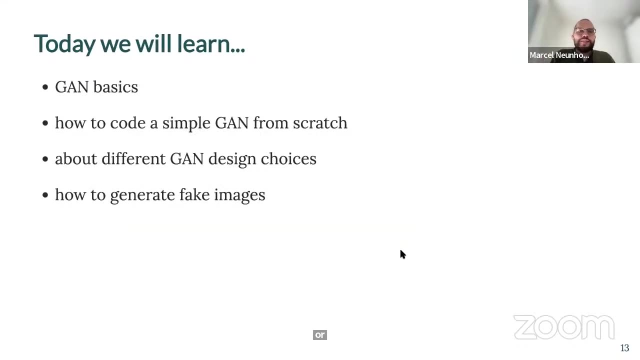 the survey experiment and then using them as a stimuli in an experiment is also a very cool idea for the use in data science or social science. All right, so that's like the short hype intro. I hope like it's generating a bit of hype. 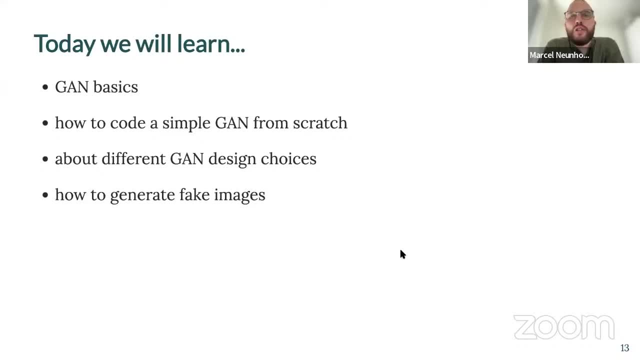 And now I will give you an overview what we will learn until 2 pm today. And we will start with, like, the very basics of GANs, first on slides, and then we will code a simple GAN using those basics from scratch in Torch and R. 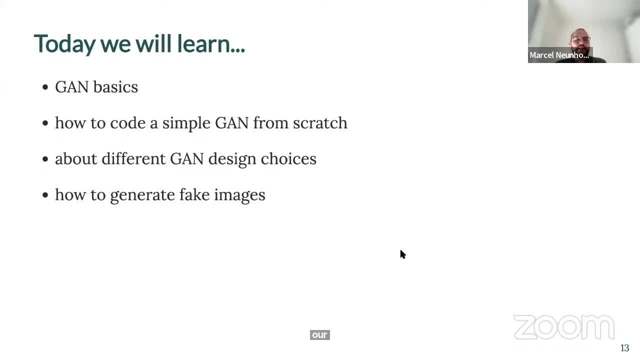 And when we go through that, we will see that at different stages of like writing or coding up that GAN, we have to make different choices And there is like many, many different design choices that you can make along the way. And so in the second half of the course – so that's gonna probably start after the break – 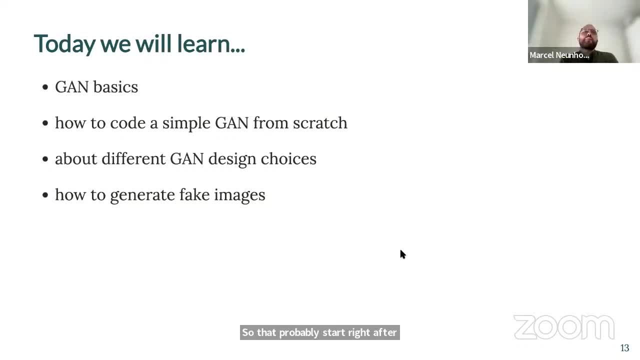 we will learn about, like those different design choices in depth so that you understand where the current research frontier is. I have lots of listed GAN models here, A few subjects, recent references in there, like if you want to catch up on what what GAN research is doing. 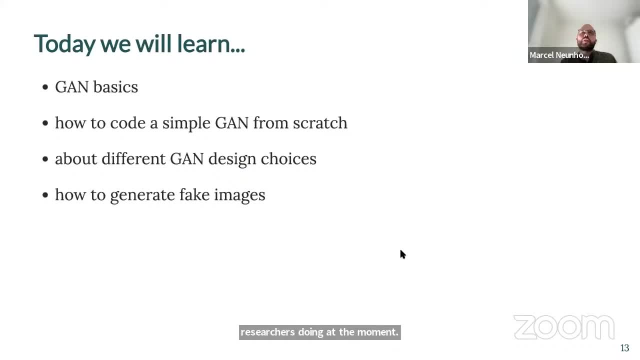 at the moment and also think about and talk about like, how those different design choices can be implemented. and then one example of like making different design choices is then, instead of like our simple GAN, where we will really just use simple tabular data, how we can adapt, like a GAN, to generate fake images. 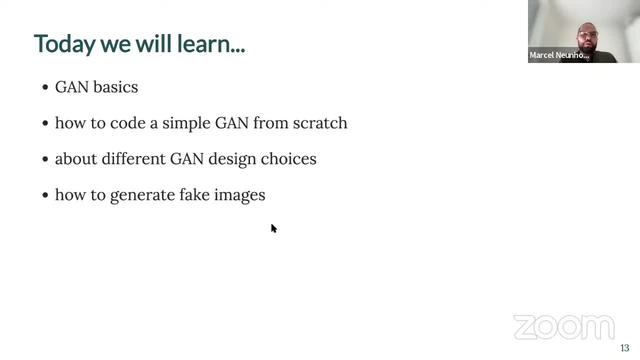 and actually implement that as well. but I hope no one expects to see like high definition, like faces, as we've seen in the intro, because, like the time we have to train today is just not sufficient to do that. but we will see faces like we will learn faces. 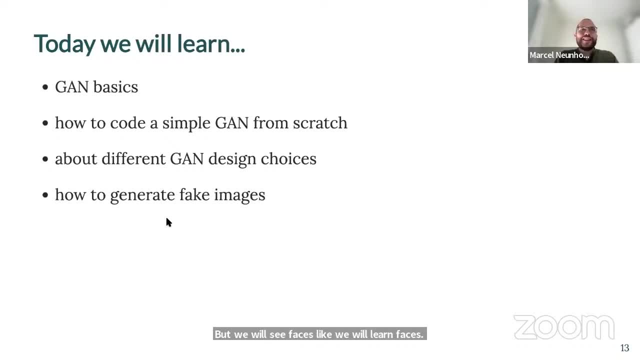 but just not enough, not as HD as as the ones in like the intro here and then, if time permits it and I hope we can, we get there- I have like a section on my work with GANs and how this could be used to generate privacy protective synthetic data. 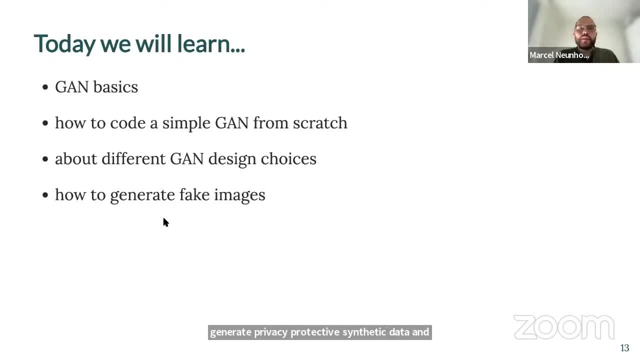 and like. in doing this, there's like two, two interesting concepts that could also be useful beyond that application, and one is how to train with formal privacy guarantees like neural nets and, in this special case, generative adversarial nets, and then also how to post process the output. 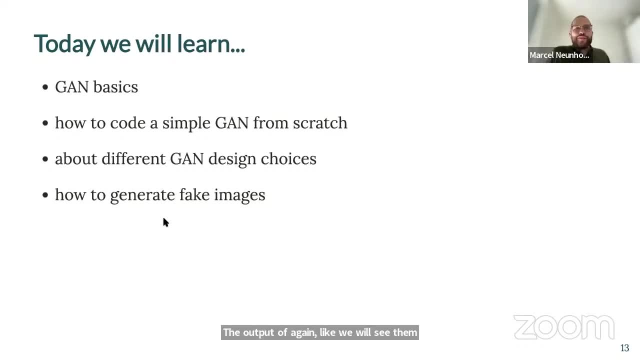 of a GAN, like we will see, that training GANs can be hard or is definitely harder than training most machine learning models. that that you might have seen before. all right, are there any questions? at this point, like I just see like the number in the chat running up, but I'm not sure if it's. 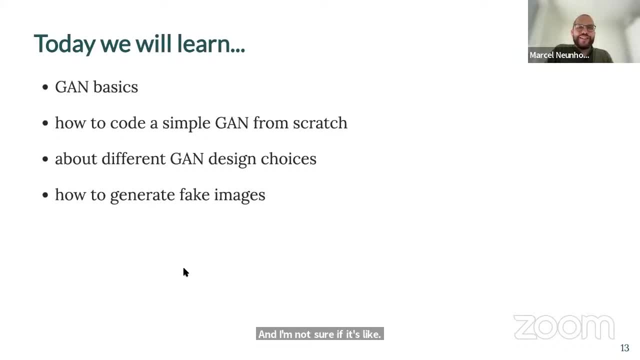 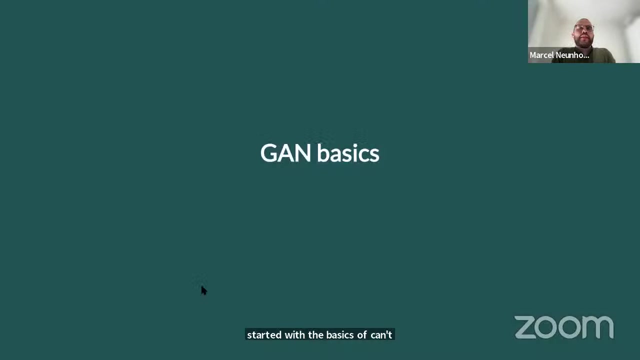 like anything that I should address here. okay Okay, Oh Okay. If that's not the case, we can jump right in and get started with the basics of GANs, Alright, So this is a little bit more of a demo. 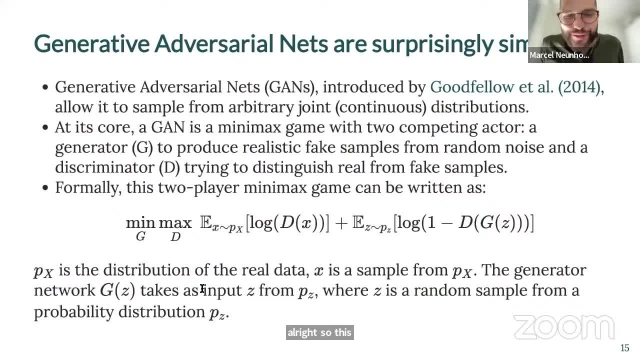 Okay, a lot of text and I tried to like- I won't read the text to you, but I tried to use the illustrative example- that Goodfellow et al. so that is Ian Goodfellow, and he was then, like in 2014, a PhD. 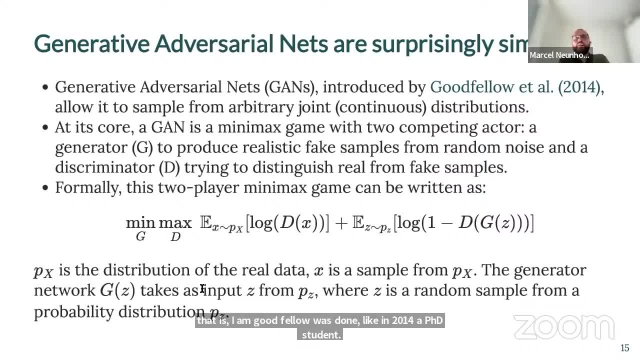 student in computer science and he came up like with those generative adversarial nets, like within a research group. and so basically the game- and that's where the adversarial in generative adversarial nets comes from- is between two different neural networks, where you can think of one of those networks as 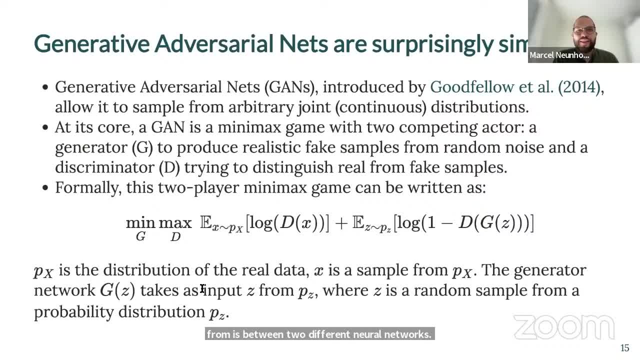 like money counterfeiters, like a group of bandits who want to fake money like, let's say, euros, and a discriminator, like a second neural network that you can think of as like the police or like a financial investigation unit- wants to, like, get 100 percent of fake money off the market. basically, they want to detect fake 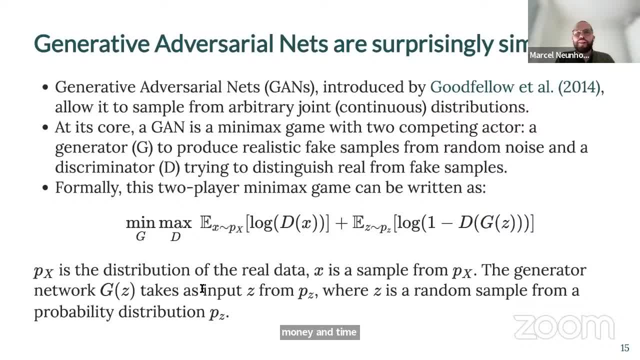 money and punish the bandits if they like get caught with fake money, and those two groups they basically don't ever really interact. so basically the uh group of bandits comes up with like a first guess of what and they don't see actual money. um, comes up with the first guess what like uh money, uh, or like a 10 euro bill could look like. 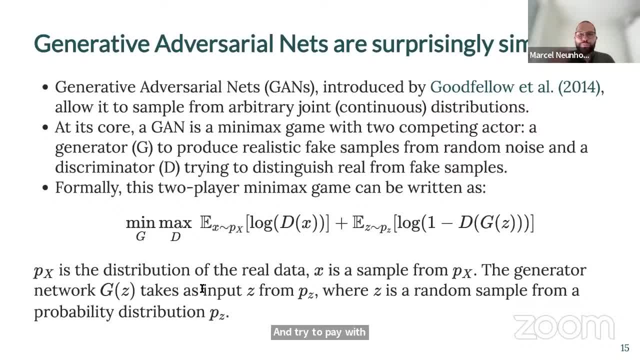 and try to pay uh with that or try to pass it, basically uh by uh, the police, um, and the police get to see, like, the fake money that those bandits generated and, of course, real money, and they can compare those two um and um. then basically, uh, give a feedback, uh, to the bandits, um, in the form of, like if they 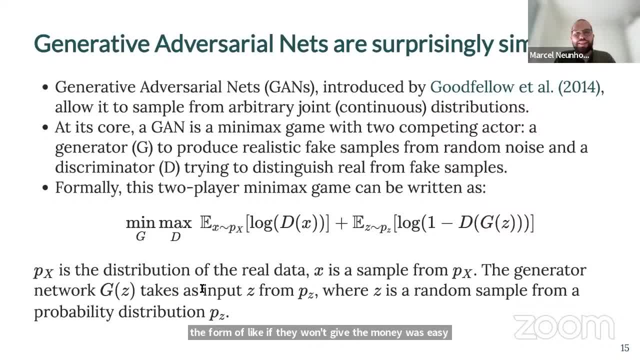 uh, like if the money was easily, it was easy to see, for uh the police uh to see that, uh, this is not real money, then they will lock them up, so they will punish them. and if the money is good enough to pass as real money, uh, then the bandits will also know right, because then they 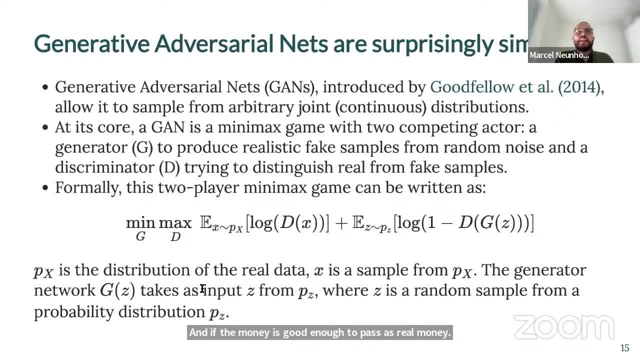 could pay for goods using um that, um that fake. and so those two players like the bandits and the police. they play this for like uh, multiple iterations. so bandits come up with fake money, try to pay something and get them, uh, like the feedback from the police, who compares um the real. 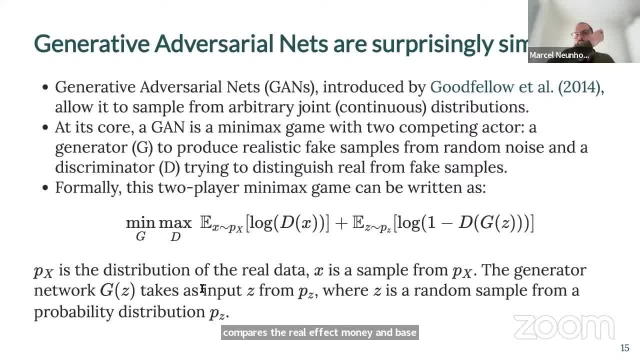 fake money and um based on that feedback, um, they try to improve and and get better, but at the same time, the police also tries to get better. right, like they see more and more real money, they see more and more fake money, so they can also learn um better, um, like what's what's real and what's fake. 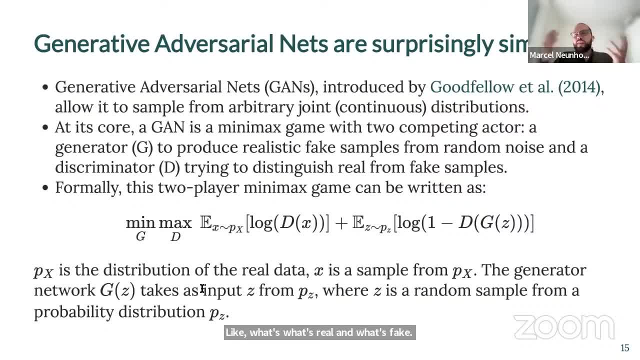 and this is like a yeah, like, like a game, like if some of you had some kind of game theory. um, like, this sounds a lot like those games in game theory and it turns out, actually, that this game has a nash equilibrium. um, like an equilibrium. uh, where? uh, this game basically? 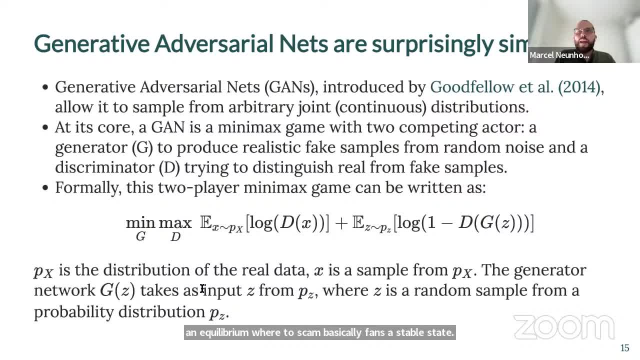 finds a stable state, and that's the case when, as soon as the bandits generate money that, like, the police can't distinguish uh from real money anymore, like if the police is uh like maximum uncertain about, like if it sees like real or fake money, then uh this, uh this game will enter a stable state, um where, like both groups, 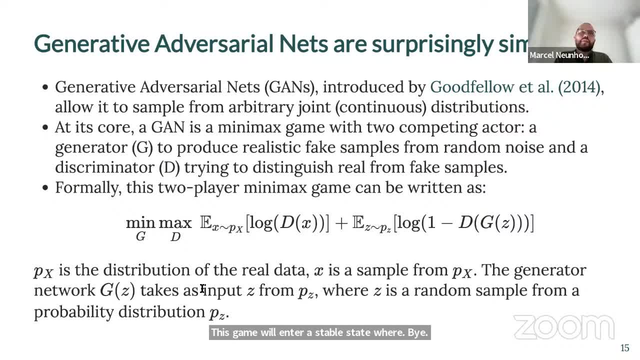 won't learn anything anymore, right? uh? because, like, basically, the police is just random guessing um what's fake and what's real, and because that's just a real random guess, as a feedback, uh, the bandits also can't learn anything anymore. and if we reach such an equilibrium, uh, that basically means that the 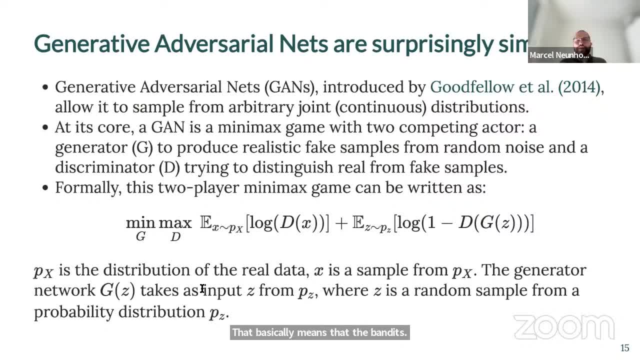 bandits sample, like their fake money, like they produce fake money um from the universe of real money, right? so they sample fake data from the true underlying data distribution and therefore it is impossible for the um police to know. um, unfortunately, like this, this nice theoretical insight that uh, like in a, in this equilibrium, like the generator, the group of bandits will actually learn. 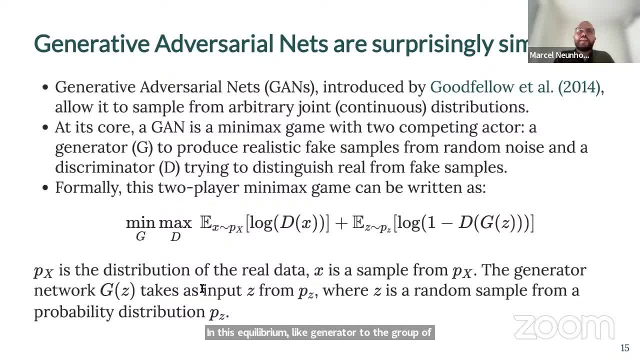 to sample from the true underlying distribution. um has the downside that uh to to actually prove that such an equilibrium exists, uh, we need um, both the discriminator and generator, to have like infinite capacity. so they must be infinitely powerful um, which is of course not um possible in in real life. however, um in that paper, uh. 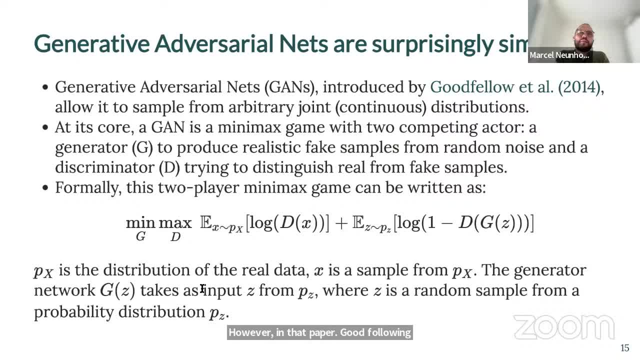 good fellow at all, showed that uh like neural networks um can be powerful enough to get to maybe like a local equilibrium or like somewhere close to an equilibria, to actually generate uh like images or fake money um that looks like to human eyes, um very, very good and appealing, and this is really cool, um, and like one of the the major 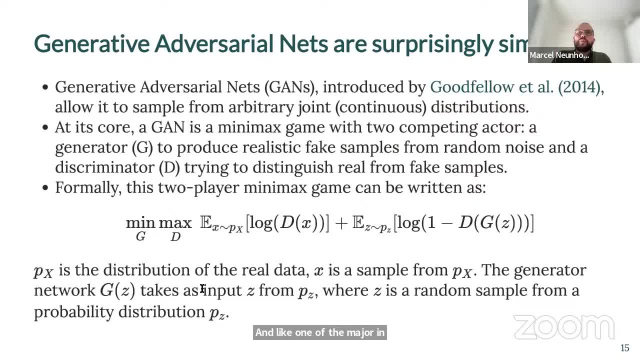 insights or one of the major um breakthroughs in this formulation of the problem is like like that: before, with generative models, computer scientists and statisticians tried to directly model like this like some generative model, And this turns out to be really, really hard right. 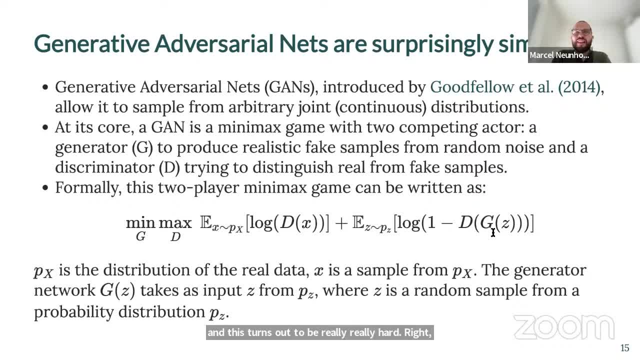 Like to come up with a generative model that produces data that is indistinguishable from like your real data is really hard And it's like what they did. basically, by introducing this discriminator, the police, they turned like this learning task of a generative model. 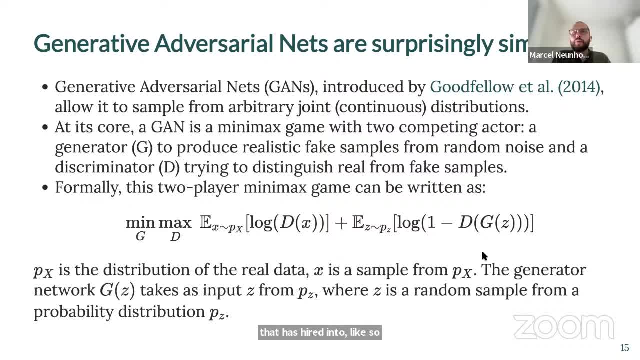 that is hard into like a supervised learning problem, right? The discriminator gets to see real data, gets to see fake data. So you have labels, you have like, let's say, the images, or like the data as features, and then you can try to distinguish. 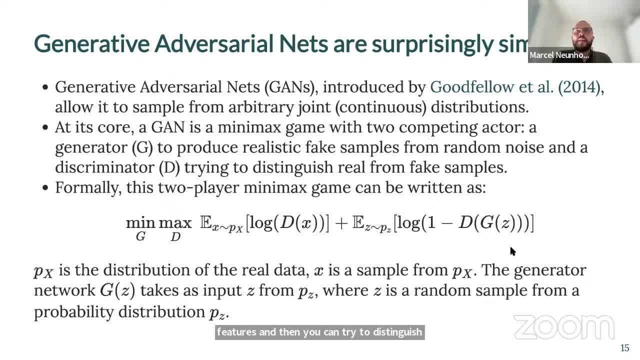 or try to discriminate between like real and fake, And this is surprisingly easy, and setting them up in this adversarial manner actually produces a system that makes use of like discriminative through a learning using the discriminator to update a generative model. So this is a very powerful thing. 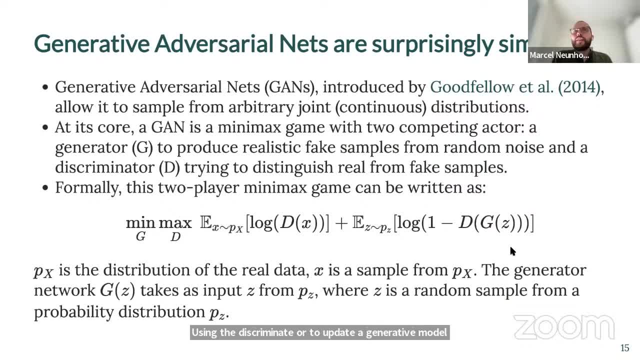 So this is a very powerful thing, idea um, and for that reason um like is cited very heavily and there's so many different um guns out there and at the same time, it's surprisingly simple, right like. if you look at this um formulation of the game between the police and the bandits in like math terms. 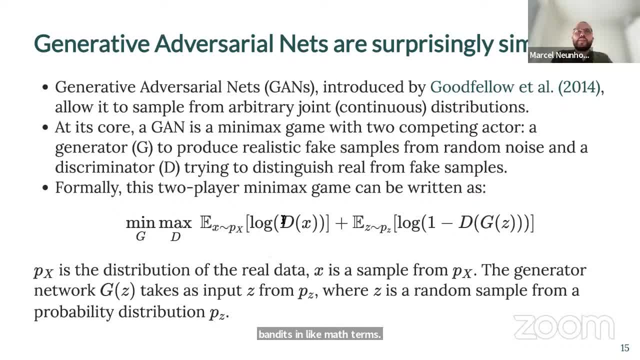 you have, uh, two terms in here. um, the first is basically the expectation of discriminator scores over real data and the log of that. so the discriminator puts out like a probability between zero and one whether that example is real, and then you log that and take the expectation over all the examples that you see. 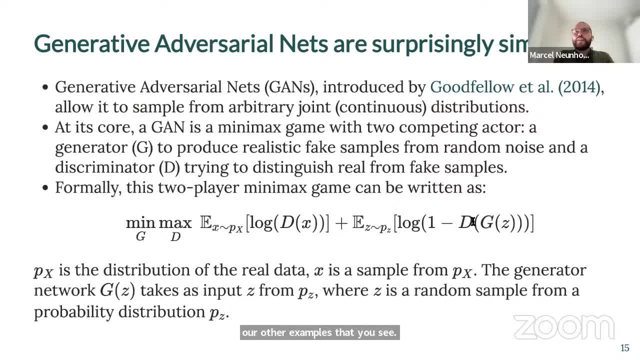 and um like the same thing. basically, uh for fake samples. so fake samples are generated by putting a random noise c through a generator and then just applying the discriminator to that and using one minus um, uh like, uh the probability here and log that uh. so basically this, uh like it's called a value. 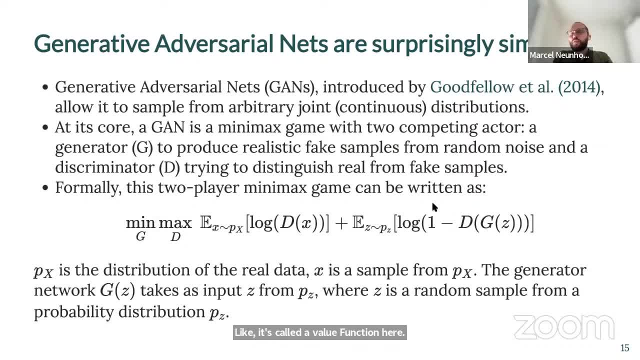 function here, um, but in classical machine learning models this would be like similar to the, to the loss function. it's very closely related to binary cross entropy loss or logistic regression. um. so, um, you, you might have seen like something like this before and now, as we have like those two networks. 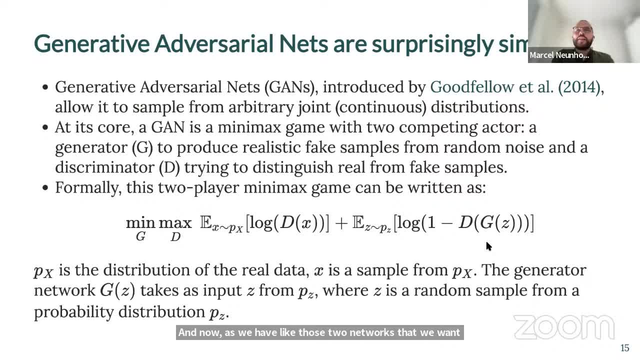 that we want to learn. um. like one tries to minimize this function. uh, the generator um tries to update its weight such that, like, the value of like this function is minimized and, at the same time, the discriminator tries to maximize this function. um, and this is how. like this adversarial game. 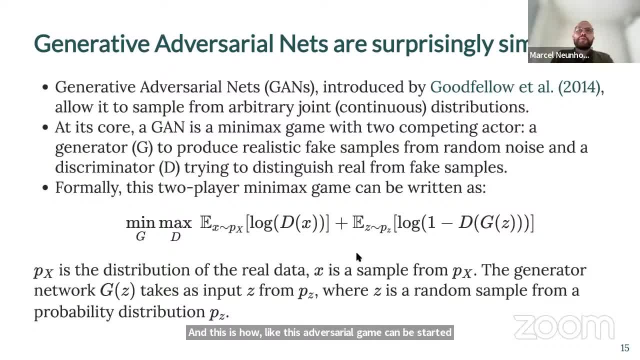 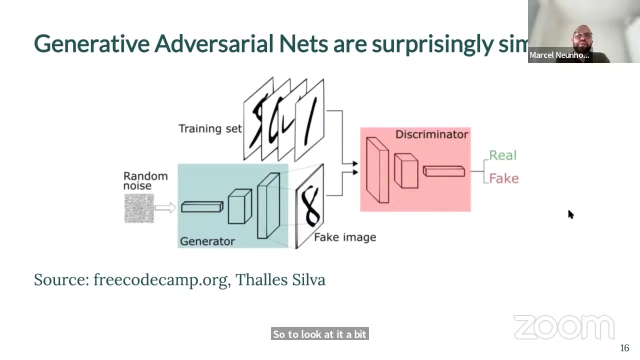 um can be started in um, like math terms, um, and since they are playing against each other, we, we can also not reach like a minimum or a maximum right, like we can only um try to find like this a stable equilibrium state. So to look at it a bit in a bit more visual terms, 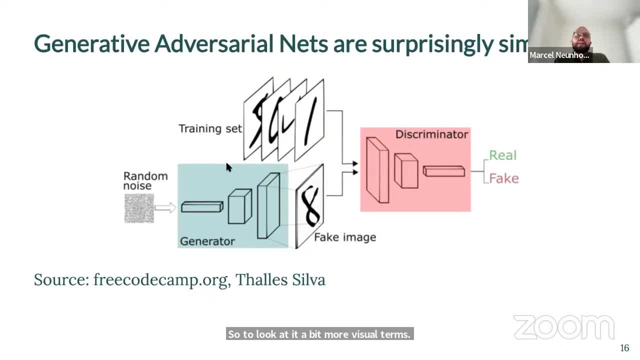 what you can see here is basically the two networks that we need, like the generator here and the discriminator here, And like all the inputs to like those networks. So the generator only gets- really gets- random noises input, And you will see in our coding exercise. 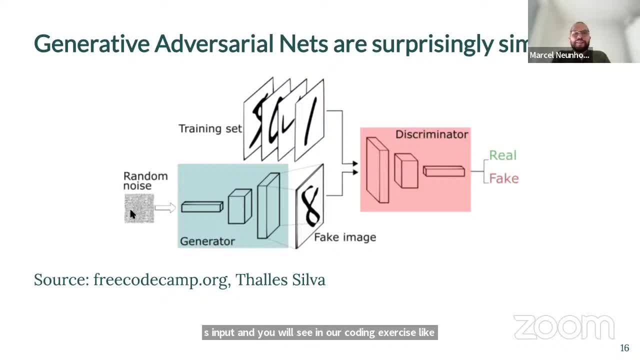 like that. it is really just random noise And I'm always fascinated that, like this network learns to produce something useful out of this random noise that is parsed like to this generator neural network. So here this visualization is probably some sort of like convolutional architecture. 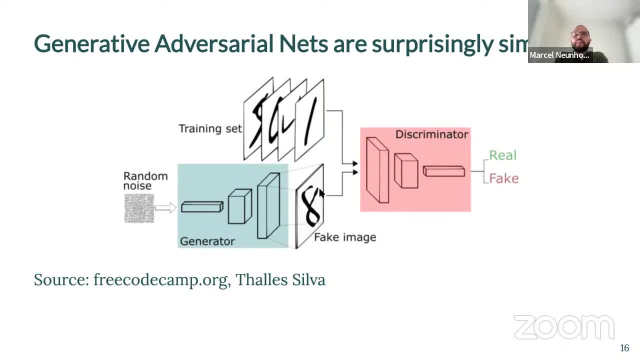 but like we will talk about architectures later- which makes sense in this example because, like this, is using MNIST handwritten digits like as an example here and tries to produce like a fake number in this example, In this case, then the discriminator gets to see: 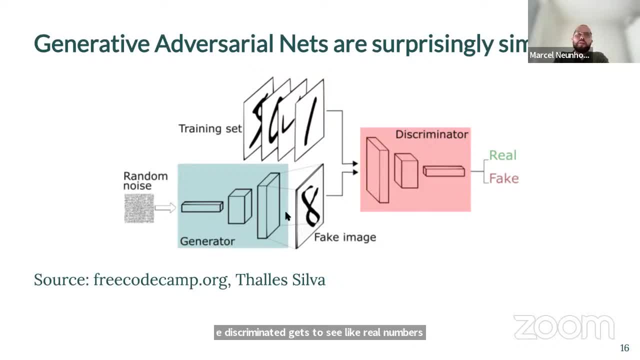 like real numbers from the training set and fake numbers that are generated from the generator, and tells whether like this is real or fake, And then with this feedback, the discriminator is updated And with this feedback also the generator is updated and playing this for long enough. 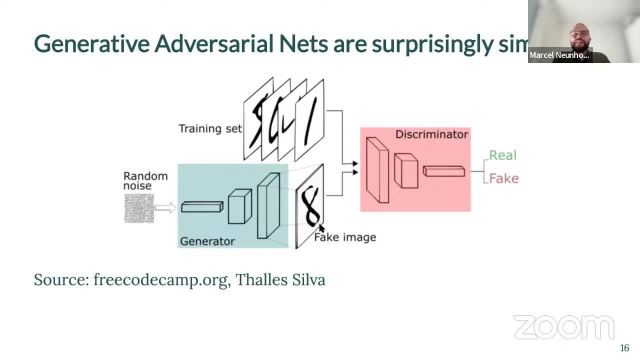 we'll get you to a point where you will actually start to see something that looks like numbers. Marcel, there is a question in the chat: What are random noise for this case, especially the type of noise some characters So like. the person wants to know what exactly. 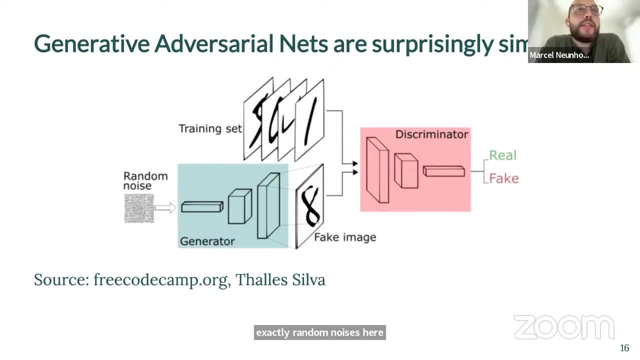 random noise is here. Yeah, that's a great question And we will also talk about it in depth, in like the second section, because it depends on the application, but typically it will be just, let's say, n dimensional vector of independent draws. 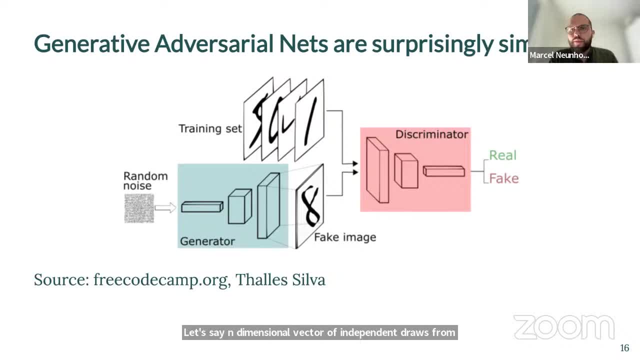 from a normal standard, normal distribution. That's what we will use in the first example as well. So we will have a vector of the dimension that we think, and this will also be like at the same choice, especially if we are thinking about either this: 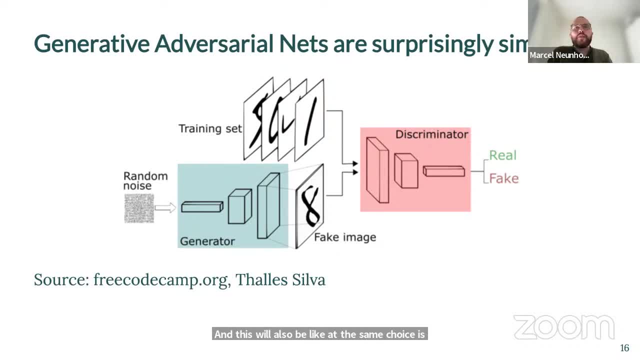 or the other function that should be discrete at this point. But what we'll see is that the distribution for random noise or the function for random noise is very sufficient to like cover basically the feature space of the big data that we want to generate. 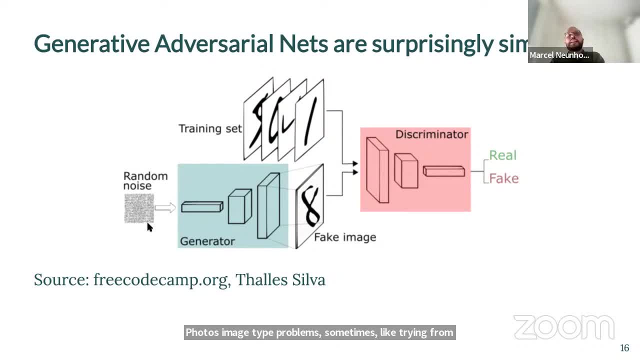 And each entry is just independent, independently drawn from standard normal. often you can bound the input space because you know that the output space is also not unbounded. And then there is some very recent research about how to come up with smarter noise distributions. 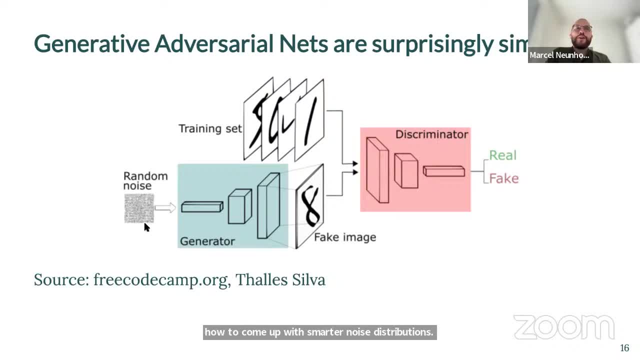 because it turns out that not every point in this latent space. so basically, we set up a latent space that maps to real images or fake images that look like real, And not every point in that latent space is equally likely to produce a good-looking image. 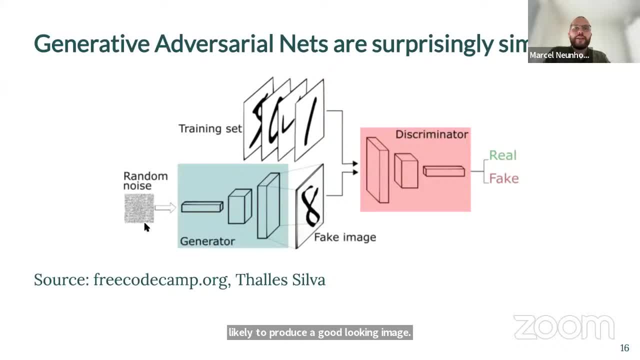 And there is some heuristics about how to figure out what points in that space actually make sense to sample. Yeah, Yeah, So that's a great question And it's a very active area of research, So there is no definitive answer from me at this point. 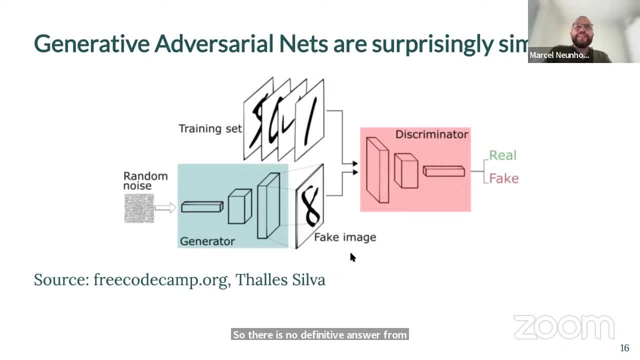 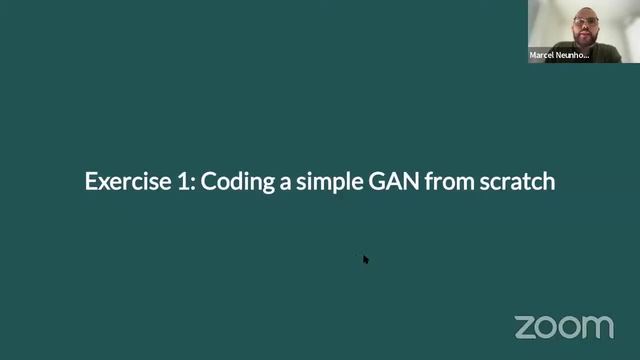 But we will use a vector of the sample from a standard normal in our example. Are there any other questions? If not, we can jump into the Q&A. If that's not the case, we can directly jump in and try to code. 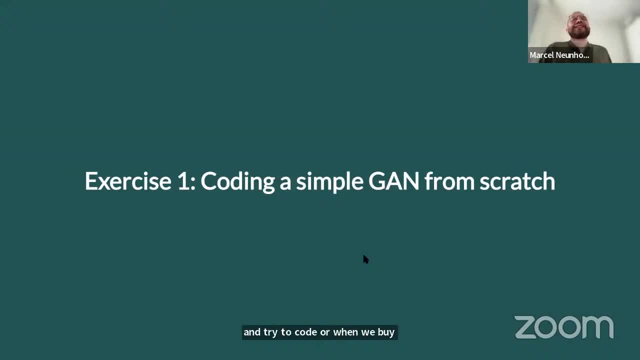 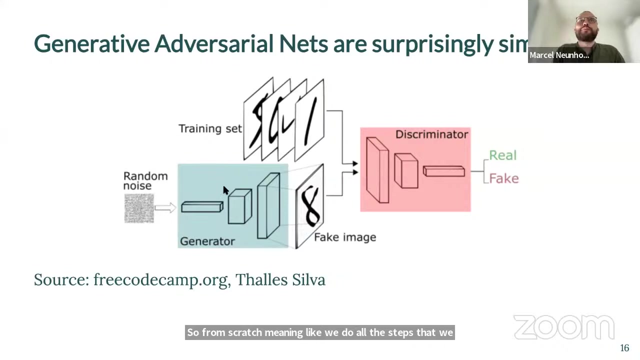 or we will code a simple generative adversarial network from scratch. So from scratch meaning we do all the steps that we can see here in this slide, And we'll just show you the picture by hand. There's no wrapper function around it yet. 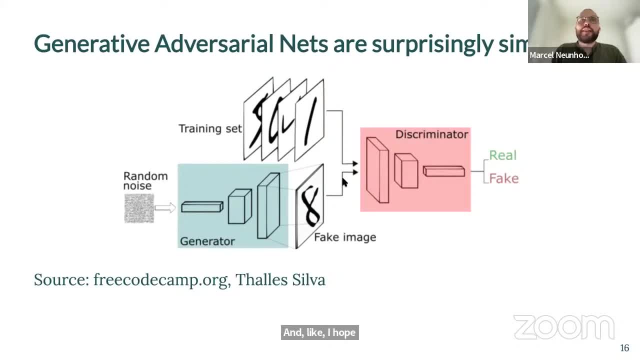 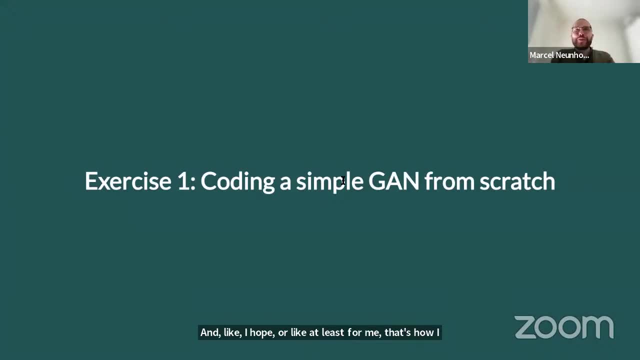 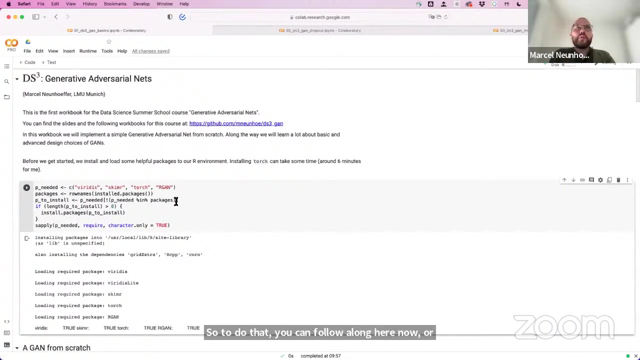 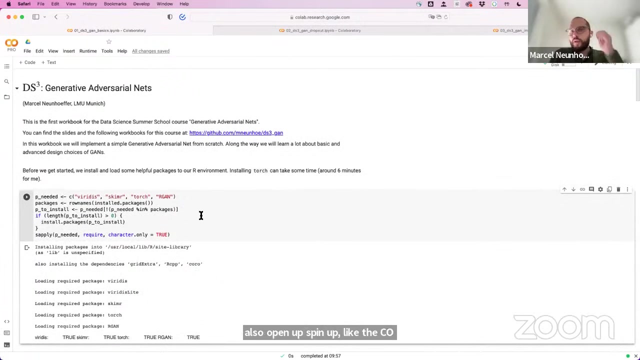 And I hope, or at least for me, that's how I typically learn a lot, by actually going through code and thinking about how those abstract concepts translate into code. So to do that, you can follow along here now or you can also open up, spin up the Colab workbook. 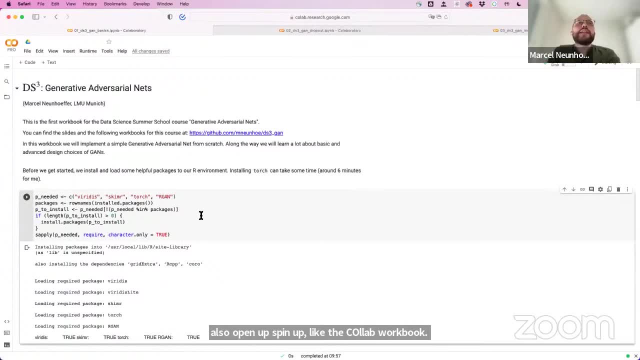 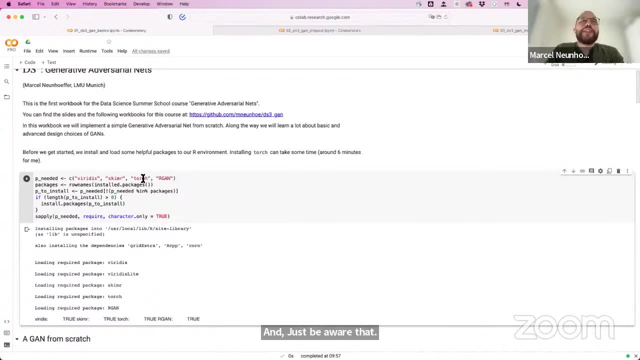 from the GitHub repo And just beware that this first code chunk loading, or installing and loading the libraries, takes about six minutes. So if you want to run this, this will take some time And it doesn't get stuck, And unfortunately Colab is not providing real-time output. 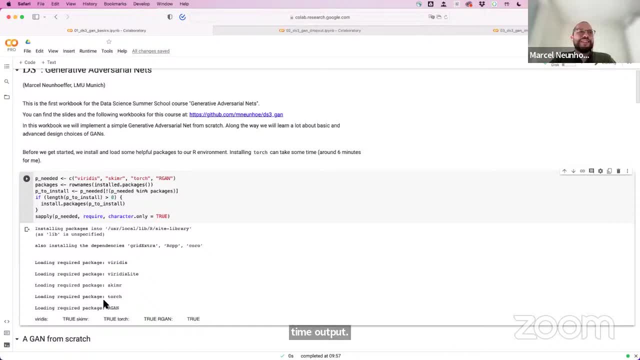 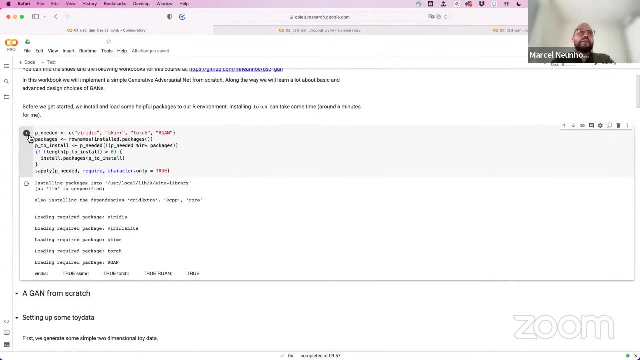 at least not very helpful. So at first I thought, oh, maybe it doesn't reinstall what it should do, But it works And I reloaded it. Marcel, can you Sorry for interrupting? The font seems to be a bit too small for people. 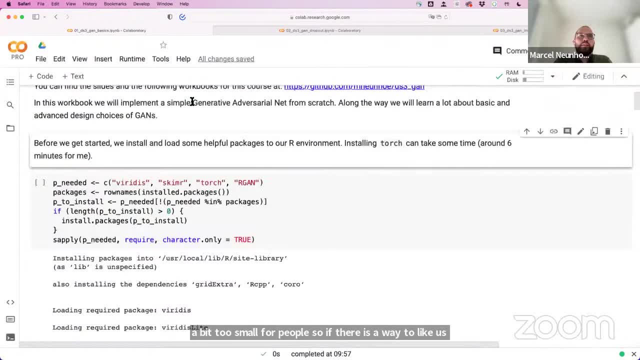 So if there is a way to zoom in, that would be great. Thank you, There is, Yes, There is always a way. Is this better? I hope so. I mean, for me it is definitely better. Yeah, That's good. 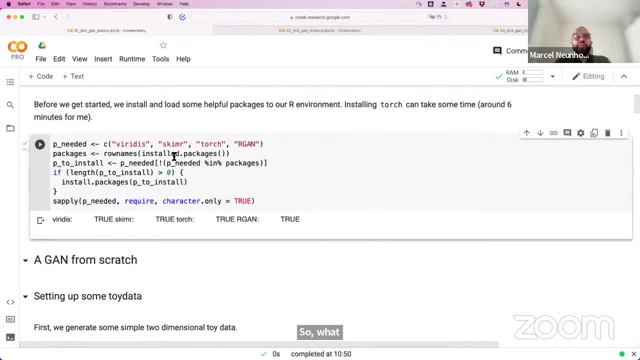 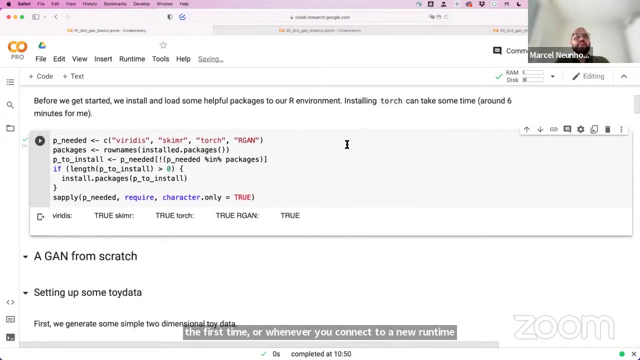 So I preloaded those packages just before starting the session today, So this runs immediately. But if you run it for the first time or whenever you connect to a new runtime- and this will take some time- It takes around six minutes for me. 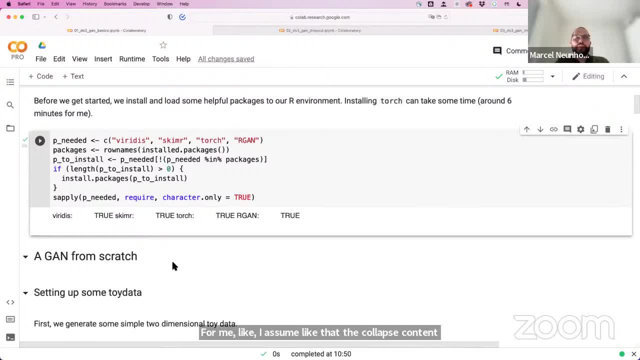 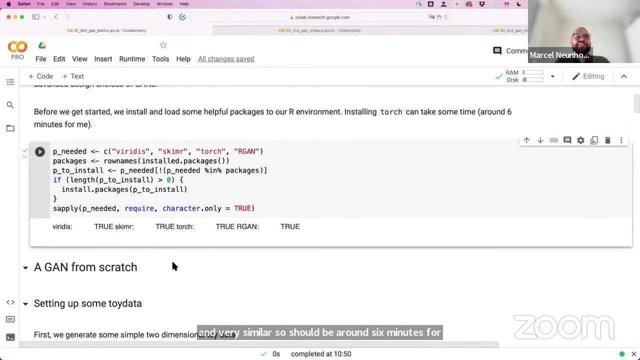 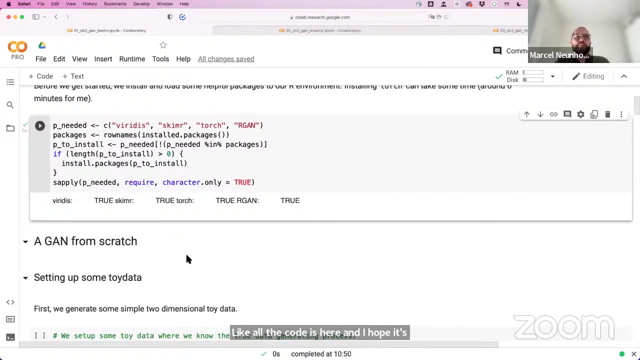 And I assume that the Colab runtimes are very similar, So it should be around six minutes for you as well. So don't worry about that. All the code is here And I hope it's with good comments, so that you can follow along right now. 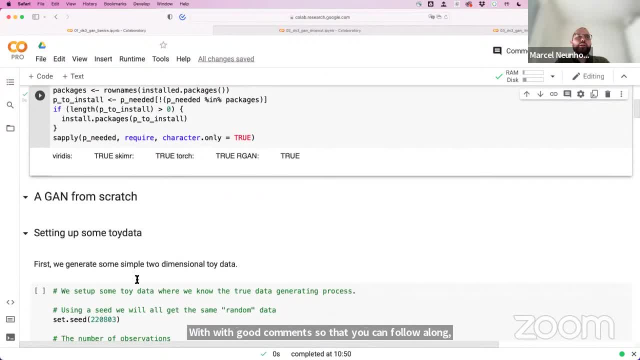 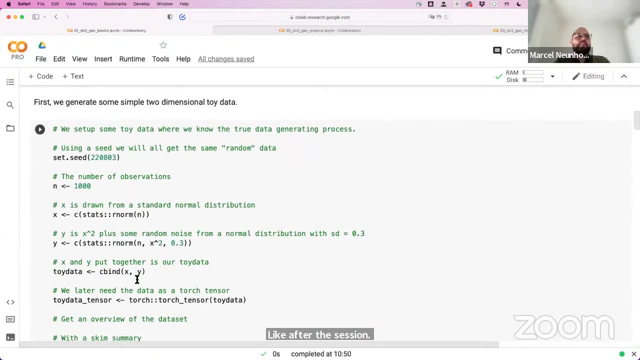 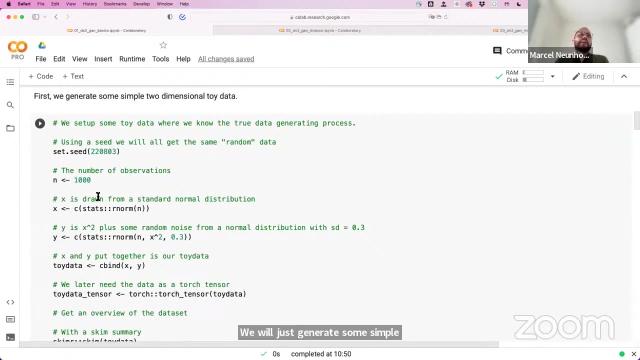 and also follow along when you want to work through it. So I'm going to go ahead and start the session. So in this first code chunk we will just generate some simple toy data, And I'm using R here, But you could certainly do a very similar thing. 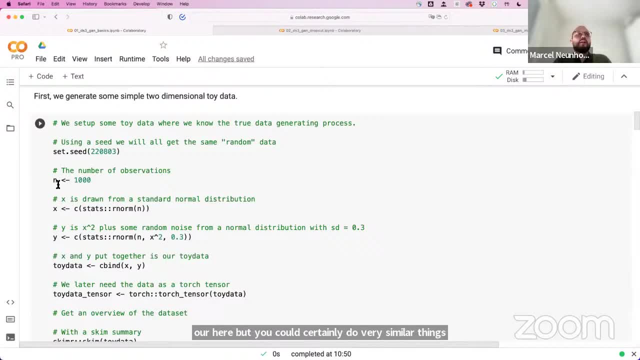 using NumPy and Python. So we just set a seed so that everyone gets the same toy data. We set a number of observations, to be 1,000. And then I will show you what this toy data looks like in a moment. Generate first variable x. 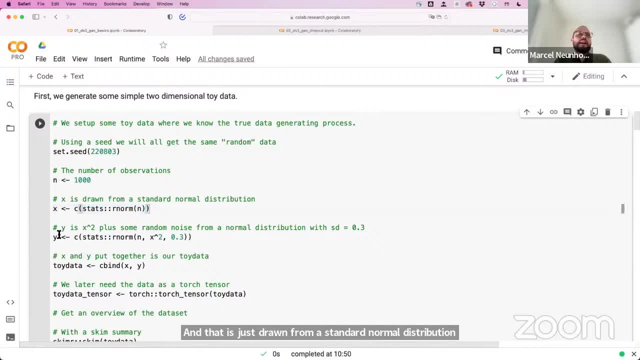 That is just drawn from a standard normal distribution, And a second variable, y, That is a transformation of x plus some random noise, And it is taking the squares of our x's and adding basically a draw, And then we just put this together from a normal distribution with smaller standard deviation. 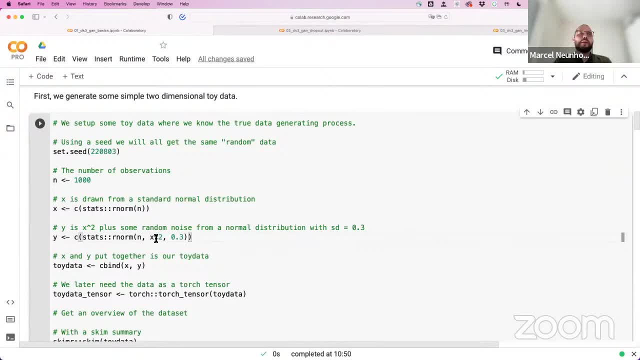 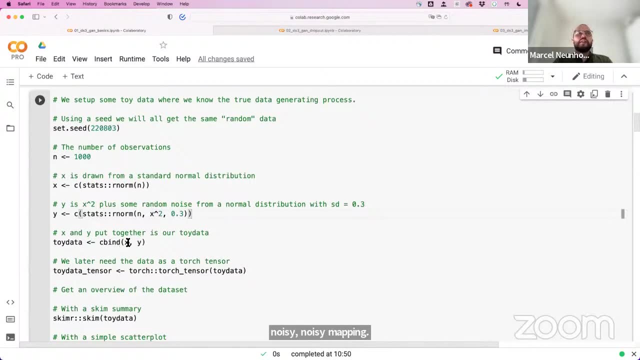 so that we get noisy data. So it's not a perfect mapping from x to y, but a noisy mapping. Then we just put this together in a matrix in R. The first column will be x, The second column will be y, And that's our toy data that we will work with. 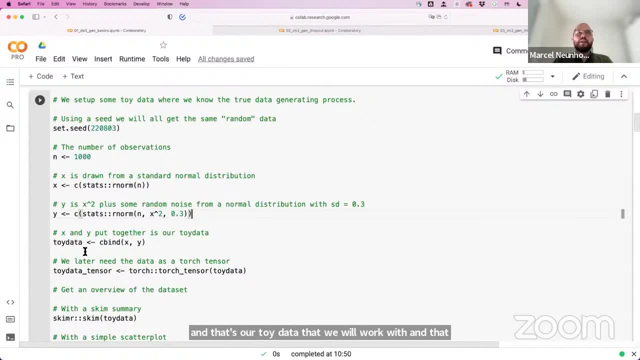 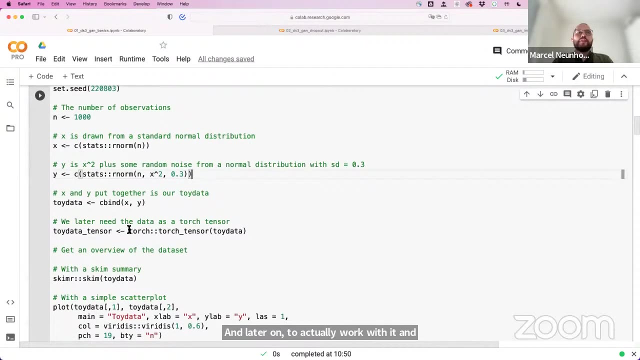 and that we will try to do And we will try to synthesize like we want to generate like a synthetic copy from that toy data And later on to actually work with it in Torch. and if you have worked with neural nets before, 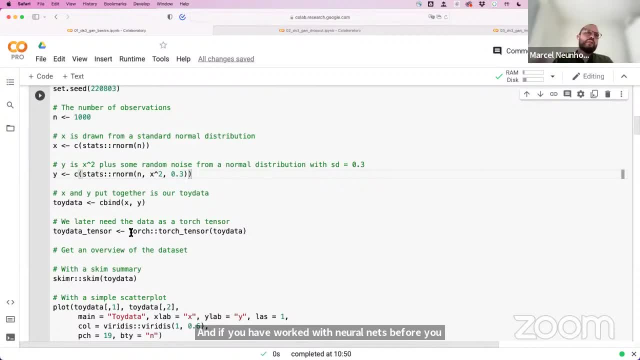 you probably know this- from PyTorch or also from TensorFlow. We need to transform like this object. We need to transform like this object. We need to transform like this object To a Torch tensor here, so like a type of object that the Torch library can work with. 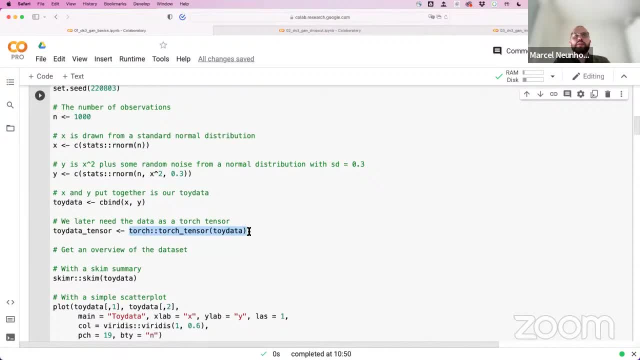 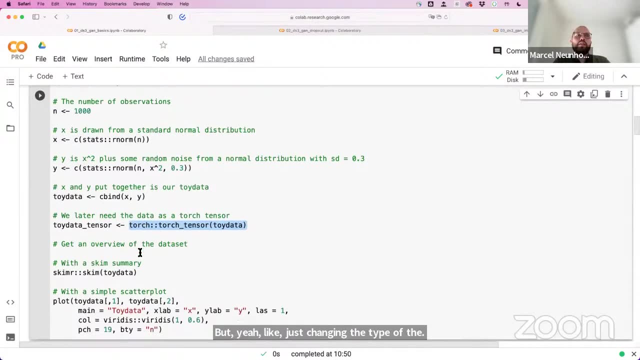 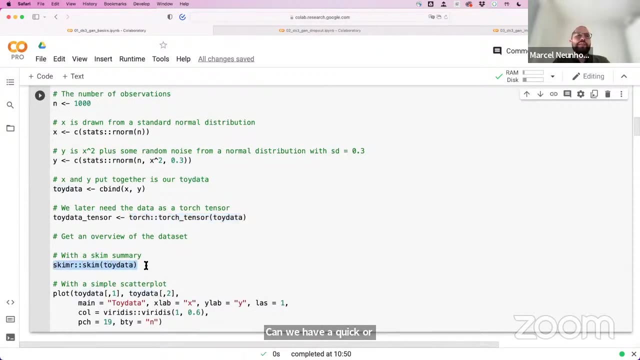 So that's just transforming or just changing the type of the toy data such that Torch can work with it. Then we have a quick overview skim of the toy data using the skim R, And also we have a package which is a very nice library. 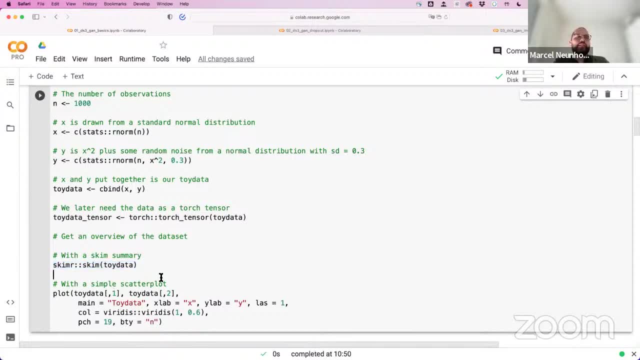 to get quick overviews of data and a simple scatterplot, And this will probably show the best what kind of data we are working with here. And, of course, if you want to work with this and play with this a bit, you could come up. 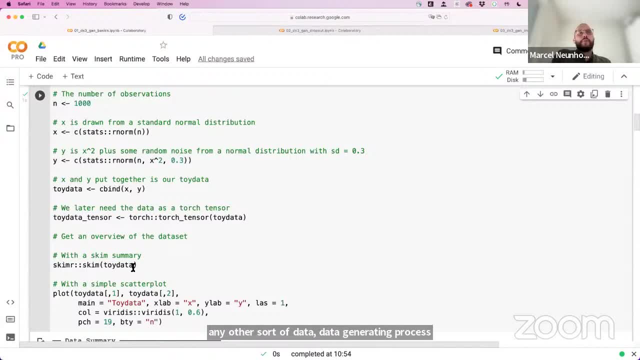 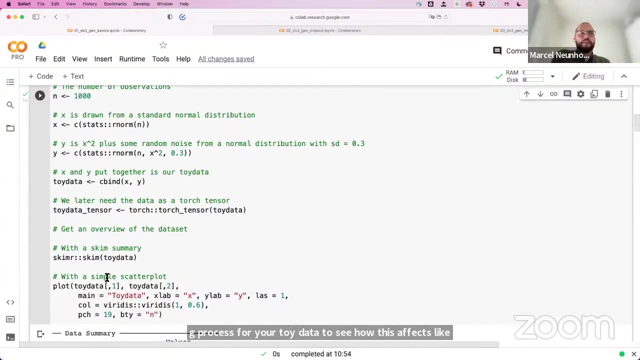 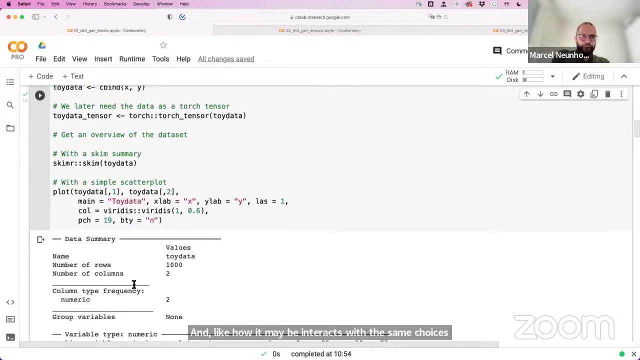 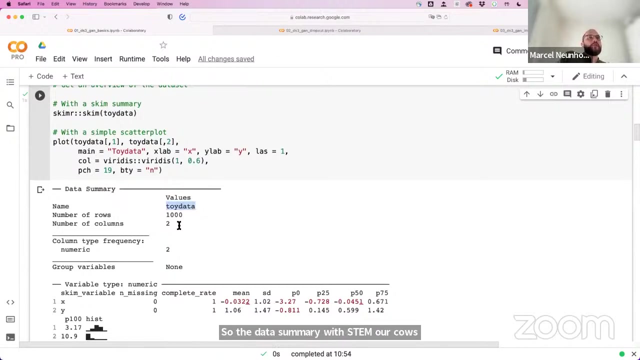 toy data: data generating process for your toy data, to see how this affects your training later on and how it maybe interacts with design choices that we'll talk about later today. So the data summary with StimR tells us: OK, this object is named toy data. 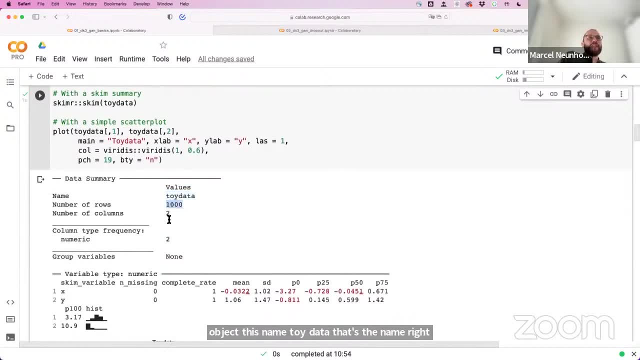 That's the name I came up with. It had 1,000 rows- That's the number of observations we set- And it has two columns. Both of those columns are numeric, which makes sense since it's a draw from a standard normal distribution. 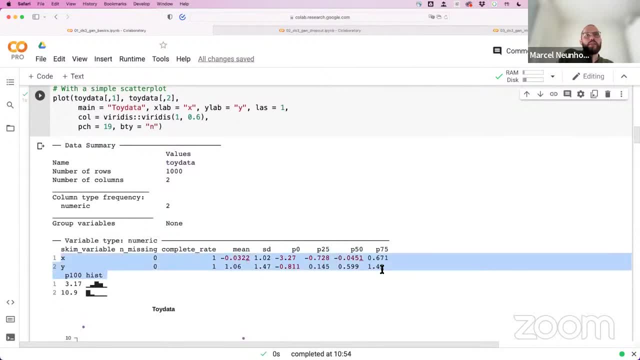 and a transformation of that. Then we see some statistics, like the number of missing data, which we have, none here- the mean standard deviation and some percentiles of our data. and the same thing for y, So for x. nothing surprising here. 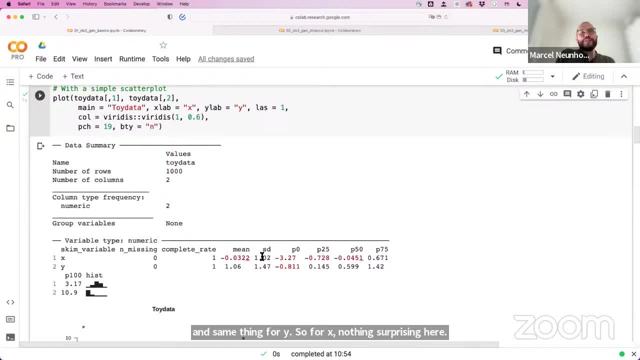 That's what a standard normal should look like: a mean around 0 and standard deviation 1.. And for y we have this skewed-looking data, which makes sense since our transformation is squaring, And we have the x And, I think, some of the data that we're going to talk about. 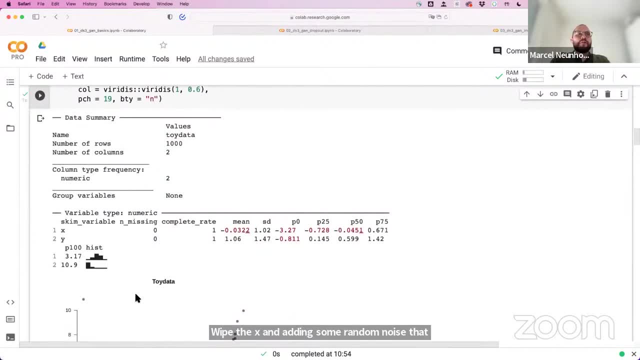 now is going to be a little bit more interesting, So I'm going to start off with the random noise. That means that very negative values, so like a minus 3 on x, gets something larger than negative 3. I said something positive when squaring it: larger than 9.. 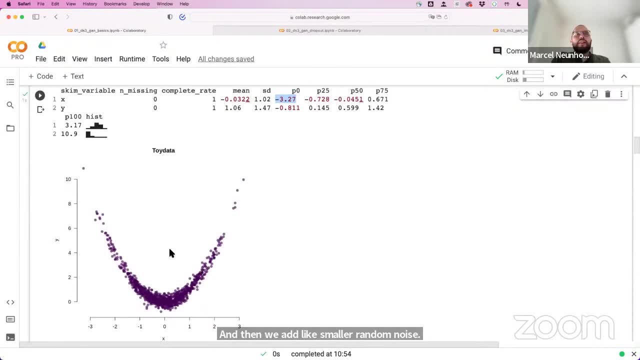 And then we add smaller random noise And we're going to think about a random noise like a random variable. So what does this data set look like and why did I choose this particular form? It looks like a parabola, right. 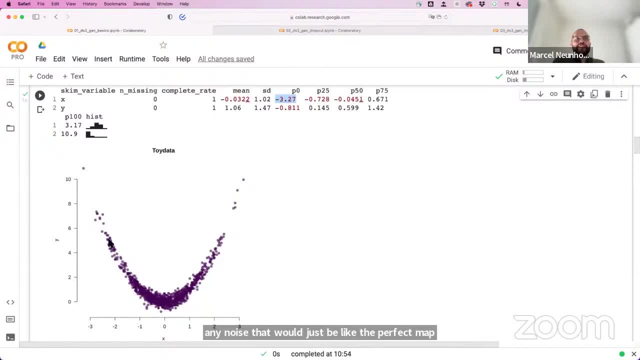 Like if we didn't add any noise, it would just be like the perfect mapping, from x to x, squared, And now we have some random noise that we added here so that we actually get something that looks more like real data that we typically work with. 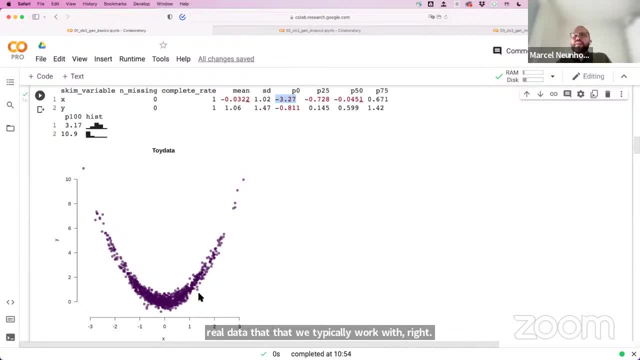 Right, this noise somewhere. And why did I choose this kind of function? Because it's not like from a statistics point of view, it's not like. without knowing, like the data generating process, it's not really straightforward how to come up with a generative model for this distribution. 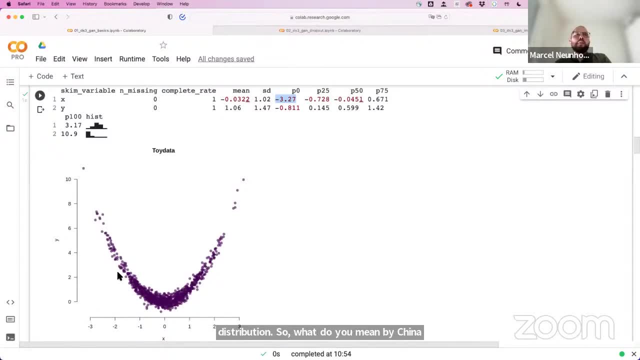 So what do I mean by a generative model? We want to produce a model that samples new points that follow the same relationship And it's definitely non-linear, right And also has like if we would try to view that from the perspective of why the issue. 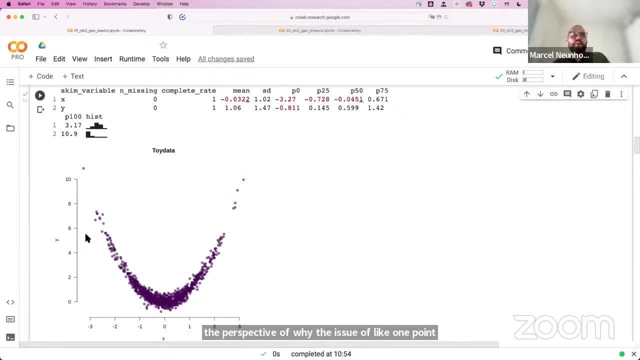 that like one point? and why maps to multiple points in X, Like if we go down here, like probably, like if you know the true function, a 6 in Let's make it a 4. and why could map to minus 2 or to 2?? 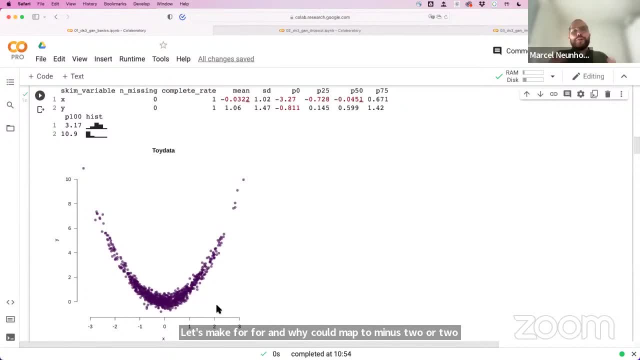 It's easy, it's two dimensional only And we know perfectly what the relationship is. but it's not too studying, simple right Like that. we have an immediate idea of how we could learn a generative model for that, And now we will try to come up with a GAN and train the GAN such that we can actually 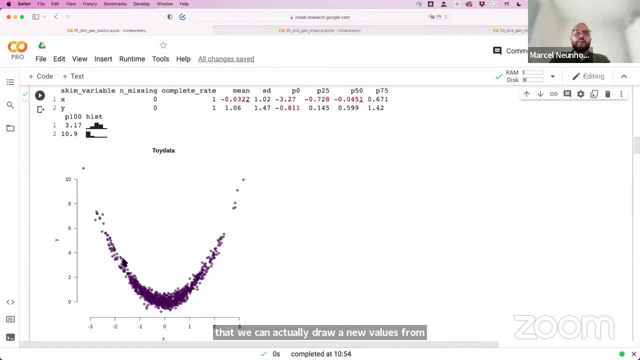 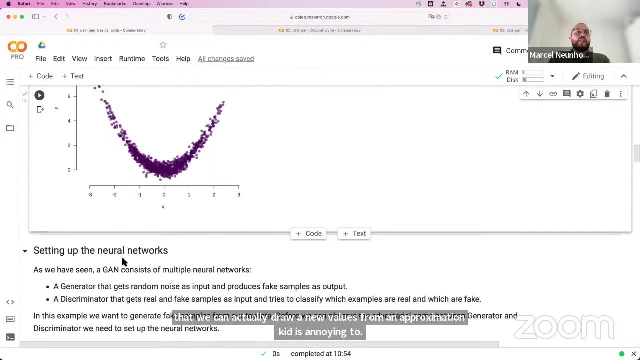 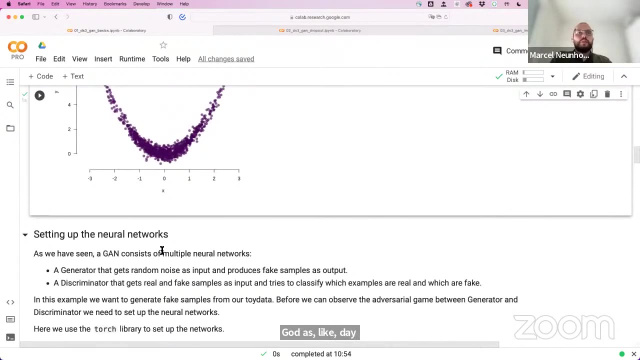 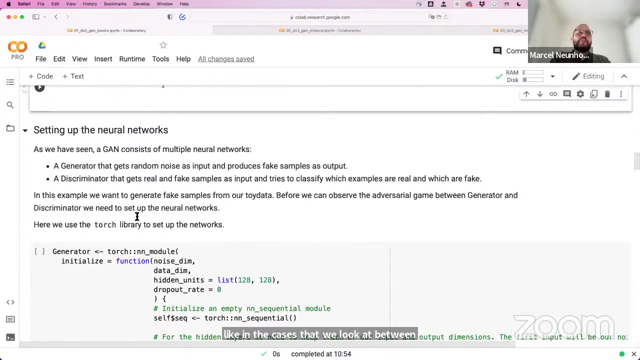 draw new values from an approximation to this annoying true function. All right, as we have seen before, like a GAN is like a game between multiple neural networks or, like in the cases that we look at, between two neural networks. The first is the generator. that 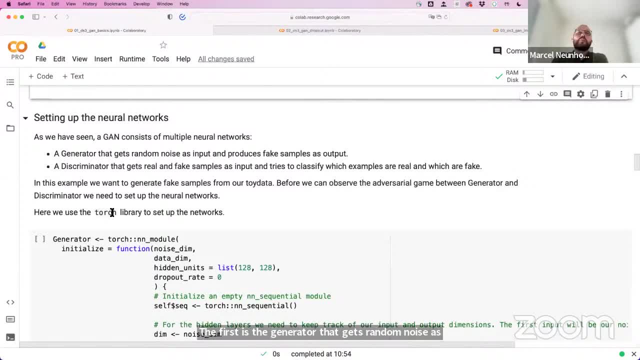 gets random noise as input and produces fake samples as output, And the second is a discriminator that gets the real data. And the second is the discriminator that gets the real data And fake samples as input and tries to classify which examples are real and which are fake. 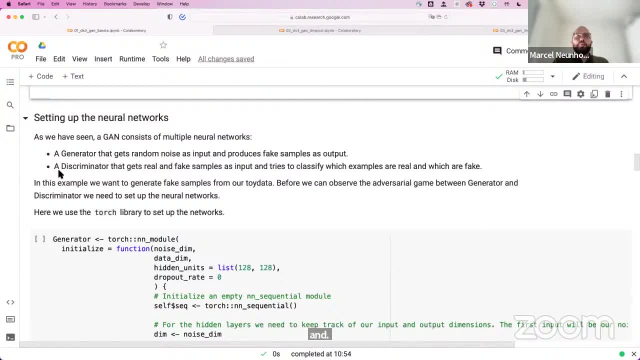 And, as I said here, we want to generate those fake samples from our toy data And so we want to learn this distribution and sample fake data. So our goal in the end is to have this generative model And, of course, before we can observe this adversarial game, we need to set up those. 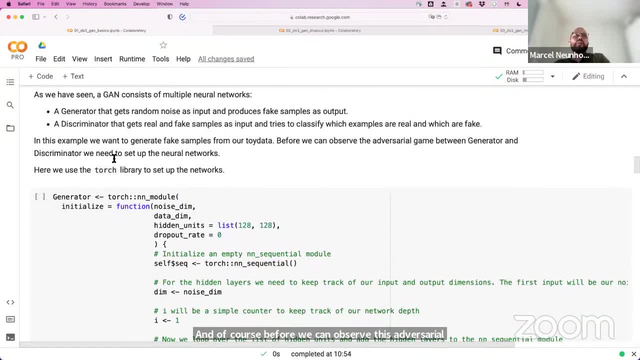 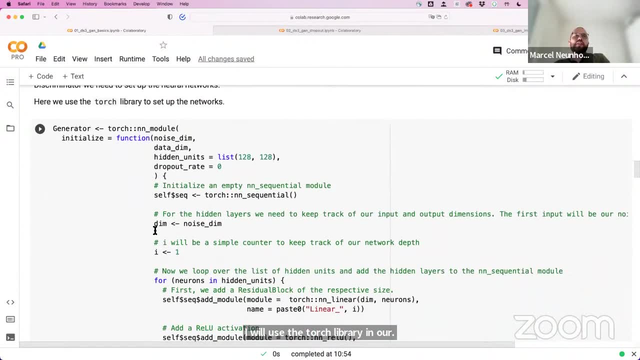 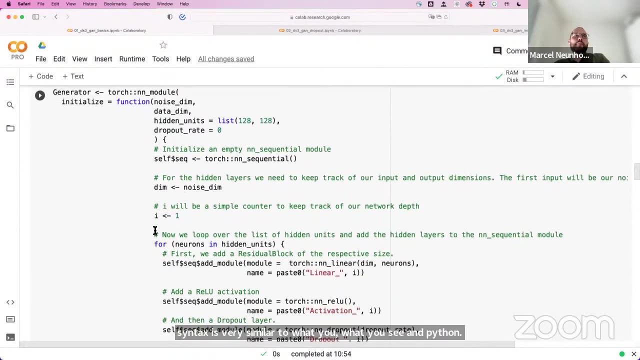 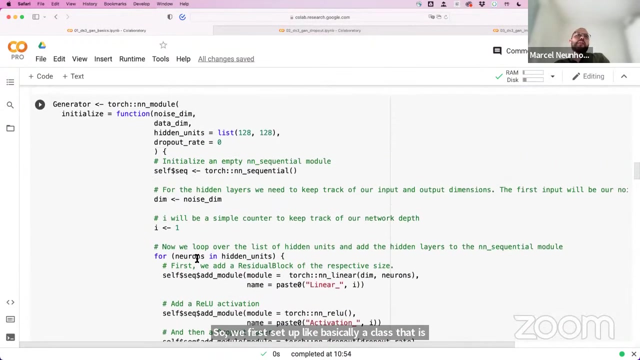 neural networks, And to do that here I will use the Torch library in R And like. if you're used to PyTorch, the syntax is very similar to what you see in Python. So we first set up like basically a class that is fairly general, so that we could easily use these. 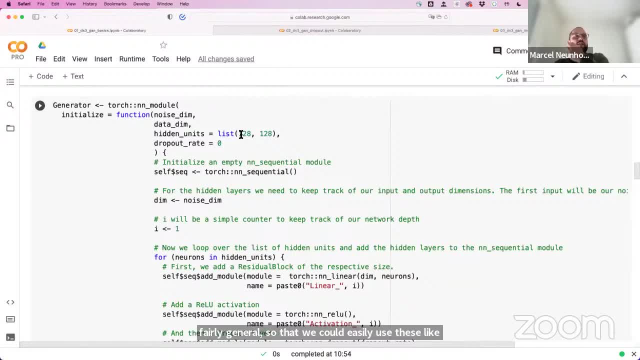 different, like parametrizations of the neural network, And there's two important things for, like the generator network that we need to take care of. And the first thing is- or that's true for any neural net and in particular with GANs, it's very important to think about it Like what is the 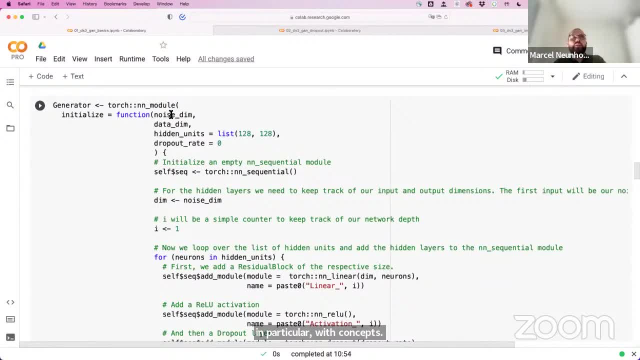 dimension of the input, and the input to the generator is our random noise. and what is the dimension of the output? and this is probably a bit different to neural nets that like if you ever used or if you ever coded a neural net for prediction- the output dimension is 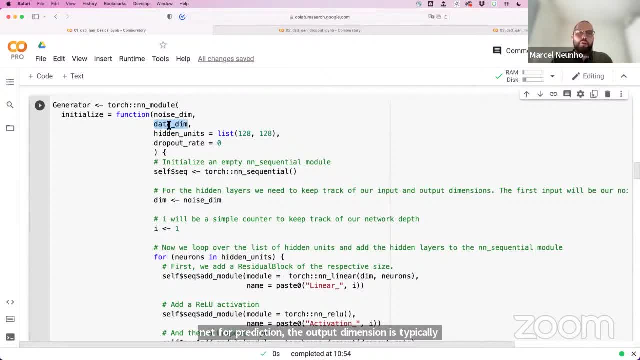 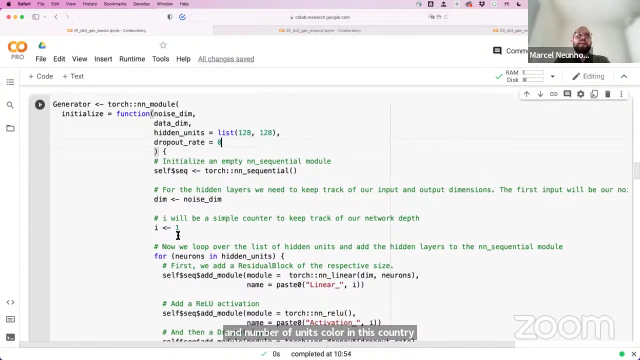 typically like one or maybe, if you have like a multi-class problem, the number of classes, but here it will be the exact same dimension as our original data set. then we can also customize the number of hidden layers and the number of units per layer in this particular like class, and we could also add: 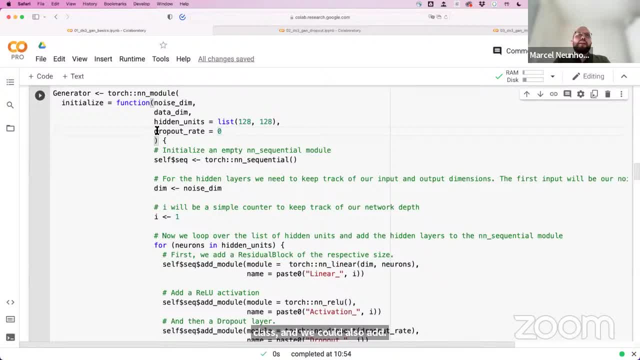 and we will experiment with that later today- the dropout to the hidden layers. so dropout is like a way of getting additional random noise into the network, which typically helps to converge a bit quicker and also has a nice side effect that we will look at later. then it's just set up as a 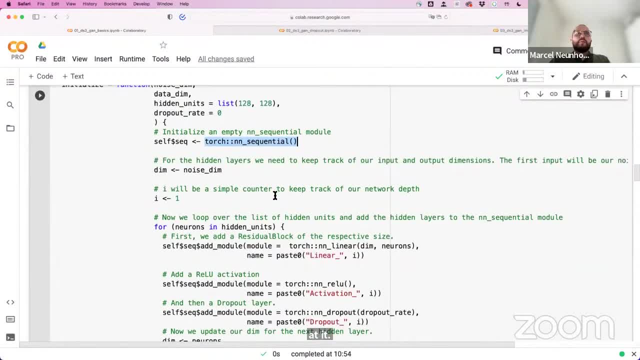 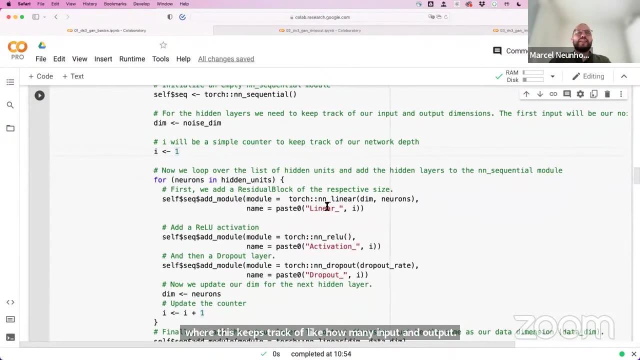 sequential neural network module where this keeps track of like how many input and output units we need and then just stacks like a linear layer with the right numbers and with a re-lure activation and potentially a dropout layer, or it will add the dropout layer no matter what, but like this is exactly the whole idea of hyperlogatic model. so i think that's 1.5. 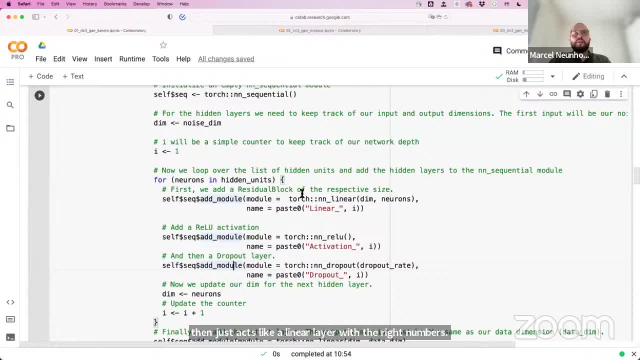 cycles. i think it's, at this point, okay. we're done on the refusing transport autopsy, so i think this is okay to start, like shops, but tell me your view. yeah, anything you wanna add, like talk to me, matter what, but if our dropout rate is zero, 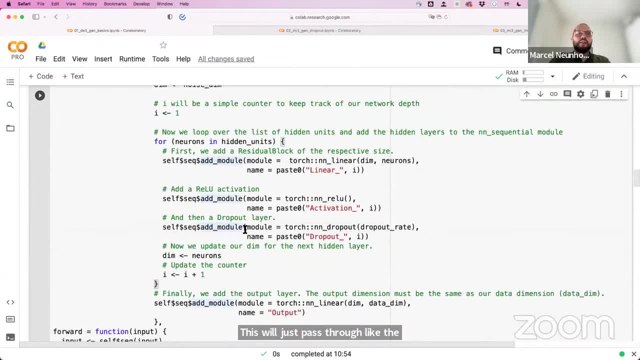 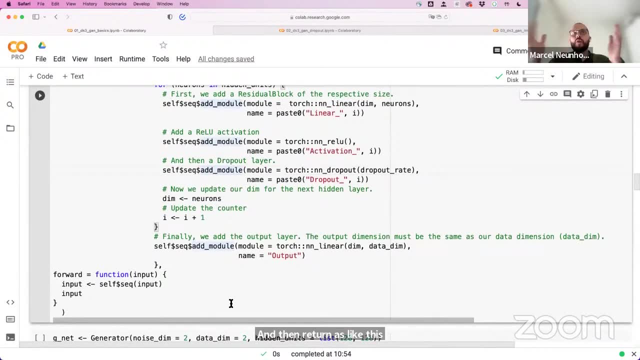 this will just pass through the previous activation And then return as this whole neural network module where the output layer for the generator is just a linear layer, so a fully connected linear layer where now the output has to match our data dimension. So this is important, so that we can actually 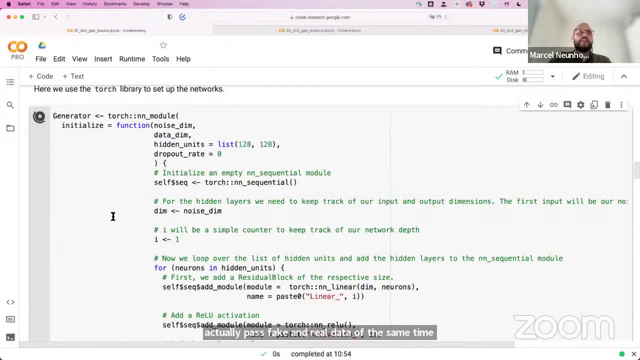 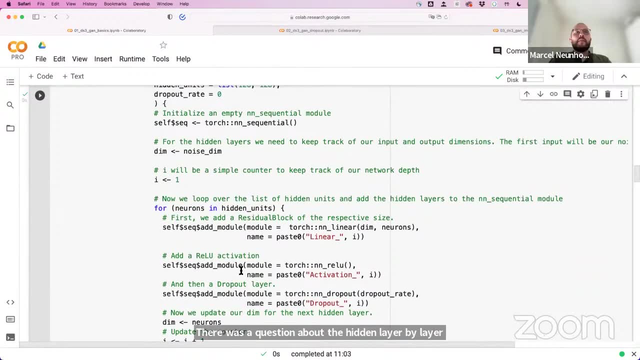 pass fake and real data of the same dimensions to the discriminator. Marcel, there is a question about the hidden layer. Valeria is asking about the necessity of a hidden layer. What is it needed for? So maybe you can elaborate about that. Yeah, right, 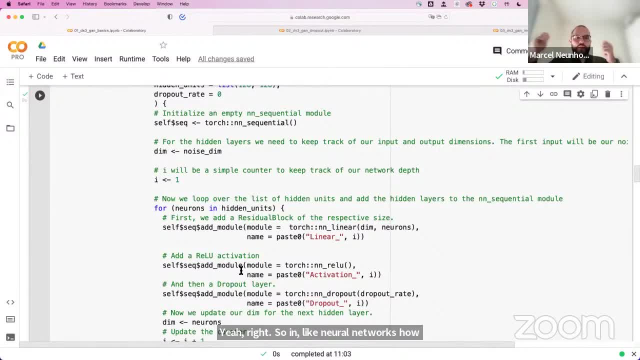 So in neural networks, how you get this flexibility of learning non-linear functions basically is that you stack. So basically you have two options. So you can go very wide And research has shown that a network with one hidden layer- and we all have a hidden layer- 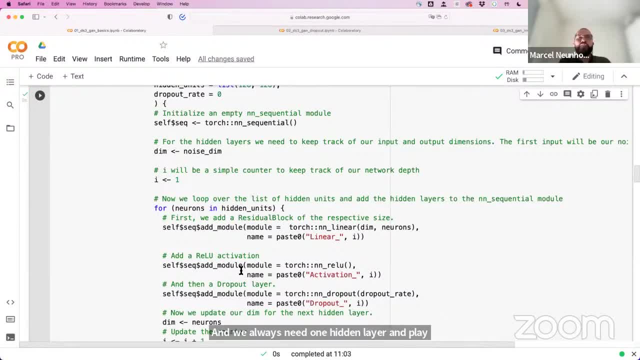 And so if you stack the input layer, you always need one hidden layer, And the hidden just means you have an input layer that basically takes the input as is and passes it to neurons. Then we have a hidden layer that is basically taking care of all the nonlinearities. 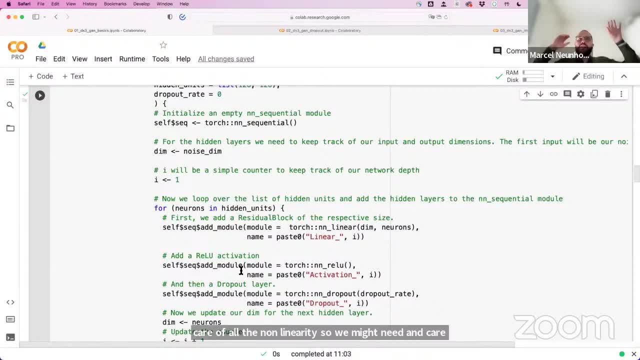 that we might need and care about and an output layer And the hidden layer is named hidden because we typically don't care about the input and output output of that. We care about the input at the data level that goes into our network and we care about the output. 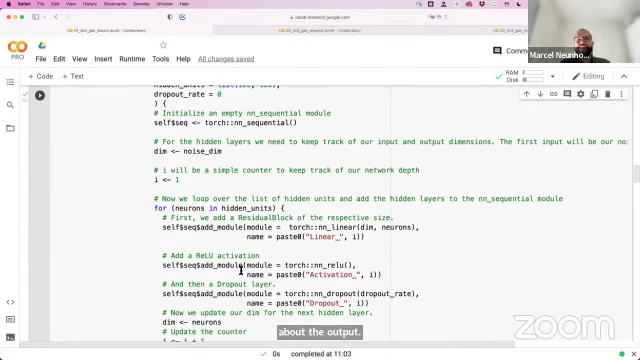 And therefore this name hidden layer became a convention And a neural network. with one hidden layer and enough width, so enough number of neurons can approximate arbitrary functions already. However, empirically it's very hard to get enough width. It has been shown that adding multiple hidden layers so going deeper, and that's where the deep and deep neural networks comes from. stacking multiple hidden layers on top of each other, It helps to get those non-linearities with less width. So there's basically a trade-off between width and depth. 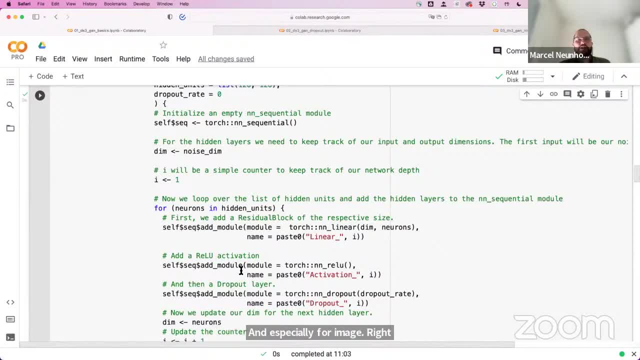 And especially for image recognition and then also image generation later today, the standard of deep, so multiple, hidden layers, convolutional neurons and that. But if you want to know more about that, I guess there is a great course from last year of this summer. 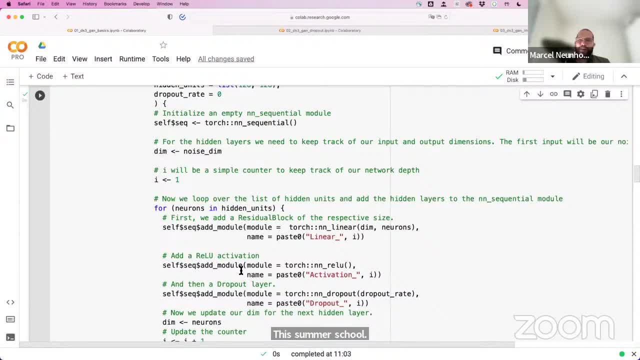 school. that should probably still be on YouTube. that goes a bit more in-depth about what this means and how these neural network architectures work, And I take them a bit as a given here because it would be too much to cover it all, But I hope this was helpful nevertheless. 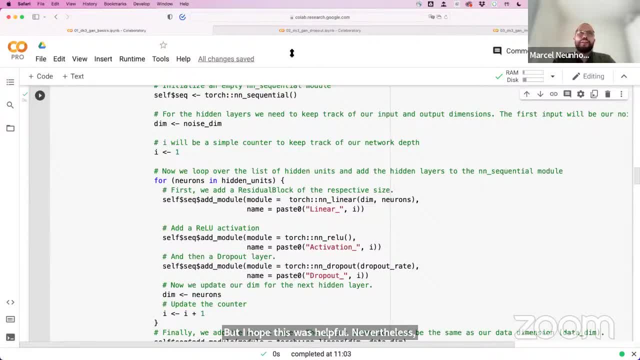 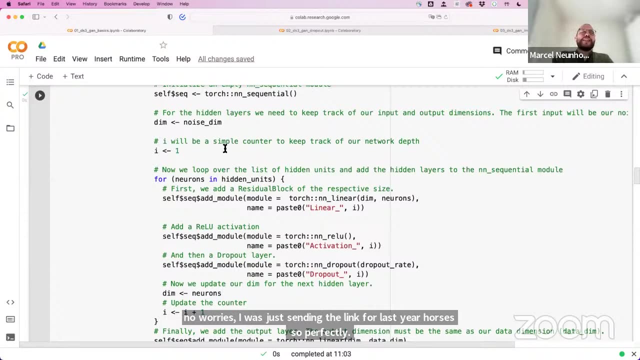 Is there a follow-up question? I just always see the number going up. Hi, no worries, I was just sending the link for last year of courses, Perfect Right. So Yeah, Like with this function, we basically can now generate neural networks that. 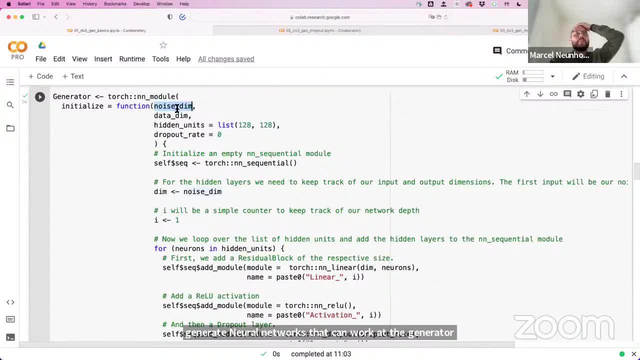 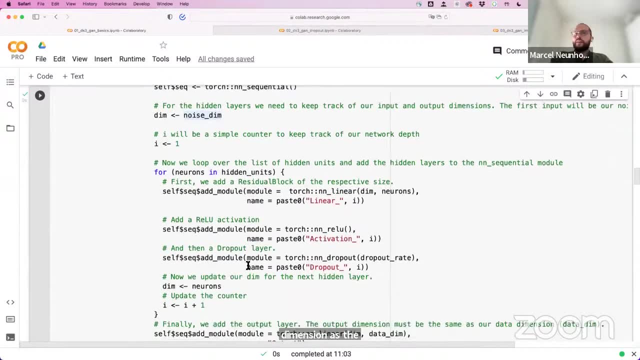 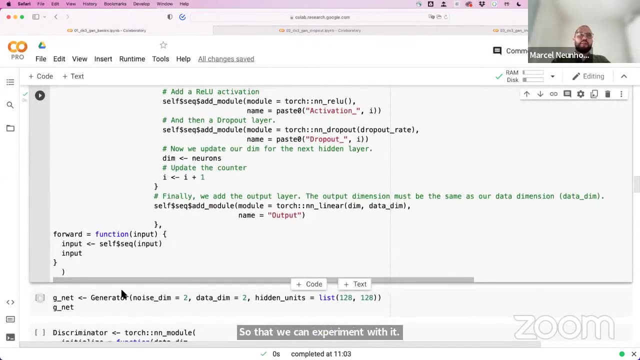 can work at the generator because we have those noise dimension as the input and the data dimension as the output, of arbitrary depth and width, so that we can experiment with it. So if we have this function, we can now initialize generator net. And here 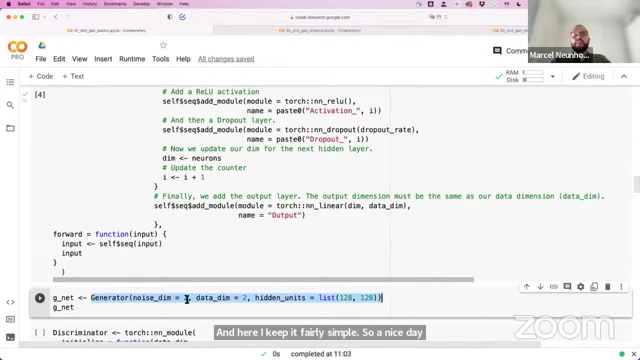 I keep it fairly simple. So a noise dimension will be just like a vector of two independent draws from a standard normal distribution. So it will for each generated fake example we will take as an input like a vector of two draws of independent normals. 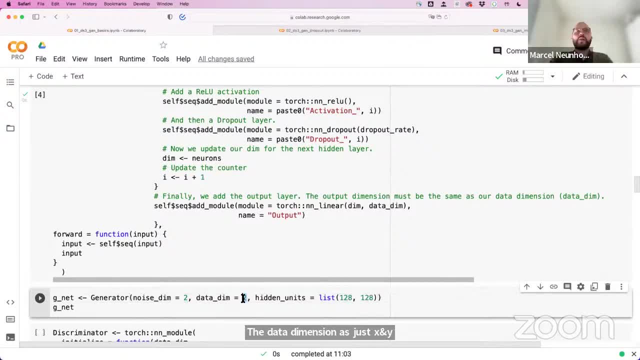 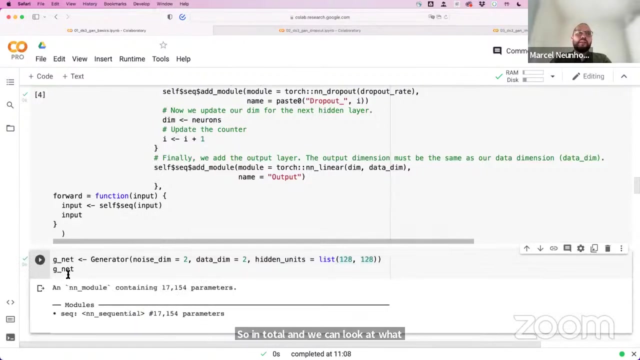 The data dimension is just x and y. right, We just have those two dimensions. And this is- yeah, it's a medium-sized neural network with two hidden layers and 128 neurons per layer here. So in total, and we can look at what this call to this function. 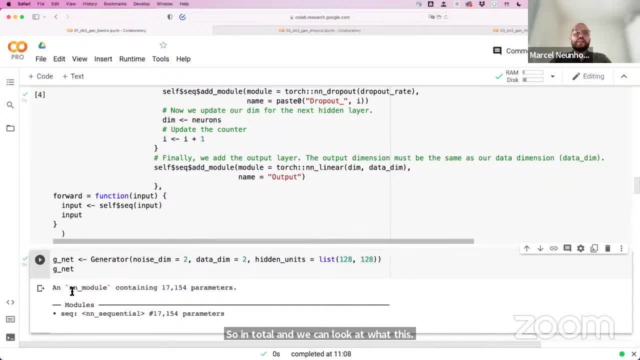 and generating this gnet object here generates, And this is now an nn module. So that's like a torch Neural network module that has 17,154 parameters that we can now train. So that's like, yeah, it's more than in our typical logic. 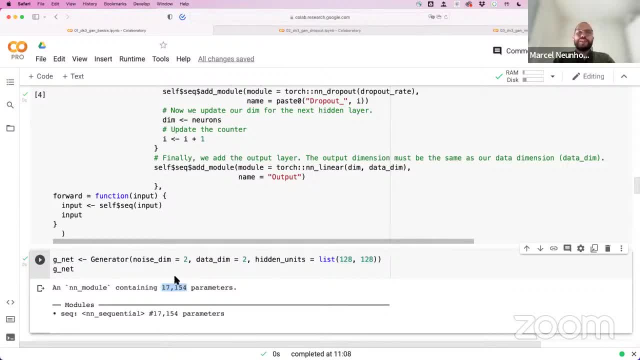 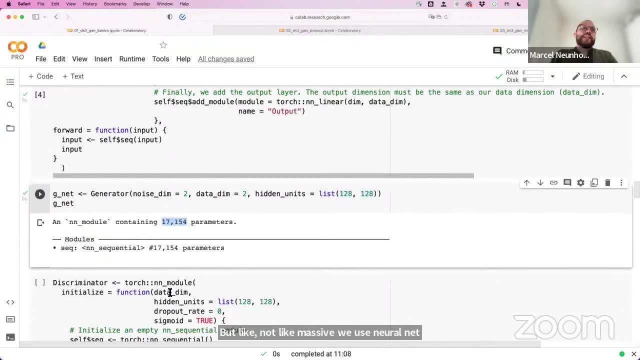 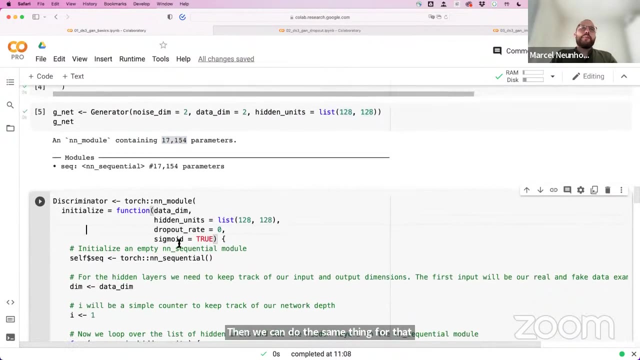 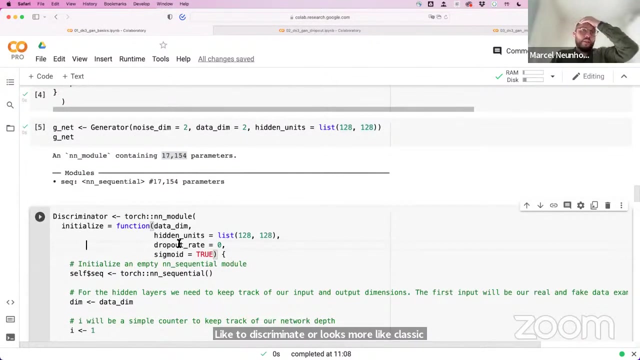 regression model, but not like a massively huge neural net with millions of parameters. Then we can do the same Same thing for the discriminator. And here the discriminator looks more like classical neural nets that you might have come across, because it is basically 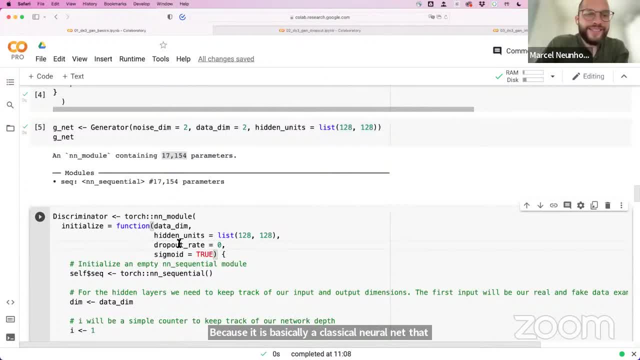 a classical neural net that tries to predict labels right, So tries to discriminate between fake and real- So that's the labels- And takes us an input like our data And we will later in the training we'll make sure that it looks at fake data and real data. 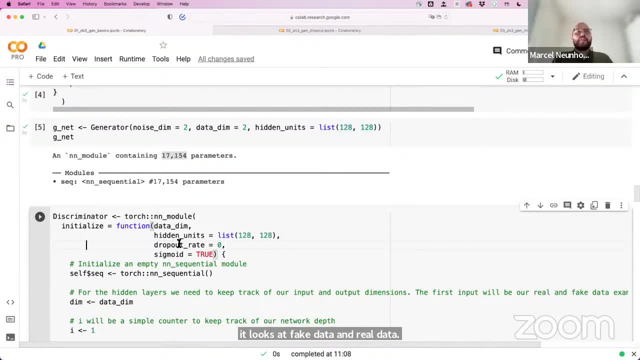 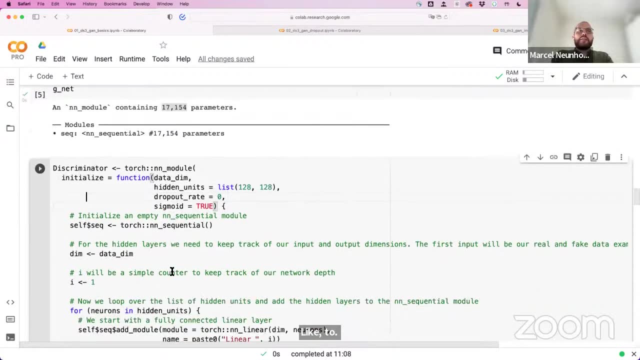 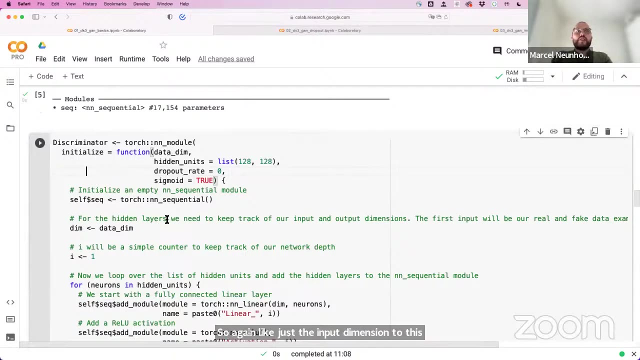 and then uses that to learn the way to distinguish between the two. So again, like this: the input dimension to this neural network should be the data, The output dimension. we don't need to specify an output dimension because that will just be one. 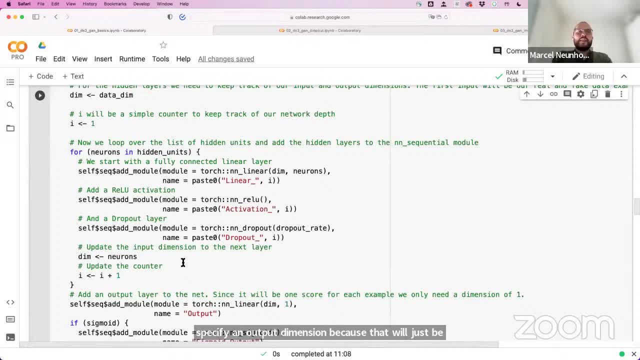 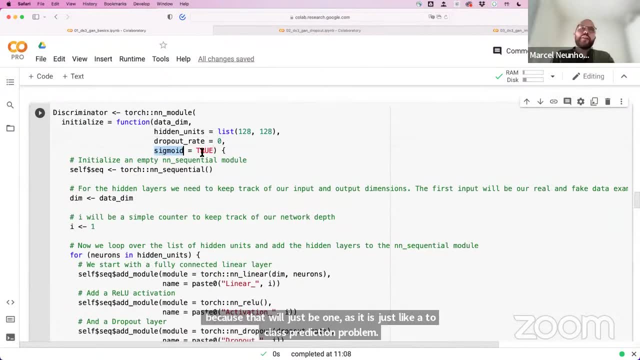 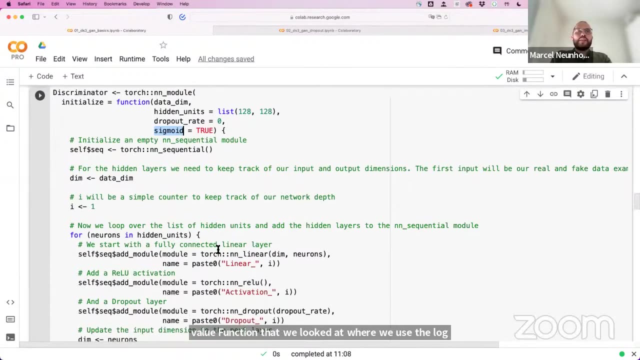 as it is just like a two-class prediction problem And we will need to add, like for this classical GAN value function that we looked at, where we use the log of those discriminator scores, which comes from this binary cross-entropy formulation. 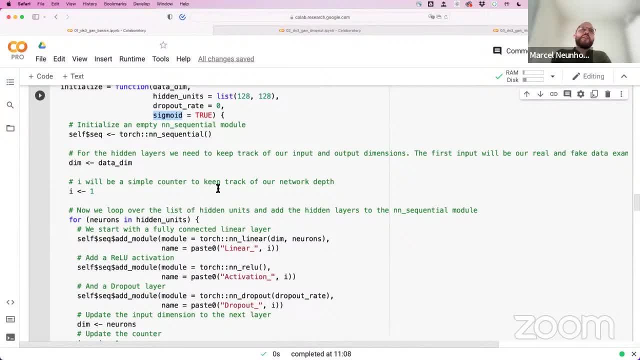 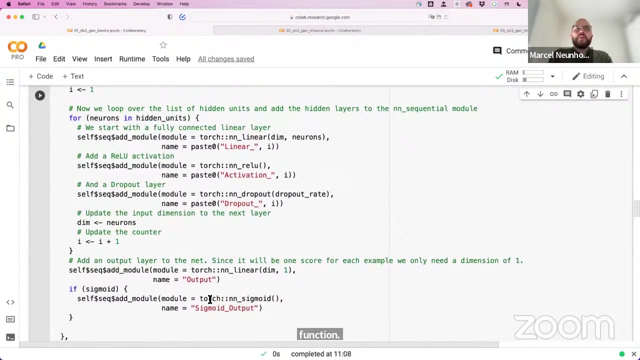 or from standard logistic regression. we need to make sure that the output of our discriminator net is probabilities between 0 and 1. And one way to do that is to use a sigmoid activation function after the output layer. right, So it will be a blank. 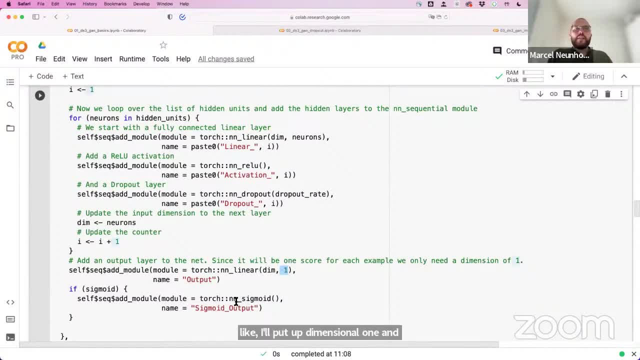 So it will be the output of dimension 1. And using this sigmoid activation, we force the output- each individual, basically prediction for fake and real samples- to be a prediction of a predicted probability of being fake. So, like the sigmoid function squashes, like the, you know. 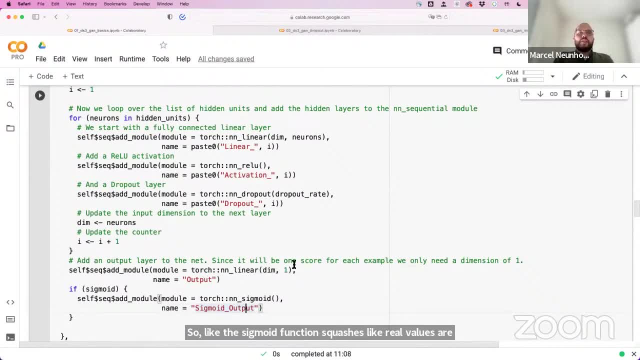 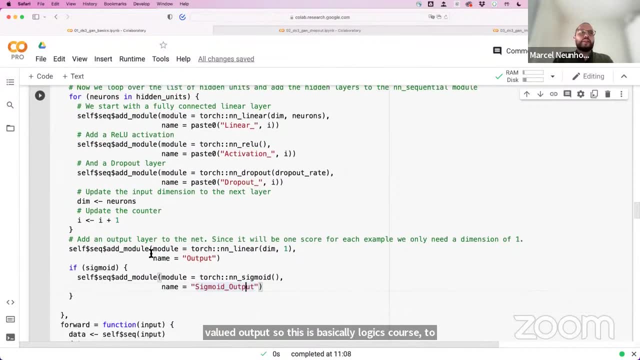 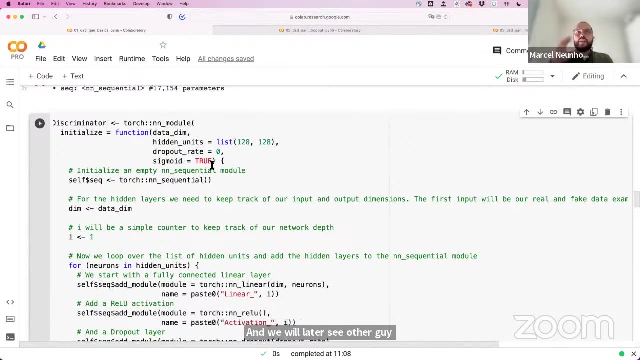 real valued output. So this is basically logit scores to the interval between 0 and 1, so that we actually get probabilities And we will later see other GAN value functions, other GAN architectures where we don't necessarily need this anymore. 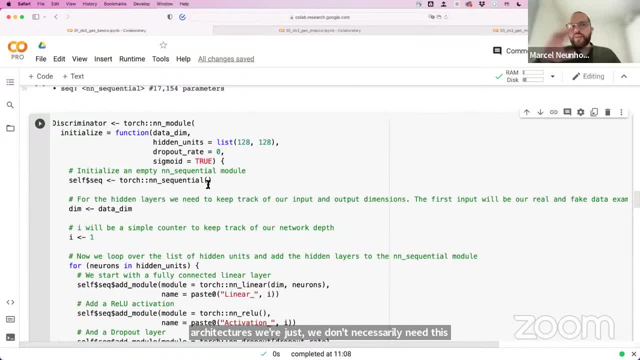 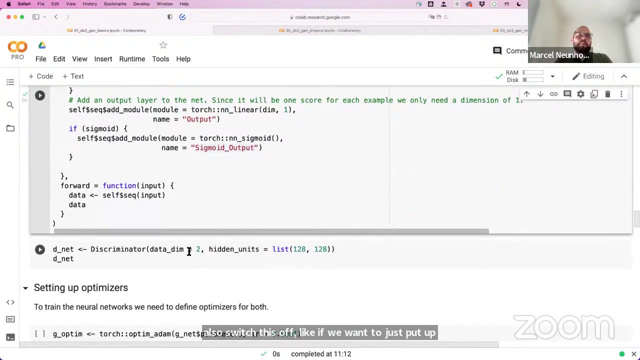 where the discriminator works a bit differently And uses like real value input for the value function And therefore we can also switch this off, Like if we want just the output of the linear output layer And, like in this example, I basically mirror the architecture of the generator. 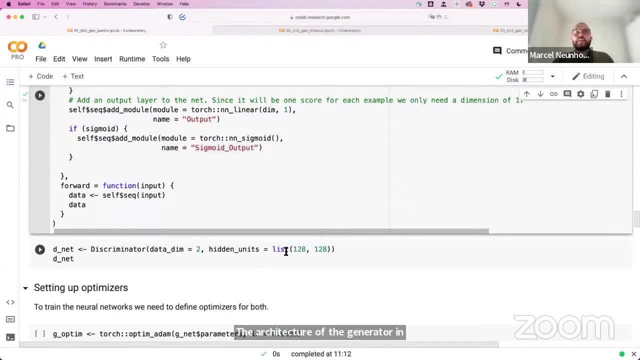 Right Right, Right, Right Right in the discriminator as well. So it has the same number of hidden layers and hidden units, And this sort of like became the convention in GANs. like that, the generator and the discriminator are basically mirrors of each other. 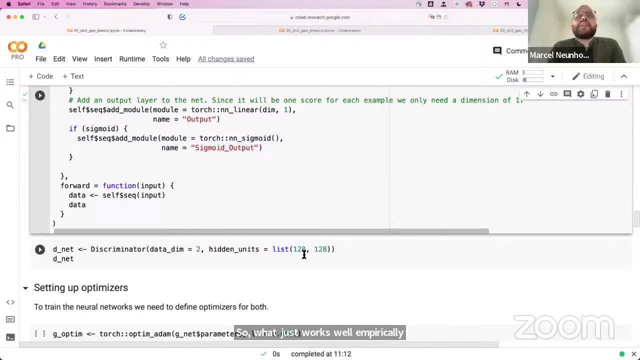 as it like, just works well empirically and also ensures that, like, one network doesn't overpower the other network. Because, like to learn this adversarial game, we want both of those players to be of similar power because otherwise, like if one can learn faster. 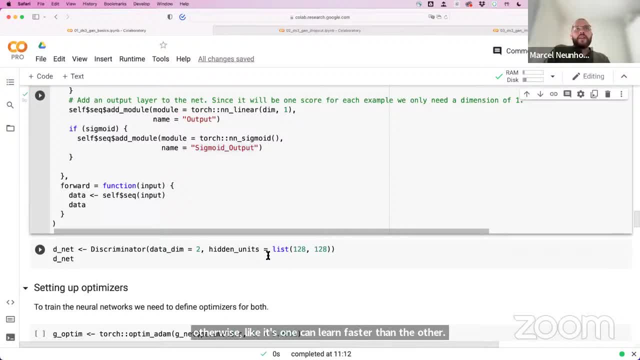 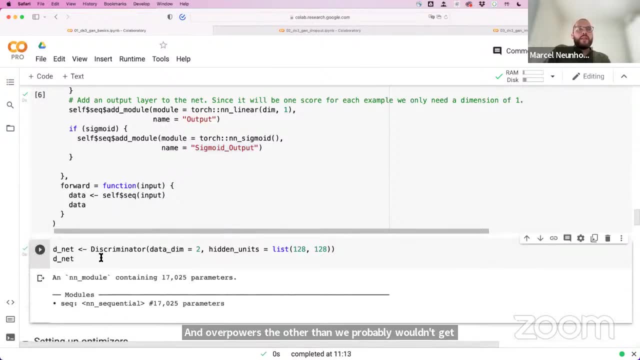 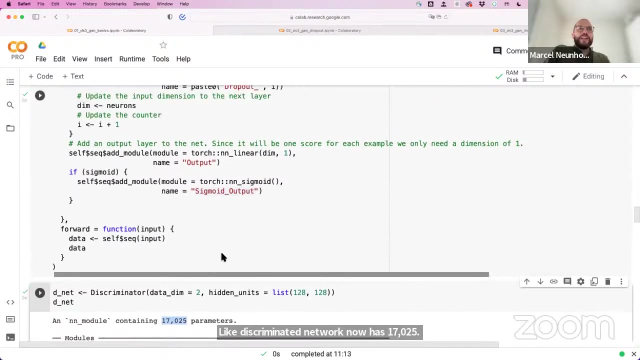 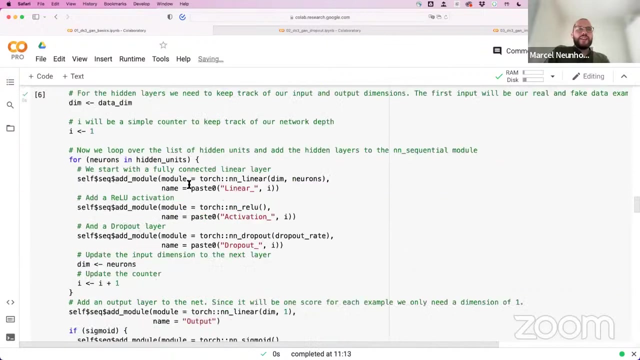 than the other and overpowers the other, then we probably wouldn't get to the equilibrium. Like the discriminator network now has 17,025 parameters. Does anyone have an idea why like this is like a like about like 150 parameters less than the generator network, 130.. 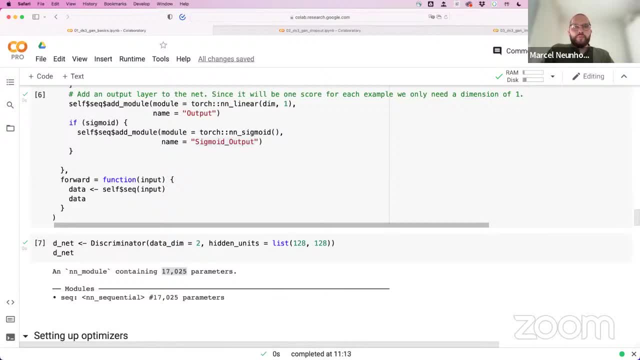 It's just a quick like knowledge check. Yeah, that's. I can see the answer in the chat because only one dimension I don't know. It's like the answer slash question in the answer. but that's exactly right. So in the generator we have like two inputs. 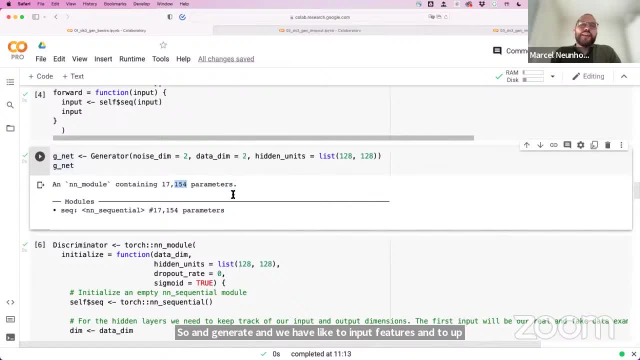 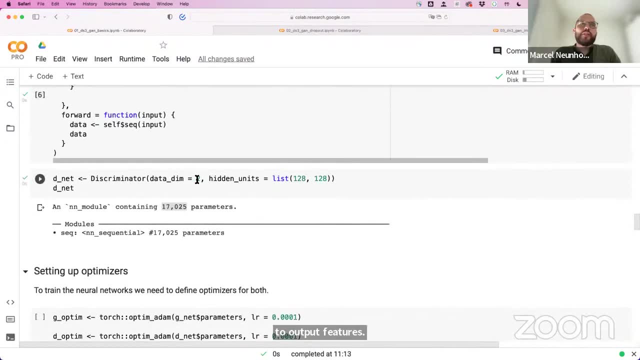 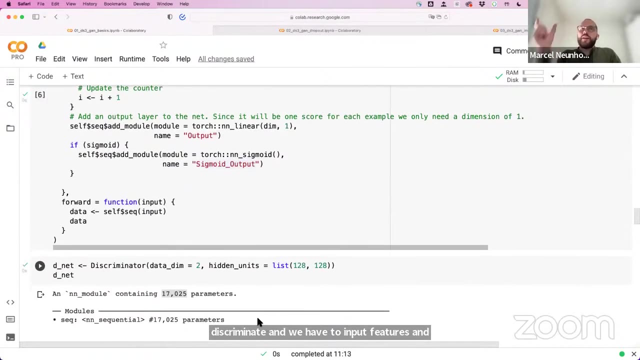 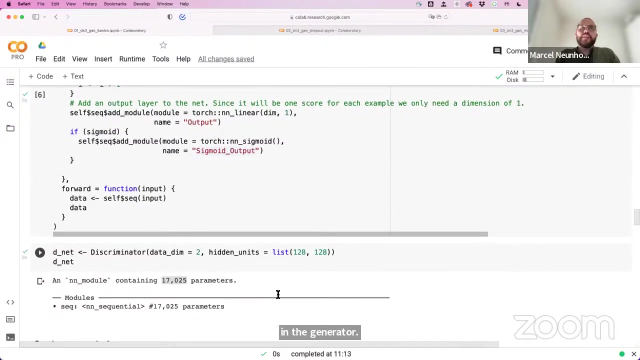 two input features and two output features, And in the discriminator we have two input features And, as we could see here, only one output feature. So, like the last layer will have less parameters than in the generator. So this explains like this tiny, tiny difference. 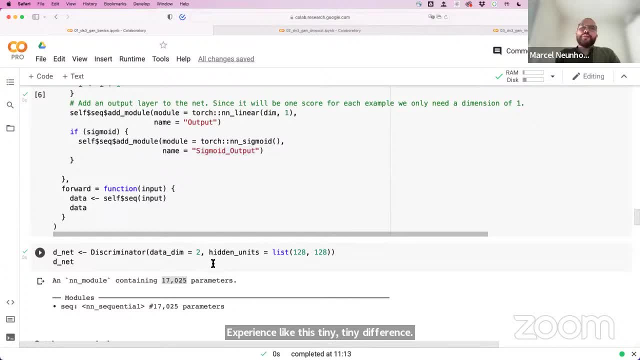 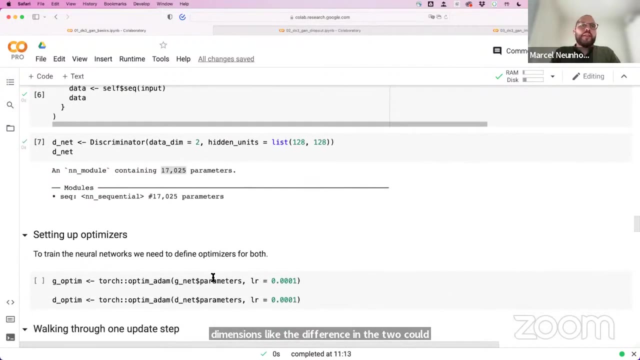 here. but of course this means like if we have like data with more dimensions and like, depending on how we choose our noise dimension, like the difference in the two could be larger. All right, then we need optimizers for both of these networks. 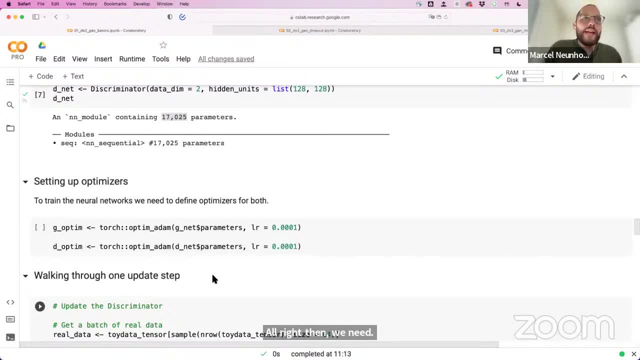 And here I just choose, like the Adam optimizer from the Torch, PyTorch library with like standard momentum parameters And we need to tell it which parameters like this one should optimize. And for the step to update the generator, we only want to look at the generator parameters. 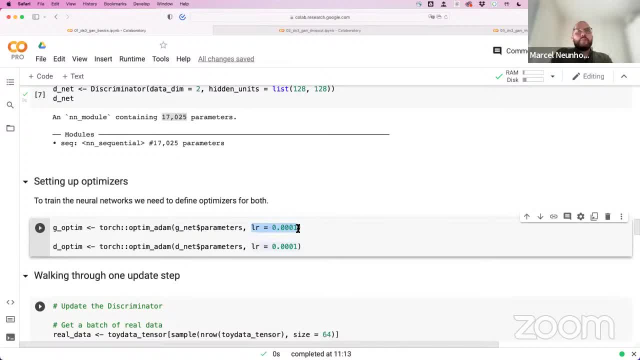 and we need to set a learning rate- And this is like a very small learning rate- that also make sure that, like those two networks don't overpower each other too quickly and make like huge jumps in like different directions And use, in this example, the same, exact same optimizer. 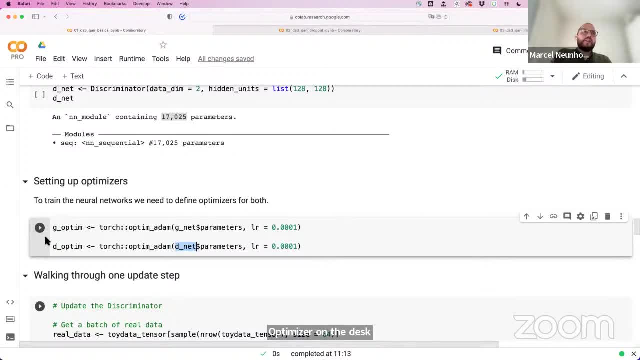 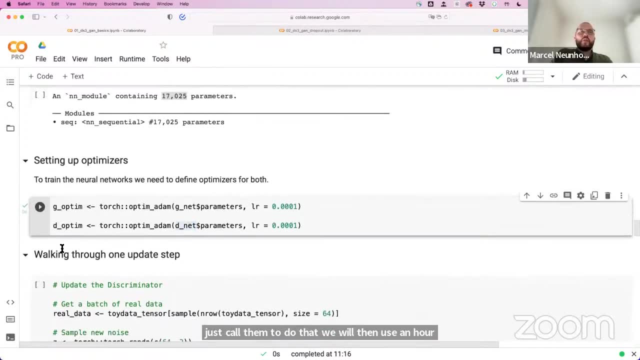 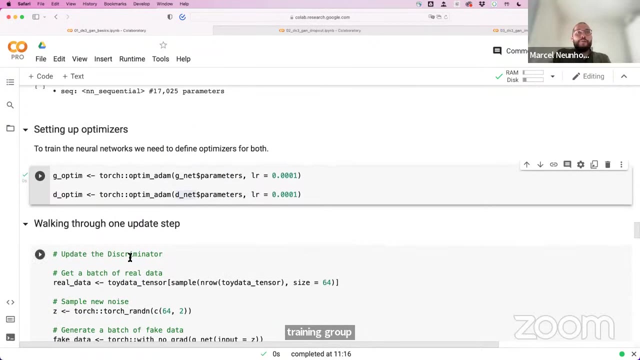 on the discriminator net parameters and just call them. So we can just use the Goptim and the optim that we will then use in our training group to update like this. Okay, and now we are at, like the exciting step where we can put this all together. 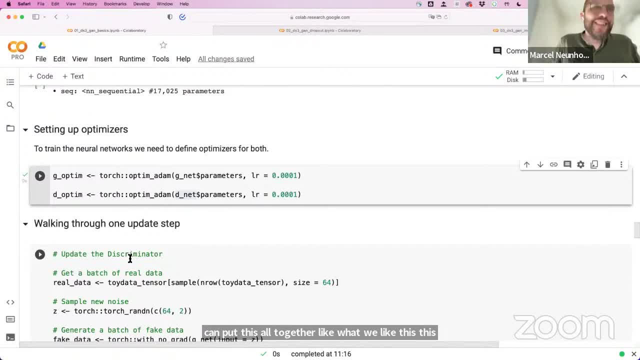 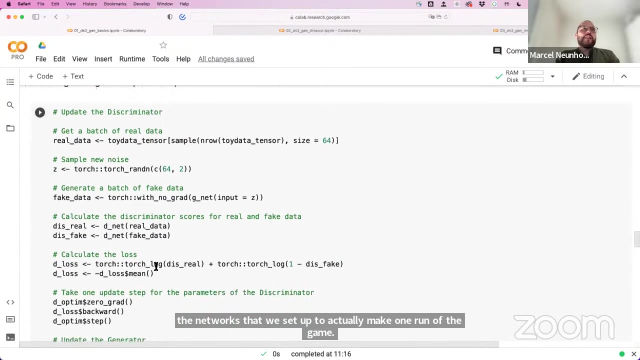 Like what we like, this, this game between bandits and police, the formula and the networks that we set up to actually, you know, make one run of the game. So to make one run of the game like we first sample a batch, a mini batch, from our real data. 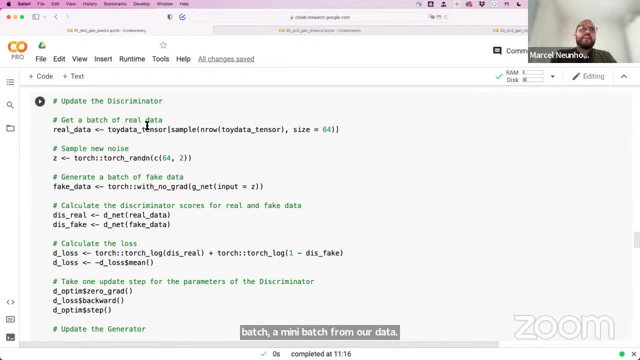 So here we use our like toy data that we transform to like this torch tensor object and sample like. the sample command in R says that we want to sample like basically 64 indices from like a thousand potential indices and then use those indices to pass like a mini batch. 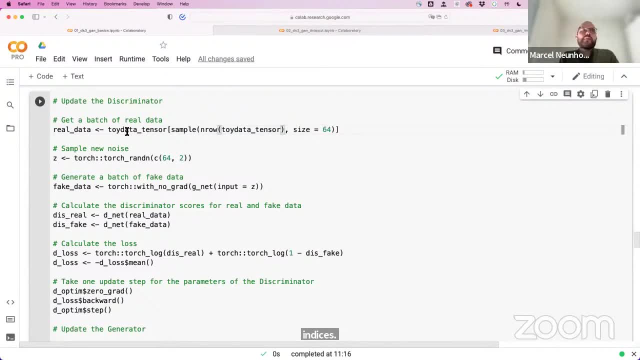 of actual, real data. Then we sample units. We get the noise 순 and torch ran is sampling from a standard normal distribution with the given dimensions. So we make sure that, like the mini batch size we use, 64 here matches like the mini batch size. 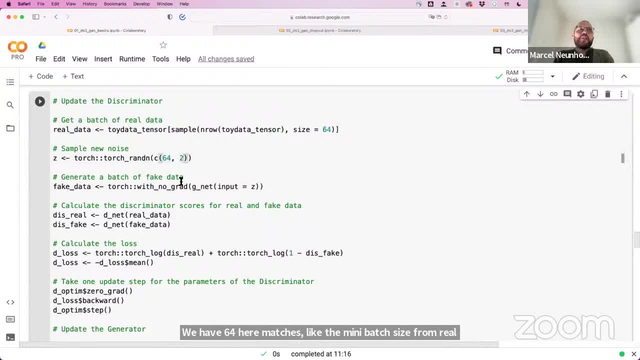 from the real data and our noise. dimension is here, So just will directly sample like a torch tensor object with dimension 64 by two. So can think of it as a matrix with 64 rows and two columns And in each of those cells 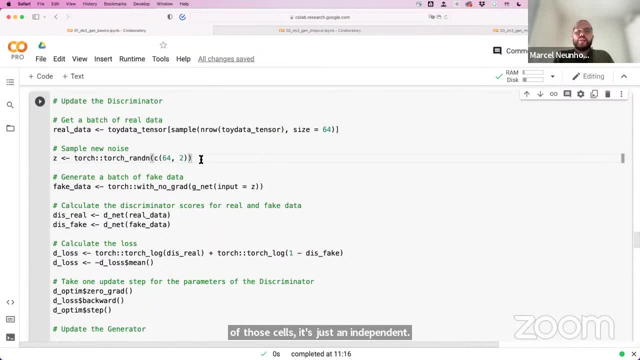 it's just an independent draw from a standard normal distribution. Using that, we can now use our generator to generate fake data right Like we pass, like this noise. that's exactly what we saw in this picture as input to the generator: net. 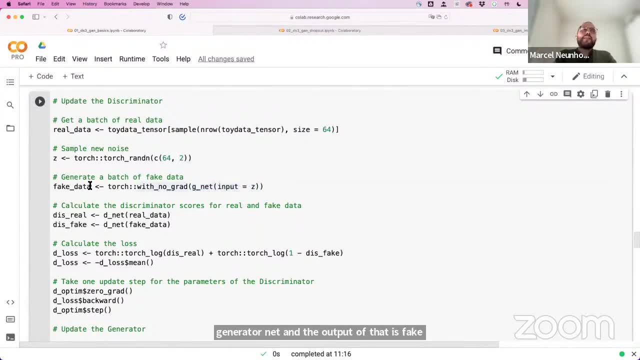 And the output of that is fake data, As like in the first half of like this update step, we only update the discriminator. We don't need a gradient here. So there's just this, like for efficiency reasons, that we don't calculate gradients for something that we don't actually need here. 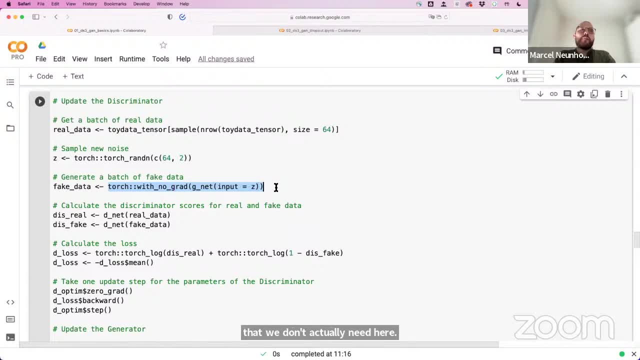 And like: get a tensor, a torch tensor, back, like that holds fake data. So in the first round, and like we will run through the first round, like for this code chunk in a bit. This, of course, is like the bandits who have never seen money trying to come up with. 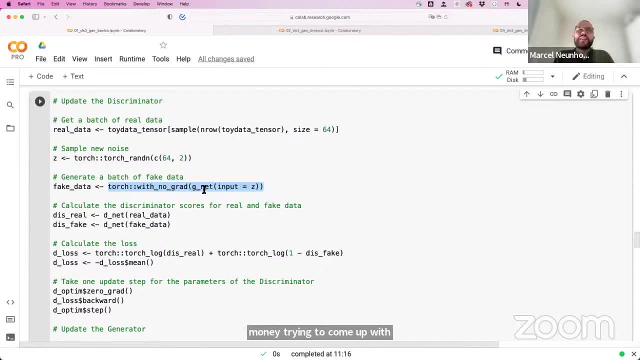 so this is like the bandits who have never seen money trying to come up with something like this. So this is like the bandits who have never seen money trying to come up with something they think is money, So this will not look like anything close. 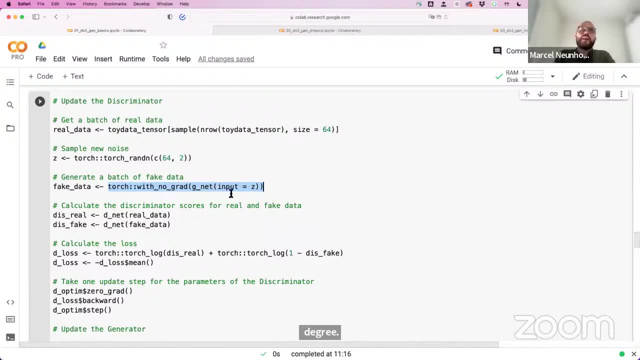 to the real data, right. So in the first round this will look like random noise as well. typically, Then we use our discriminator net to calculate the scores. So the probabilities of being real on the real data and on the fake data. 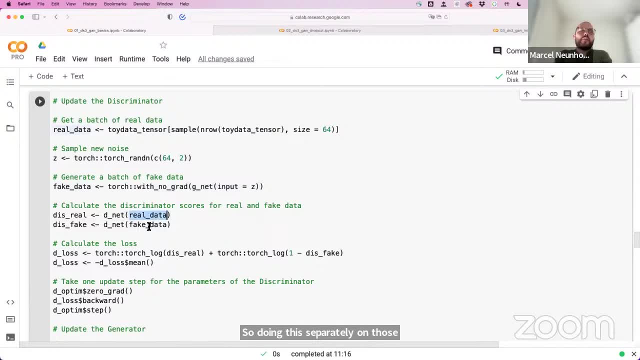 So doing this separately on those two sets of data allows us to calculate the loss in a way where we don't actually need to append labels as well, And this is basically exactly the value function that you've seen on the slide. So this is the original Kahn value function. 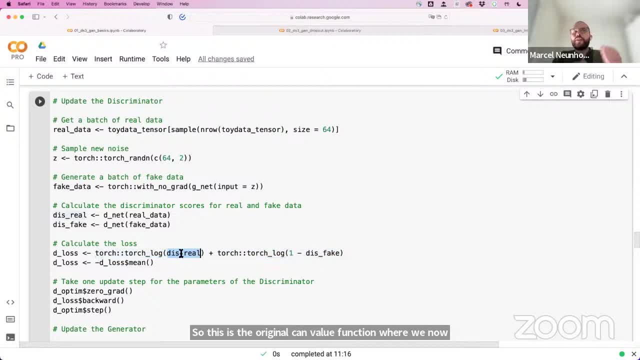 where we now use the log of those predicted probabilities of being real for real examples and add the log of one minus the probabilities of fake examples being classified as fake. And as like we want to like, as the discriminator wants to minimize this, we just use the negative mean of like that. 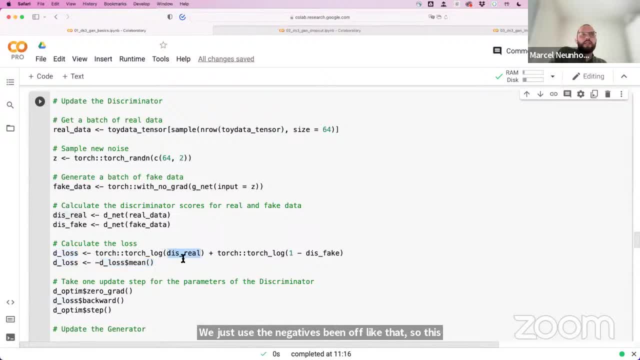 So this will be a vector, right. So this is a vector of 64 scores. This is a vector of 64 scores, So this adding this up was like a vector of 64 scores and now taking the mean of that and putting the minus sign in front of it. 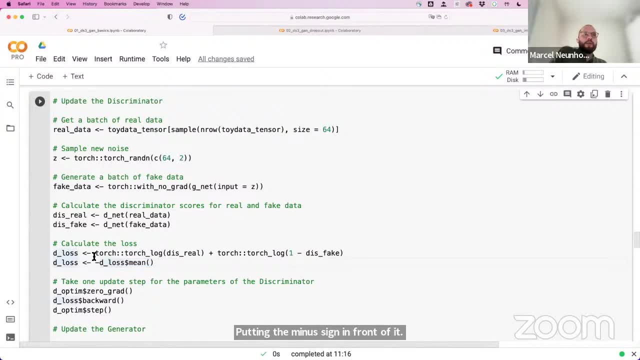 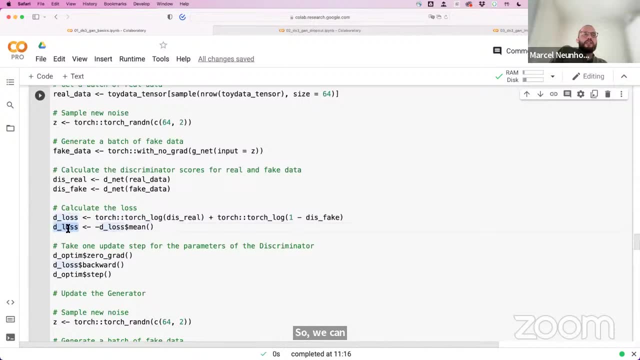 Make sure that we minimize, like this, portion of the loss. So we calculate the loss, So this is just a scalar, So that's just a value, a number, because we just average across, like this, a vector and take the negative of it. So this is how, in Torch, PyTorch, or Torch in R. 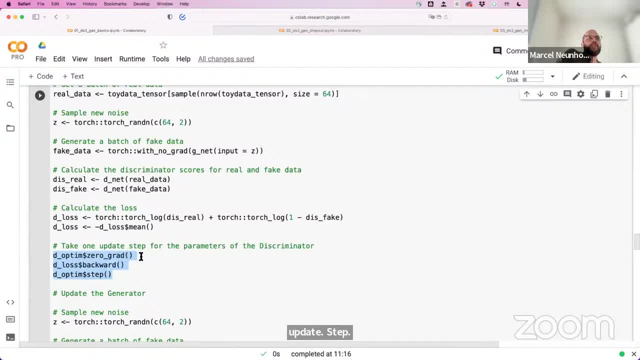 one updates. So this is what this step looks like. So we first zero all the gradients so that we don't have like weird accumulating gradients over time. So we are only interested in the gradient at this step. Pass the loss backward through the network. 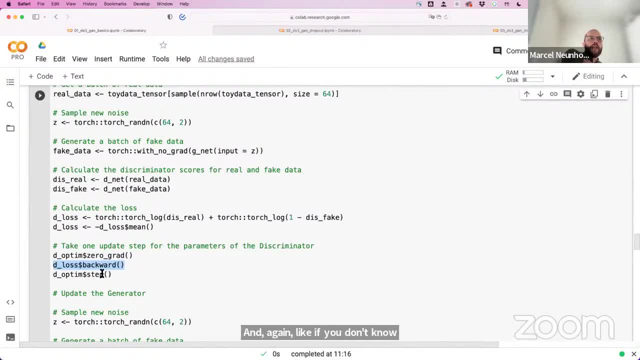 And again like, if you don't know what like back propagation means in neural networks, you're very welcome to dive into. like the video of last year's summer school on neural nets And when we calculated the basically the gradient update for every neuron, for every parameter in our neural net. 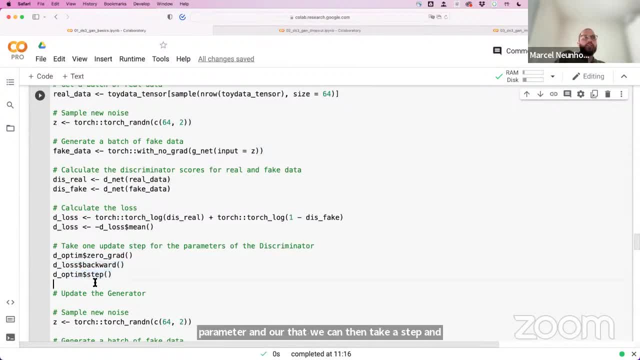 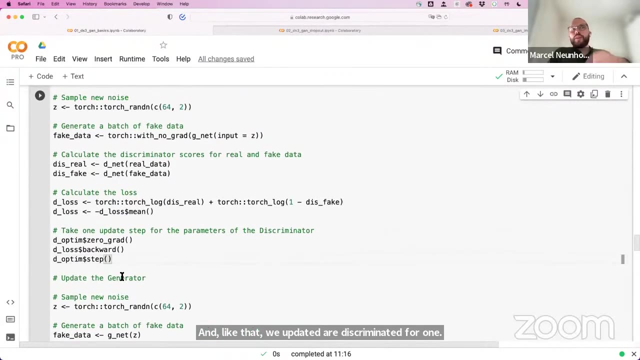 we can then take a step in that direction using our optimizer And, like that, we updated our discriminator for one step In classical neural networks. this would be it, Like we would put this into a loop, right, And then try to minimize this loss. 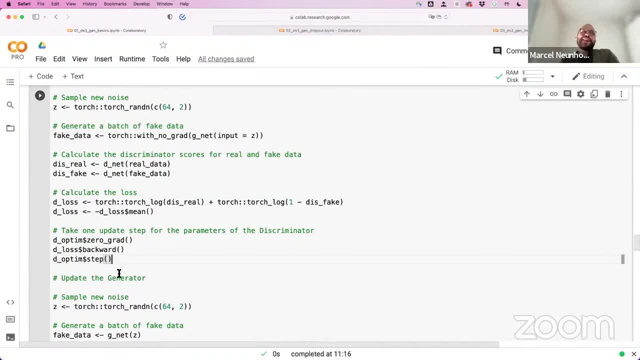 until we get, like, the best prediction between real and fake. But here we have, like this adversarial game right. So like this is only the first half of an update, step off like a gun. We also need to take care of the generator. 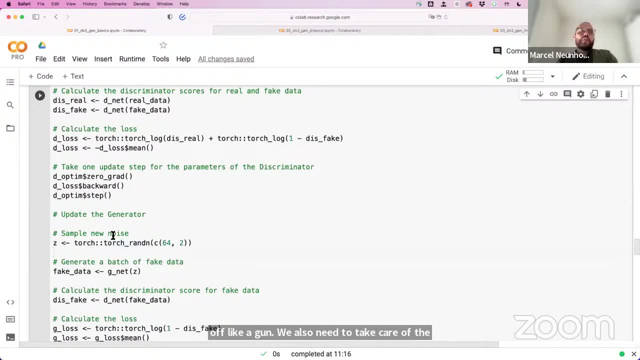 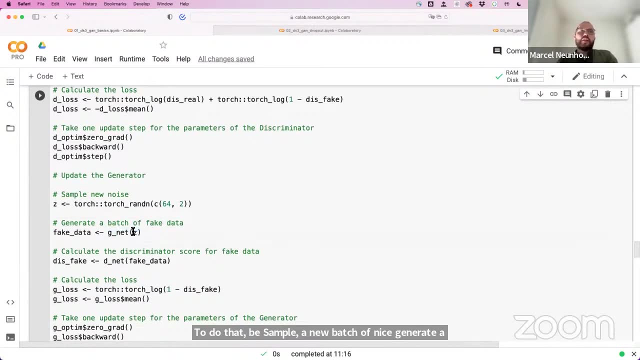 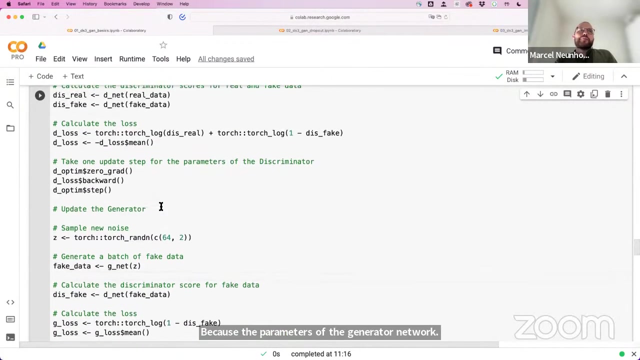 To do that, we sample a new batch of noise, generate a new batch of fake data, And we actually only need fake data in this step, because the parameters of the generate a network only depend on fake data, right Like in החсол. 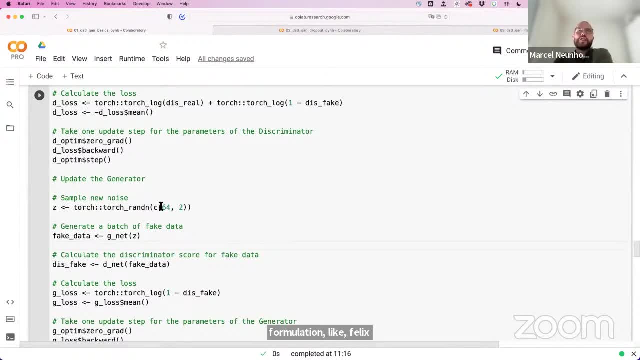 formulation like if feel we get at the real data data, we'd say that there is no G around there anywhere. Then we calculate the discriminator score for fake data, then just take the second portion. So actually we want to maximize this whole thing. 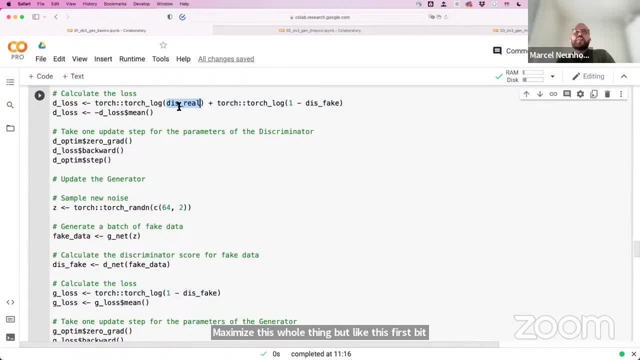 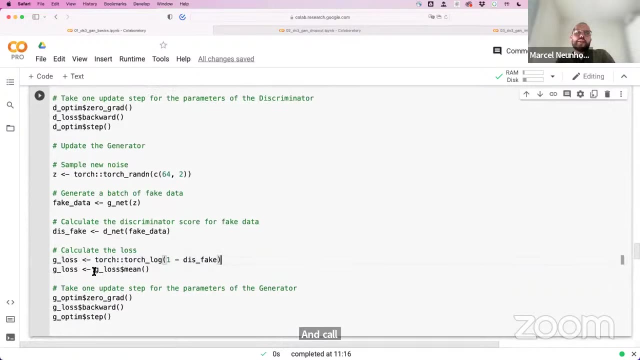 but, like this first bit doesn't depend on the generator at all, So we can drop it out and just maximize the second portion of it And calculate the- now, since we want to maximize it- the positive mean of that- and then take one update step. 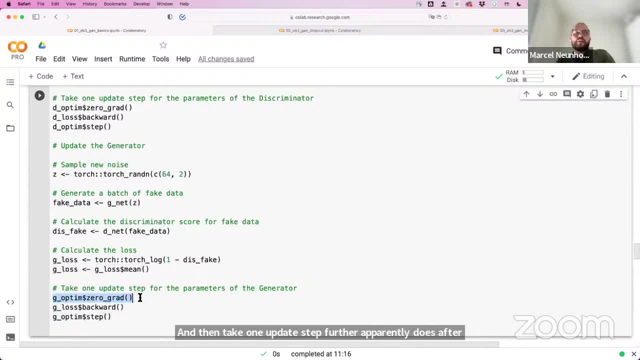 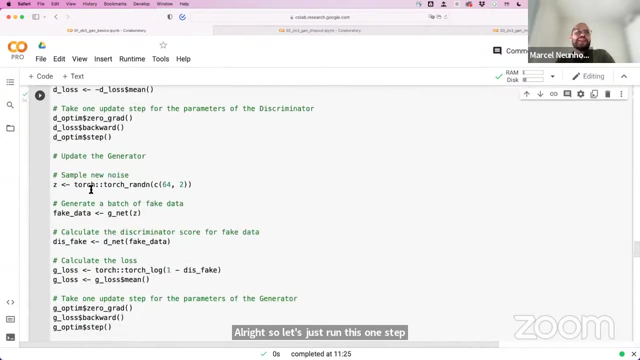 for the parameters of the generator, where we also zero out the gradients, first pass the loss backward and then take a step of our optimizer in the right direction. All right, so let's just run this one step for now, so that we can actually use our generator net. 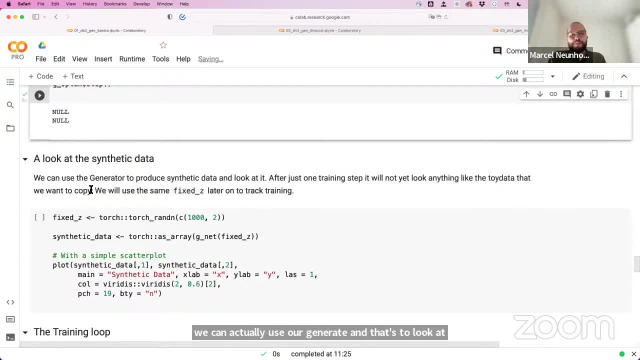 to look at some synthetic data after the first step. So we basically now, by running this code chunk, trained our first scan for one step on 64 examples, like a mini batch of 64 examples- real examples and 64 fake examples. 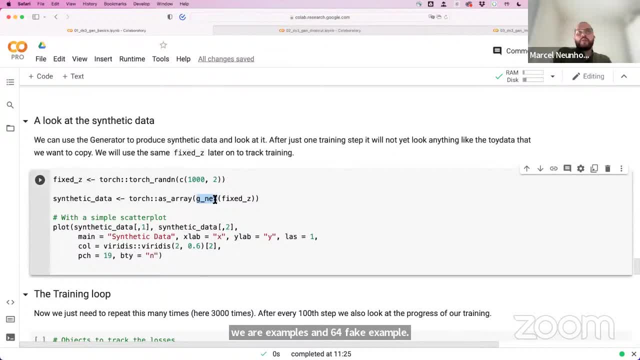 And now we can just use our generator net to produce synthetic data, right? So we just pass noise through the generator net and this torch S array. make sure that we get back in our object instead of a torch tensor, so that we then can have a look at it. 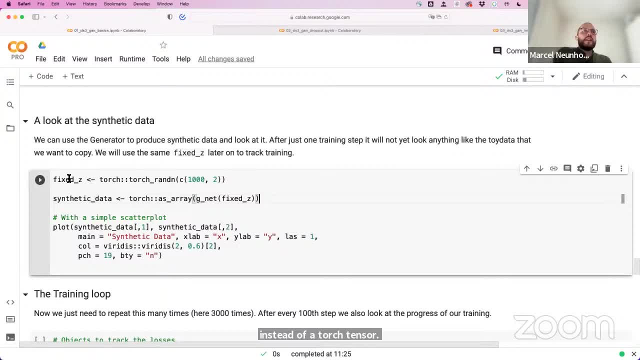 and plot our synthetic data after the first step. Here I will use a different noise vector than in the training. like this will just be a fixed noise vector. but it's not. it's just a fixed noise vector, Like drawn from the same noise distribution. 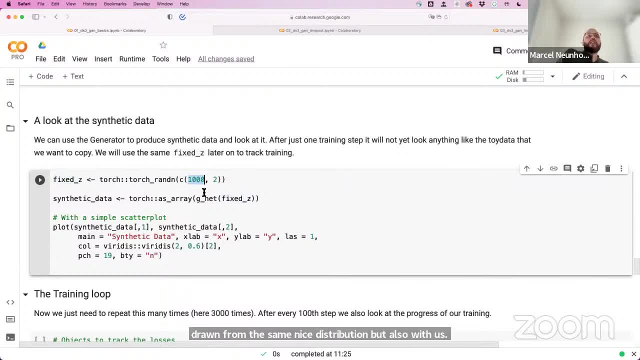 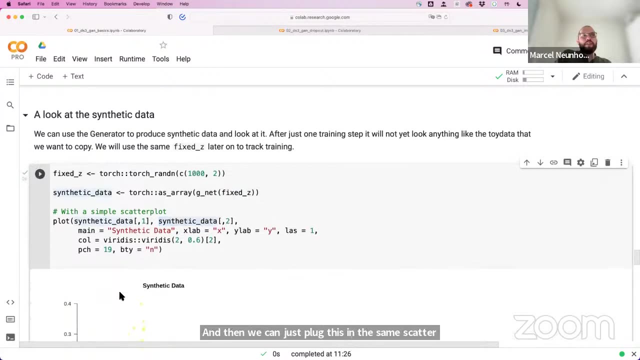 but also with 1000 examples, so that we get as many fake points as we had real points. And then we can just plot this in the same scatter plot as we had before And, of course, like you remember, like for the real data. 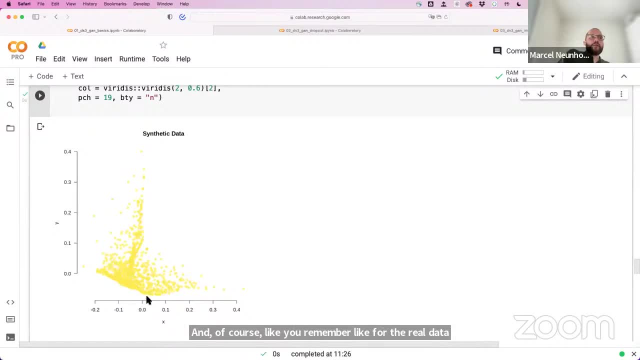 we had like this parabola around like the, a minimum, around zero, and then like it was going up to like eight and nine and 10.. So this doesn't look like anything like the real data, right? So this is just after the first step. 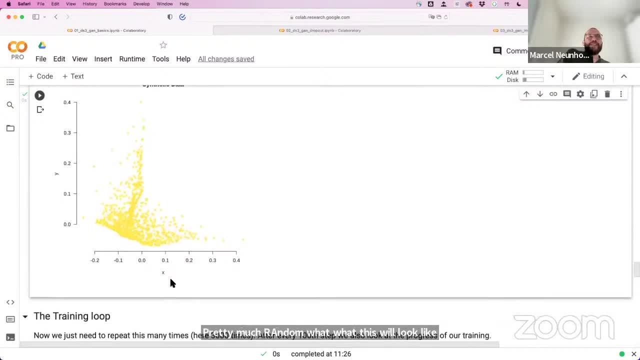 pretty much random what this will look like. So what do we need to do now? We, of course, need to train this for longer, so that we can actually get closer and closer to this equilibrium or, in the best case, even reach an equilibrium state. 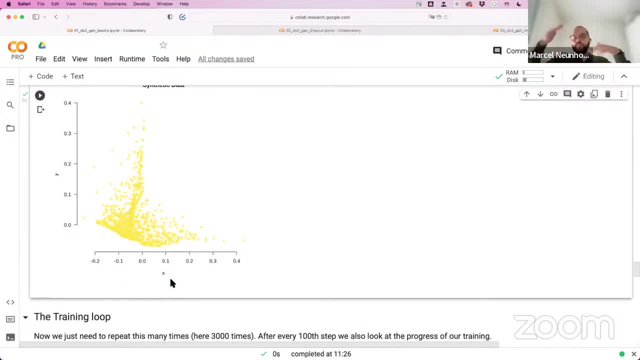 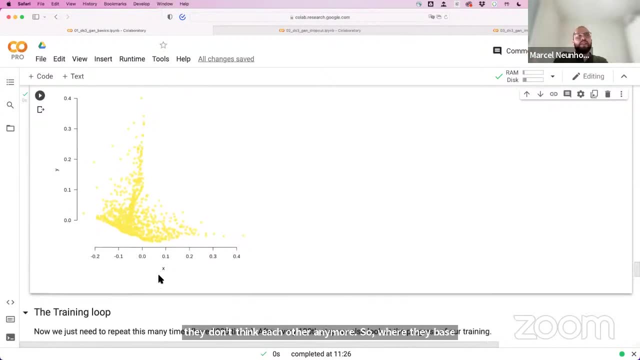 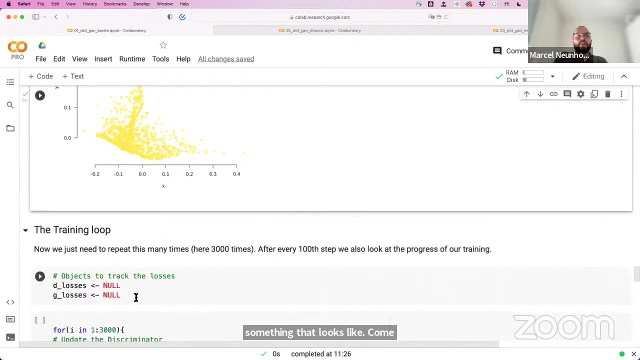 between the generator and the discriminator, where, like, they don't update each other anymore, So where they basically are in a stable state where the generator samples something that looks like coming from the true data distribution. So we will do this now for 3000 times. 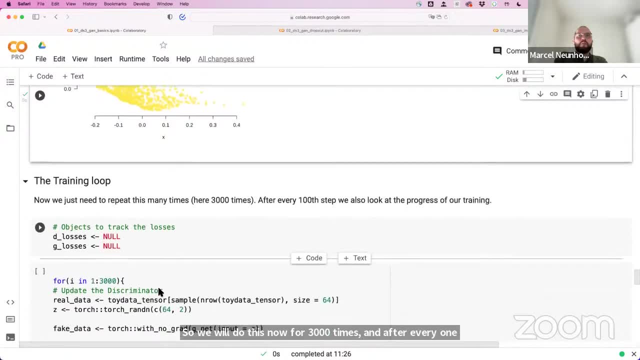 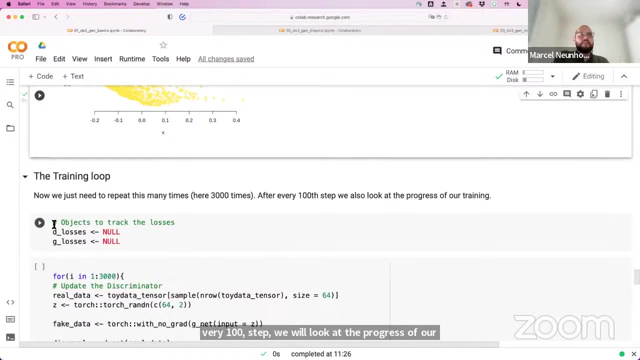 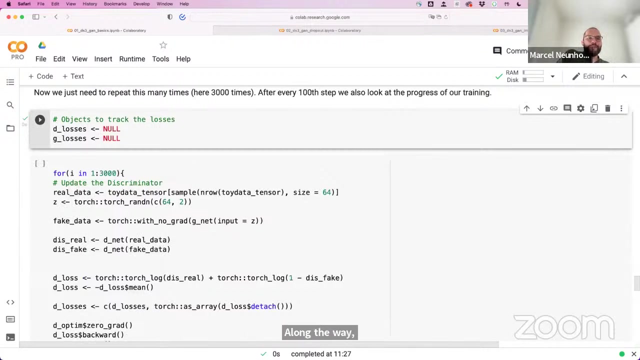 And after every 100 step we will look at the progress of our training, to observe. And since we observe the training along the way And there's like a great question in the chat I just saw in the corner of my eyes, So should everyone have a random plot? 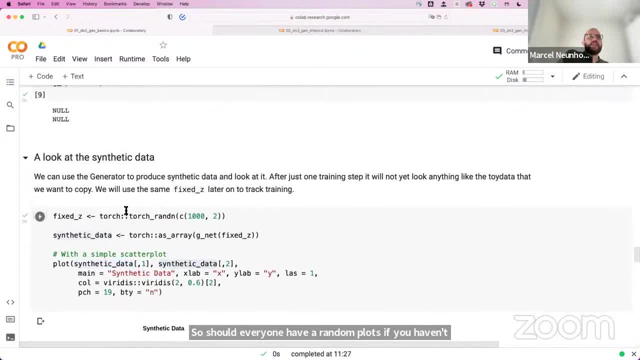 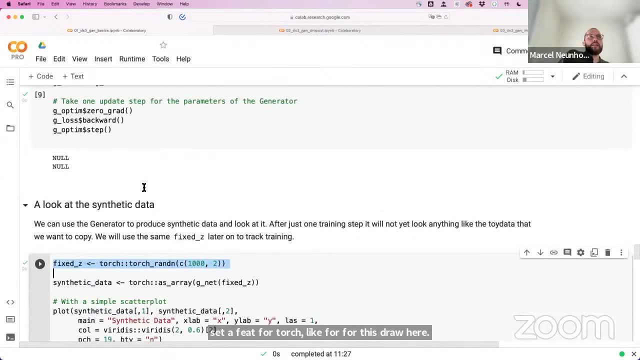 since we haven't set a seat. That is exactly correct, Like we haven't set a seat for torch, like for this straw here, So that's different for everyone. And we haven't set a seat also for the initial state of the networks. 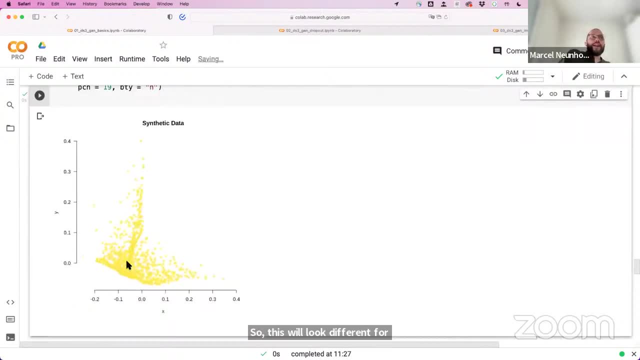 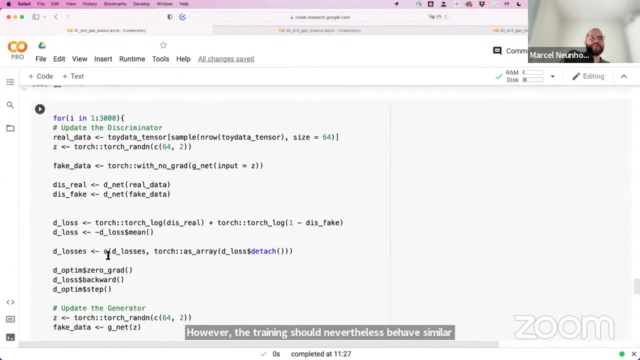 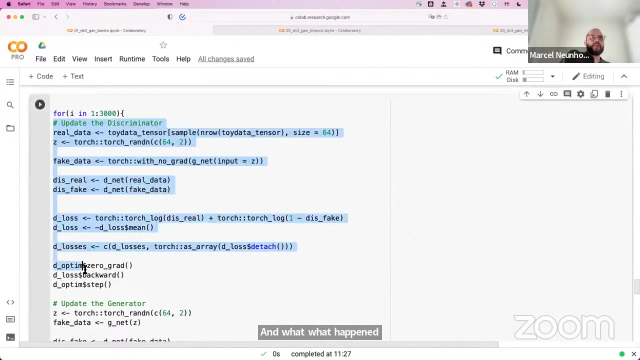 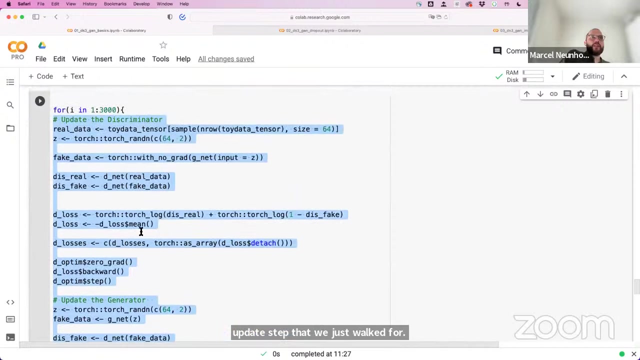 So this will look different for everyone. However, the training should nevertheless behave similar for everyone as well, And what happens here in this loop now is like the, the update step that we just walked through, right Like those two parts first updated discriminator. 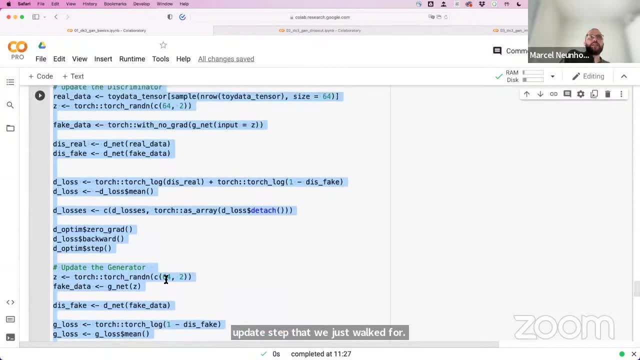 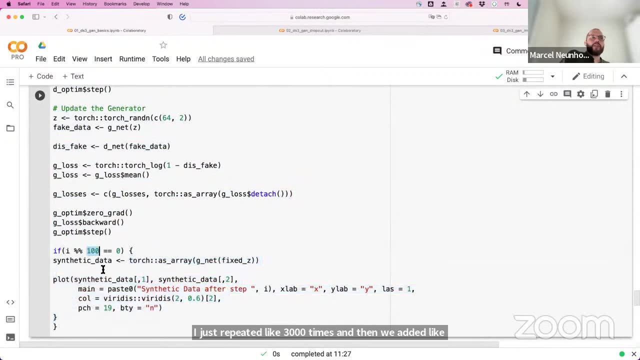 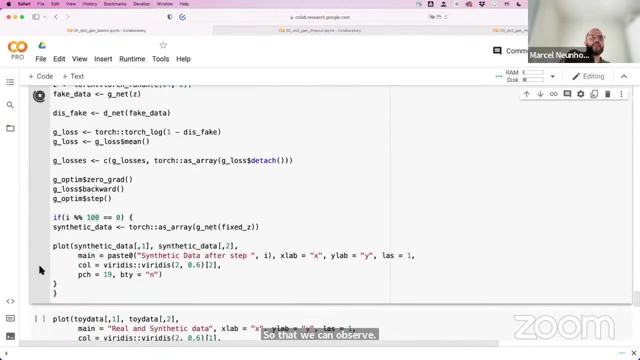 then update the generator. I just repeated like 3000 times. And then we added like this: getting synthetic data and plotting it after every 100 step so that we can observe training. So that's really from scratch, and just now we'll take some time. 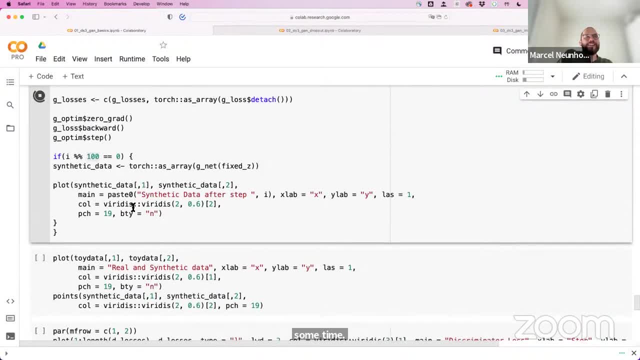 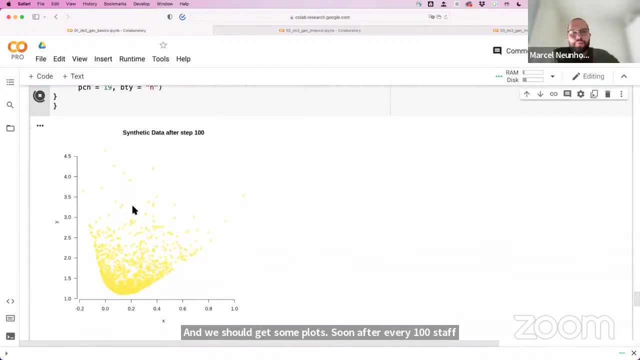 we should get some plots soon after every 100 step. Marcel, there is a couple of questions in the meantime. So there was someone was asking: there is an error of G underscore, NAT not found, So which means that probably that object was not created. 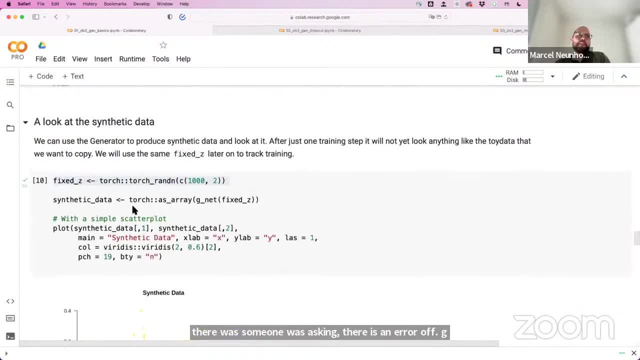 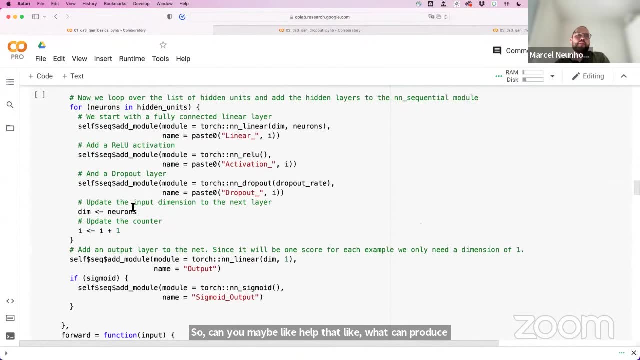 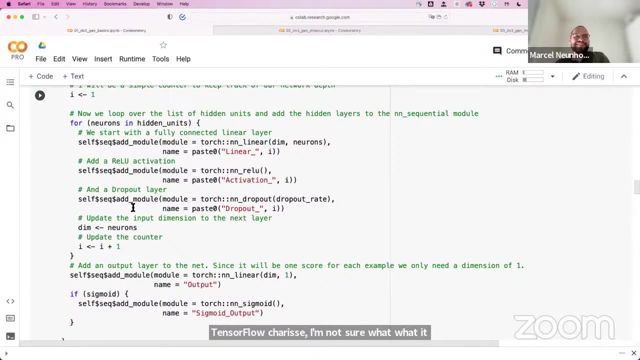 So can you maybe like help with that? Like what can produce that error? And another question is: how about TensorFlow, Keras? I'm not sure what exactly is the question about TensorFlow and Keras, but if the question writer wants to ask out loud, 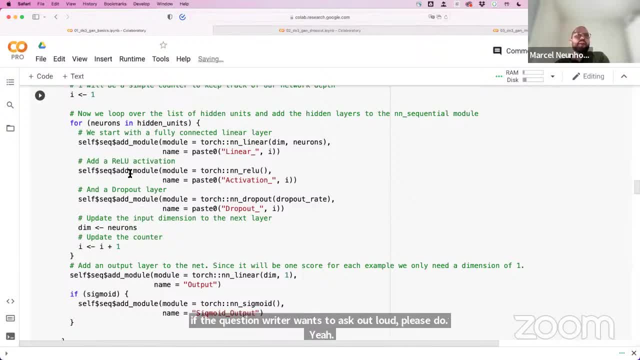 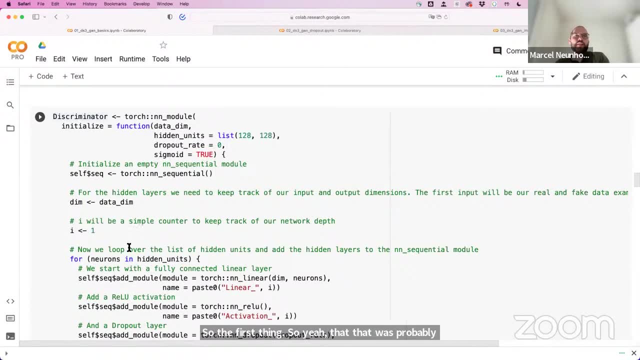 please do. yeah, So the first thing. so yeah, as Olga said, this probably means that, like the G NAT wasn't created before calling it and that like this training stuff. So just make sure that, like, everything is run in order. 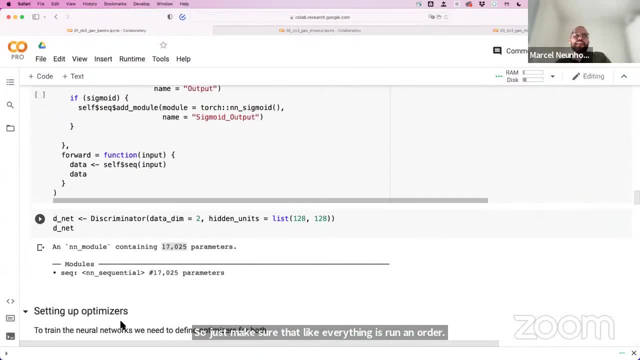 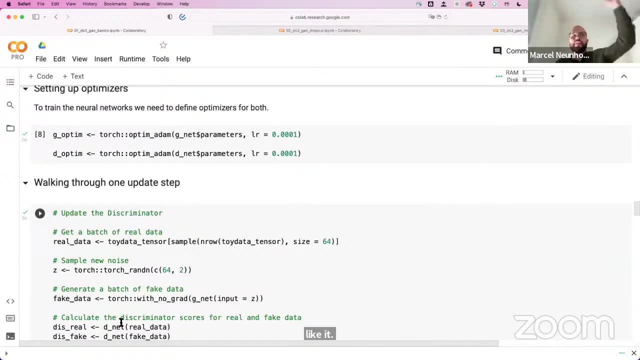 So that, like it can actually access like those objects when they're needed And if it doesn't just go back up, like to wherever G NAT is graded and start from there again and run the whole sequence again. How about TensorFlow Keras in place of PyTorch? 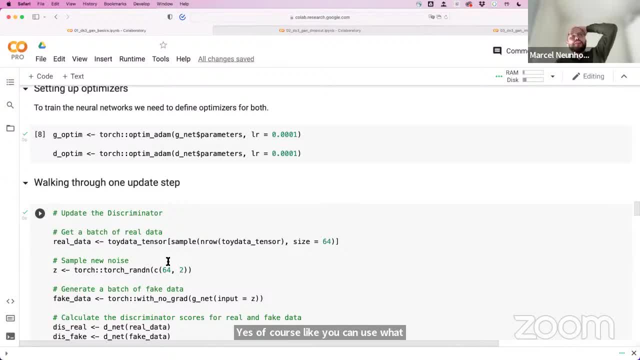 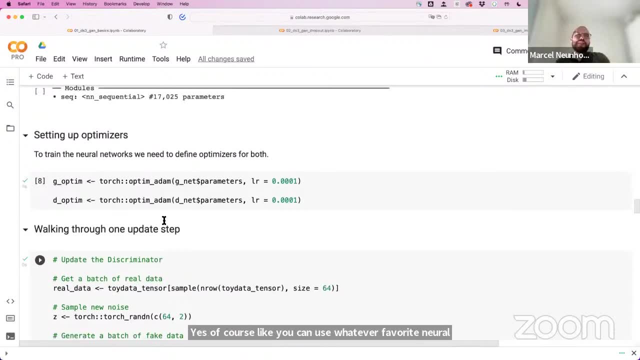 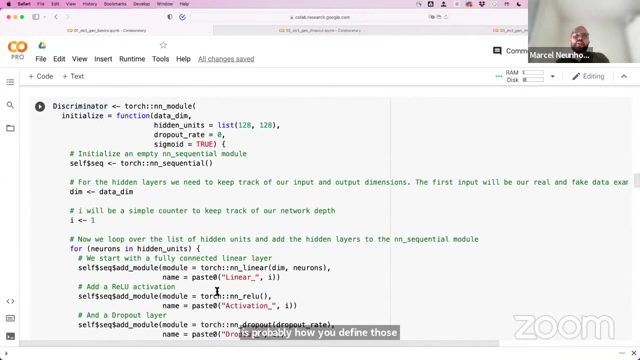 Yes, of course, Like you can use whatever favorite neural network API, or even your own neural networks, in place of that right, So what you would need to swap out is probably how you define those networks, So using, like the Keras or TensorFlow API instead of that. 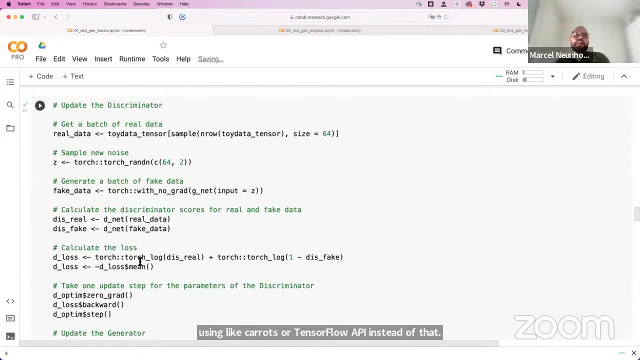 And, like then, calculating the length of time, the loss and back propagation, is very similar. You would need to use TensorFlow functions here instead of torch functions. just make sure that you actually use functions from the neural network API that you work with So that, like, all the gradients are calculated. 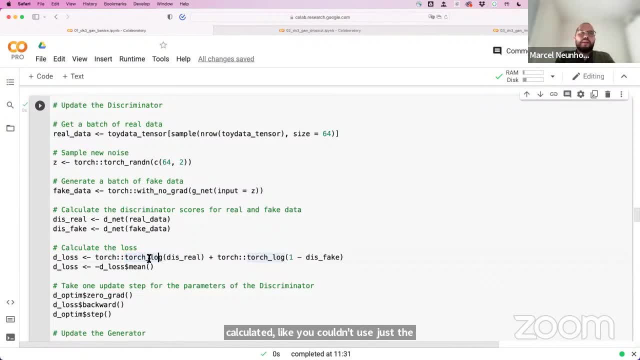 like you couldn't use, like just the base are log here, for example, Or in Python it is often compatible with like NumPy log, but like it would be very similar in principle And then the updates that might look a bit different as well. 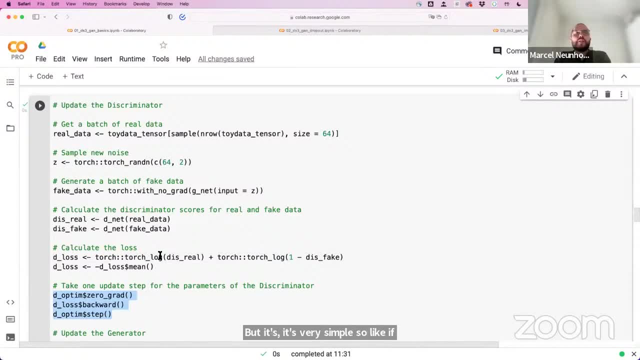 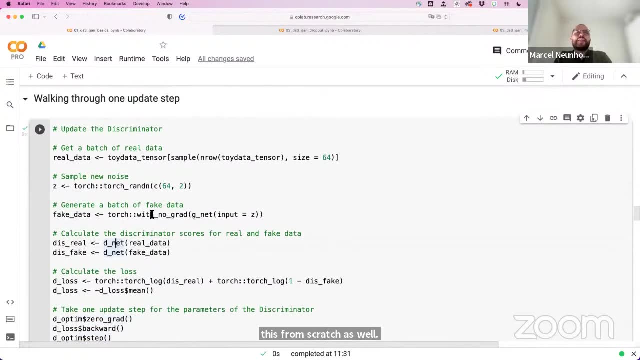 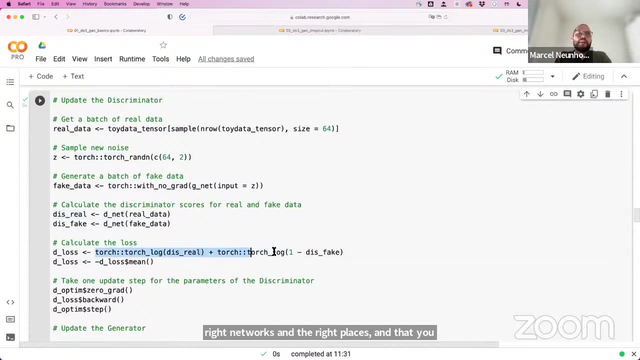 but it's very similar. So, like, if you want to do this from scratch as well, like, you basically just have to make sure that, like, the right networks are in the right places and that you calculate the loss in a way that, like, the gradient is calculated in the network API. 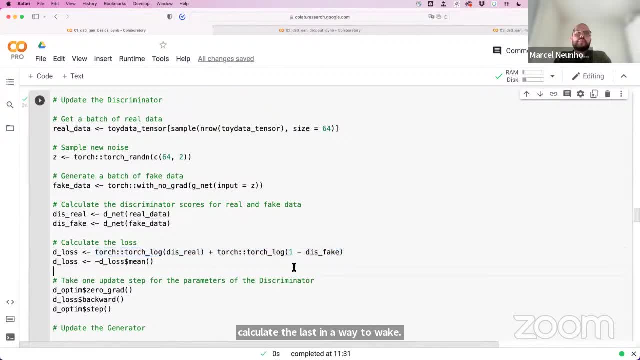 that you want to use, But I don't have no like code for this in TensorFlow Keras, if that's what you were hoping, but it would be perfectly like translatable. All right, let's look at like what our network does actually. 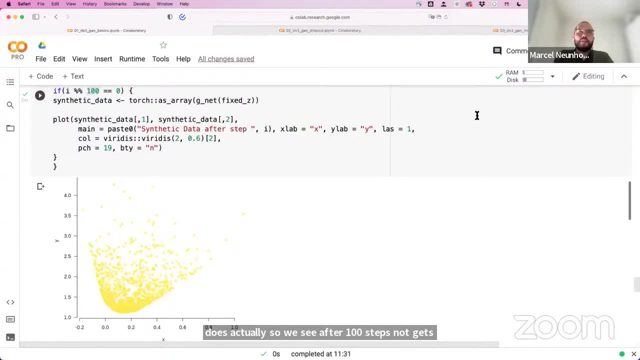 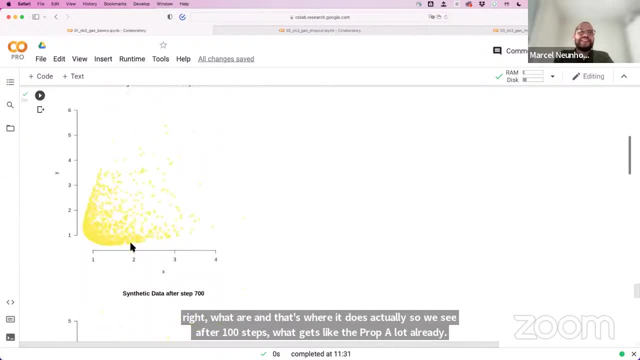 So we see after 100 steps, well, it gets like the problem already, which is great, but then like flips it around a bit, This looks weird. Let's see where we are Actually: ran for 3,000 steps already. 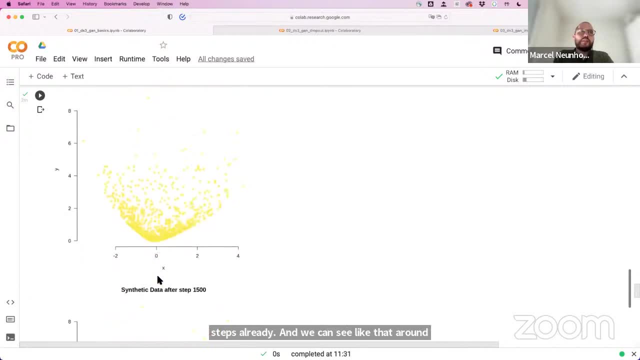 And we can see like that around, like step, 1,400, 1,500. It just looks weird. It starts to produce something that at least looks like in the similar demand as our original data, And then this gets better and better. 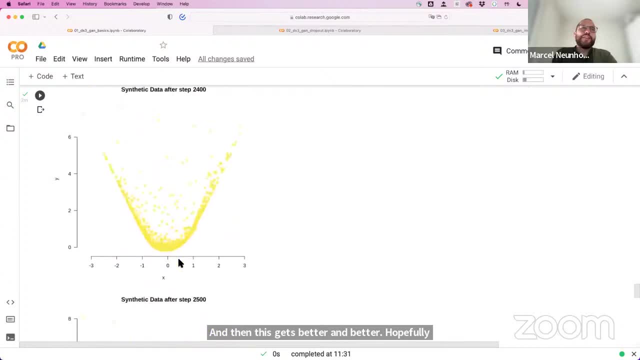 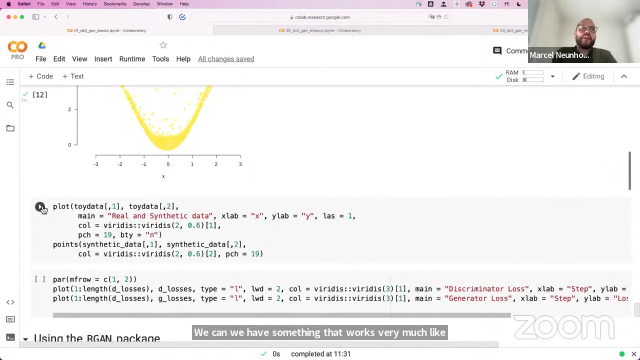 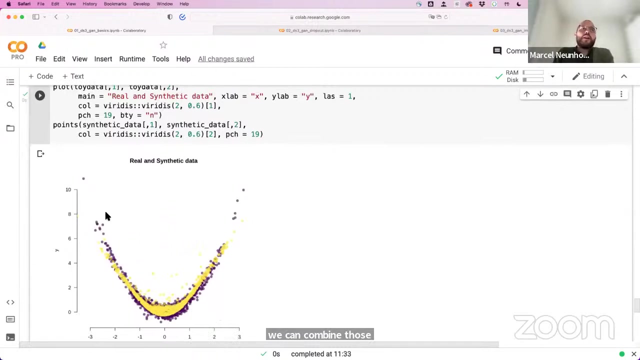 Hopefully it does, So that after the 3,000 steps we ran it, for now we can- we have something that looks very much like the parallel that we had To actually see, that in one plot we can combine those two data sets. 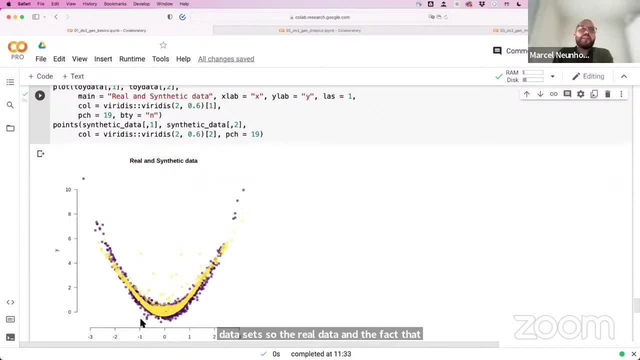 So the real data and the fake data into one plot And we can see that it's actually pretty good, Like there's still some noisy top points inside the parabola here And like it might be a bit off here, but like this might get better and better. 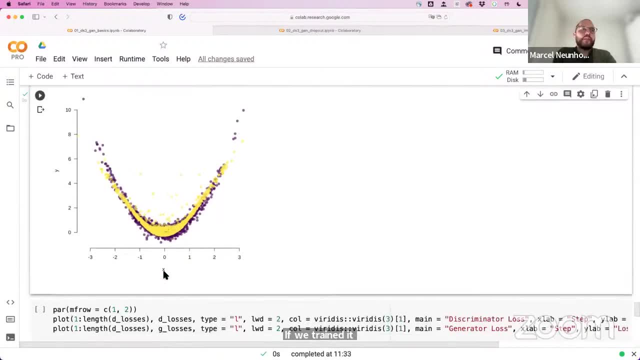 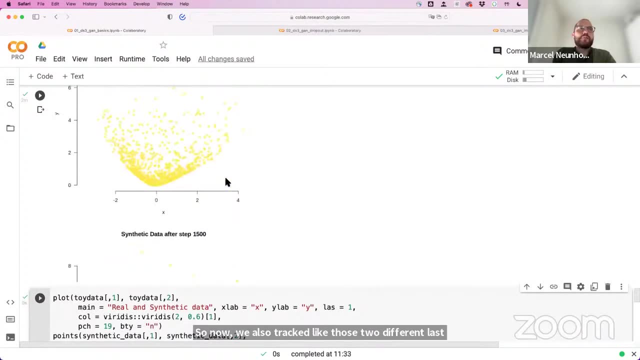 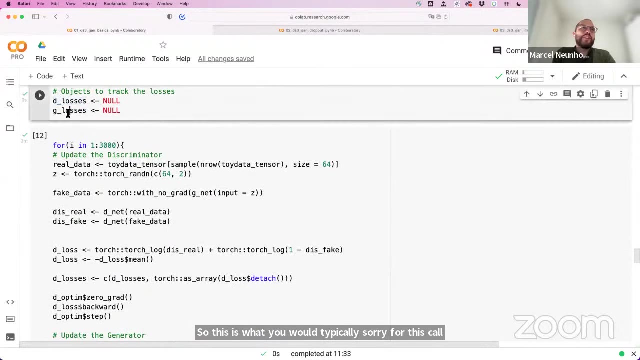 And then we can see that we've trained it for longer. So now we also tracked, like those two different losses, right? So this is what you would typically sorry for the scrolling here. So those two objects here where we add each iteration. 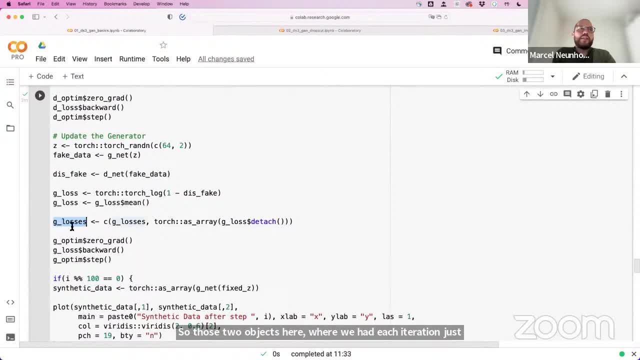 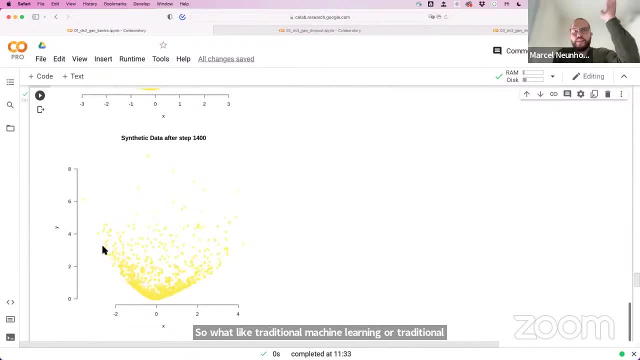 just stored the loss into a vector and here again, So with like traditional machine learning or traditional neural networks, we can see that we have a lot more data. So what we would like to see is like a decreasing loss curve, right Like we would like to see that this approach is a minimum. 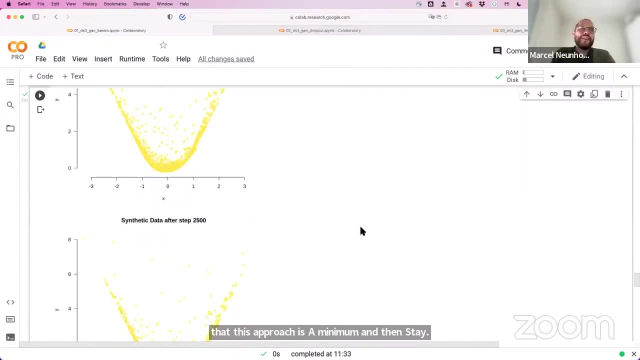 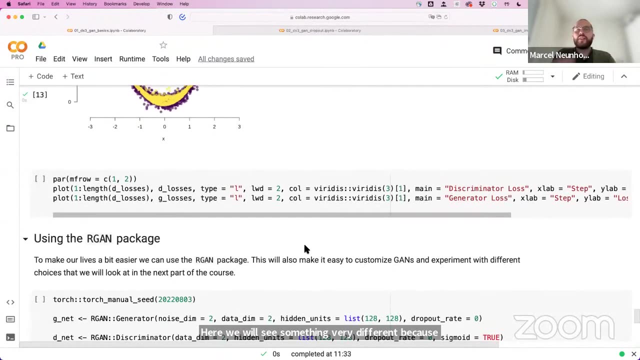 and then stays stable at the minimum. Here we will see something very different, because we have like this adversarial nature, like this game, where those two networks are pitted against each other, And so the first plot will just be the like a line chart of the discriminator losses. 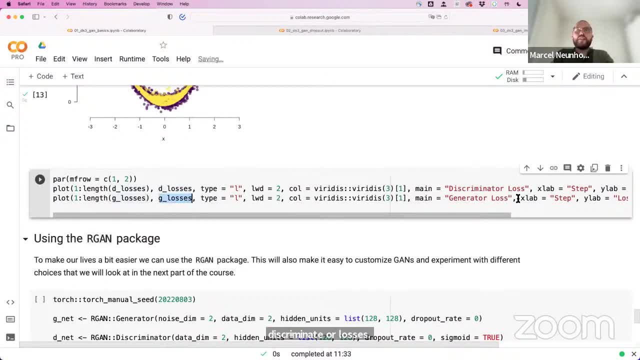 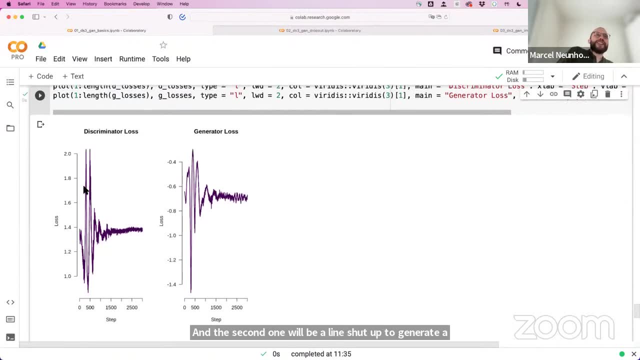 And the second one will be a line chart of the generator losses. And we will see that this doesn't have like this nice shape of like where we have a nice like decreasing curve as we probably know them from like a lot of machine learning models. 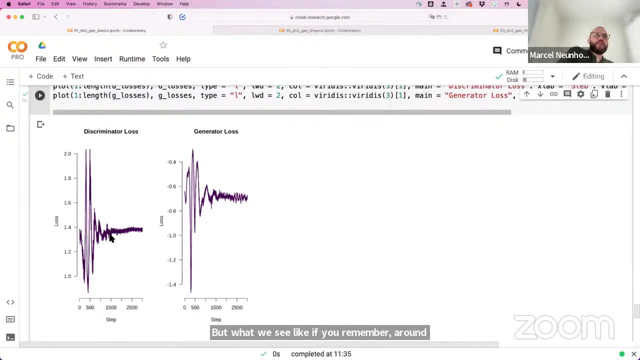 But what we see like- if you remember, around step 1,400,, 1,500, the generated synthetic data looked all in the right domain already, and then better and better. So what we can see is basically that here, like those two networks really fight against each other. 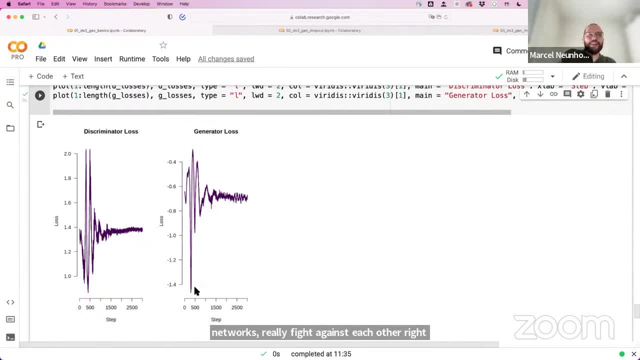 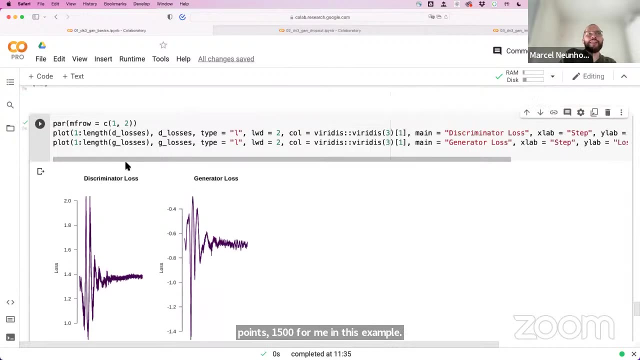 right, Take one step in this direction, another step in the other direction And then it starts to stabilize around like this step- 1,400, 1,500 for me in this example- And stays rather stable there. And this is like also when we like, see that, like the quality. 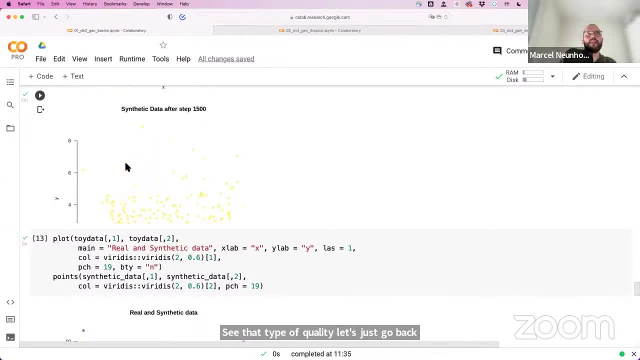 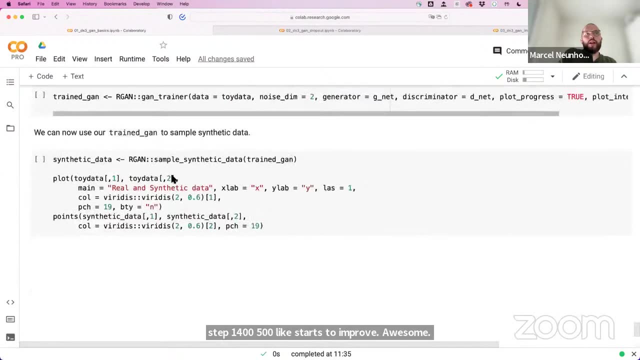 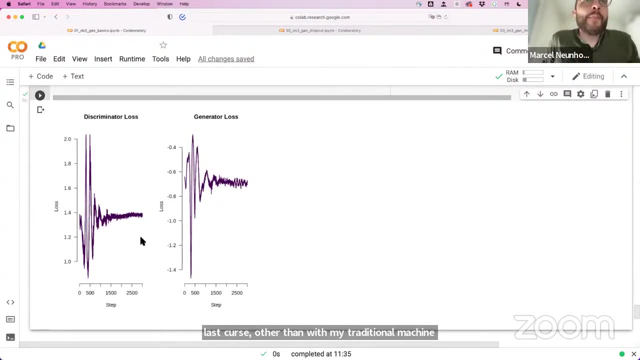 let's just go back to this. what's that? 1,400,, 500, like starts to improve also Like. one problem with those GANs is like from those loss curves other than with, like, traditional machine learning or neural network models. 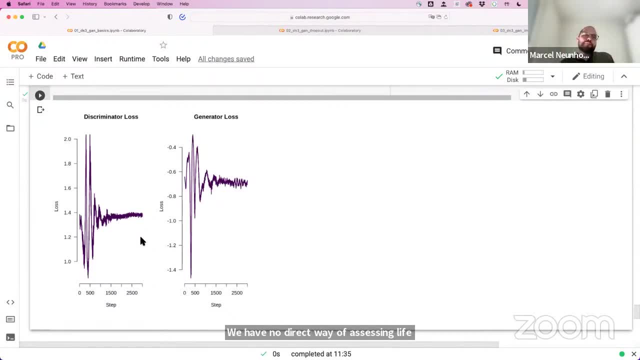 we have no direct way of assessing like the quality of, like the generated data there, So like it's therefore also hard to come up with, like early stopping rules, or like trying to figure out when to stop training, and like- yeah, I guess the best heuristic we have here. 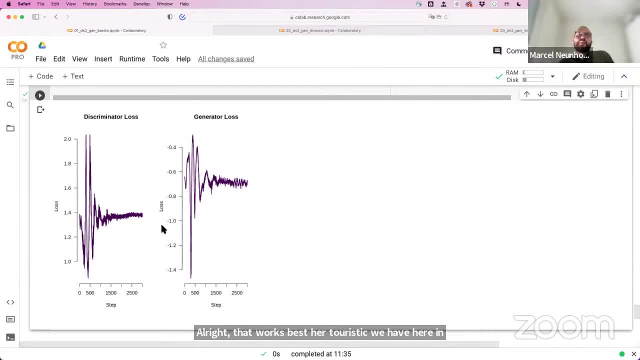 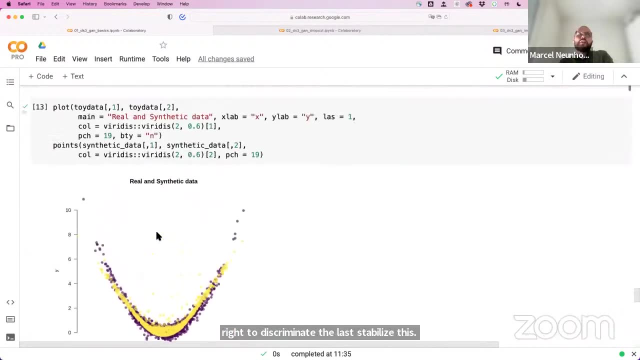 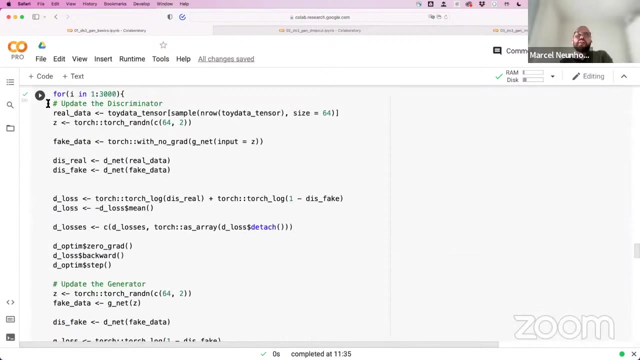 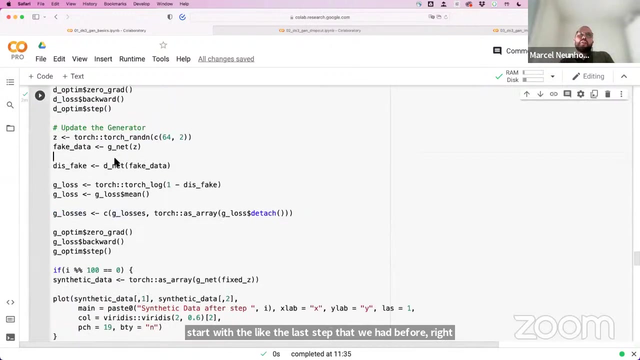 in this traditional GAN framework is to see whether rights, just discriminator loss, stabilizes to some extent. And now you could, of course, continue training, right, Like we could just rerun this, and then it would start with, like the last step that we have before light. this is all stored in those. 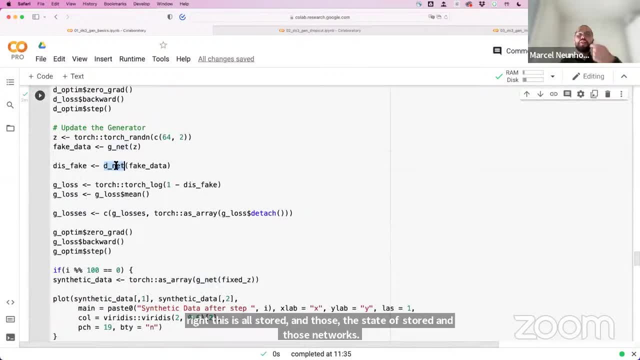 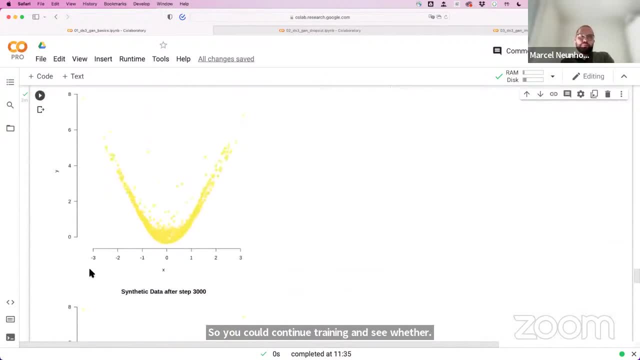 the state is stored in those networks so you could continue training and see whether- and it probably will improve the synthetic data even further. however, i'm satisfied with like, satisfied with this outcome, like uh, and i hope, uh, you are too like, i hope that, um, you can see how, like this, these two networks, um, and this training loop that. 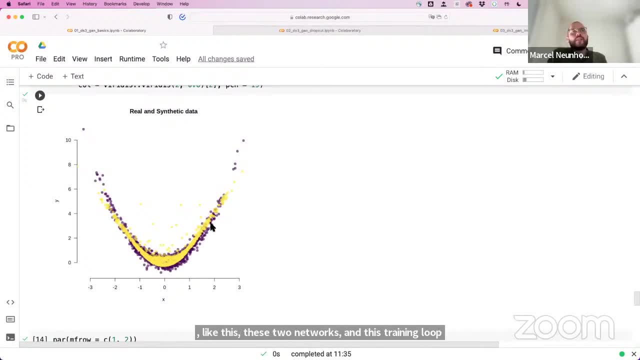 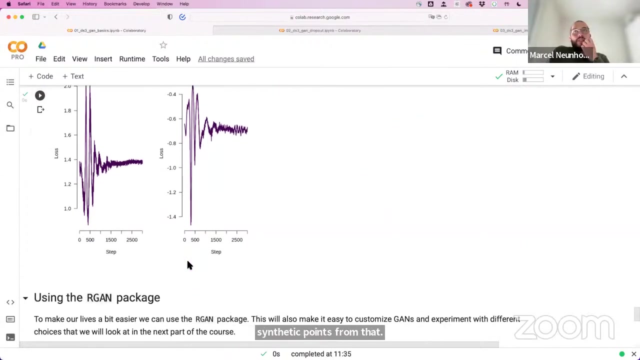 we coded from scratch, produced a generative adversarial network um that we can use to learn, like this two-dimensional, rather simple but still like not trivial uh distribution and actually sample new synthetic points from that. so because, like this is of course very laborious and you don't want to do this um every time again. 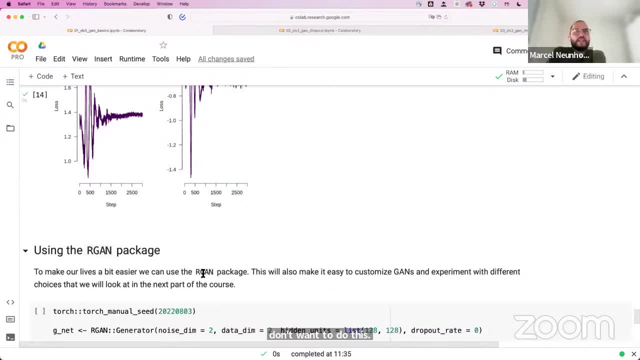 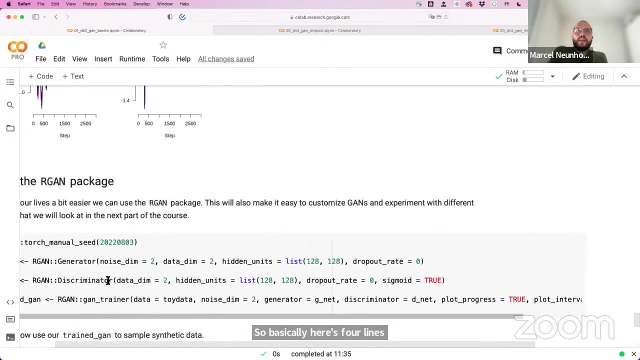 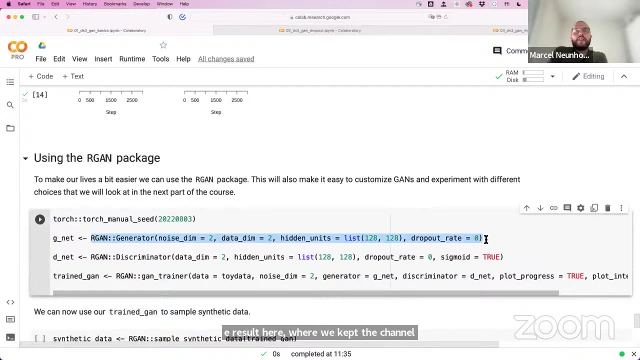 um, i coded up a little r package that makes makes your life a lot easier. um. so, basically, here's four lines: um, how to achieve the same result here. um, where we get, like the generator, and it's exactly the same function that you, that you see above. um, from the package to the. 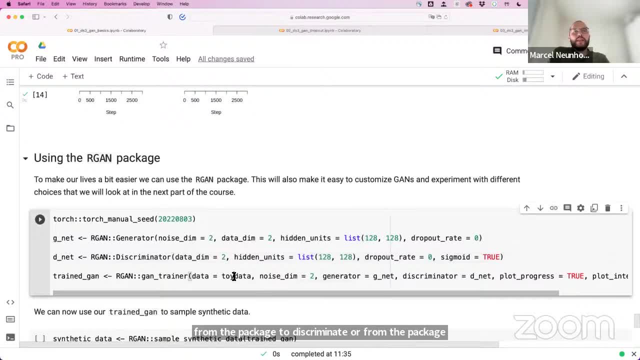 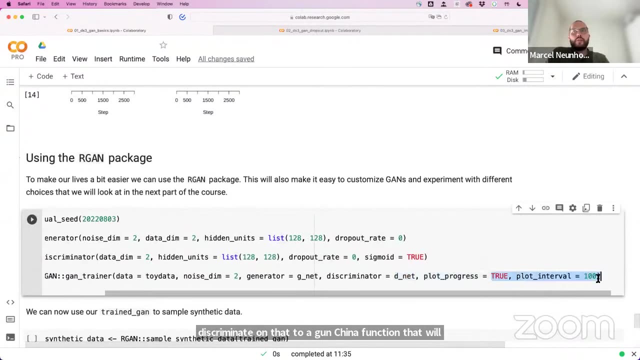 generator. then on the связzy block um to the discriminator network. you can just uh, generate the discriminator from the package and then you can just pass the data, the noise dimension and the generator that and the discriminator net to a gone trainer function that will take care of. 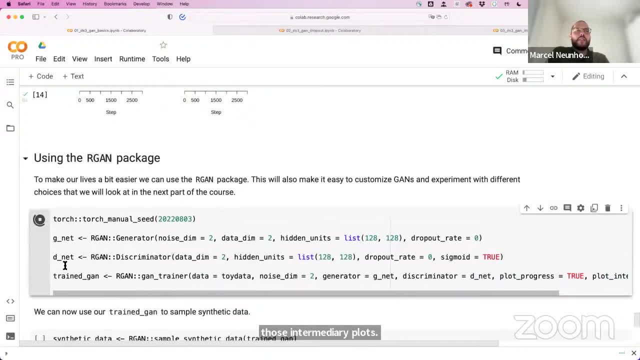 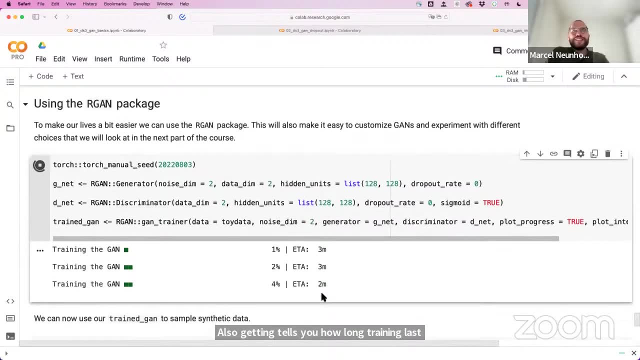 everything else, um, and you can also generate those intermediate plots, um, so that package um also tells you how long our training will last, which is not that interesting and not very useful in our example right now, because it's rather quick, but it will be very interesting as soon. 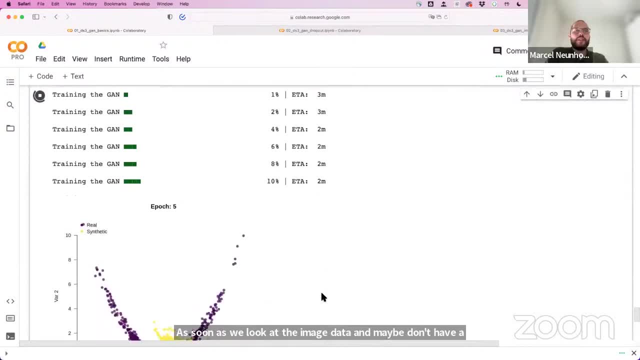 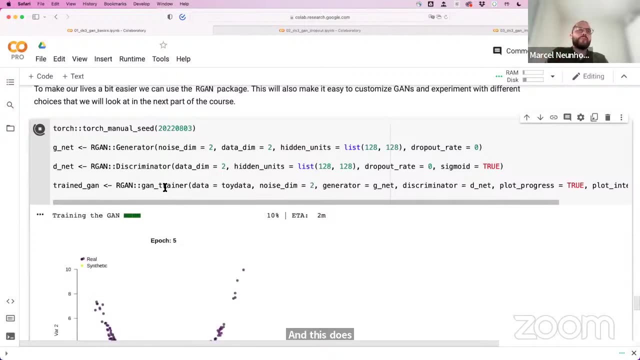 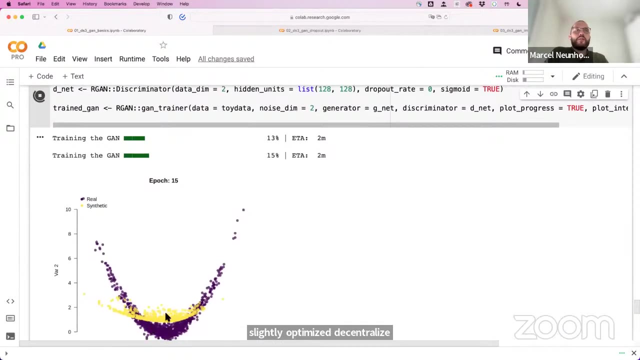 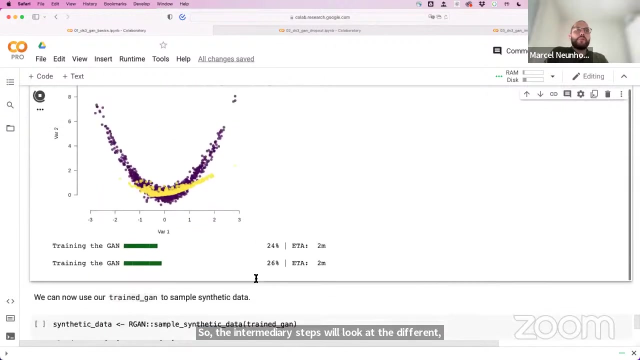 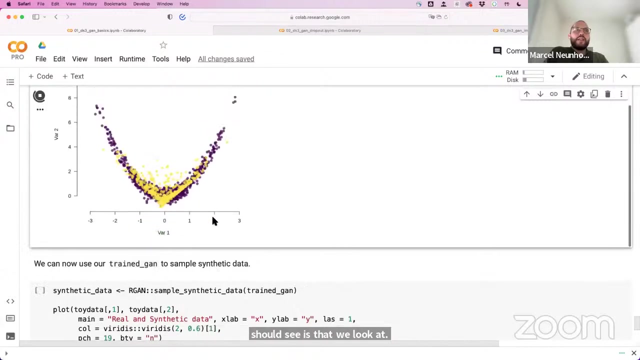 as we look at image data and maybe don't have a GPU available, and this default option of the GAN trainer uses some slightly optimized design choices that we will cover later, so the intermediary steps will look a bit different, but in the end, like after those two minutes, what we should see is that we will get like synthetic data that 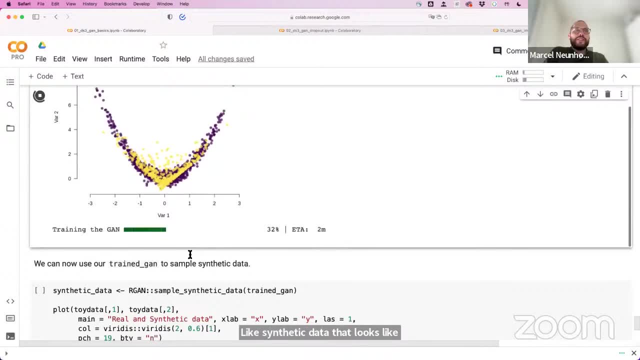 looks like it could be drawn from the real data. so 35%. so that's a good time to ask questions, and I see one in the chat like: why does the loss not give us information about data quality? that's a good question and it's like 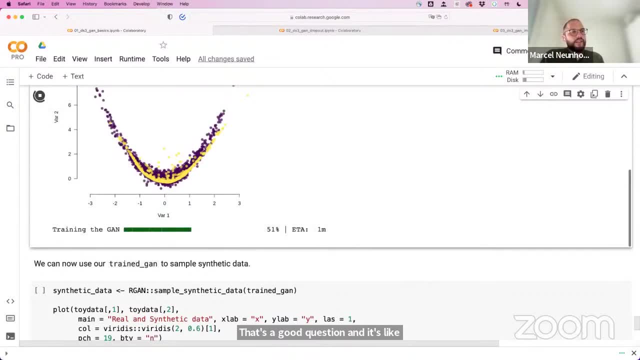 hard to answer. but essentially what we model here is not data quality directly right like we model like a game, adversarial game between two actors that try to reach an equilibrium. and we know from theory that in the equilibrium we should get like perfect data or perfect draws from the underlying data distribution. but 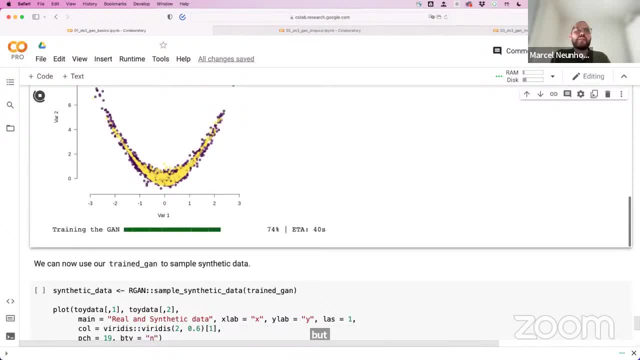 like we don't model data quality directly and classical neural networks, classical machine learning for prediction. like we directly model, like the loss directly models how good we are at predicting and therefore we can use directly this loss about for like maybe like early stopping, figuring out, like good points. 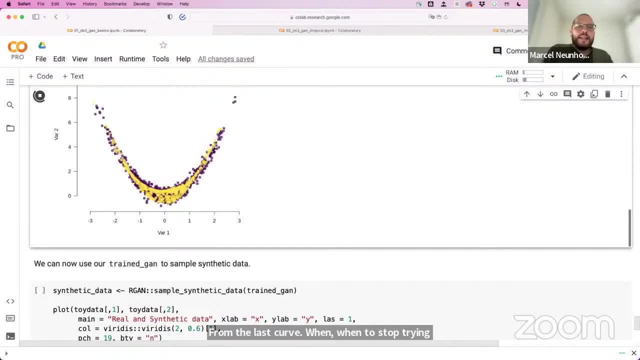 from the loss curve when to stop training, and in the classical GAN this is not possible like we're. all we get is like a feeling about whether we are close or in an equilibrium, but it doesn't tell us whether it's actually equilibrium. however, there is some like modifications to the value function. 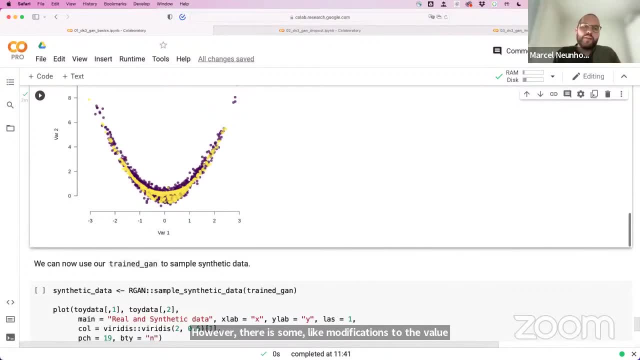 that allow us to actually directly interpret, directly interpret the losses that we get as some sort of quality indicator. so like that's only true for the, for the classical original GAN, but like there's improvements that will allow us to get a score that is correlated with quality. 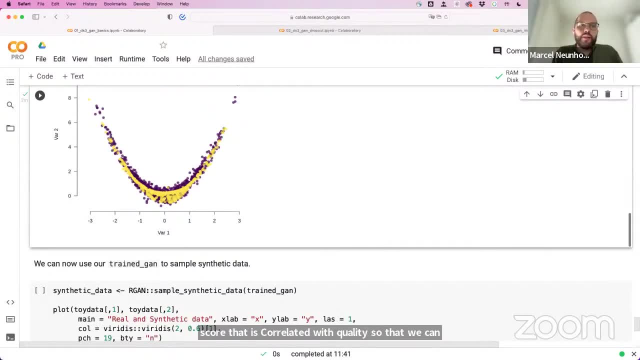 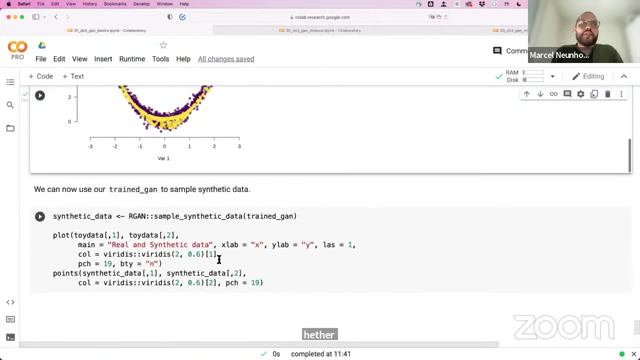 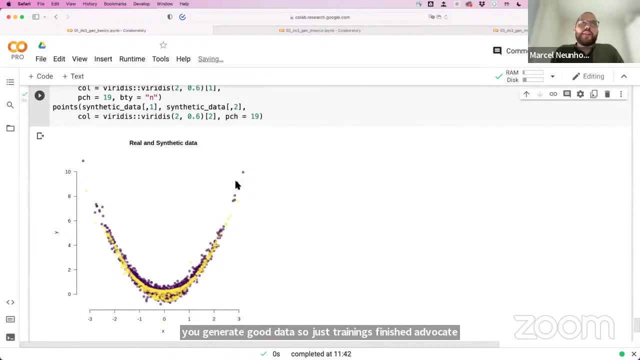 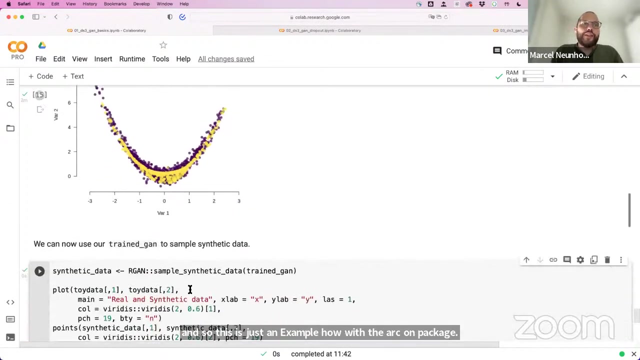 so that we can then actually also run those scores and for whether you generate good data. so this training is finished and we can look at the real and synthetic data as before. and so this is just an example how, with the argon package, it's a lot easier to train your GAN and to to look at it so like there's two more. 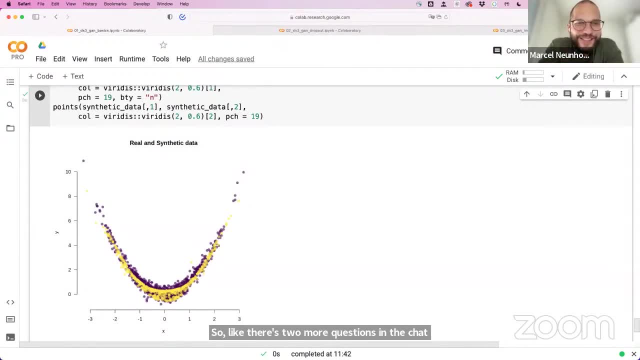 questions in the chat that I will try to answer. so if the first one is, if you would use a GAN to obfuscate privacy sensitive data, would you change the objective to each e-commerce close as possible to the original regression results as stated in your paper? that's a good suggestion and like that's a good way to incorporate, like. 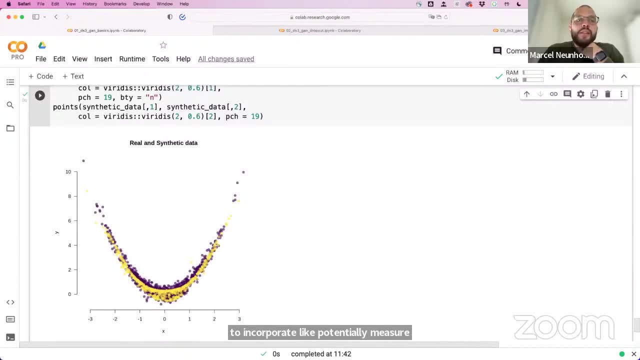 potentially measures you care about. however, it has the downside that you basically encode those models into your generative model as well, and if you use GANs, and especially for synthetic data that you want to pass along to other researchers maybe, where you don't necessarily know ahead of time what kind of analyses they would like to run, 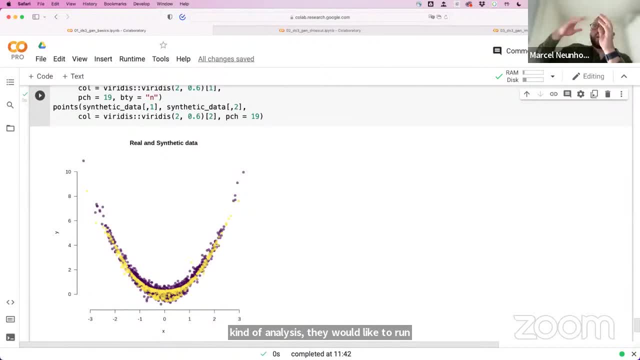 this is probably not what you want, right? if you know exactly that you want to run this regression or the set of regressions, then this would make sense and this should also improve, like the utility for those tasks as, yeah, you will directly minimize or maximize, like this. 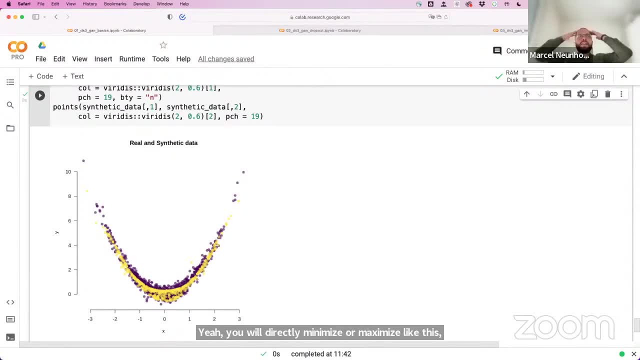 this loss when learning the GAN. but then the question is, why would you need a generative model at all? like couldn't you just learn, like those regressions privately on the original data and then report those regression coefficients? if that's all you're going to do, 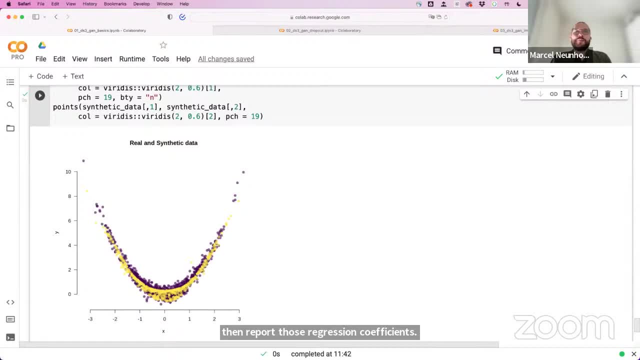 Thanks Janice, Thank you Alex, Thanks Gideon, Thanks care about. So I guess this is a trade-off of the GAN trying to be as general as possible, also learning relationships in the data that you don't explicitly want to encode, Of course. 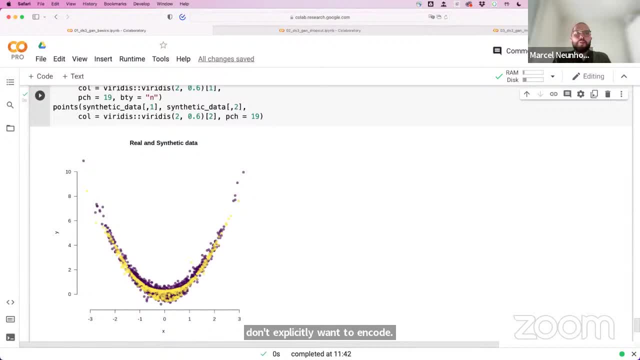 with the GAN loss you also encode implicitly some relationships that you care about And at the same time having high utility for a specific task, like if the goal was just to be accurate on those tasks. it would make a lot of sense to add this to the value function in some. 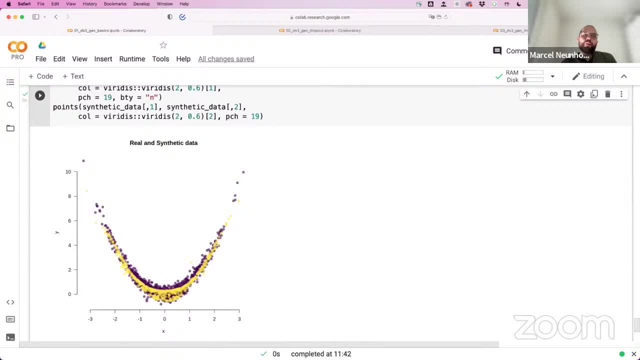 way. But the goal with privacy protective synthetic data is to allow more analyses, and analyses that you maybe don't even know about. like that, downstream users can choose. And then there's a second question: Could you quickly explain the dropout rate again, and are there any cases where noise dim should be different from data dim? 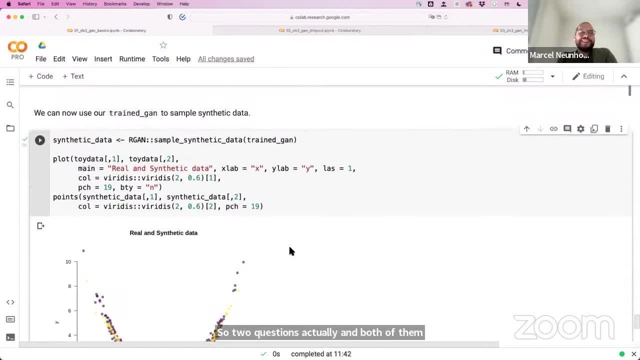 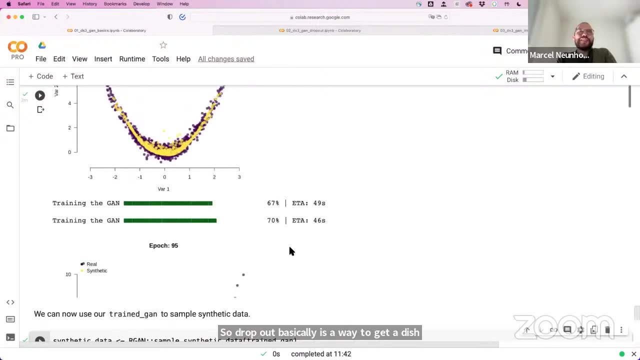 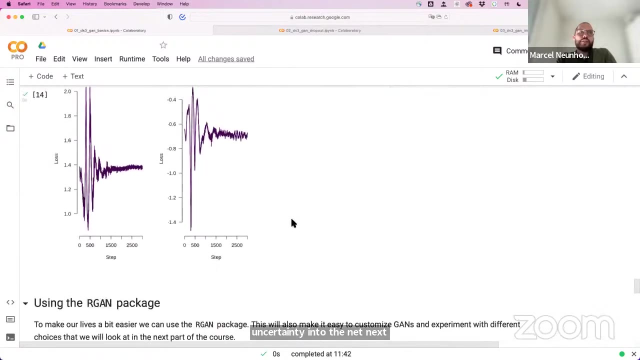 So two questions actually, and both of them very good. So dropout basically is a way to argument falling out That's the mild layer measurement that goes into it. So what dropout set basically is what you get- additional noise uncertainty into the networks. 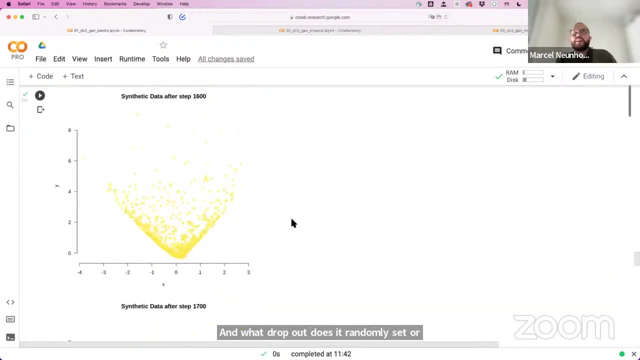 Let me just scroll up. sorry for the quick scrolling. And what dropout does it? randomly sets, or basically: Speaker 3: Speaker 1. Speaker 3: takes out. crosses out Speaker 1. Speaker 3: Pre-specified percent contrasts. 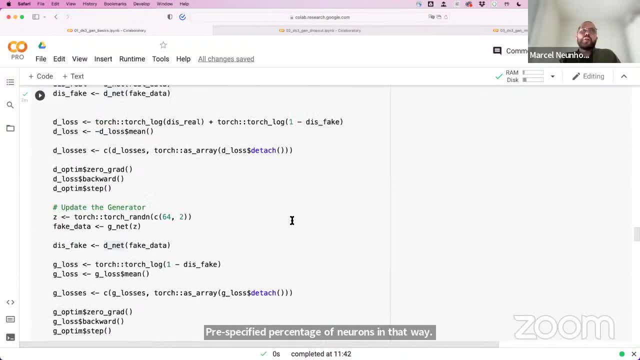 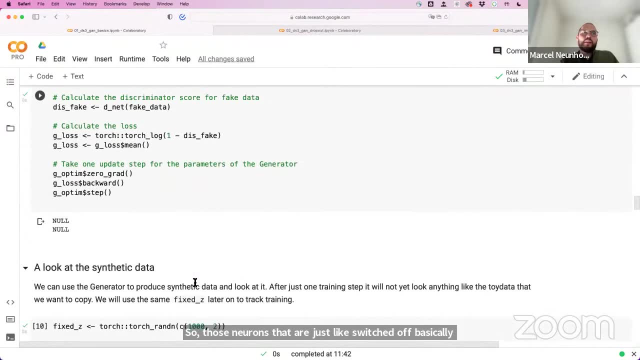 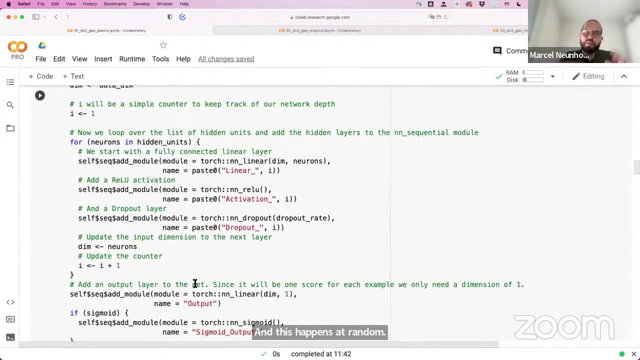 of neurons in that layer. so those neurons that are just like switched off basically- and this happens at random- don't contribute to like the prediction or to the generation of synthetic data in this particular step. however, they still need to learn something or they will learn something, because they are not switched off in every round, right? 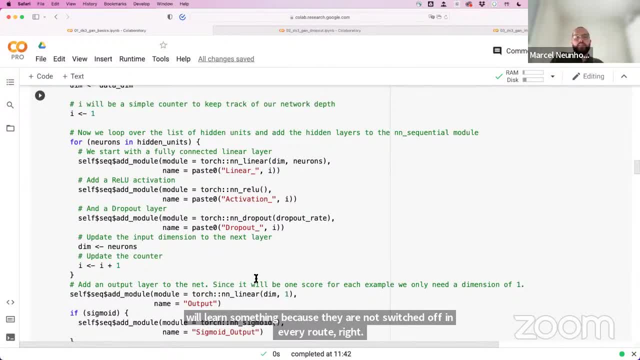 so basically, you have like only a subset, a random subset of all the neurons available at each training step, and what this helps is that helps against overfitting because, like, basically, all neurons have to learn to generalize in some way right and in a combination- um, they cannot specialize on like one. 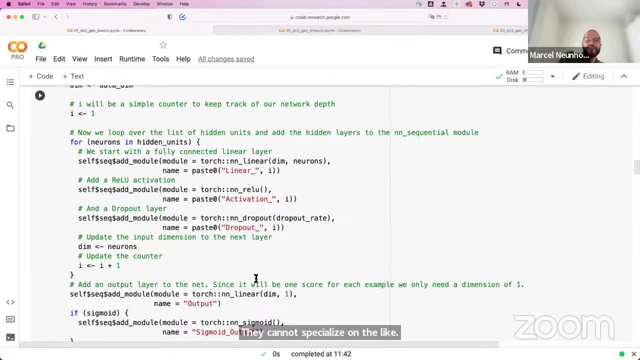 one, one feature, one point. uh, the, it's harder to overfit and um this and we will do an experiment with drop out later. um in the second half. um also allows us to quantify the model uncertainty of neural networks to some extent, um which um will allow us to sample better from from. 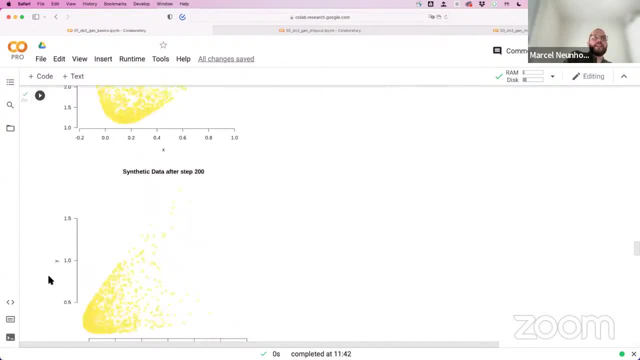 underlying distribution: aalahm secret uh. 1, 5, 8, 7, 7, 18, 9, 21, 22, 23, 28, 29, 30, 31, 32, 28, 1, 22, 43, 43, 33, 42. 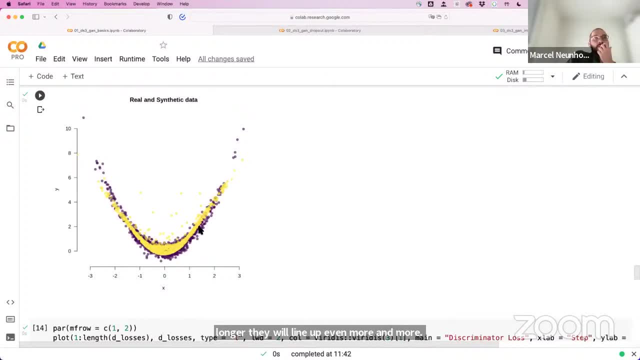 each fake point will be a pretty good representation of the underlying function, but we lack like fidelity, like diversity in those generated examples. So therefore, this dropout when using to generate synthetic examples can help to get like a more diverse, more diverse like synthetic data as well. 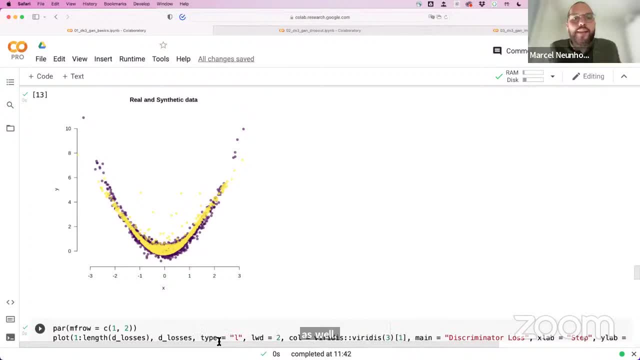 The second question, and are there any cases where noise DIMM should be different from data DIMM? Yes, like we will see those as well later. So this is just coincidence here and like to keep the initial network rather small and it is also sufficient in this problem. 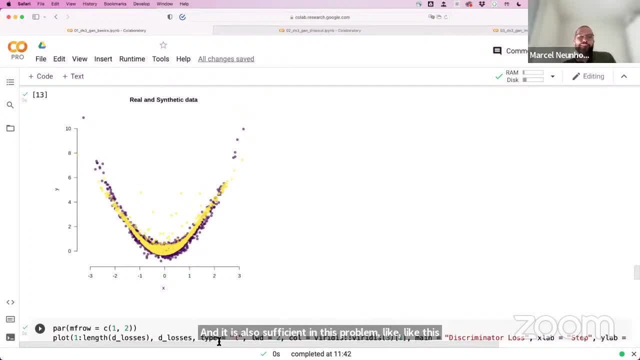 like this: the function can be represented in a two-dimensional space. So, basically, the noise dimension restricts your latent feature space, like how many dimensions your latent feature space can have, And for images, for example, like the data dimension, can be really huge, right. 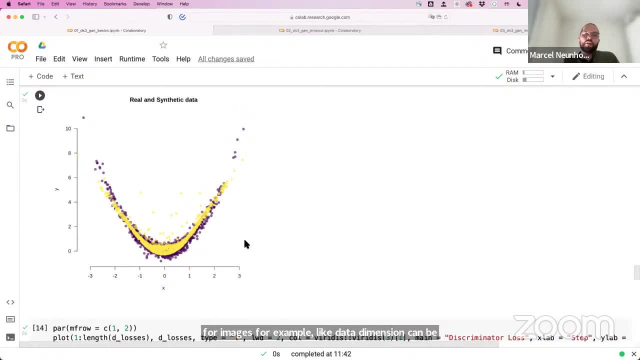 Like, if you think of like a 64 by 64, you have the data dimension right: 64 pixel image, that is, 64 by 64 features and 64 times 64. So that's a lot of features, but you would expect that, like that feature space. 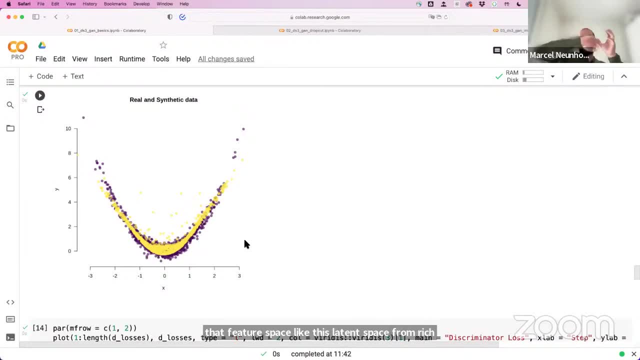 like this latent space from which we learn, like to map new images, has fewer dimensions than like this. So then the noise dimension would be typically less than the like data dimension, And if you use convolutional neural networks, the data dimension will be also will look a bit different. 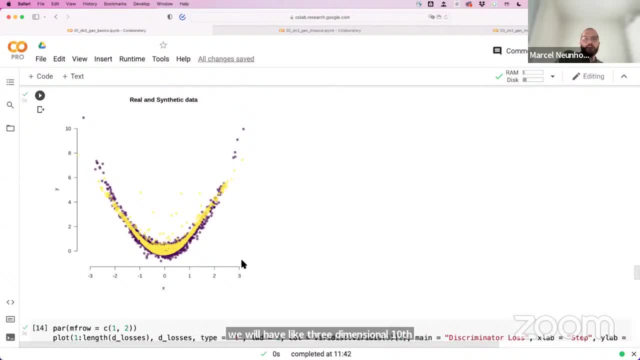 Like we will have like three-dimensional tensors as the data dimension. And then there is another question about- I will just read it again: Can we use CUDA or other parallel computing packages to speed up our Gantt training for large amounts of data? Yes, that's the beauty of Torch. 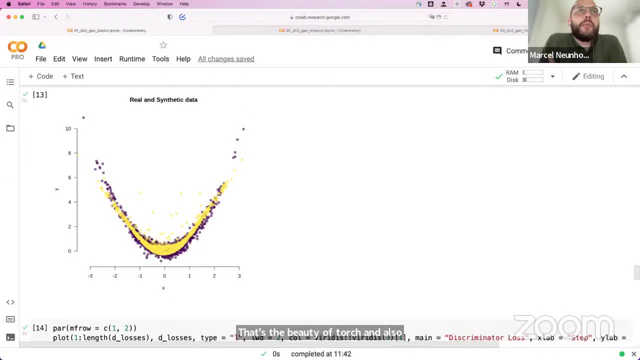 and also Keras and TensorFlow. It will work with GPU as well, And also the R package will work with the GPU if you have one. Unfortunately, and I just figured this out this morning- the Kuda speedup instance doesn't have the right version of CUDA installed. 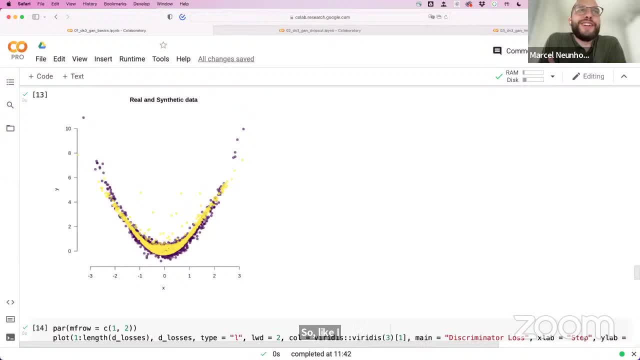 So, like I will show you the CUDA speedup on my machine later. but yes, this is definitely possible And the speedups are typically the largest if you work with like higher dimensional data, like images and, for example, deep convolutional neural maps. 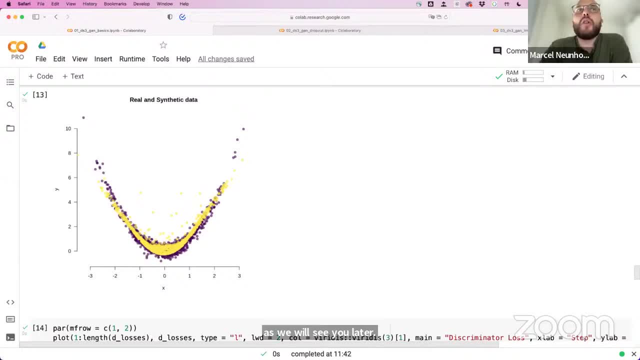 as we will see later. So training in the Colab notebook will take about four hours for one epoch, Whereas on the GPU it will be just like somewhere between 15 and 18 minutes. So that is a huge speedup and certainly possible. 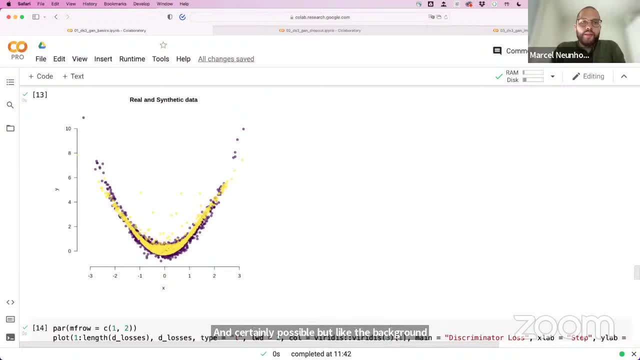 with, like the pipeline that we have here, How to increase accuracy and speed of Gantt. Accuracy is maybe the wrong, the wrong goal here, but, like if you cross out accuracy through quality of synthetic samples, I can try to answer this question. 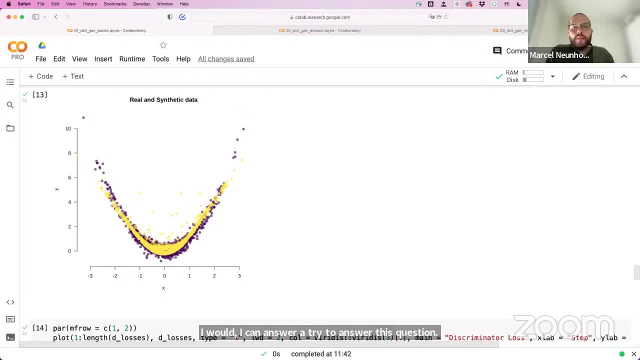 So a lot comes from like different design choices that we will look at. So there's many different ways of how to optimize your Gantt pipeline or your GPU or whatever else it is, or your GAN, and tailor it to a specific use case. 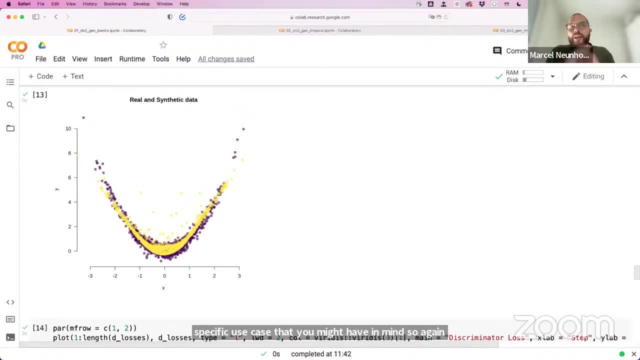 that you might have in mind. So a GAN for an image will look very different from the simple GAN that we had here. And speed, yeah, that's like hard. So that, of course, depends on the kind of networks you want to use. 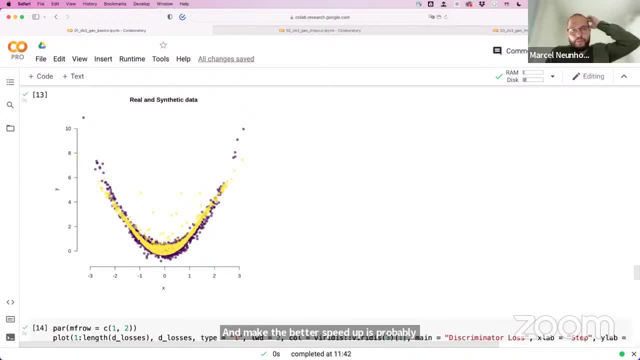 And like the biggest speed up is probably, if you work with images and deep convolutional networks, having more GPUs available. But that, of course, often crosses like with a budget constraint. And like the last question is a very interesting one- If you have a low accuracy of the data at the start, 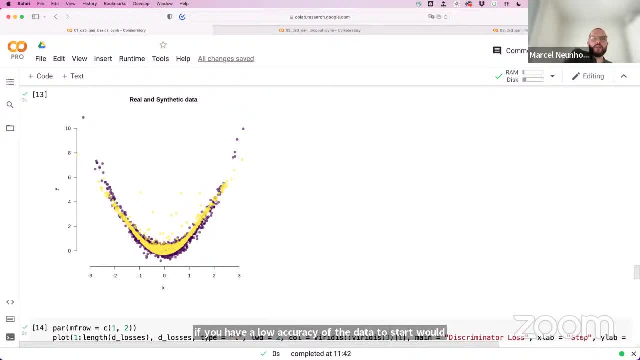 would it be possible that the GAN training slows down and doesn't run at all? Yeah, with different architectures, or like also with this architecture, you can have cases where you have vanishing gradients, Like if the discriminator, for example, is very bad, like underpowered and doesn't learn anything. 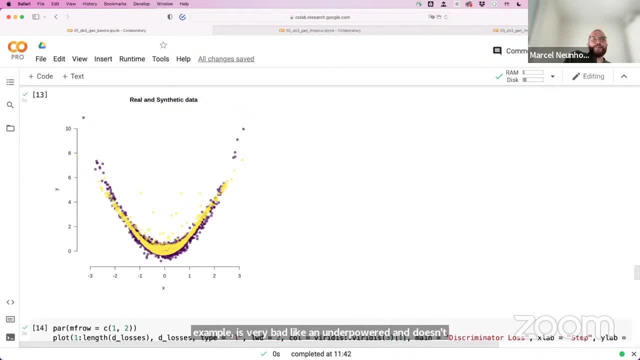 It just says anything. it sees it's 50, 50 real or fake. That would be a case where, like the whole network system couldn't learn at all. right And yeah, like that can certainly happen And like you can try to find an example in this workbook. 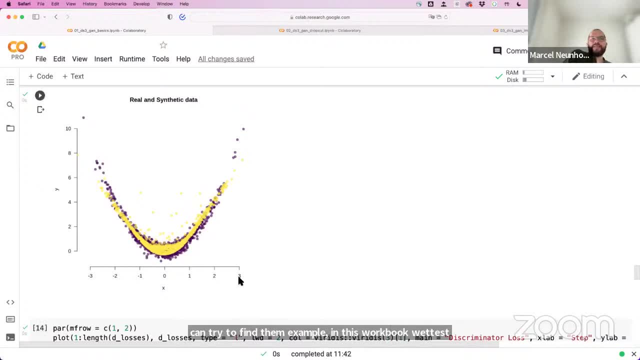 where this happens. And then I guess trying to find strategies to like identify this during training would be super helpful to not like get stuck in a long training And there at all. but in general, like the hyper-parameter and architecture, optimization of GANs is like a very 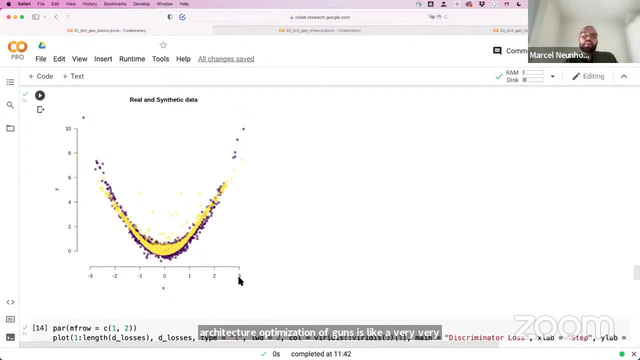 very open research field and like the current research frontier. So it's hard right, Because there's so many moving parts and it's not even clear what we optimize for. or it is clear, pliscidly: one better quality of synthetic data, but like how to define this method. 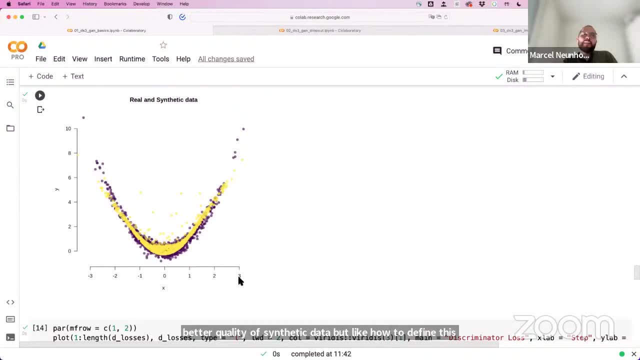 mathematical definition. it's not always easy and then trying to optimize this for speed and accuracy and like maybe also kick out bad runs early on is definitely worthwhile And like. I hope that the second part will answer some more of that and I can point you. 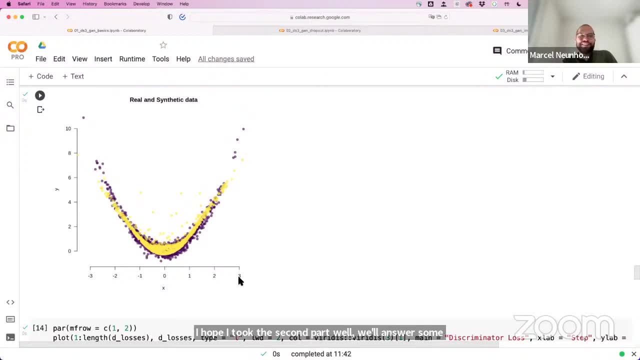 in the right direction, Ada. any more questions for now? There's one on YouTube. I'm just going to read it out loud, if that's okay. Do you have a question for Ada? Yeah, Do you know about the performance of guns? 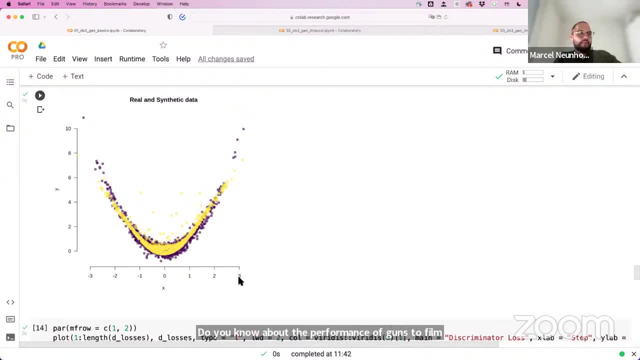 to fill missing data in multivariate time series data sets versus more common procedures like multivariate imputation by chain equations- Great open research field again. So I have looked at the context of multiple in the context of imputation: data imputation. 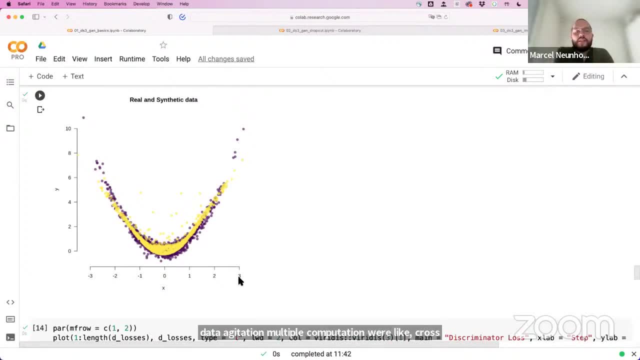 multiple imputation with like cross-sectional data, but not evaluated. It's in the case of time series data. In the case of cross-sectional data, it really depends on the underlying data structure, right? So like those, especially those change equations, 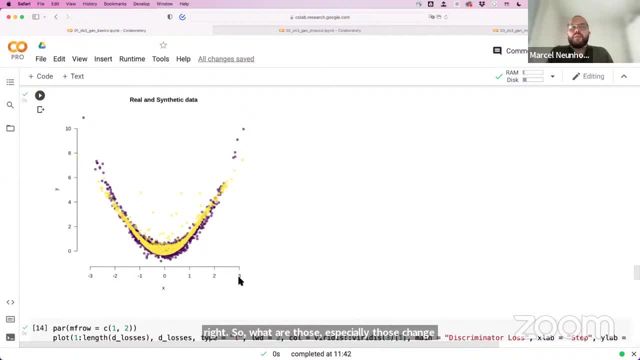 can do a pretty good job, especially in combination with like predictive mean matching- Really hard to beat but like as soon as you get like, and I would argue that this is most often the case in real data applications where you don't know exactly. 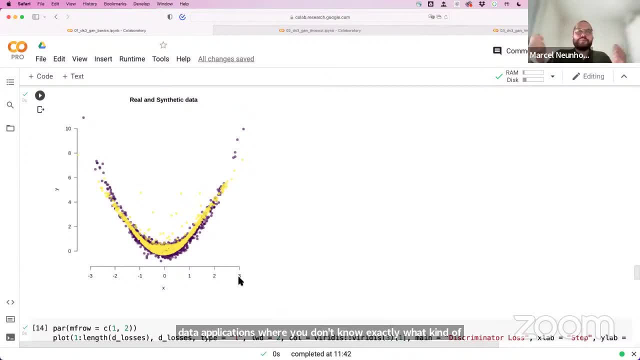 what kind of underlying link, correlations and inflation you have. guns can pick up better, like those weird cases, And I would assume that something similar is true for the time series data. However, like for time series data, like the gun architecture would need to take into account. 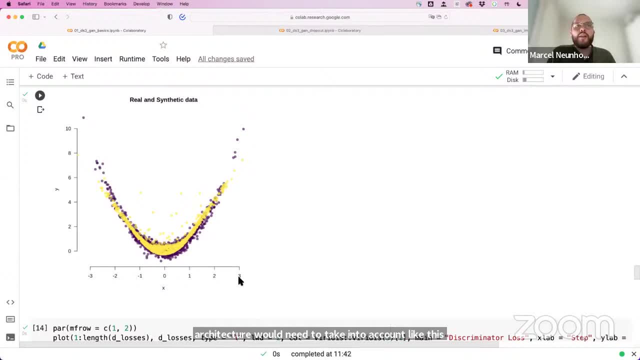 like this time series structure of the data as well. So one way to do this would, for example, be using like recurrent neural networks or also convolutional neural networks, so that you make use of the structure that you have in your data, So like the architecture that we have here. 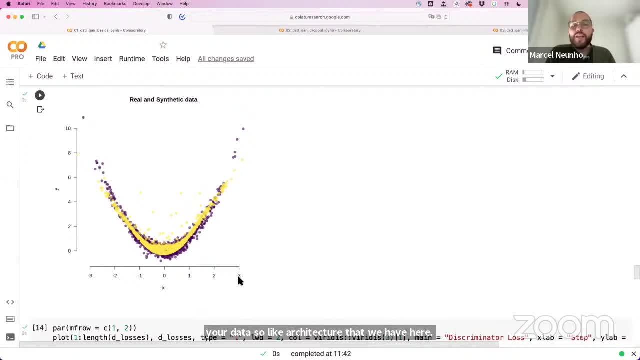 wouldn't probably be very helpful for time series data at all. And this is maybe before we break for a little bit. but one big takeaway that I think that everyone should take out of here as well is that, like generative, adversarial nuts are really more like a framework where you can have many. 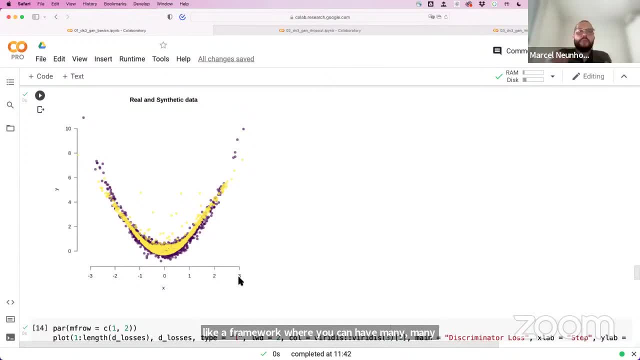 many different forms, many, many different architectures for many different problems, And it's not just like one model right. It's not like logic regression, like there is one model and then you try to you do one task with it, Like it is really a framework that is built around. 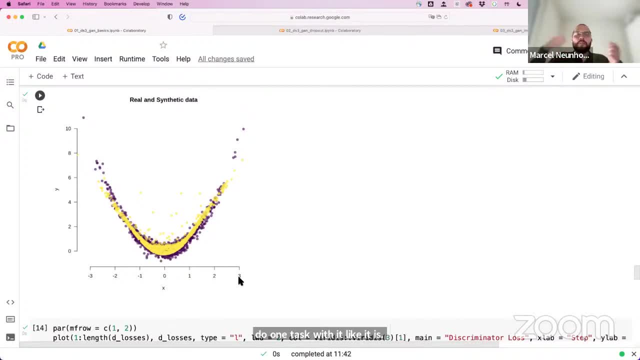 like this idea of this adversarial game And then, depending on what kind of data you want to synthesize what your exact goal is, you need to like build your own model within that framework. So there is like endless possibilities, endless combinations. 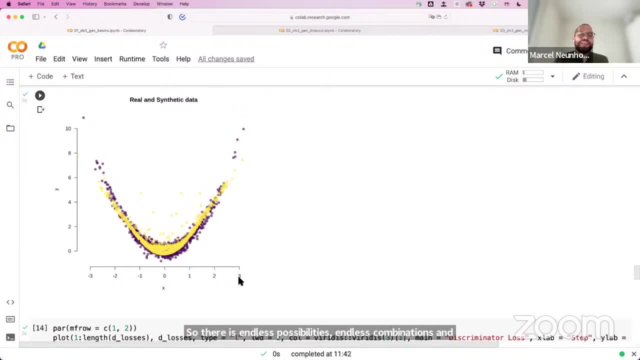 And I would assume that, like I am not saying that, this is that there is also a good way to impute time series data. but to find that model is hard, All right. but thank you for all the great questions And at this point I would close. 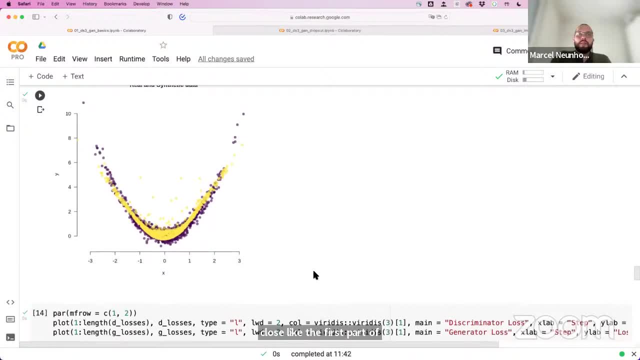 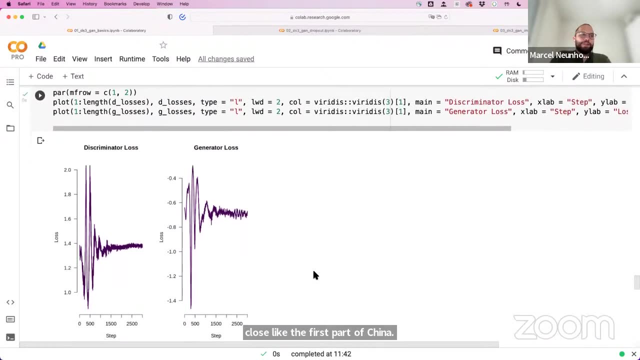 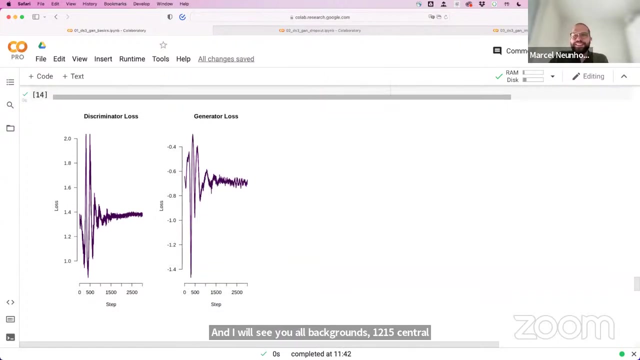 the first part of the generative adversarial net course and break for 15 minutes. I guess I need to get some water that my voice can keep going And I will see you all back at 12.15 Central European Summer Time, so in exactly 15 minutes. 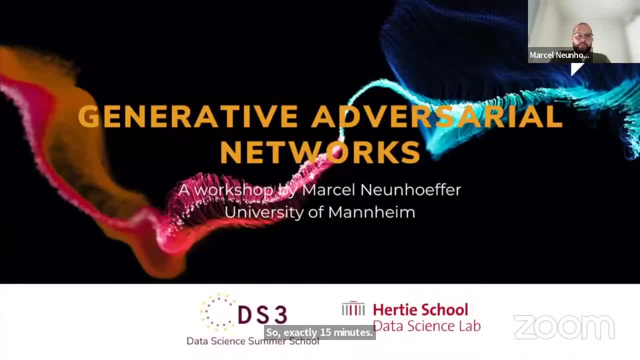 Thank you very much for watching And I will see you all back at 12.15 Central European Summer Time. And I will see you all back at 12.15 Central European Summer Time. Thank you very much for watching And I will see you all back at 12.15 Central European Summer Time. 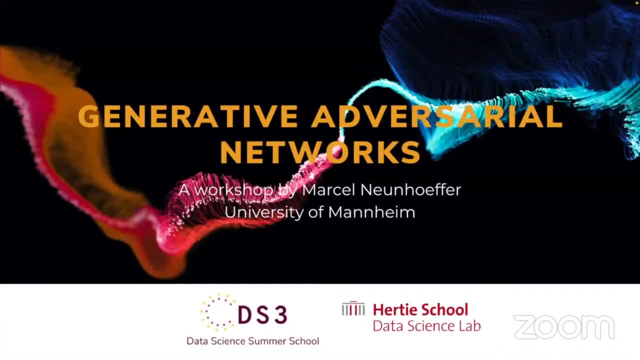 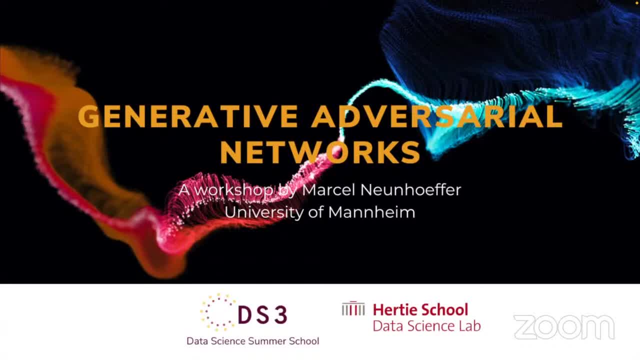 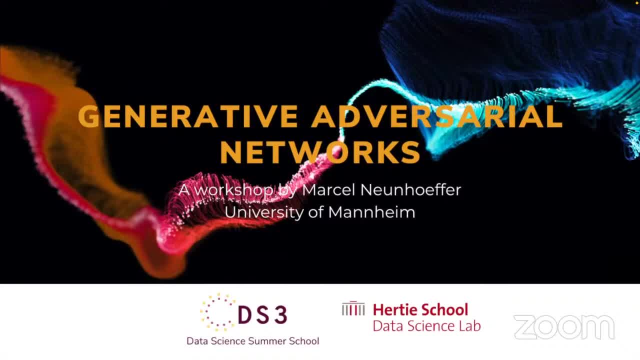 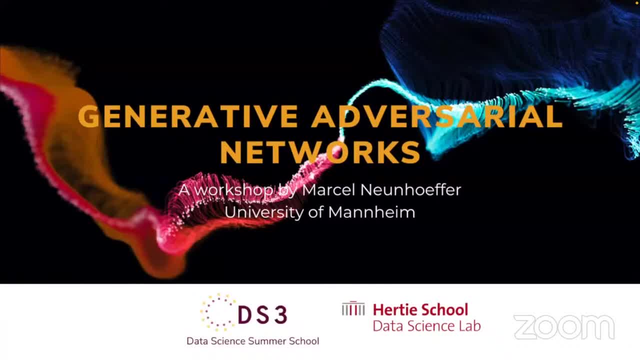 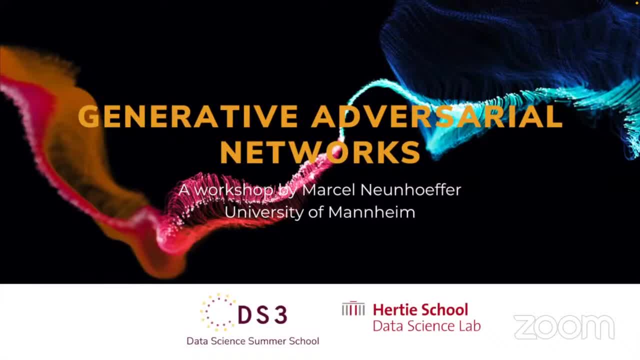 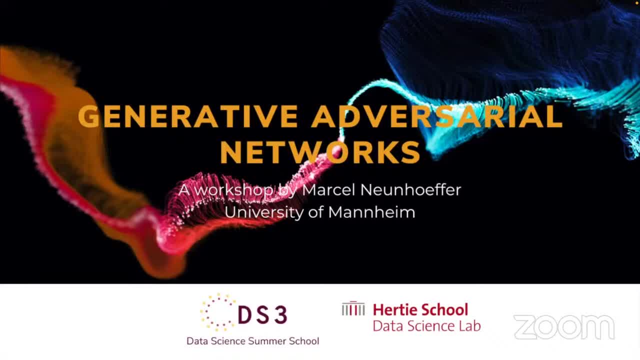 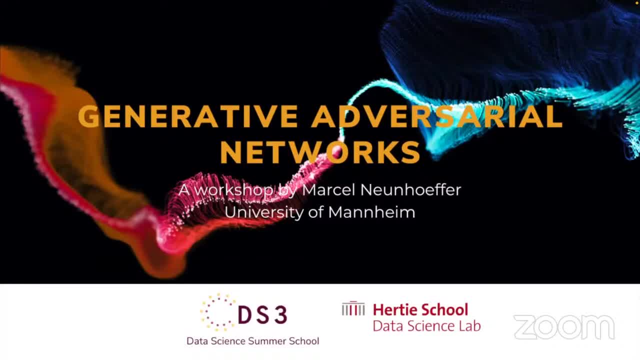 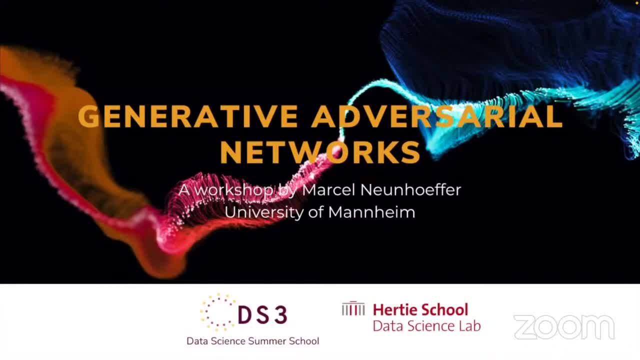 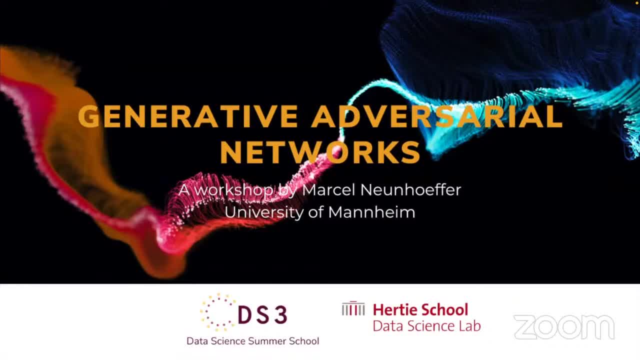 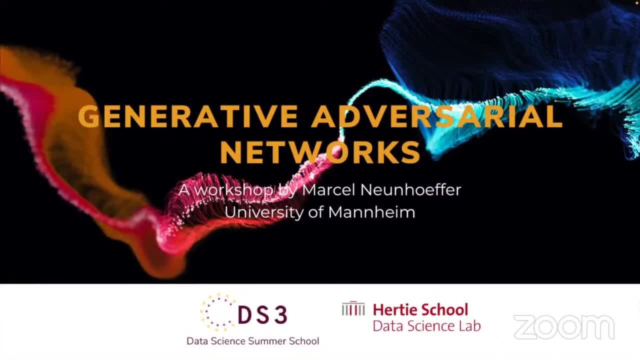 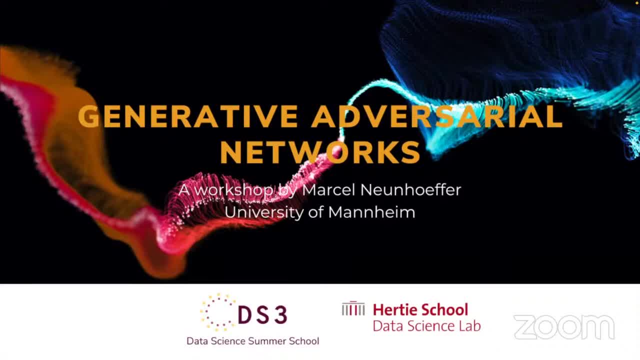 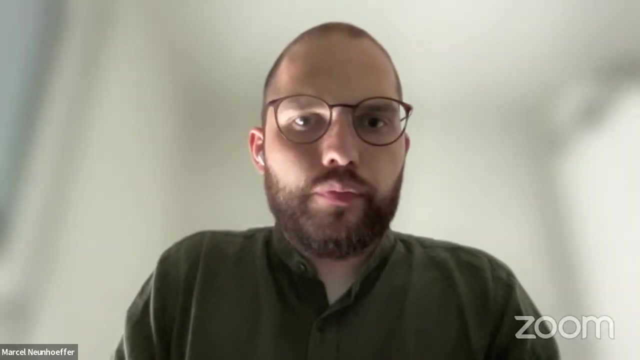 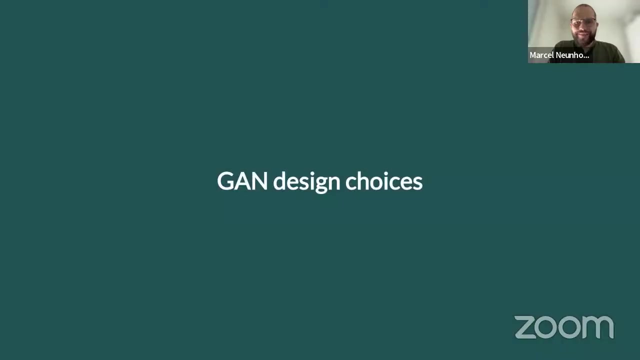 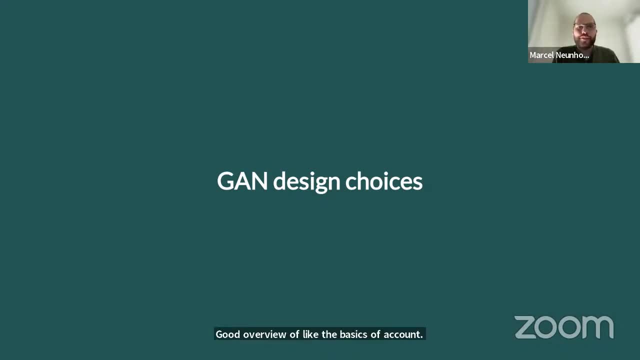 we coded one ourselves and we have seen in the code and also especially in the questions around it, that there is like a lot of things that we need to think about. right, We needed to think about, like the network, the network architecture. We needed to think. 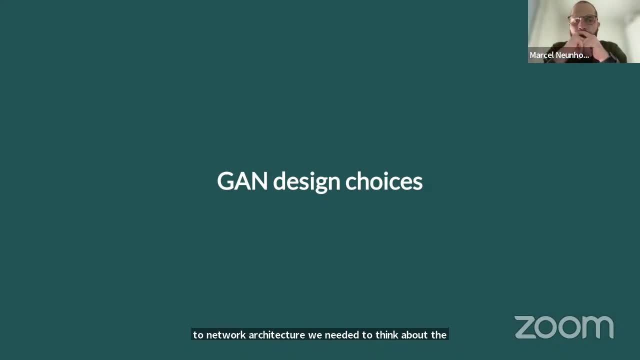 about the value function And I hinted at like that there is different other value functions that also allow us to interpret like the lost love, Like what we can see as a quality indicator. Then there is different optimizers potentially. then there is different- we had this question in the beginning- different noise. 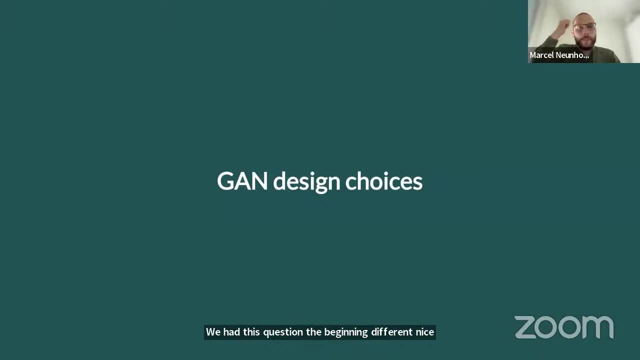 distributions that we could pass to the generator, and so on and so on. So, basically, in every step along the way, we can make different choices, and this again speaks to the fact that, like generative adversarial nets are, or how I like to think about them, is really as a framework of many, many different models that then can be. 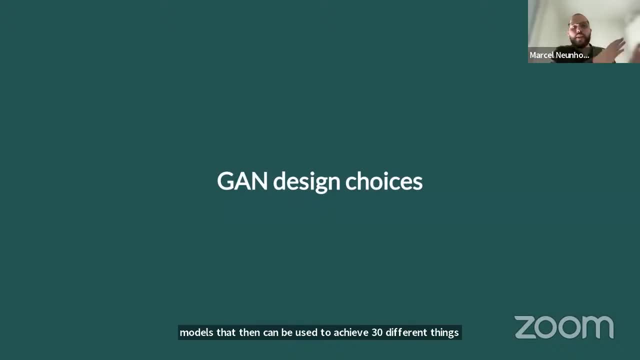 used to achieve very different things, like from synthesizing images, as we've seen, like in the introduction to synthesizing speech, those networks, those guns will look very different to synthesizing tabular data or even time series data. so let's, in this next bit, talk a bit about 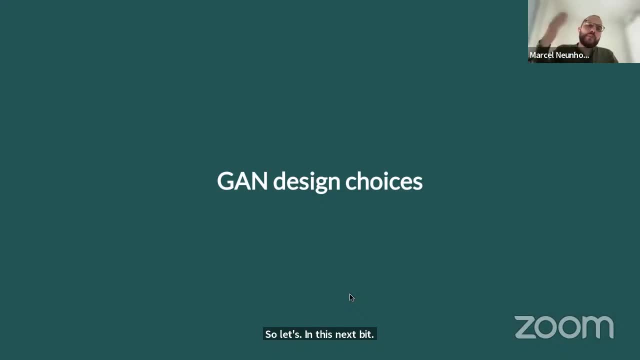 those design choices. so the next bit will be mainly about those design choices, and then we will have two little workbook exercises: one where we will look in depth on dropout in the generation of synthetic data and how this might help to generate more realistic data, and then, of course, like we try to build a gun that can. 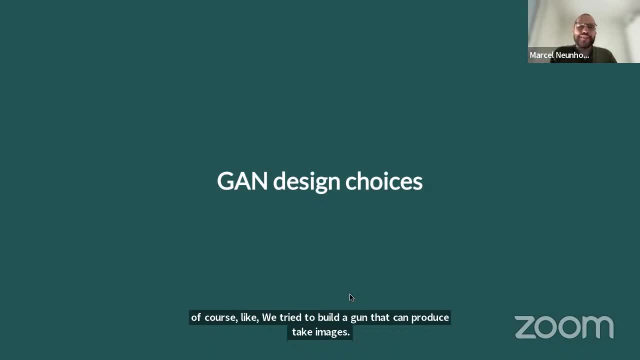 produce fake images. so I guess, or I hope at least- some of you came for synthesizing images and like this basic, simple example was really just to get a good understanding around, like what's actually going on. all right, so in those design choices, let's start like with the one that I also started. 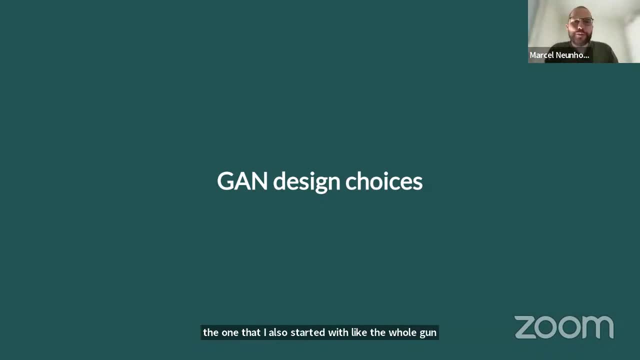 with like or the whole gun framework is basically built around on this idea of this adversarial game and just this value function of trying to, and just to, discriminate, or trying to predict what's real and what's fake, and then the generator trying to maximize this and the discriminator trying to minimize this. there is 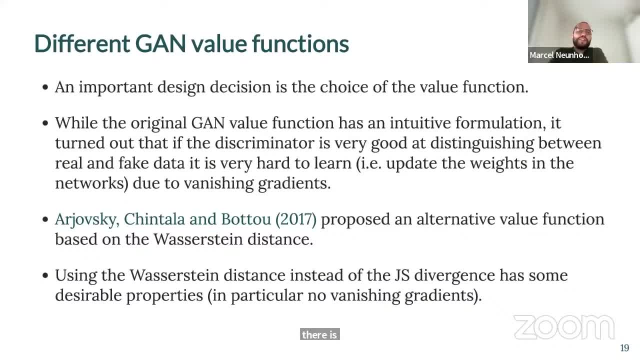 and, yeah, this is probably the most of one of the more important choices in in a gun and I really like the original gun value function where you can actually see this kind of function, especially to introduce new people like you, to generate a first area, and that's because it has like this intuitive 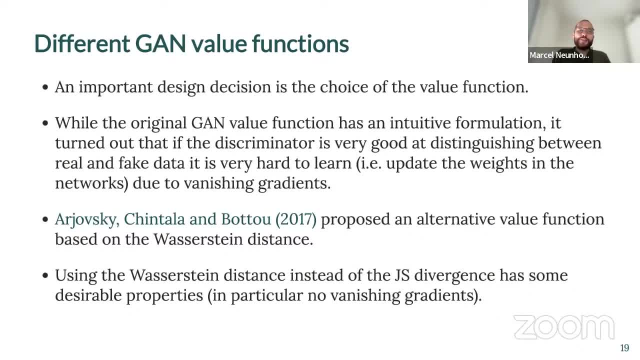 formulation of like this, trying to predict what's real and what's fake. however, it turns out that, like if the discriminator is very good at in real fake data, it is really hard to learn, And also if it's like too weak, but like if it's really really good at distinguishing. 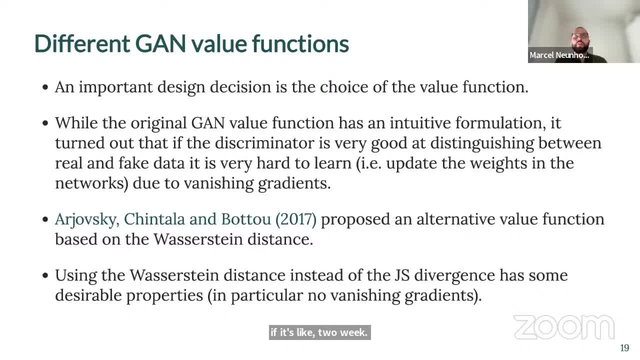 between real and fake, we will get something that is known as vanishing gradients in machine learning and neural networks, Like, if you think of, like the sigmoid curve and if you get like predictions that are very close to zero and very close to one, the slope of the 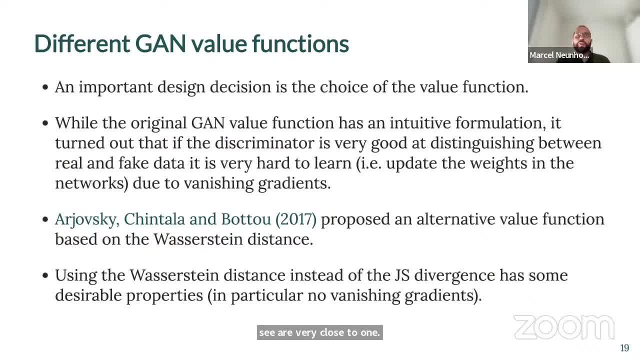 the loss function at those points is very, very close to zero. So that means that like, if we back, propagate like the loss or like the gradient of the loss. this means that like, as the gradient is the slope of that function at this point would mean: 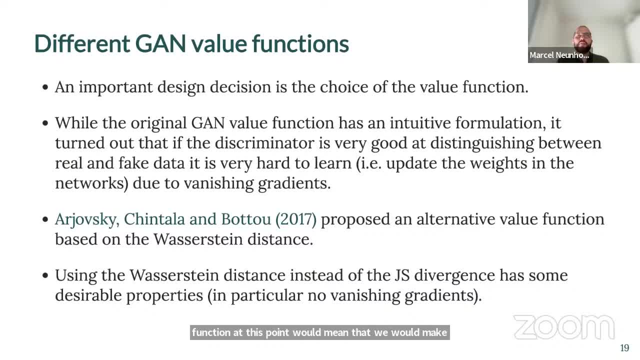 that we would make tiny, tiny, tiny, tiny update steps, if any at all. And this means that, like, if we have, like, a discriminator that is very, very good at predicting zeros and ones like what's fake and what's real, 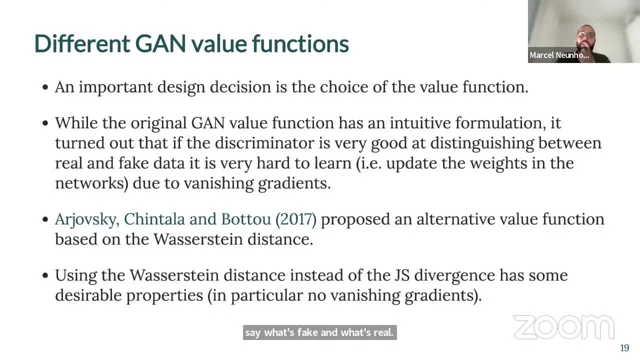 then we can get stuck there and generally that just doesn't learn anything useful anymore, And this is, of course, not what we like, because this doesn't get us any closer to the equilibrium that we like to find. So therefore, like for you, I think it's really, really, really important. 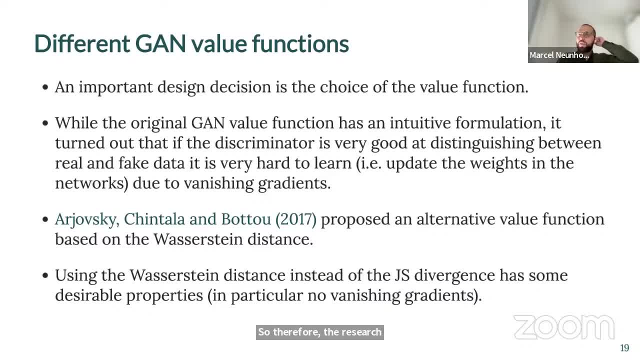 The researchers proposed a new value function a couple of years after the original GAN and it's also a very influential paper in the GAN literature And like it's linked- like all the papers are linked- directly in the presentation, So if you want to have a look at it, 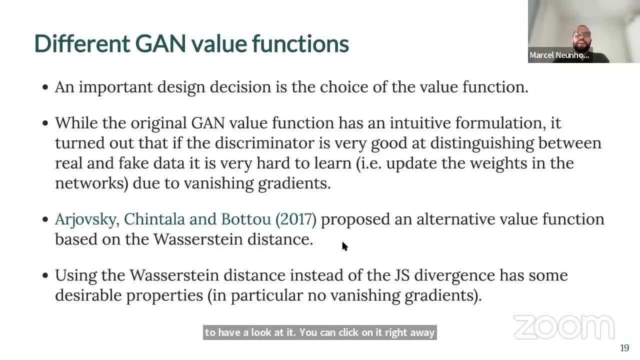 you can click on it and you'll find the paper right away. Propose an alternative value function based on the Wasserstein distance- or maybe some of you have heard from- like the Earth-Hoover's distance, which is a measure of how far apart. 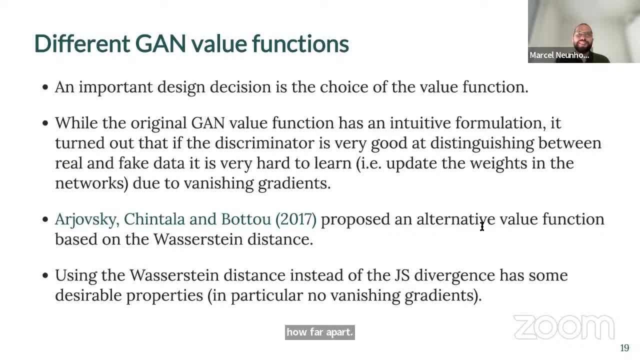 like two probability distributions are basically, And the intuitive idea there is: like how much Earth do you have to move from? like oh, oh, oh, oh. How much Earth do you have to move from? like oh, oh, oh. How much Earth do you have to move from? like oh, oh, oh. 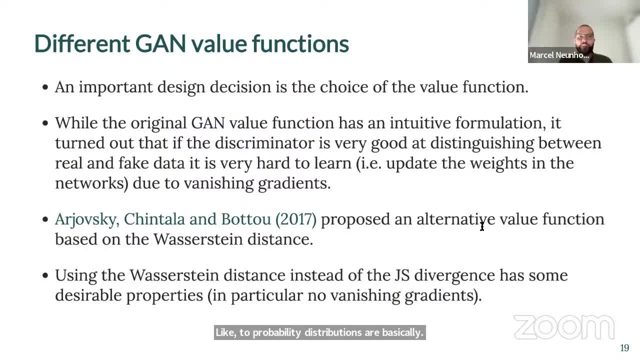 How much Earth do you have to move from like oh, oh, oh? If you think of those distributions as piles of dirt, how much dirt do you have to move to get from, like, the first to the second distribution? And this turns out like swapping out, like the JS divergence. 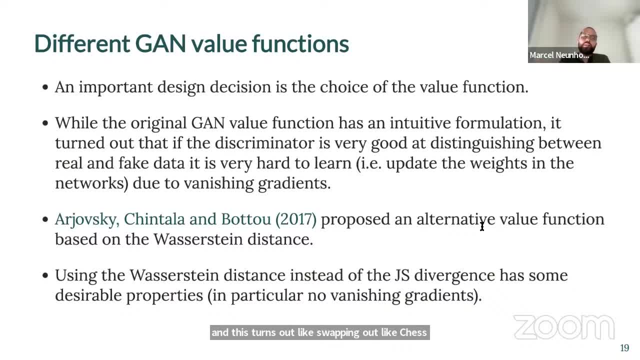 which is like if you reformulate the original GAN function, you can see that it's basically using the JS and some Shannon divergence between two probability distributions, like using the Wasserstein distance there instead of the JS. divergence has some very desirable properties And in particular, the first one is that it has 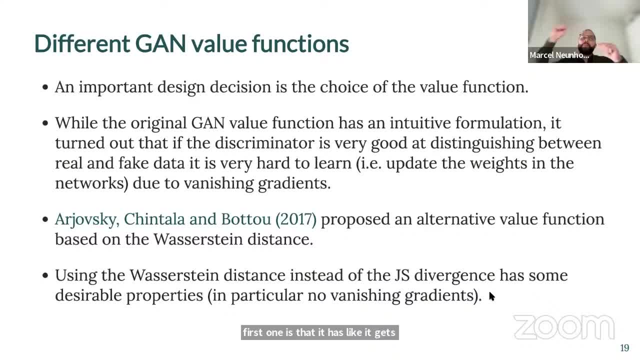 like it gets rid of this vanishing gradient problem because we don't need the sigmoid function anymore. We can just use the linear output layer in the discriminator, And therefore this leads to better results or more consistent results as well. And another nice feature is that, like 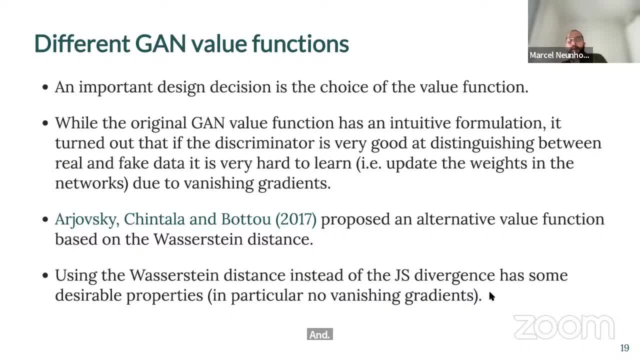 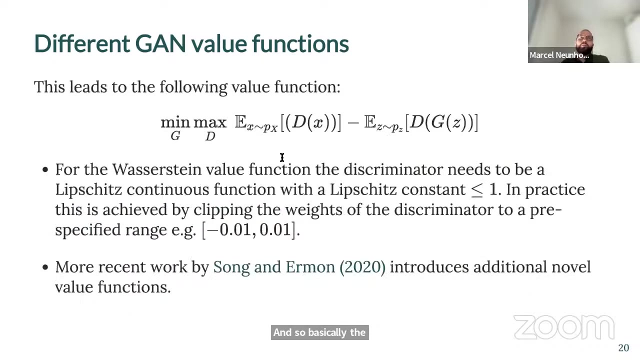 we can interpret this Wasserstein distance between those fake and real scores as like it is correlated with quality of the produced, And so we can see that it's a very good way to interpret the value of the data as well, And so, basically, this leads to the following value function: 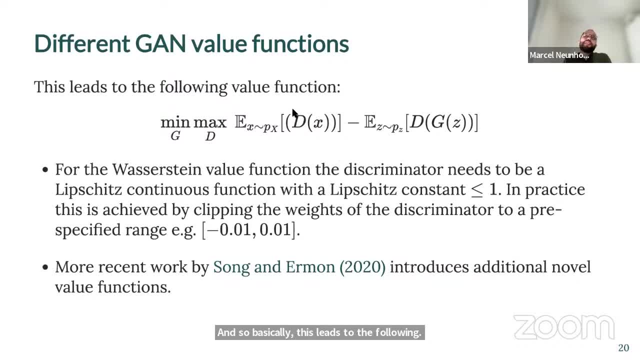 It's a lot simpler, even than the original one. So remember, before we had the expectation of the log of the discriminator scores plus the expectation of the log of one minus the discriminator scores on generated samples, And now this reduces, like if you use the Wasserstein distance here. 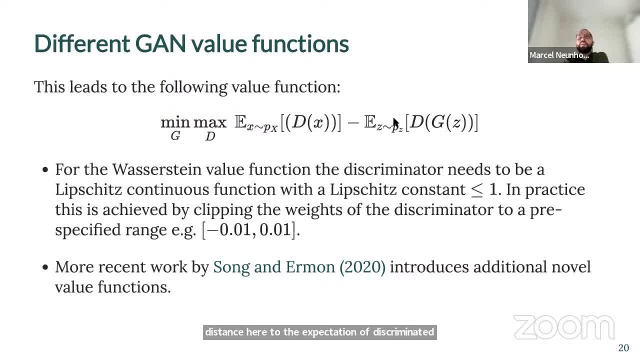 to the expectation of discriminator scores on real data, minus expectation of discriminator scores on fake examples. However, this comes with like one as we work on the real value discriminator output now, like this comes with that downside, namely that the discriminator needs to be. 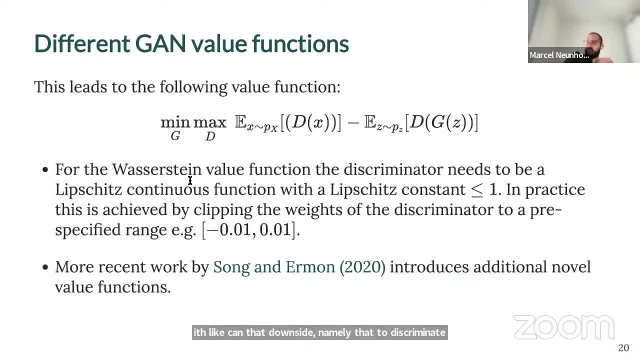 a Lipschitz continuous function with a Lipschitz constant smaller or equal to one. This is needed that this value function can converge to an equilibrium, And we don't like we basically constrained the space in which we look for an equilibrium. In practice, this is, or this can be achieved: 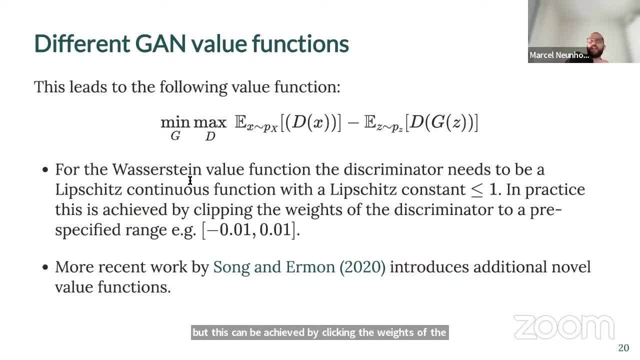 by clipping the weights of the discriminator to some pre-specified range, for example minus 0.01 to 0.01, and making sure that all the weights after updates are in this range. So this will constrain this, to like such a space. 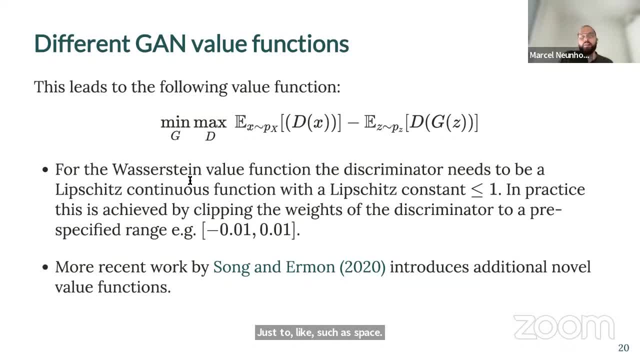 Other alternatives are: you could can also use like a gradient penalty on the Wasserstein value function, on the Wasserstein value function, on the Wasserstein value function. that also ensures automatically that this property is material, that this value function, that this Lipschitz continues. 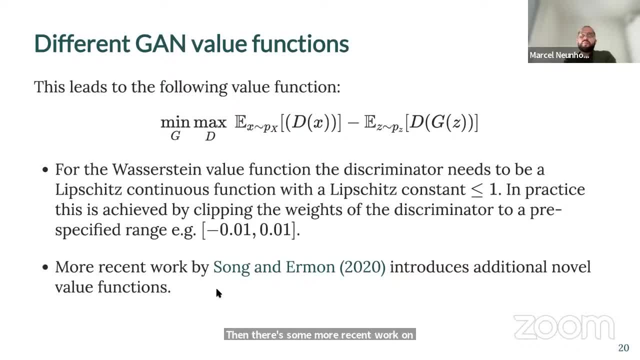 Then there is some more recent work on value functions that try to bridge- or we try to use other different differences as well: KL divergences or in general, F divergences and bridge guns in this whole space of potential divergences between those probability distributions. 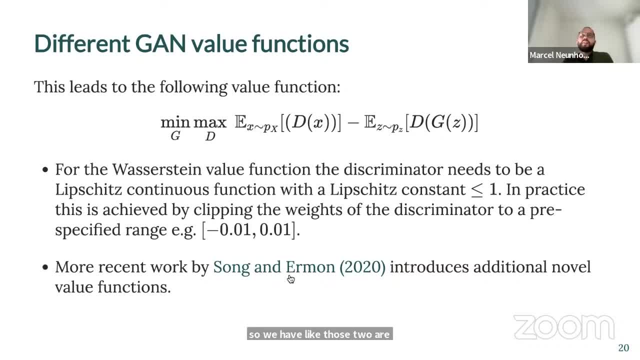 that we have, like those two probability distributions And this seems to be particular promising paper that comes up with a new value function that also gives more stability in training And also gives you a loss or the values of the losses that are correlated with quality of data acceptance. 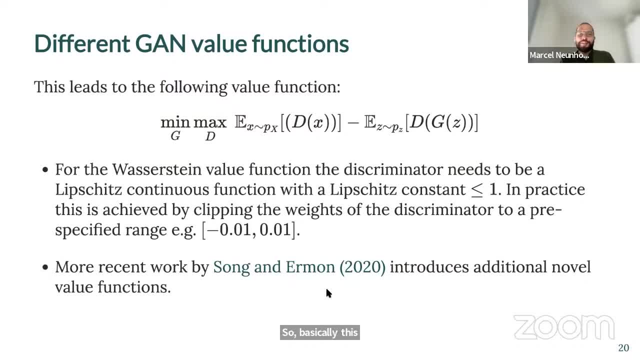 So basically this is directly addressing some of the questions we had earlier. So there is ways to like, improve on this. original gun functions And you know, I think it's really interesting and this work so far basically came from addressing weaknesses on the computation math side. 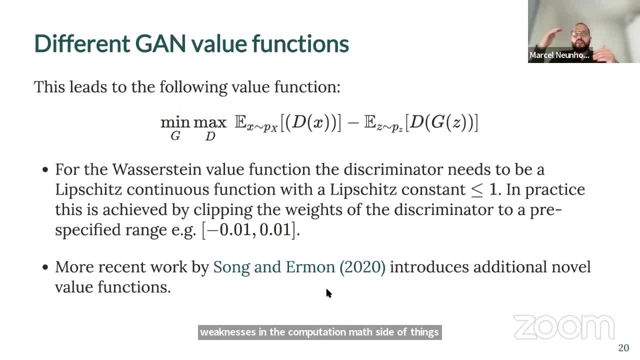 of the original gun value function, like the vanishing gradient problem. However, like what I think might be a promising research avenue, that, like if you're interested in finding better value functions, is exactly what was suggested in one of the questions before as well. 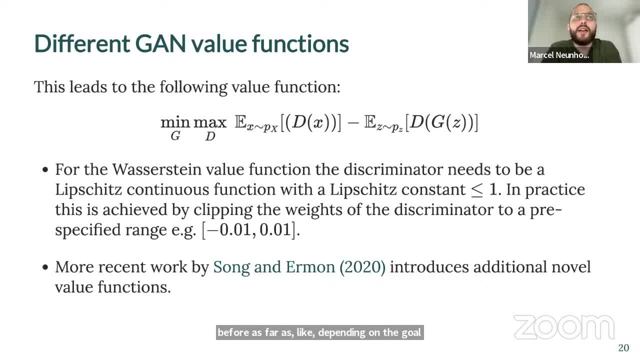 like, depending on the goal you have with your gun. for example, if you want to generate synthetic data- that's particularly good for some regression model- you can use that information to inform your value function, right Like you can tailor your value function. 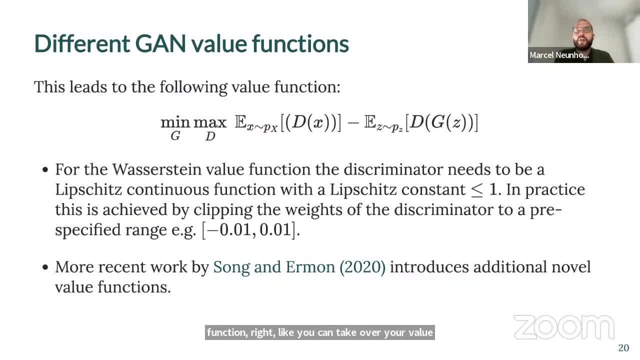 to the problem that you want to solve. So I think informing those value functions with like background knowledge in, for example, the social sciences or data science, like maybe even theoretically grounded in what kind of properties you want to achieve for your synthetic data, is, I think 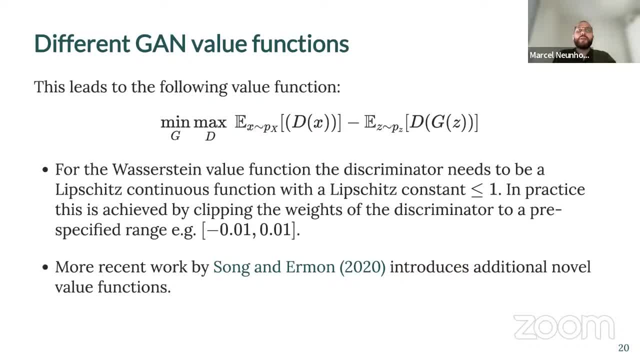 like a very promising direction of where, like gun research would like apply Like research, like subfields could merge. So that's the first thing And like, as I've said, like we don't need like this sigmoid activation function in the output layer of the discriminator anymore. 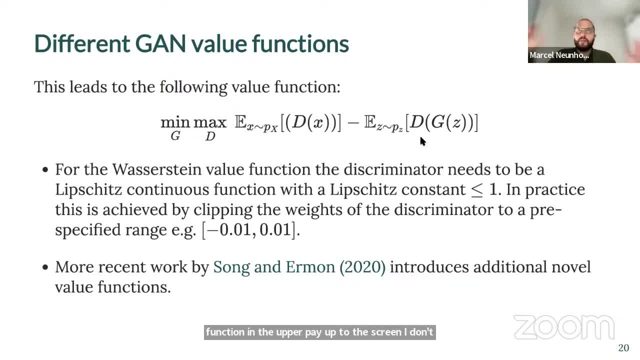 in this case we can just use the linear output layer, So putting various on the real line in those scans, like if you read up on those papers that use, like the Wasserstein value function. the discriminator is often called a critique instead of a discriminator or critic. 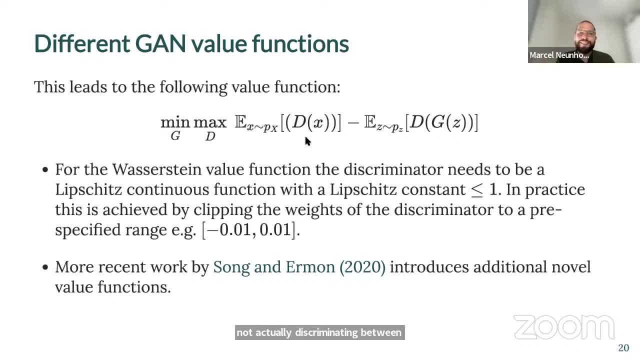 as it's not actually discriminating between real and fake examples anymore. It's trying to criticize them, like on a continuous scale, and trying to find, like the like, a way to like those two distributions match. So that's the first choice you typically can make. 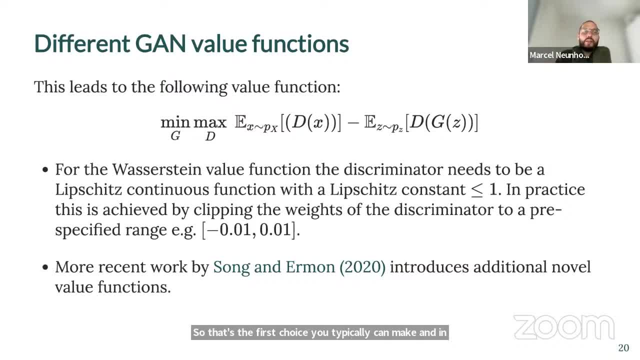 And in the Argonne package you can choose, like the original value function, the Wasserstein value function and also this KL divergence based value function by Song and Ehrman pretty easily, And this makes it then easy to try to see what those choices. 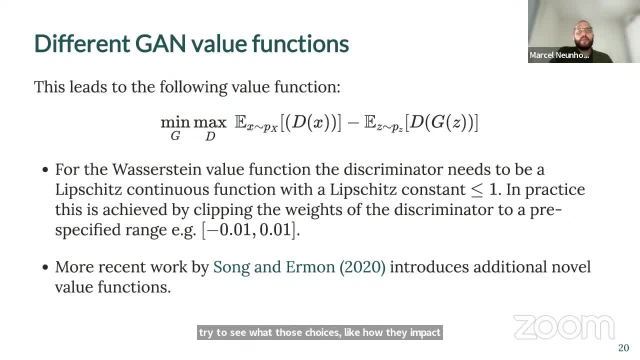 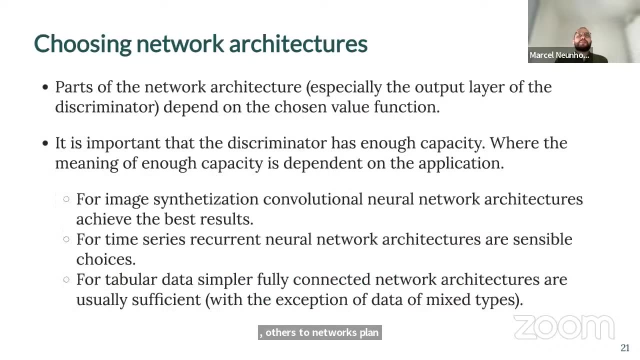 like how they impact your synthetic data. So that's the first important choice you need to make: like what kind of value function, like what kind of game are those two networks playing? Then the second important choice- and we have also implicitly made that in the first: 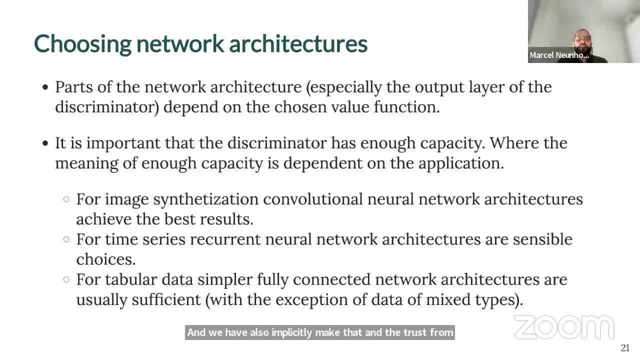 from scratch. example is choosing a suitable network architecture for both the generator and the discriminator. slash critique And parts of that network architecture, in particular of the output layer of the discriminator, depend on the chosen value function. So if we want to work with the original GAN value function, 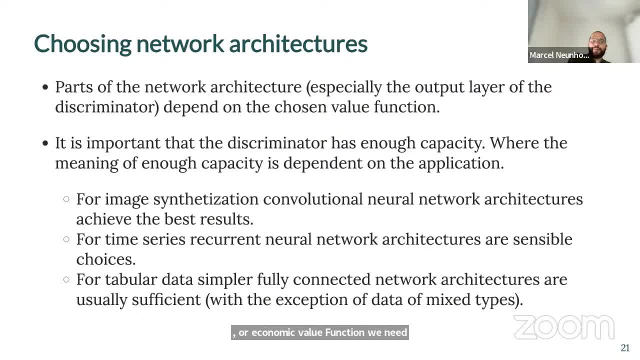 we need to have like some transformation to like those probabilities in the output layer, Whereas in the Wasserstein GAN, like if you choose the Wasserstein value function, you can have like a linear output layer. So this influences already like your network architecture. 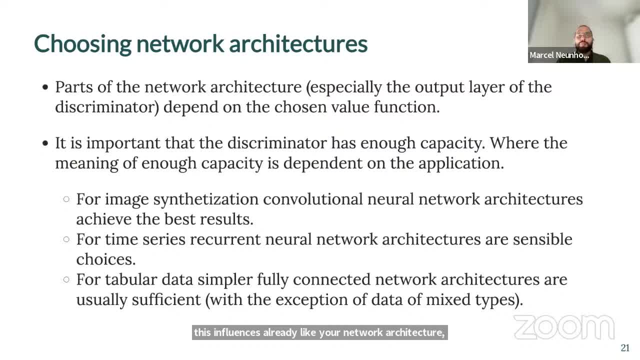 However, there's like more choices than just like the output layer right. Like we talked about width and depth, and then also about potential different architectures of those hidden layers. In general, it is important that the discriminator or critic has enough capacity for whatever problem you want to solve. 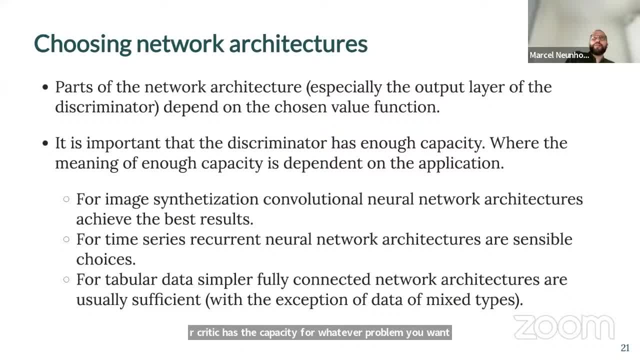 and where the meaning of enough capacity is heavily dependent on the application that you want to solve. So in practice, for example for image synthesization, convolutional neural networks achieved the best results, which is pretty much in line with like what we know from computer vision. 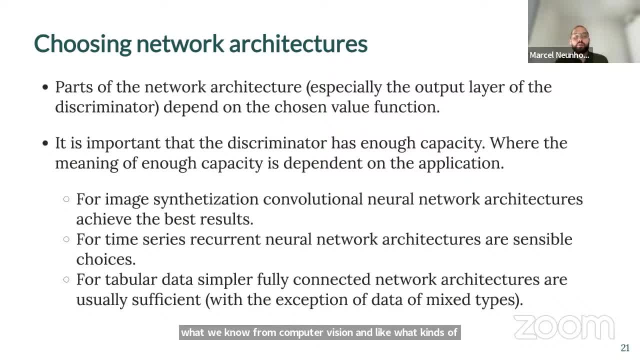 and like what kinds of network architectures work well also to do, like object recognition and images, for example. So like, if you want to work with images, you would probably need to look into convolutional neural network architectures. And like, if you follow that link of like this person does not existcom. 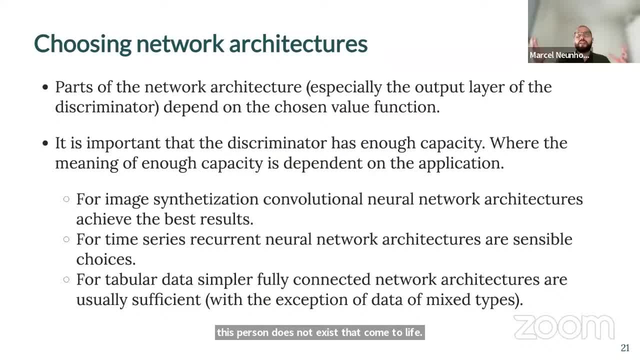 to like the original StyleGAN 2 implementation, you will see that this is a huge convolutional network with like skip connections and residual connections and like just a huge, huge network of like convolutional network. if you and we had this problem with like 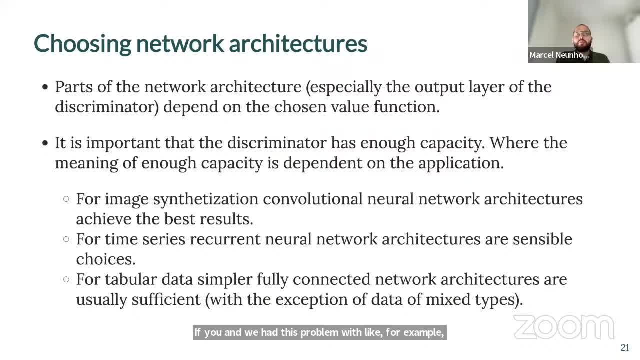 for example, imputing time series or like, if you don't even want to impute but generate synthetic time series, recurrent neural network architecture are sensible choices and if you remember, like the speech synthesization problem or example in the intro, like speech or text can also be thought of. 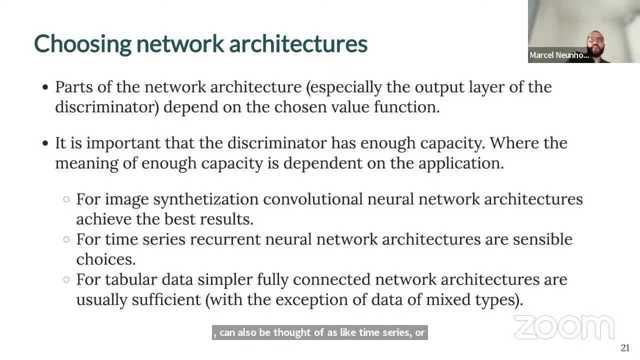 as like time series or videos as well. so for those kinds of problems, like those recurrent neural network architectures are typical sensible choices where you make use of like the time structure, like the structure in the data that you have at hand and for simple cross-sectional tabular data. 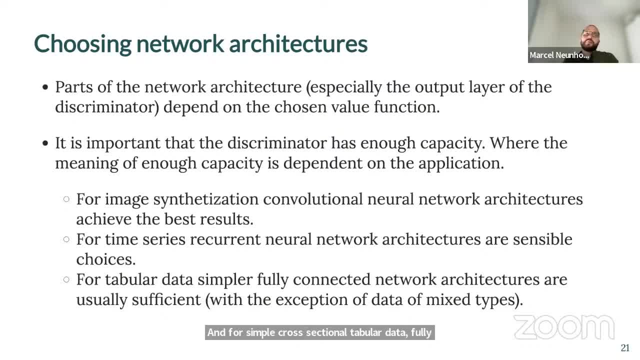 fully connected network architectures are usually sufficient, with the exception of data of mixed types, so like if, for example, you have like- and I notice as a political scientist this is a very typical data format that you have really valued and put like categories, like categorical variables, ordered variables, 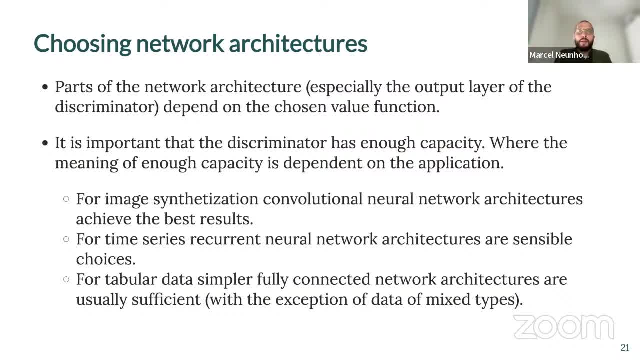 so like really data of mixed, mixed type there, like the output layer of the generator has to account for this kind of mixed data, so and also like how you encode this data. so for categorical values, usually like one hot encoded data, um vector, uh makes make sense and then like to to learn. 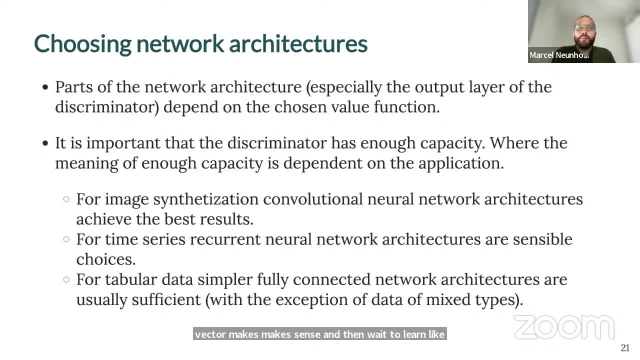 like one hot encodings. um, it takes a bit more effort, like if someone wants to read up on that. like the um gumball softmax trick is what is very useful there. so the network architecture has a huge influence on like what you can learn and depends a lot on the application that you have in mind. 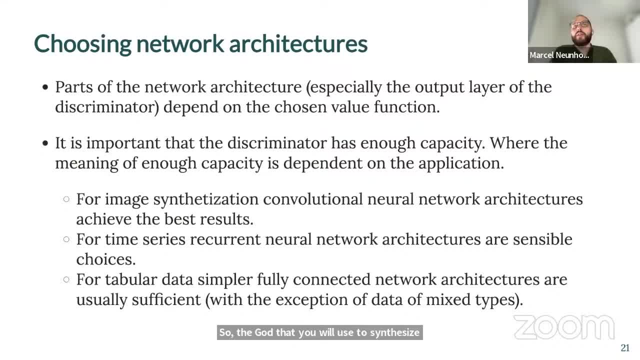 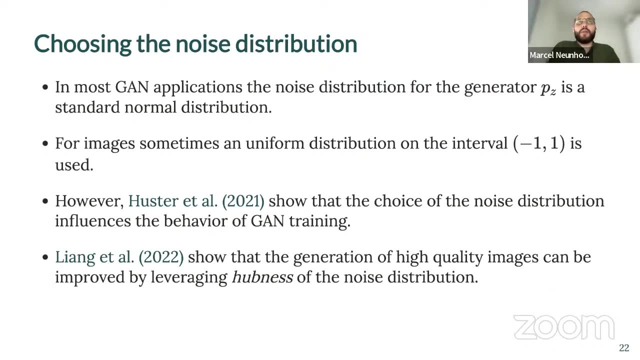 So the GAN that you will use to synthesize images will look very different to the GAN that you could use to create a synthetic data set from some data that you collect, Then like a more- yeah, recent area of research is like choosing the right noise distribution. 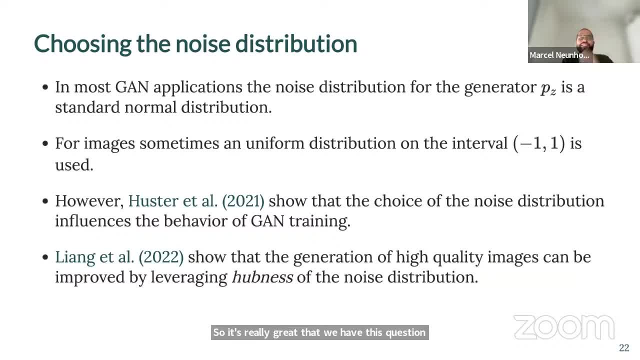 So it's very great that we had this question right in the beginning. So in most GAN applications the noise distribution for the generator is just the standard normal distribution, And this of course also has practical reasons since, like in most of those neural network APIs, 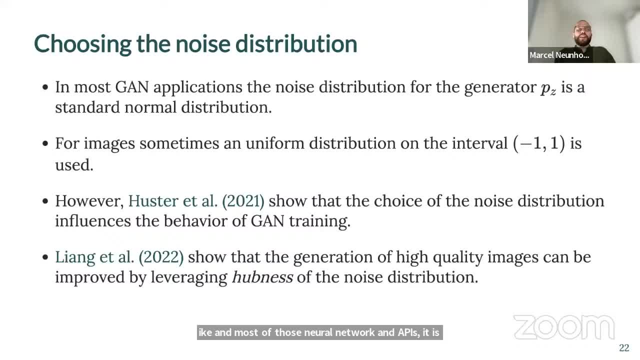 it is easy to sample from independent standard normals For images. as I said, sometimes uniform distribution on the interval of minus one to one is used, especially if you normalize your pixel values, also to lie in that minus one, one interval, so that you then can have like this, nice gray. 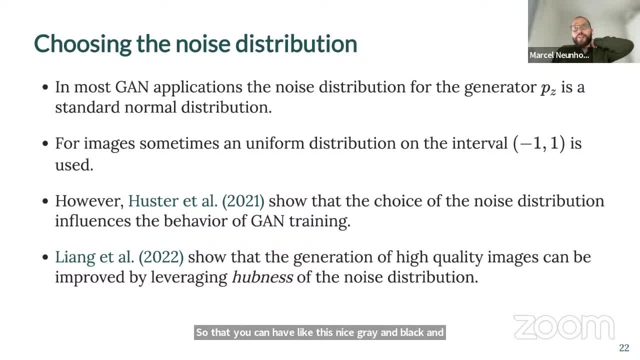 and black and white noise image, basically as an input as well. However, there is recent research that shows that the choice of the noise distribution heavily influences the behavior of GAN. training And in particular, this Huster et al paper is very interesting for social scientists. 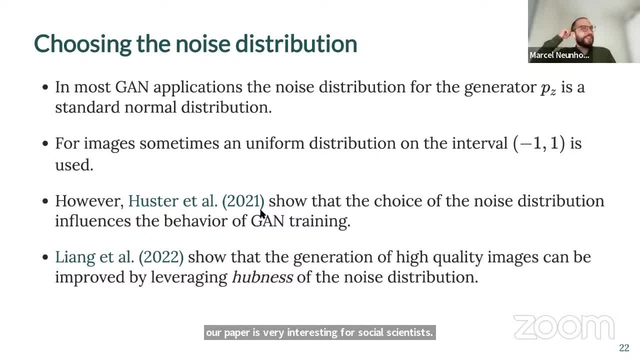 and I guess data scientists of any like flavor. They show that like it is very hard for GANs with like a standard normal noise distribution to learn heavily skewed data And as social, as a social scientist like I, come across skewed data quite often just think of like income. 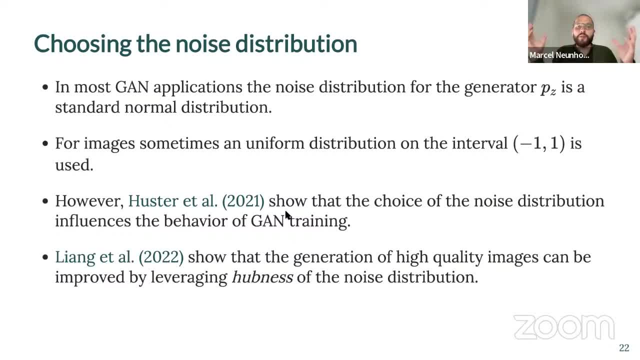 for example, or also firm sizes, like more like an economy, or also, yeah, like in elections, the number of one seats is very skewed towards, like bigger parties that traditionally did. well. So if we would, if we would want to synthesize skewed data like that, 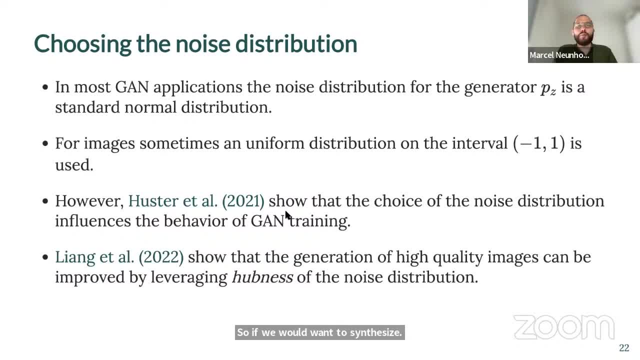 they showed that this is really really hard with a standard normal because it has like those flat tails and therefore it is very unlikely to sample like outliers in the latent space. and for skewed distributions, especially if it's like a lock, normal distribution we need like heavy outliers. 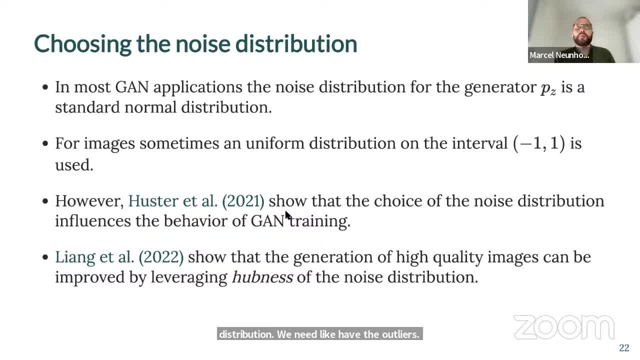 So it's. it's a very hard decision to make to learn the distribution well. So they showed that using a Pareto distribution instead of the standard normal helps with that. so that's the distribution that has fatter tails And I guess a lot of like work and classical statistics. 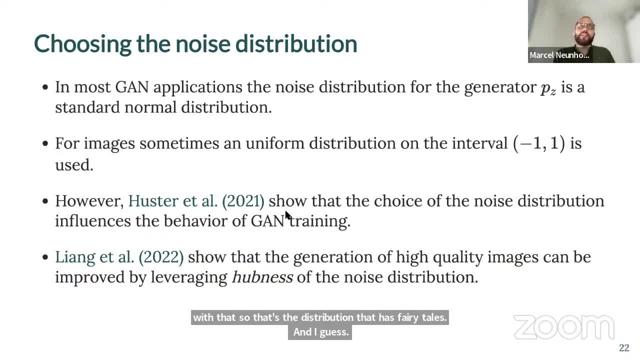 could influence those choices of the noise distribution as well, like thinking about like what distribution transforms well into, like the target distribution that we have in mind might be very helpful there. and then a very recent paper by young et al shows that in the context of image or high quality image generation, um, that like this can be improved by 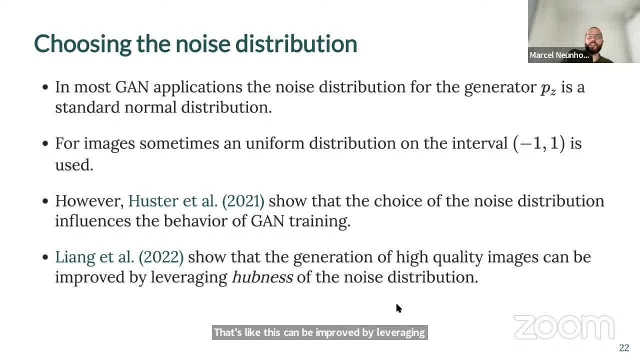 leveraging happiness of the noise distribution. so what does this mean? it means that, like in your standard normal ball, like if it's or like some higher dimensional object, not every point in this sphere, or like if we have, like a two-dimensional space, not every point, in that um pixelated noise image is as likely, uh, to produce a high quality image as as any other. 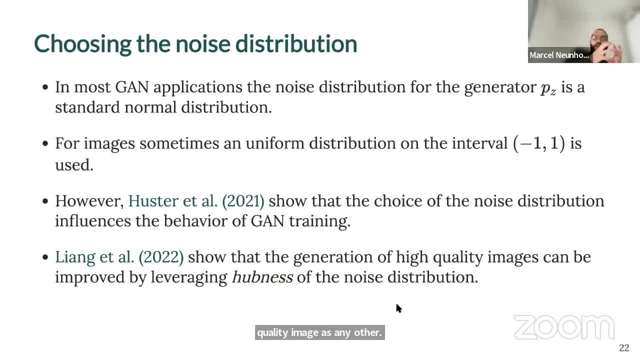 um, so, and they show that, like there is a good, um quality noise priors and that like, uh, neighbors of those hubs and you can identify those hubs- uh, like it's basically thinking of like this noise sphere as as a network, and neighbors of those hubs also have a higher likelihood of producing a high quality image. um, whereas, um just, 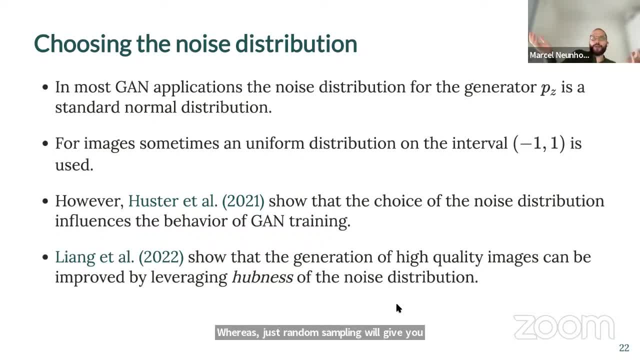 random sampling will give you like, high quality noise and low quality noise, basically. So, identifying those hubs and the neighbors of those hubs generate a higher quality images, which is a nice result, And they provide an algorithm of how to identify those hubs, So like and that like. as you can see, 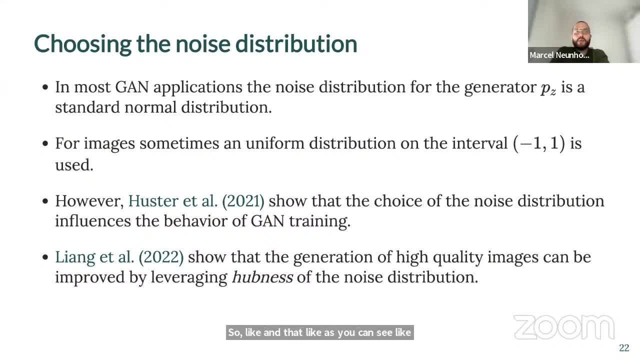 like those papers are very recent. So this is pretty much like ongoing research and it's like not trivial to give like good advice for what the best noise distribution is, for example. So it's really dependent on the application that you have in mind. 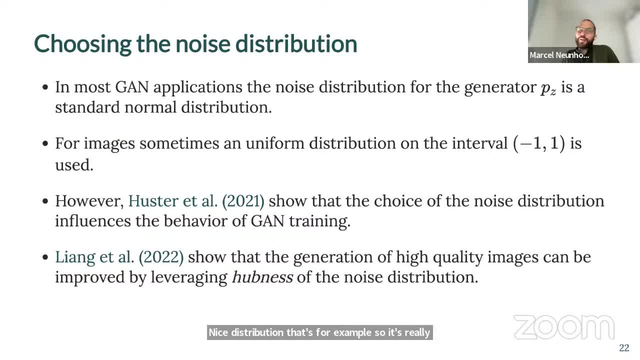 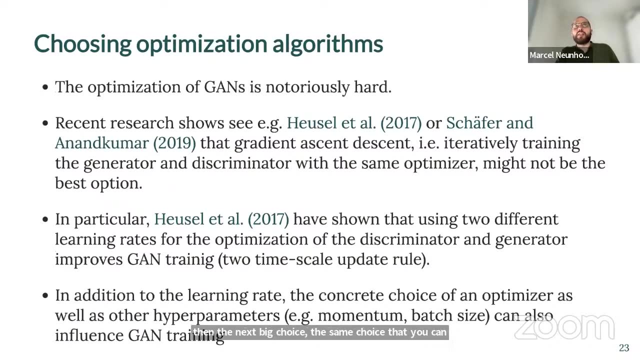 And then again like a lot of trial and error, like what works And what doesn't. Then the next big choice, the side choice that you can make in a GAN, is choosing an optimization algorithm or choosing de-optimization algorithms. 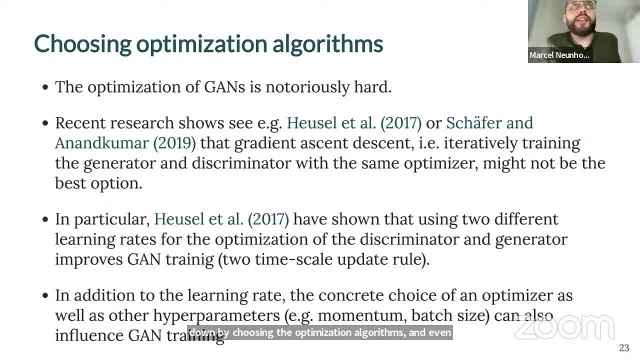 And even though it didn't look like that, but like if you start to play around with GANs for yourself, you will see that the optimization of GANs is notoriously hard, And one reason, of course, is that we don't. 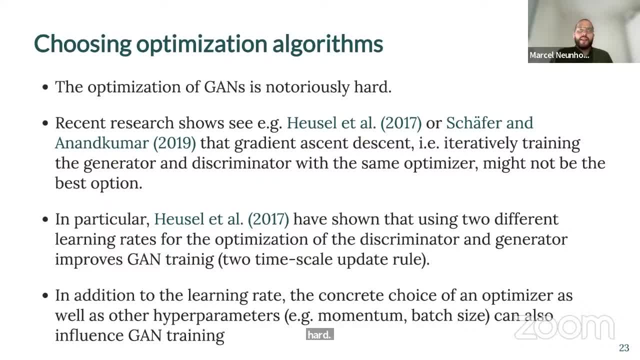 we don't have a lot of data. We don't have a lot of data. We don't have like this sort of direct feedback as we have it in classical neural networks, classical machine learning, whether our training goes in the right direction or not. 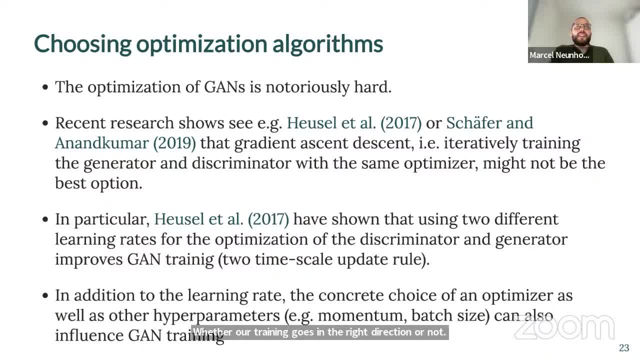 And on top of that, like we have an additional problem in GANs, So in our simple introductory example, So in our simple introductory example, and it's also what they did in the original GAN paper, and it's also what they did in the original GAN paper. 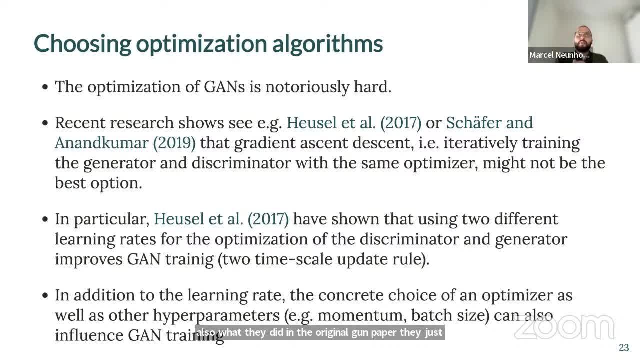 they just used the same optimizer, So the same. basically the same step size, same learning rate for the discriminator and the generator. So like one would take one step in one direction and like the other one would take a similar step in the opposite direction. basically, 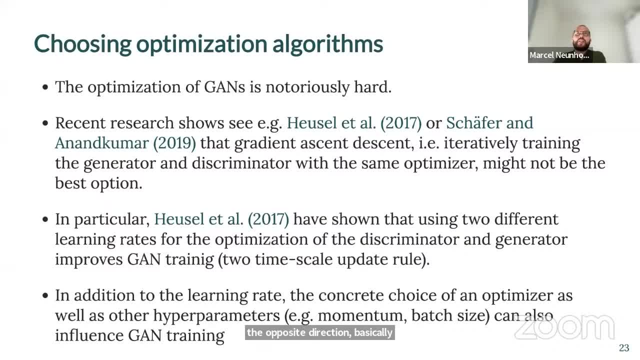 And there's recently, I don't know, and there's recently, I don't know, and there's recently, I don't know, but the research that shows that, like this symmetric gradient, ascent, descent, like because we maximize one ascent and descent, 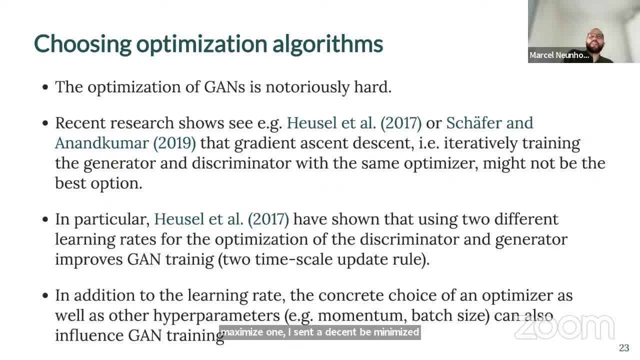 and we minimize the other might not be the best option. In particular- and this is a very cool and simple trick to implement- it very much encourage anyone to play around with that. Hoyes et al, a group from Austria, have shown that using 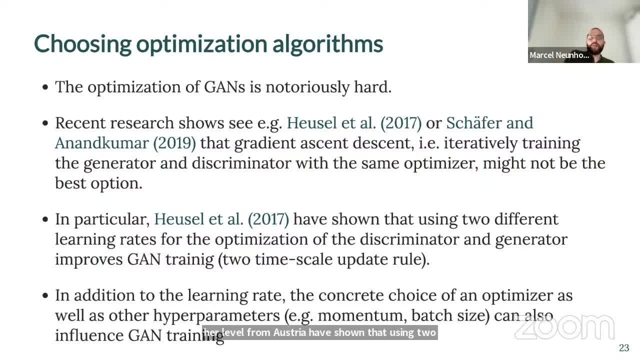 two different learning rates and they show theoretical results for that as well: for the optimization of the discriminator and generator. improves GAN training and in some cases makes it even possible to descent with the same learning rate. fails in some cases To ever get to an equilibrium because it will overshoot. 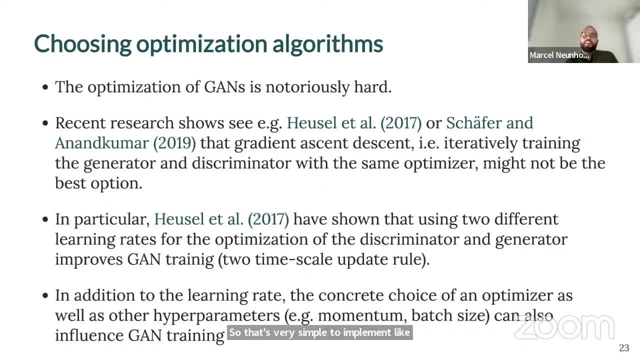 So that's very simple to implement, like just putting like those two optimizers on two different learning rates, And this usually helps to stabilize GAN training by quite a lot. In addition to like the learning rate, like and how to choose like the learning rates. 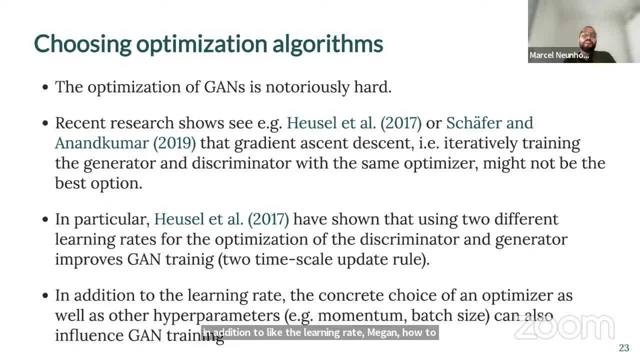 of those two different optimizers. the concrete choice of an optimizer, of course, has an influence like whether you choose like simple as a stochastic gradient descent or like those other momentum based alternatives or updates, like Adam RMS, prop and the like. 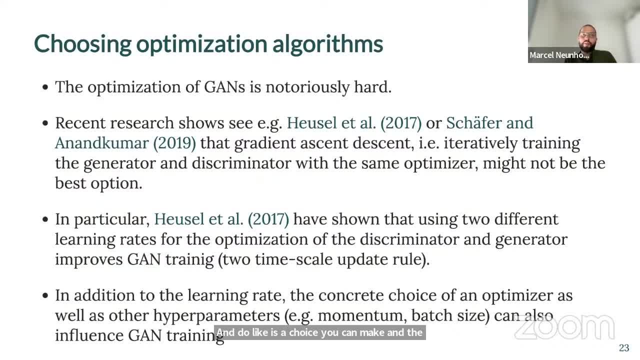 is a choice you can make and they behave very differently And they have all their own hyper-parameters that like those momentum terms on top of like the learning rate, and you can also tune the batch size. that can also influence GAN training. For images it has been shown that like larger batch sizes. 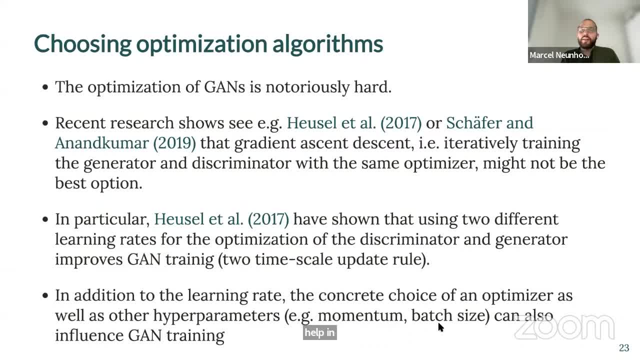 typically help in training the GAN because like it's seeing more consistent. So that's an interesting example. I see that there's a question about noise distributions. I will just read it. Is it misguided to think that we are somehow aiming at some noise distribution that are close enough? 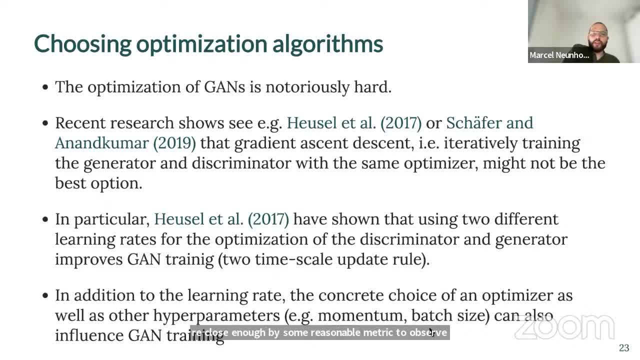 by some reasonable metric to observe distribution, but not so close as to essentially replicated? That's a good question And I guess you could experiment with that So you could, in our original example, use our toy data, like our original data, as the noise distribution and see what happens. 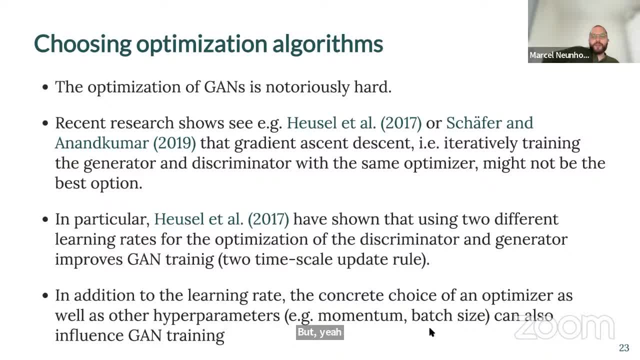 But yeah. so basically with the noise distribution- and that's not so clear with our initial example, but clear with like images and high dimensional data- Our goal is to figure out like a latent space lower dimensional than the original data, lower dimensional latent space, that represents the data wall. 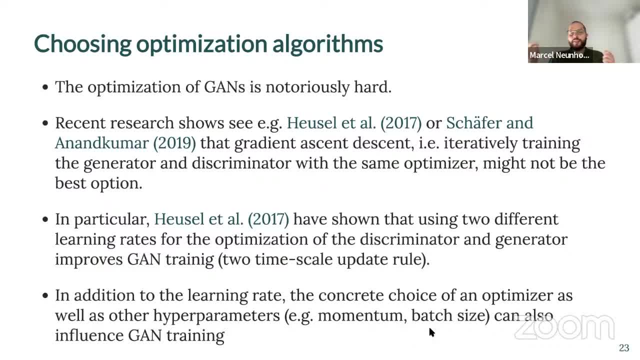 And it should be close enough in terms of like. if you have, for example- and I will show an example of that- If you have, like, holes, if you have areas where no points are, and then you have regions where, like, there's a very high 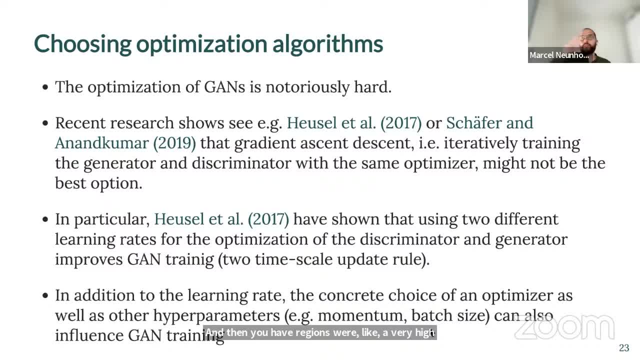 probability of points. if you have such holes, it would be very useful for the prior also to to have some structure like that, but that of course again depends a lot on like the problem at hand like, and how to come up with good priors for different problems is like an open 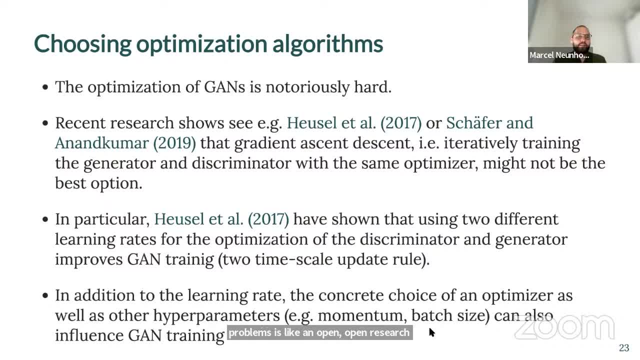 open research question. but I think, like with yours what the end of your question like with, like close enough to the observed distribution, you could run like a very cool experiment with that and see what it actually does to you know, your like synthesized distribution, because then essentially the network would have to learn to pass, just pass through any, any input as 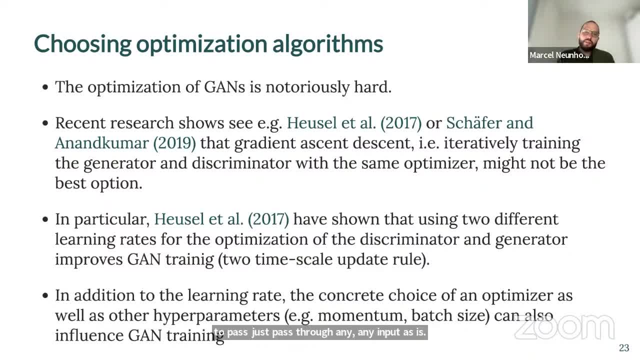 is, and if it does that like, it would just perfectly replicate the original data. so therefore, yes, like, we would like something more like a, like the, like a latent space representation. try to figure out like a latent space representation of the data, and if both are low dimensional, we could of course, use the same as well. 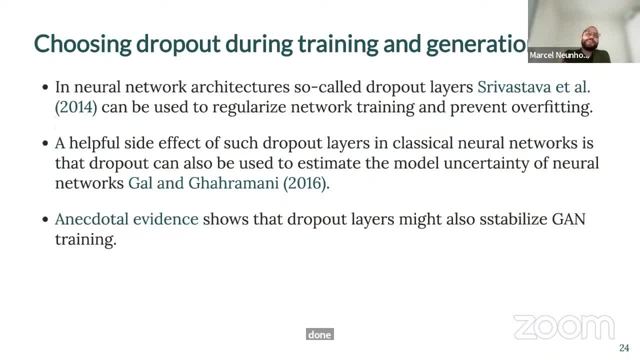 then, like one thing I talked about a lot already because I think this is really interesting, is the next thing, like choosing dropout during training and generation. So in neural network architectures in general, like those dropout layers help to regularize network training because we add noise. 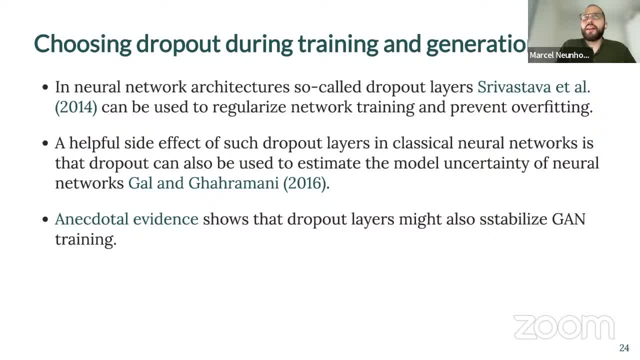 and prevent overfitting. And in classical neural networks there's like a useful side effect of that that like those dropout- like using dropout in prediction- can be used to estimate model uncertainty of neural networks so that you can get error bars around predictions. 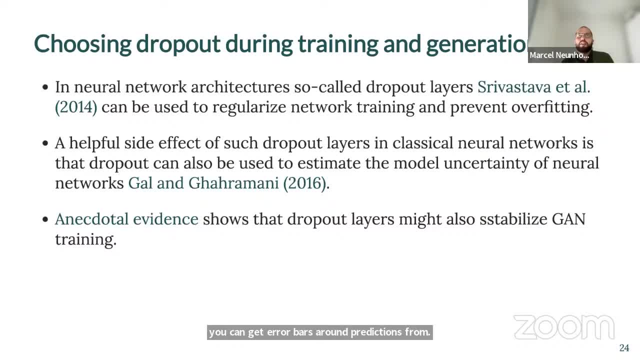 from like classical neural network predictions In empirical GAN applications or applied GANs. there are some anecdotal evidence like it's very good, like GitHub repo on, like GAN hacks and tricks on how to train them best, linked here- shows that dropout layers also stabilize GAN training. 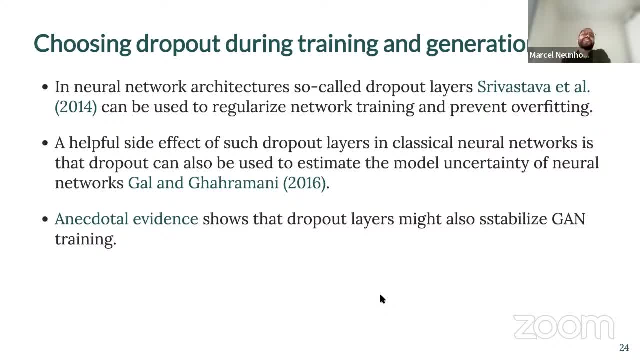 Sorry for the second S there And again, that's like that's like. that's like something you could try out very easily by just adding dropout layers during training and in classical neural networks, And what you would also do typically in GANs then is then. 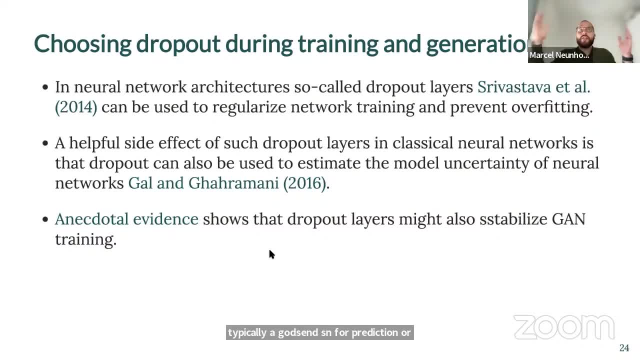 for prediction or for data generation, you would just average across all nodes so that you basically don't have, like this, randomness in predictions. However, sometimes you want this, like if you want to estimate model uncertainty, And a similar thing is true for generative address error. 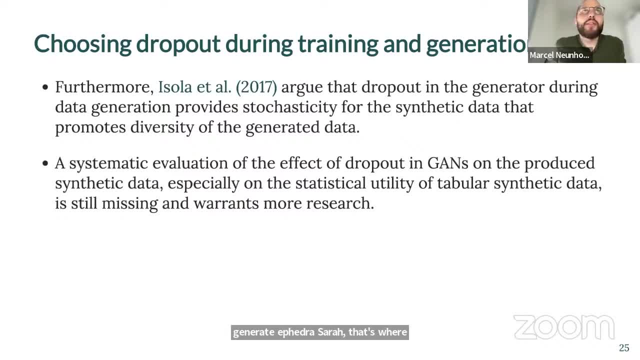 And that's where a group easily at all show and argue that dropout in the generator during data generation also provides additional stochasticity for the synthetic data generation. that in turn promotes diversity of the generated data, Like what I hinted at before and what I hope to show you now as well. 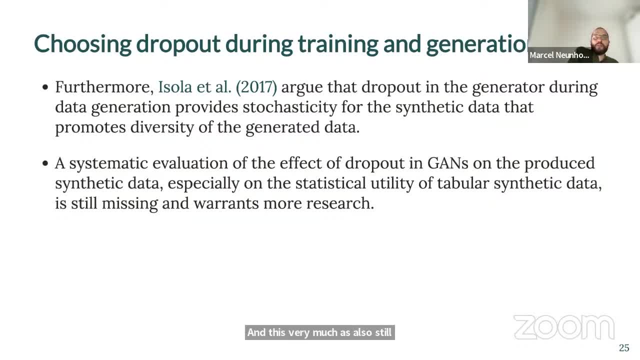 And this very much is also still very open, many open research problems that like if anyone wants to embark on moving the research frontier in the generative address error, and that's when you think about dropout, like the effect of dropout in GANs on produced synthetic data. 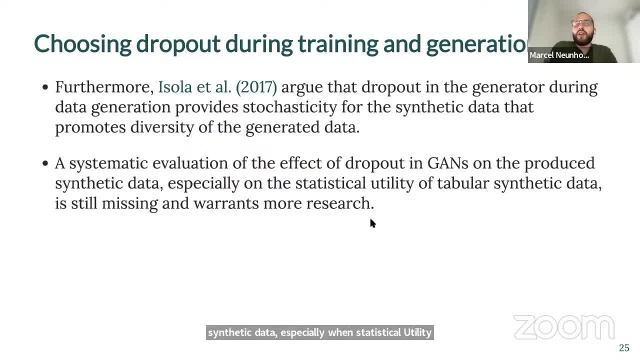 especially when statistical utility is not really researched yet, like not at all. And I think this warrants definitely more research and I will show you like a simple, quick experiment like of why I think like that easily at all, are right Like that. we need to think about this more. 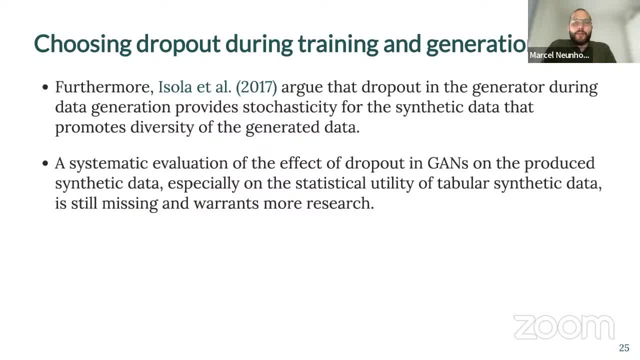 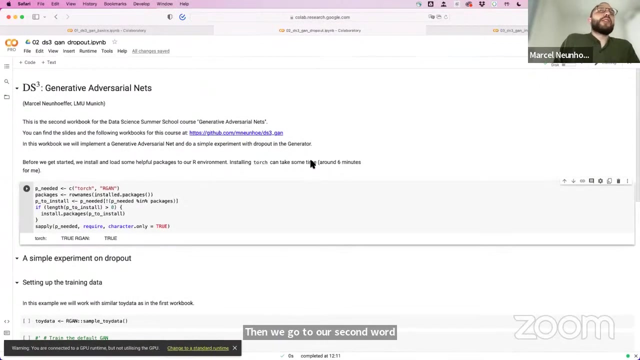 in terms of like tabular data as well. All right, are there any questions about like this design choices part, like the theoretical text, heavy part at this point? Yeah, That's be the case. Then we go to our second workbook on, which is conveniently called GAN dropout. 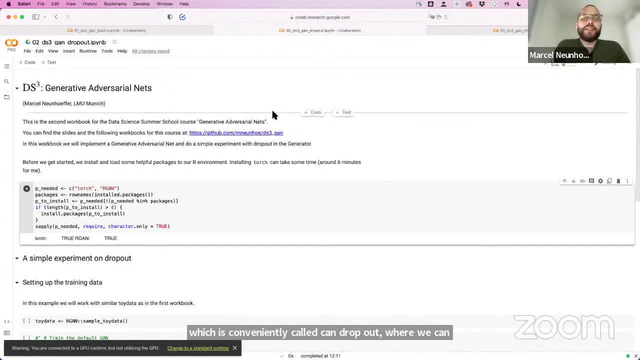 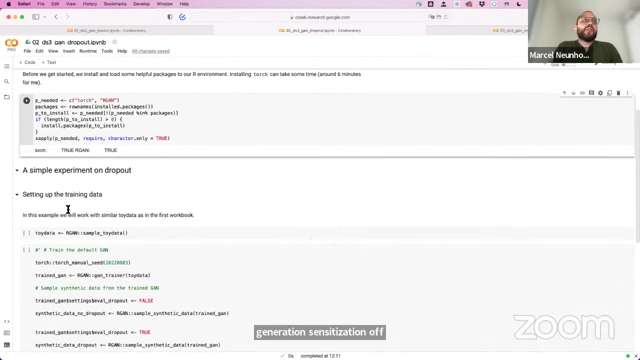 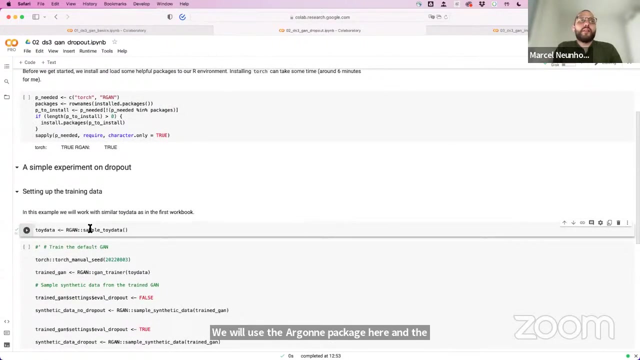 Where we can use- I look at like just simple experiment would drop out in, excuse me- during training and during generation slash. synthesization of data from Argonne. We will use the Argonne package here And the toy data that comes in the Argonne package. 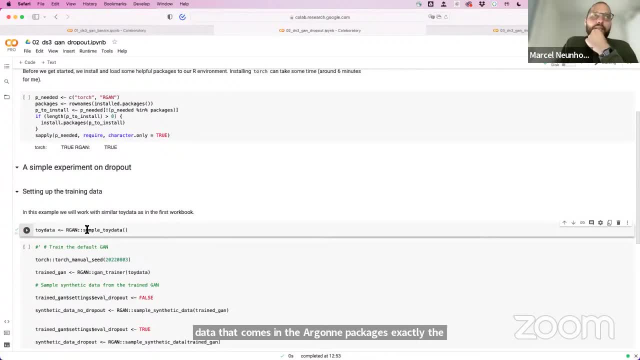 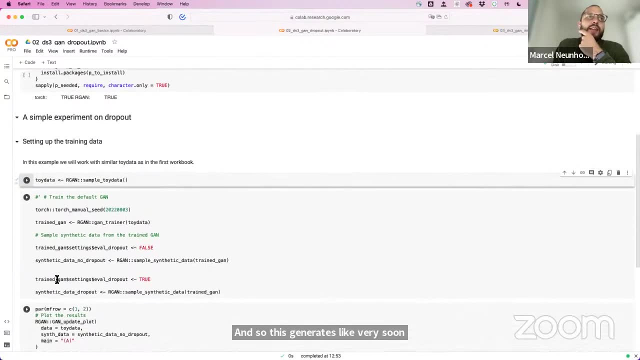 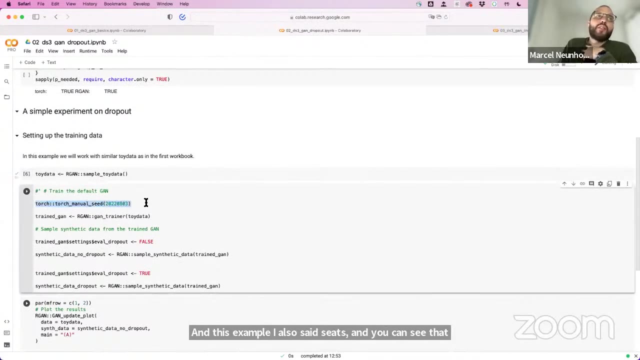 is exactly the same that we looked at before, that we coded ourselves, And so this generates a very similar data set. In this example, I also set seats And you can see that you can also control the torch seats. So if you just set a seat in R, this: 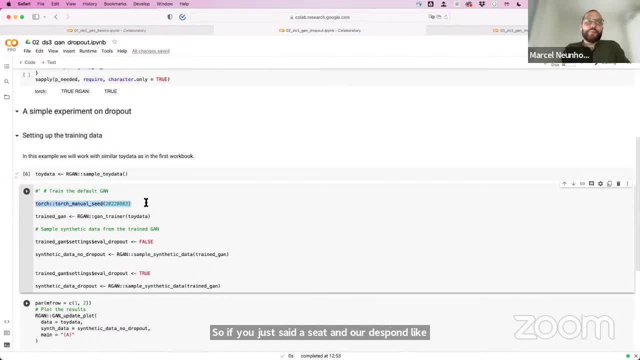 won't set the seat to torch automatically, but you can set a seat to torch as well so that you get consistent results. So what we will do here is we will just train the default GAN and Argonne on the toy data and then use the settings of the trained GAN. 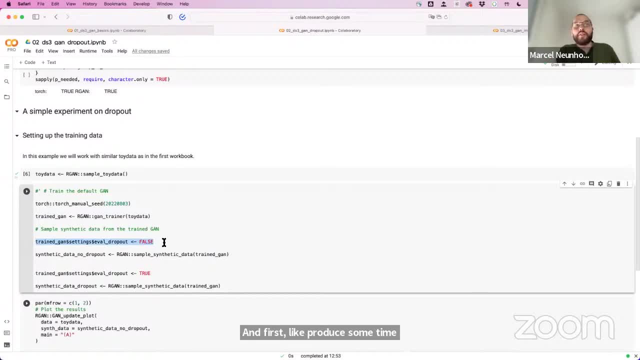 and first produce synthetic data without evaluation dropout. So the default network has a dropout during training, but this doesn't mean that we have to use it during data synthesis. So the default network has a dropout during the session and produces a sample of synthetic data. 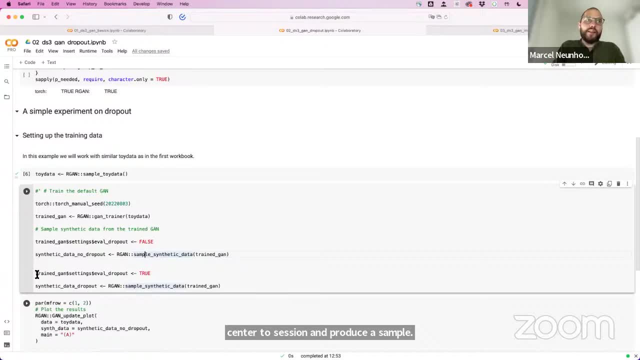 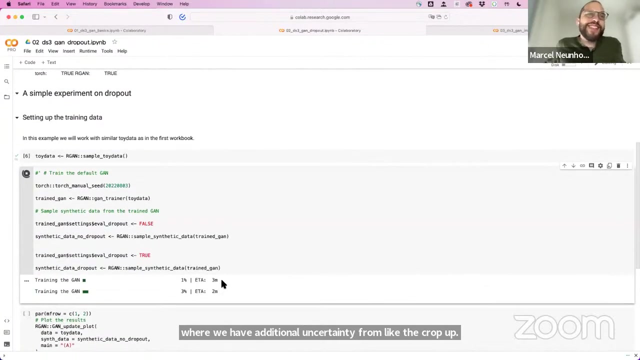 without dropout, during generation, And then a second time where we set this evaluation dropout, so during generation, to true. So the second synthetic data set will be generated from the same GAN but where we have additional uncertainty from the dropout. OK, So this will now run for three minutes and train our GAN. 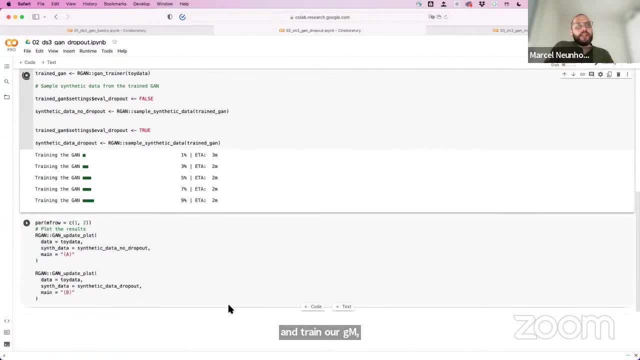 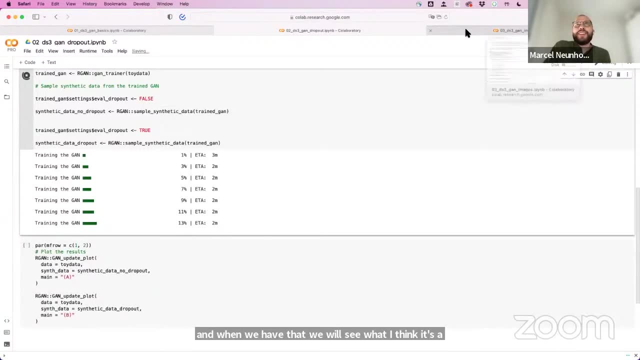 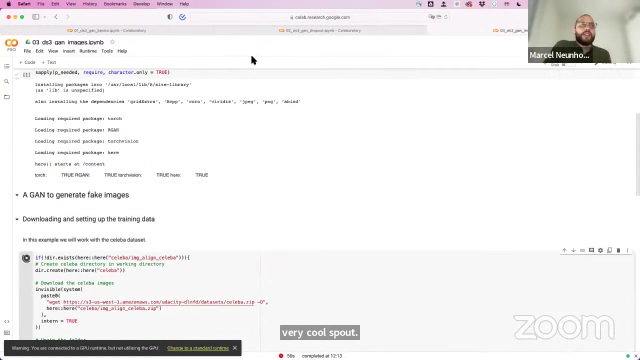 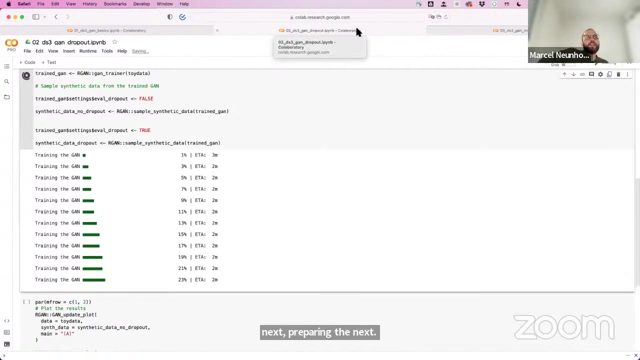 And when we have that we will see what I think is a very cool result. In the meantime, I'll just see if this looks good preparing the next Notebook. So this is now playing around with one of those design choices, namely the dropout during generation and training. 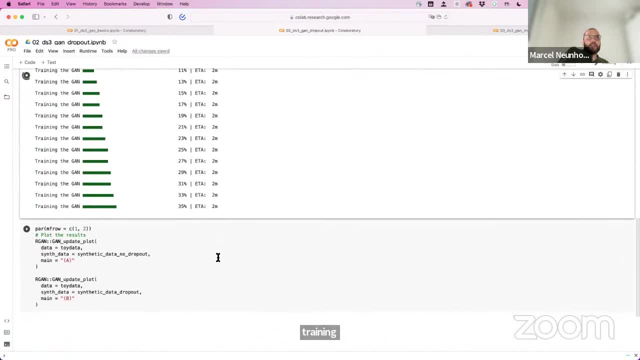 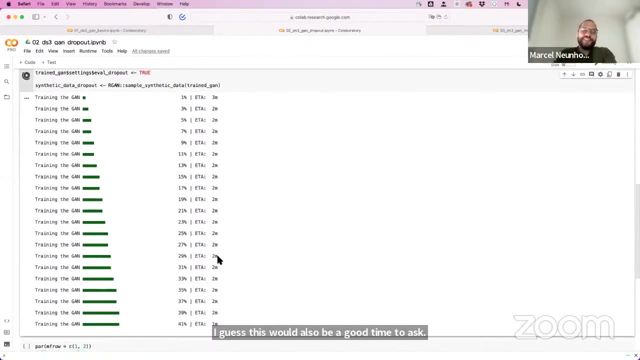 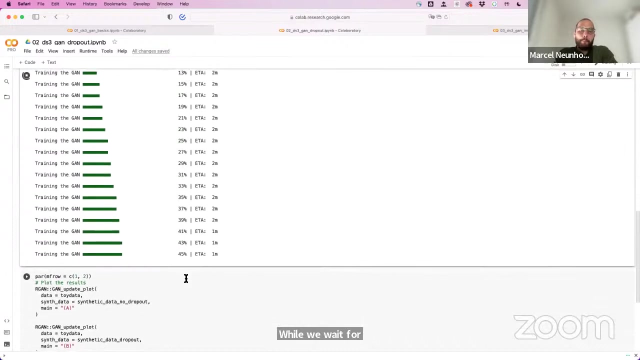 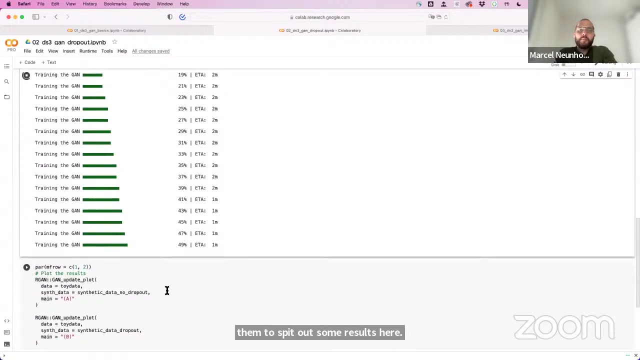 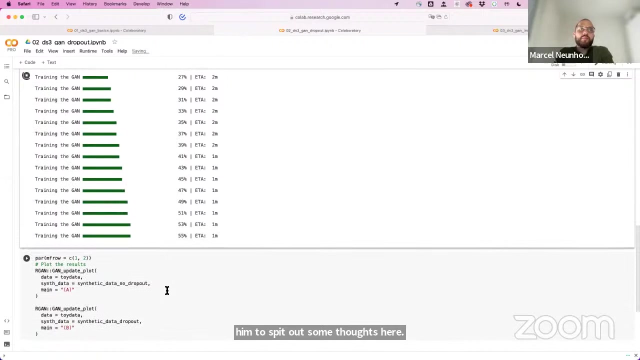 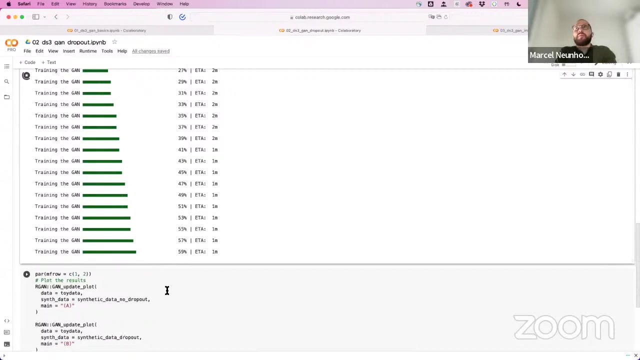 And I guess this would also be a good time to ask away any questions while we wait. OK, Great for our GAN to spit out some of her thoughts here. Thank you, Thanks a lot. Thanks for the question. Thanks for the question. 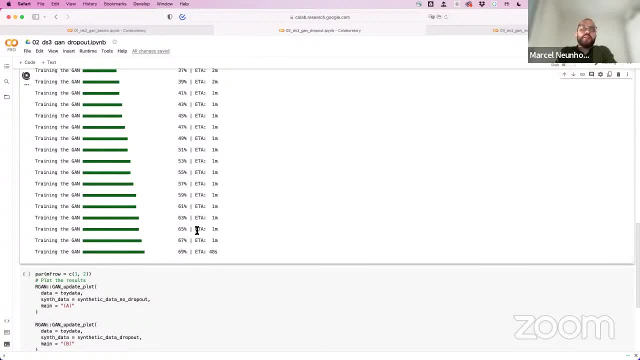 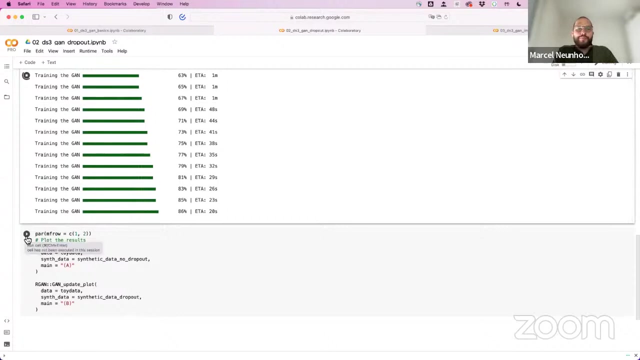 Thanks for the question. Does anyone have an expectation? what I guess I gave it away before- what we will see in those two plots without dropout and dropout? OK, We'll see. Actually, no idea. That's why we run it and we can look at it. 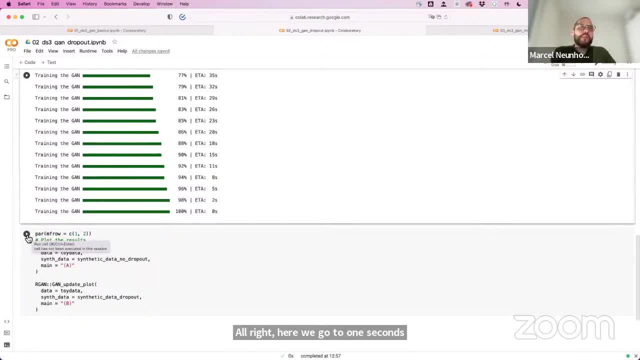 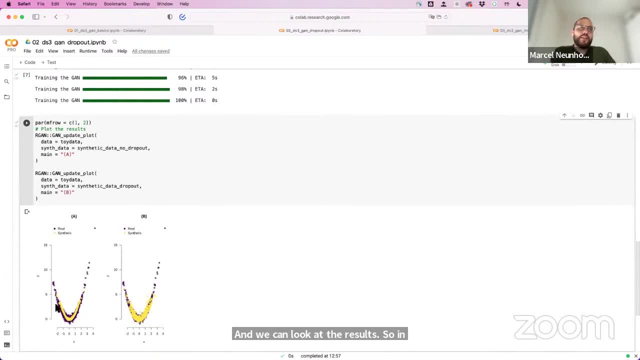 All right, Here we go Two more seconds And we can look at the results. So in the left panel, in panel A, you see the results of the GAN without dropout during generation, And what you see is exactly like this. 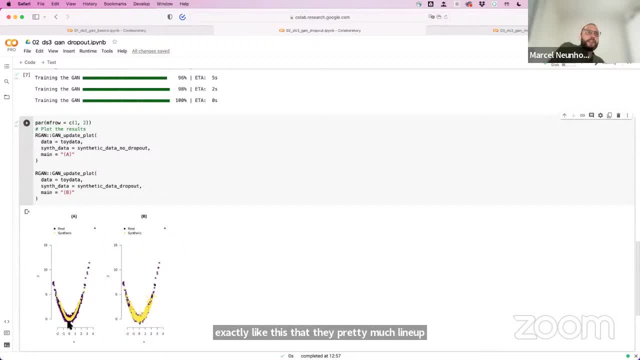 that they pretty much line up around the function. Think of it like a regression line that we wanted to learn Right. However, that means that we don't have. if we use that to sample synthetic data, we won't ever get this point or a point close to this one. 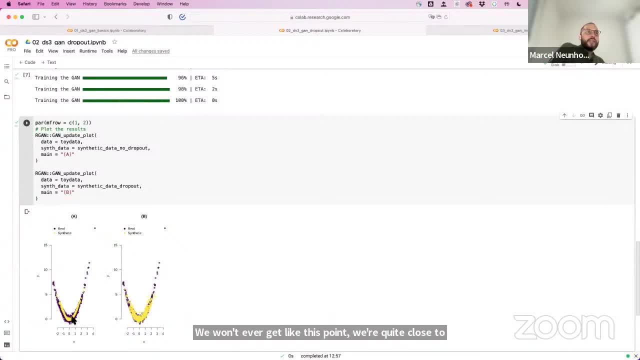 We won't ever get a point close to this one right Because it's lacking: this model, uncertainty of the GAN. Even if we would pass different noise they would all like, all the generated points would come Right. So we would have a cluster around this line here. 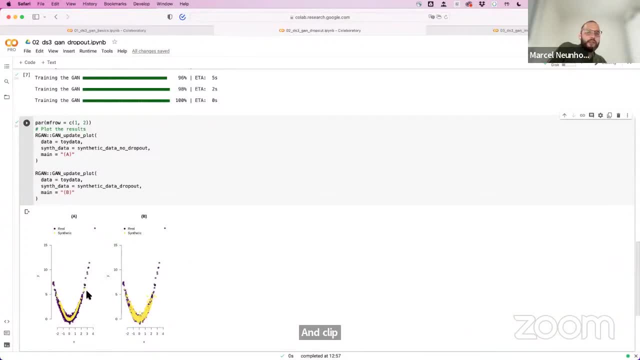 And typically this is not what we would want. if we think of synthetic data right, Especially in the statistical sense- We would hope to get something that looks really close to the original data, And it's like when we produce the synthetic data here. 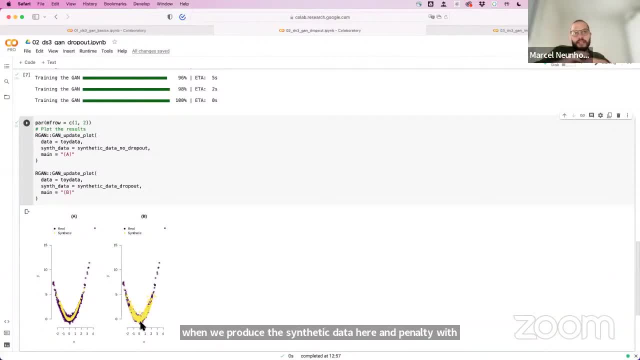 in panel B with dropout during generation. That means when we pass the noise to the generator network and generate the data, we will randomly switch some of the learned parameters off And this means we will get slightly different results even if we use the same noise vector. 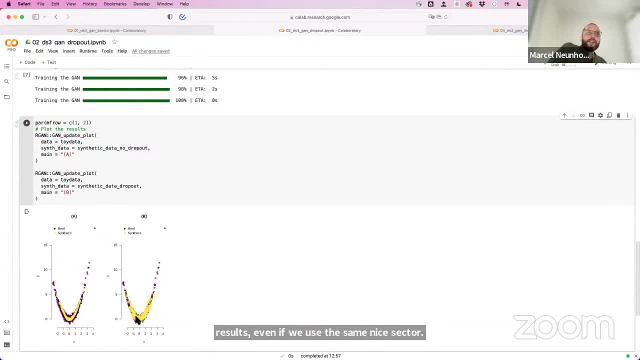 every time we run it through it, And this actually promotes diversity, right. Like we see that this now gives us like data that looks actually closer to the actual data. On average, they will be the same, right, But here we have, like this, additional variance. 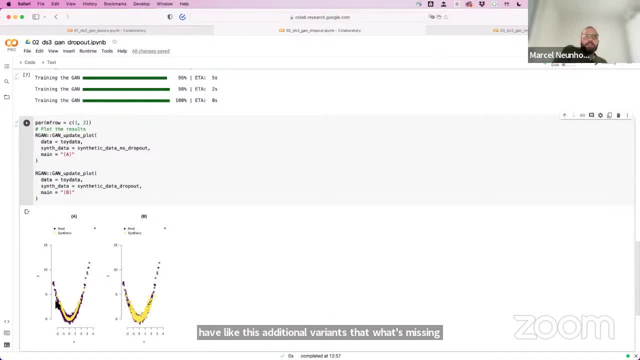 that is missing in this picture. So now I guess an interesting thing is that we have a lot of data that's missing, So we need to experiment or like. pushing this even further would be like how to assess quality of like such data, right. 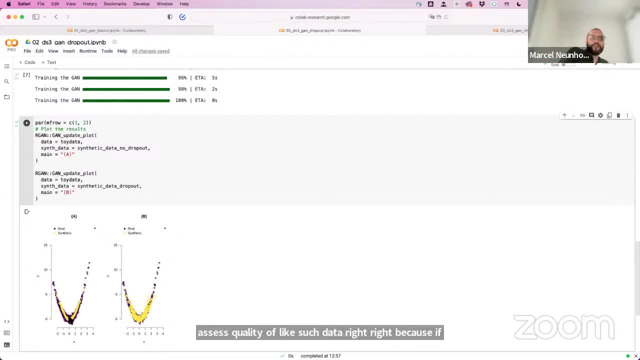 Like, because if we were just interested in like average results, then this would be pretty good And probably even better than this one, because we have higher variance here. So we need a like, a smart way to quantify, like, what this diversity means to us. 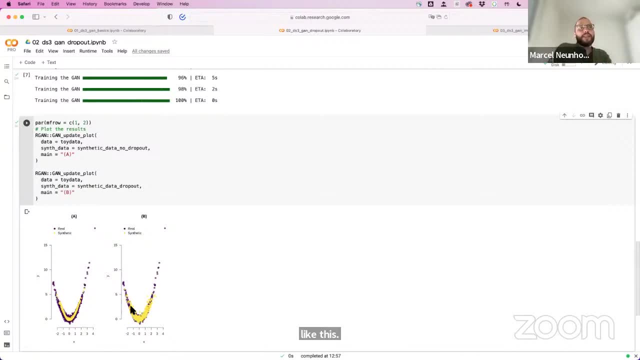 and like how it contributes to quality And, to be honest, I don't have a good idea yet how to quantify this And it's not easy to quantify this, But maybe I can get some data to show you what's the next thing that we can do to also get. 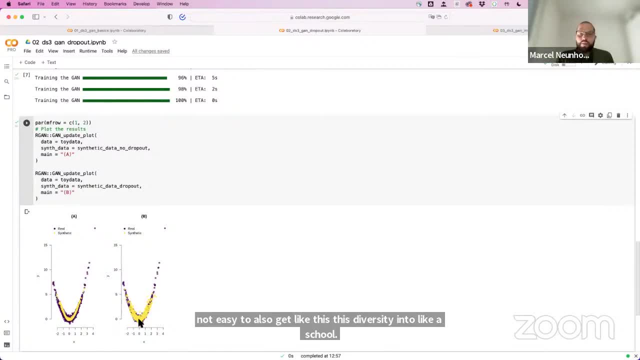 like this diversity into like a score. There is two questions, there are two questions or three questions actually. So first question is: does the kernel density look more similar in B? I'm not quite sure. like if you could elaborate on that. 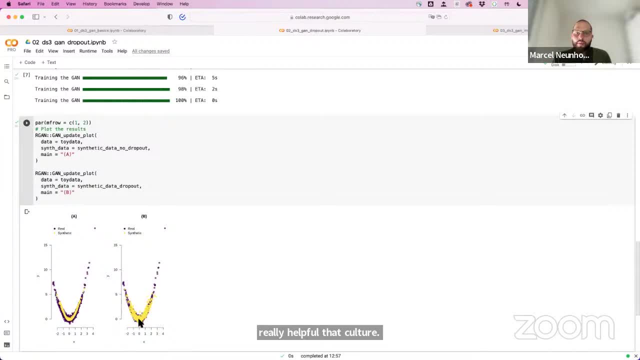 would be really helpful. Not quite sure what you mean, Or are there outlier points, Maybe something else? Do you have questions, layer points? so you mean like those, like getting this one- i guess that's that's a good question- like, um, how that noise translates into both uh dimensions. and then there's a second question, or? 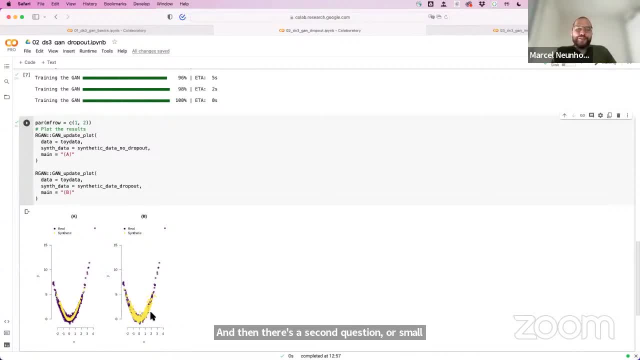 i guess more like a suggestion how to take this, uh, to take this further um. so maybe you should consider using something like a kl divergence to um quantify distributional similarity. the problem with those distributional similarity measures often is that they all they work well with the same kind of distributional similarity measures. 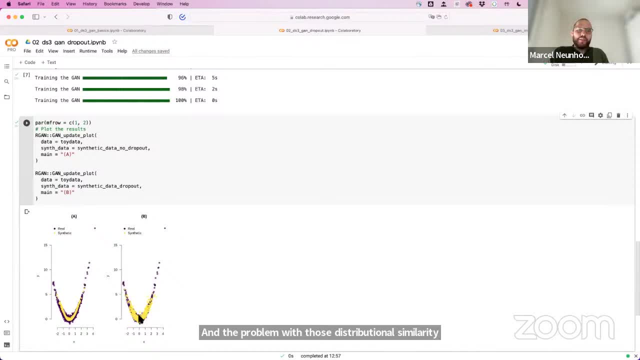 they work well with like one dimension um, but it gets really hard in in multiple dimensions um and um. so, like the Wasserstein distance, for example, for one-dimensional problems is very well defined but it's very hard uh to to assess, like distributional similarity, more than one dimension. 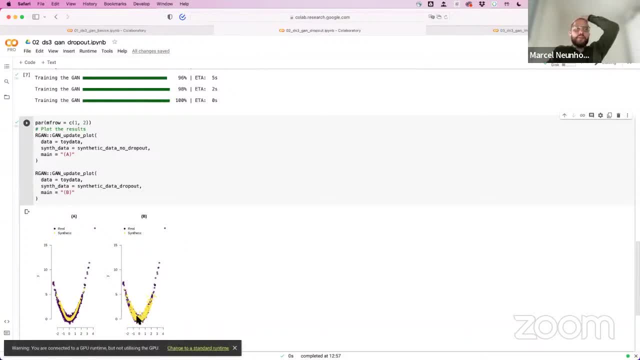 and like beyond that, um, you are running into like the curl of dimensionality and it almost becomes impossible to calculate any, any useful measures. but yes, so, yeah. so quantifying distributional similarity would be a good start. here i agree. and now back to like the first question about like kernel density plots. 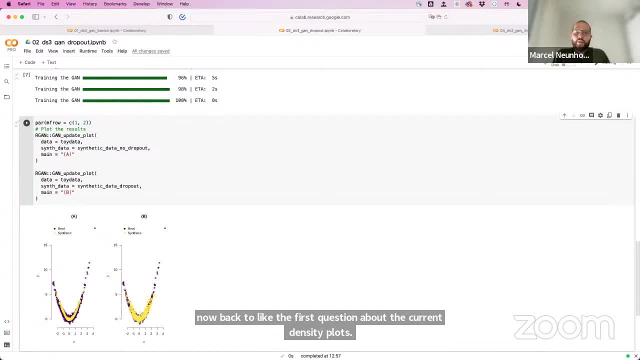 if i create a kernel density plot of the original data, i assume the points on the regression line are more common- would have higher density. yeah, that's right. i'm not sure if that's a good question. yeah, that's right. i'm not sure if that's a good question. i'm not sure if that's a good question. 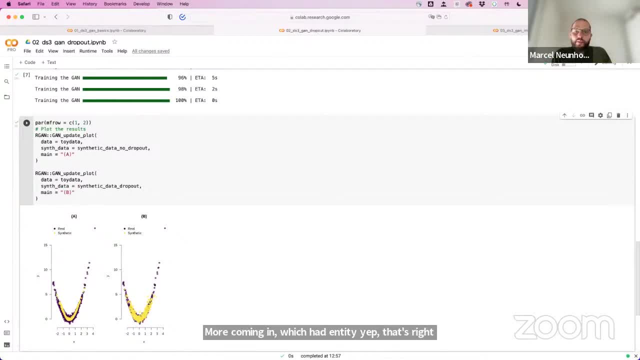 that's right, um, like in the best case. good question, so that without dropout model would probably converge to this high density points? right, because it just is more likely to be there and here. um, in the best case, i guess, uh, like the, the kernel density plots, because it's more likely to be there and here. um, in the best case, i guess, uh, like the, the kernel density plots. 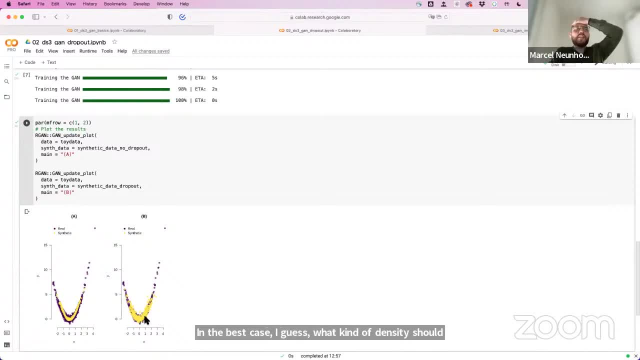 kernel density should look similar of like the generated and the original data to um to have good utility, whatever that means. um- and this, i agree, would probably be better represented by the model with dropout, because here we would have like if we ran a kernel density on the yellow points. we would have like regions where we definitely observe um. 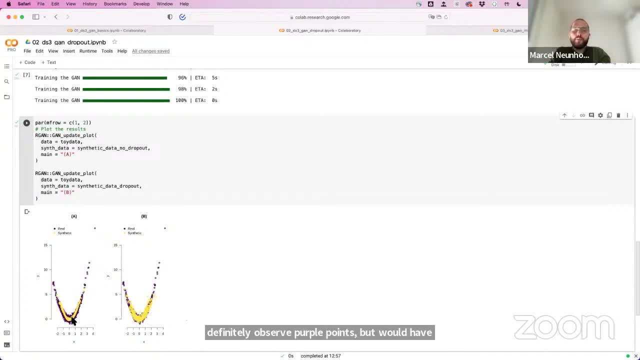 purple points but would have a very, very low probability of observing a yellow point. right, but that's two great like questions or suggestions and i encourage anyone like, if you're interested, if you're hooked uh by generated adversarial networks, to explore uh and and go down that direction. read up the literature and i'm pretty sure 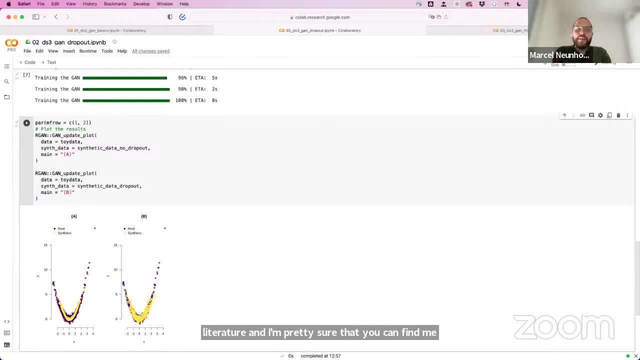 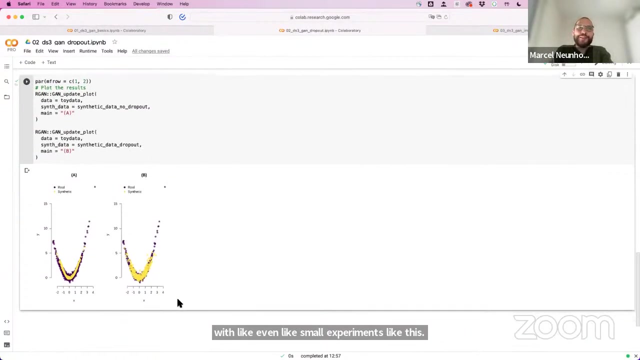 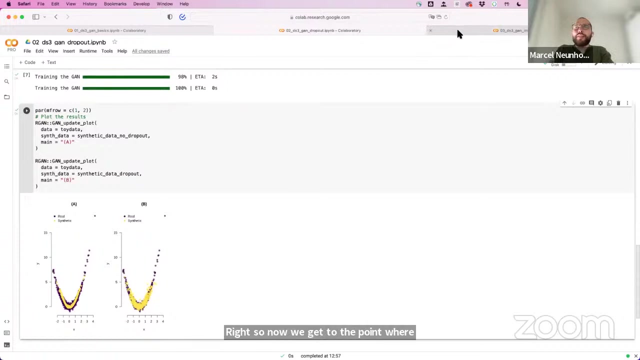 that you can find areas where you could make, uh like, very interesting contributions with, like, even like small experiments like this, um, and thinking principled about um, like what's going on, what's, what's the relationship? all right, so now we get to the point where we try to generate fake images as well and along the way, we can talk about. 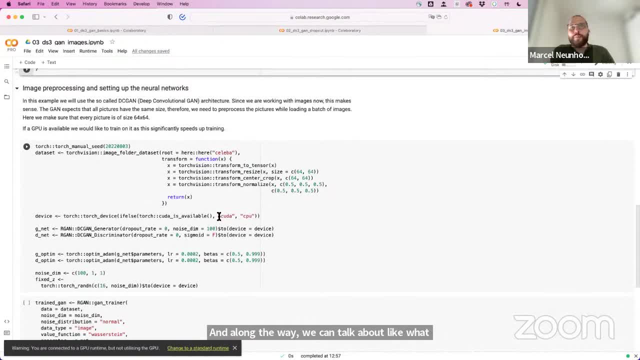 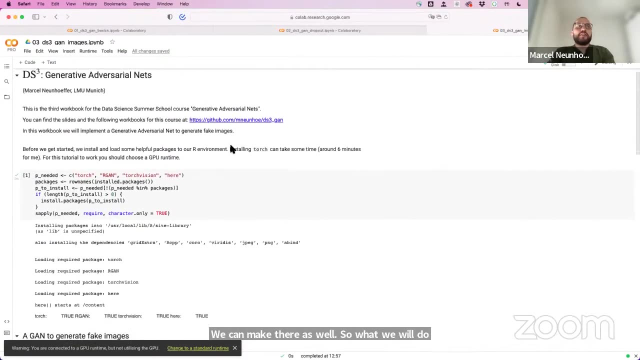 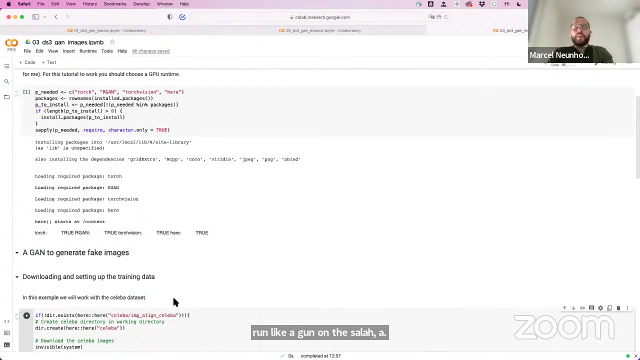 like: what different design choices, um uh, and even design choices that we have not really talked about, um we we can make there as well. so what we will do is we will run like a gun on the celeb. a so it's an annotated data set of celebrity images like portrait. 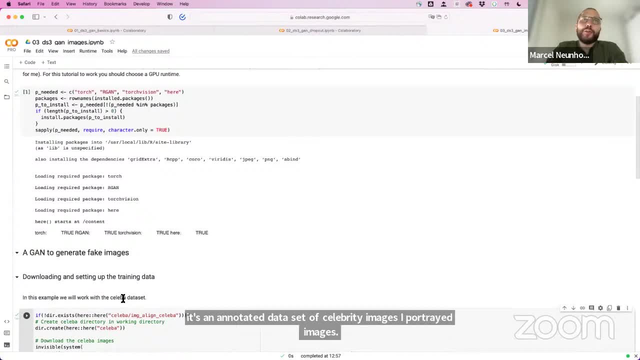 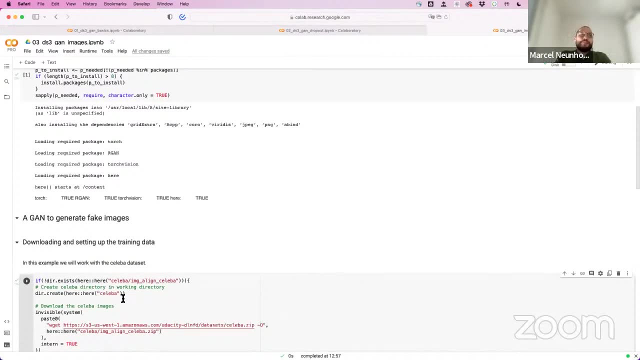 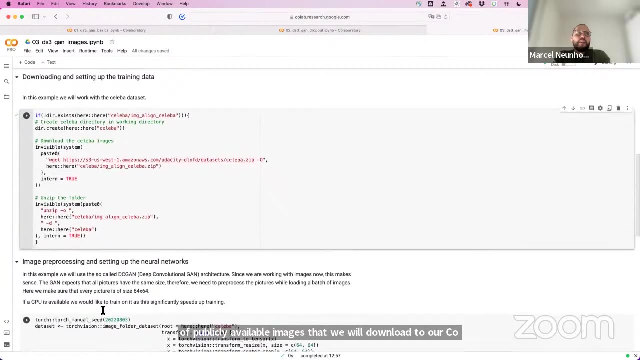 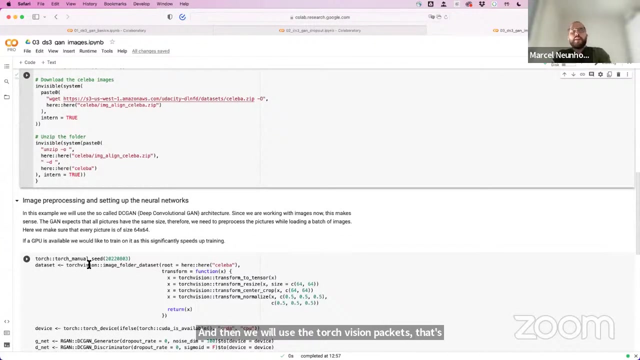 images. that is widely used in computer vision and especially guns, because it has a lot of faces of publicly available images that we will download to our colab environment here, and then we will use the torch vision package- that's again the same as torch vision api in python, where we can then use the image folder. 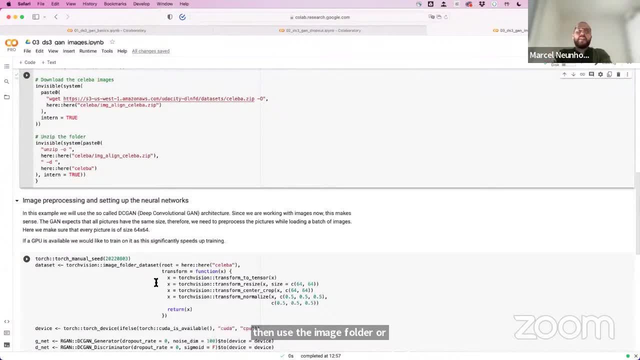 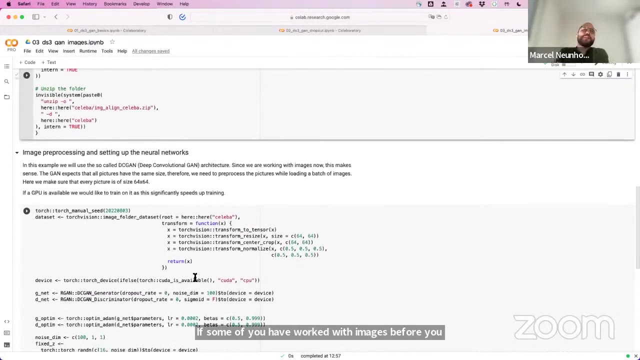 um, or use the image folder to create, like, our data set where we can then sample mini batches from um and like with images- um, if some of you have worked with images before, you have additional problems right, like, because, especially if it's like public collections of images. you have additional issues right because, like, especially if it's like public collections of images. 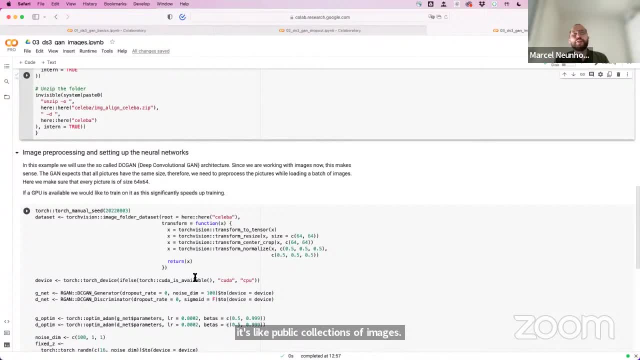 rarely do those images all come in the same size. However, for our GAN architecture, we expect all images to be of exactly the same dimensions So that we can have like one GAN architecture that is fixed across images. So to achieve that, before we load a mini batch, 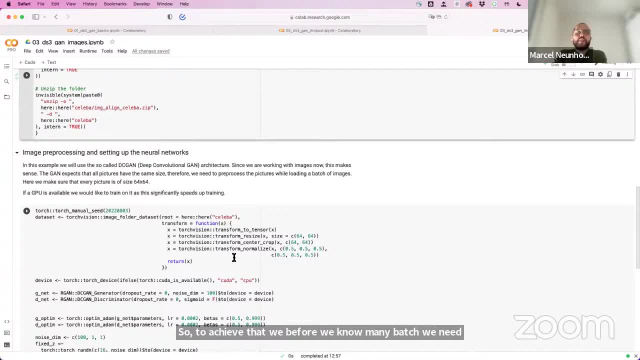 we need to make some transformations on the on the image, where we first transform it to a tensor. That's similar to what we had to do in the tabular data example. Then we resize it to like a 64 by 64 pixel image. 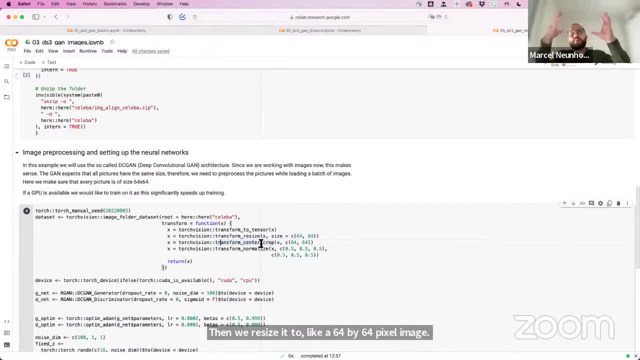 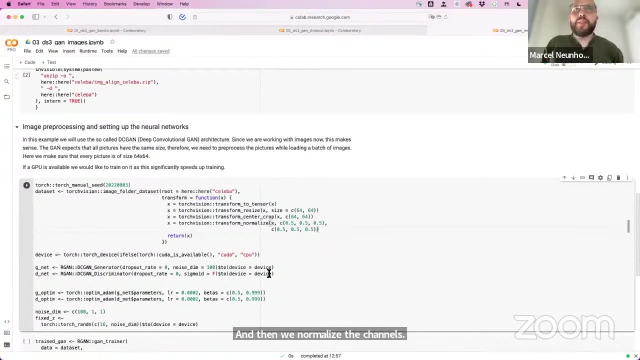 and like want to do the crop on the center And then we normalize it, and then we normalize the channels so that we can have like a good, that we have good properties of the pixels So that we work in a space of like minus one to one. 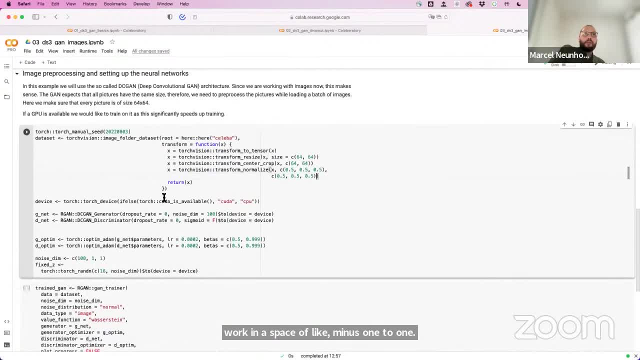 and we can then use this to transform it back to actually produce the images. Here there was a question that was came up earlier. We can look for a CUDA device like a GPU, if we have one, and use that, and it will make a difference on this example for sure. 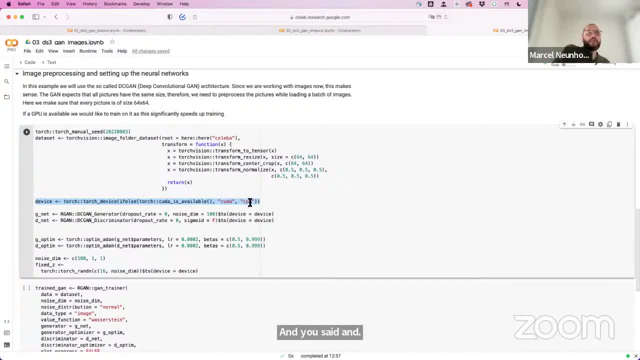 And we'll fall back to the CPU. otherwise, Unfortunately, currently the Colab CUDA version doesn't match with the torch requirements for CUDA, So unfortunately, we can only train you know, we can only train you know, we can only train you know. 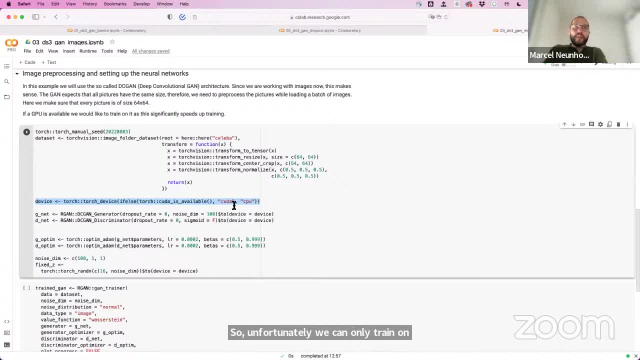 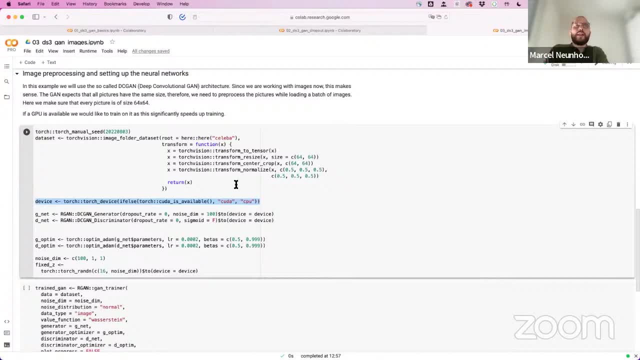 But in the meantime, if you have access to a GPU, this would be sufficient, Like if you have CUDA installed properly and install torch with CUDA installed, then this would be sufficient to choose the GPU to train up. Another thing that came up before here: 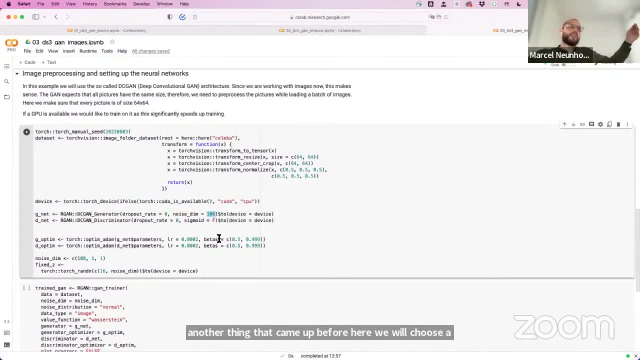 we will choose a noise dimension of 100. So, like each image will be produced from like a vector of 100 independent draws from a normal distribution, And we will now use the DCGAN architecture for the generator and the discriminator, which is like an acronym for Deep Convolutional GAN. 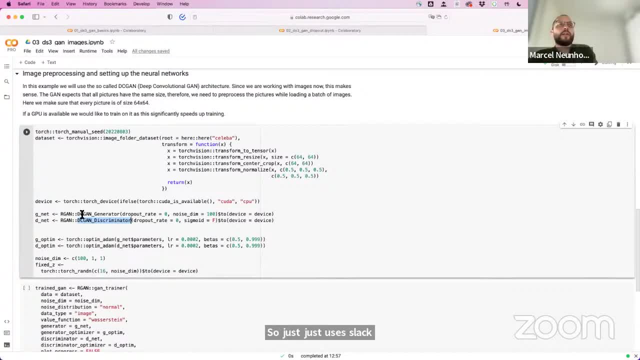 So this just uses several deep- so it's several layers- deep- convolutional modules, So that, yeah, like it was one of the first GANs that produced nice looking images And yeah, So that is simple to implement and to train as well. 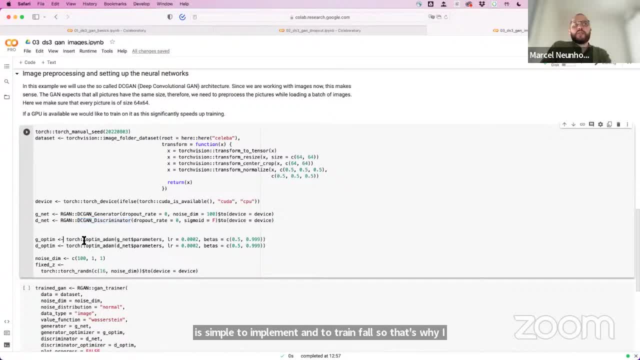 So that's why I chose that here. And then we need those optimizers again, And here I chose like the hyperparameters from the original DCGAN paper, So I didn't do any additional optimization for that, but they seem to work pretty well. 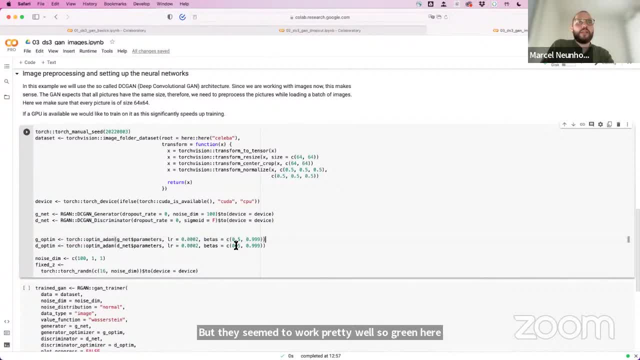 So we use the same learning rate here still, And, and the momentum hyperparameters as described by the office of the DCGAN paper, And then, to sample the noise, we actually need to produce a four dimensional tensor so that it works with this convolutional architecture. 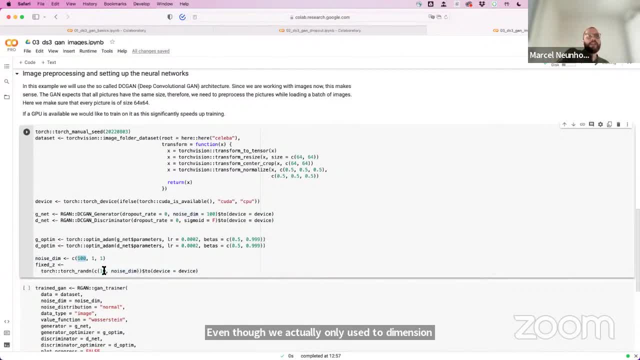 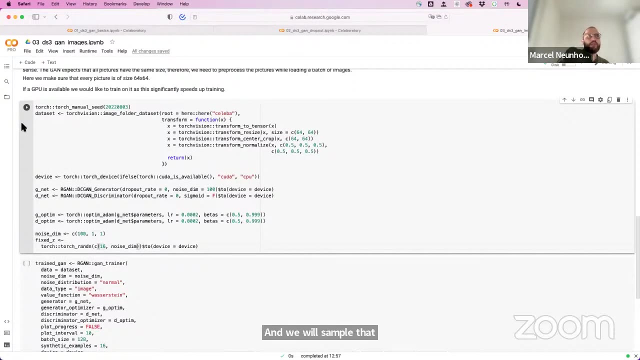 Even though we actually only use two dimensions, we still need like four or basically three channels for each image And and sample that from like a standard normal distribution, The betas in optum atom, like that's two separate hyperparameters. They're both called beta, beta one and beta two. 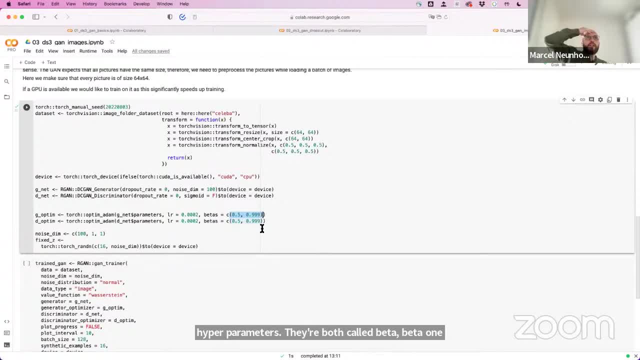 And they basically define the momentum, like of the optimizer. The defaults point 0.9 and 0.99.. And for some reason, like the office of the DCGAN paper, figured out that 0.5 and 0.999 work better. 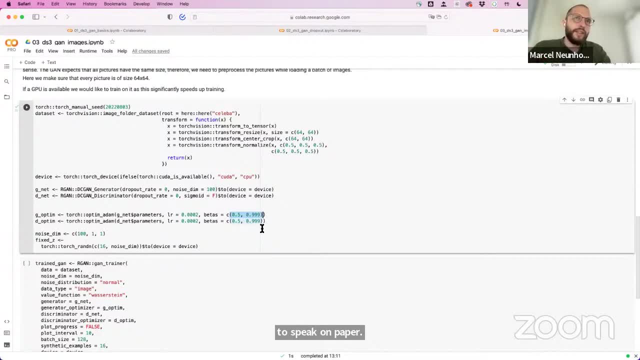 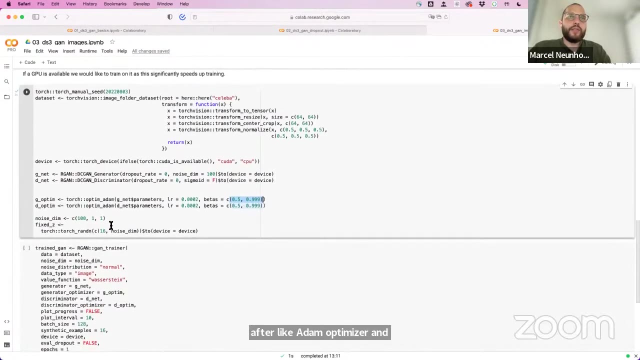 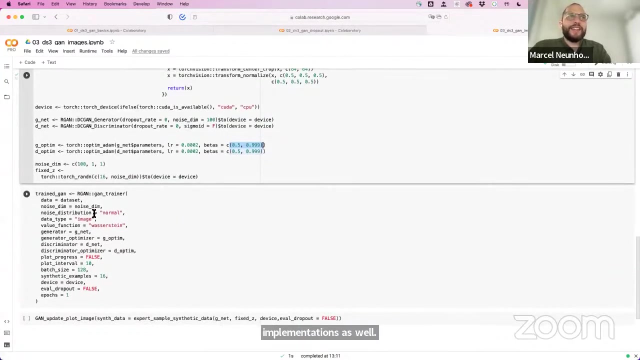 but it has nothing to do with like confidence intervals or alpha or beta levels. It's really just hyperparameters of the of the like atom optimizer, And they are called differently In other implementations as well- Bit confusing sometimes. So now we can pass all of this. 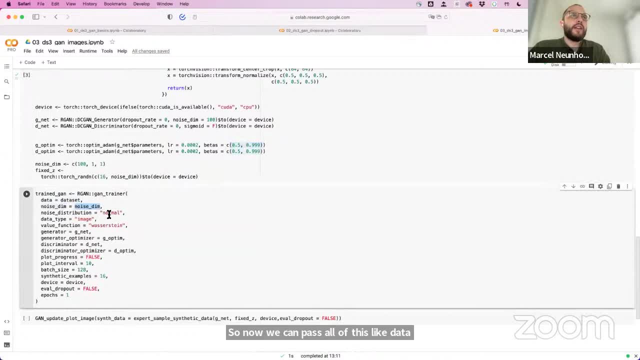 like our data set, our noise dimension, like that we want to sample from a normal noise distribution. Now we have to say we are working on images. We will use the Wasserstein value function here. pass our DCGAN network architecture for the generator. 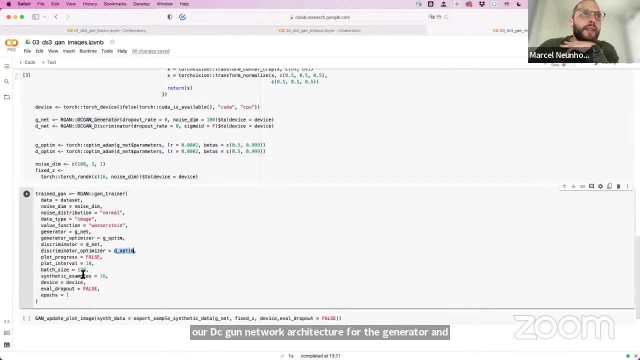 and the discriminator And our defined optimizers in here and work on a fairly large batch size of 128 images, And only run this for one epoch. So an epoch in machine learning is typically defined as the time or the number of steps it takes to 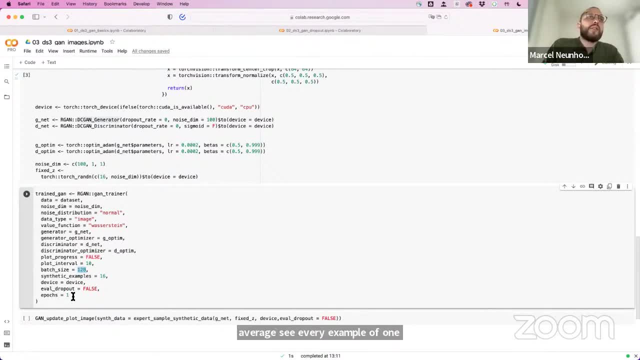 on average, see every example at once. So in this example we have around 40,000 images and use like a batch size of 128.. So that means that like one epoch has around 300 update steps. So we want to run like. 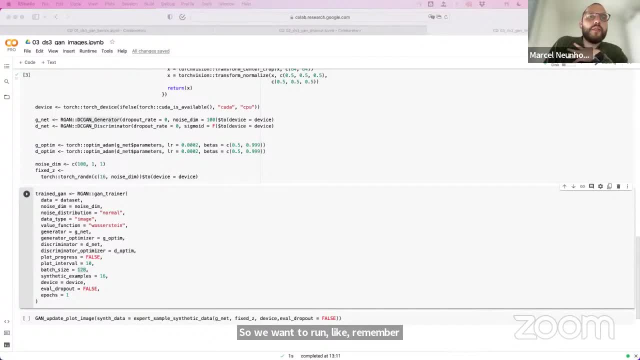 remember before we ran, like our account, for 3000 steps and it was like two minutes And now we just want to run it for 300 steps And because of like this deep convolutional network architecture and the high dimensional images and the higher dimensional noise prior. 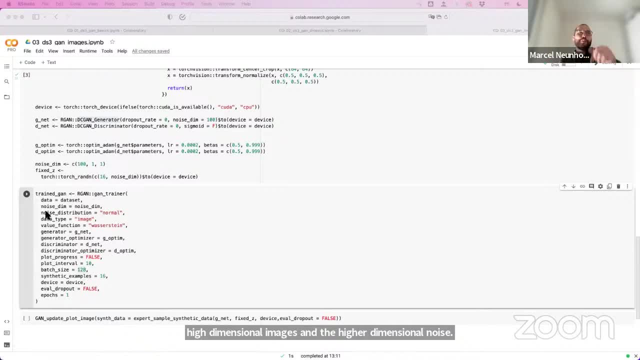 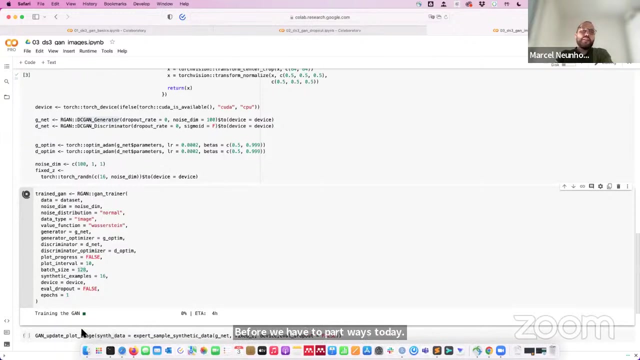 this will take longer, but I hope to show you that we still get to see images fairly soon. So I will just start this here now, but like I have no hope that this will run here before we have to part ways today, So because, like, we are working on the CPU only. 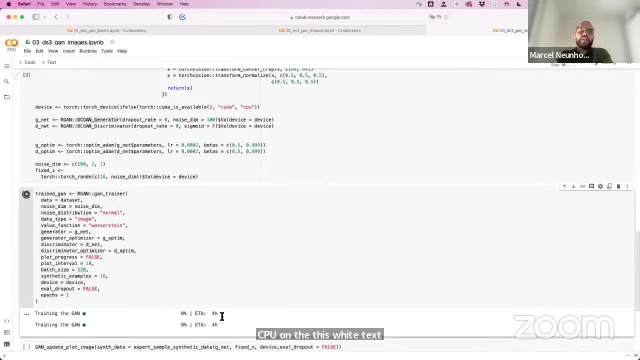 this like takes fairly long for only one epoch right For hours. that's a long time And typically you would want to run this for like a hundred, 150 epochs to get fairly good results. So you can see that, like this is really a limiting factor here. 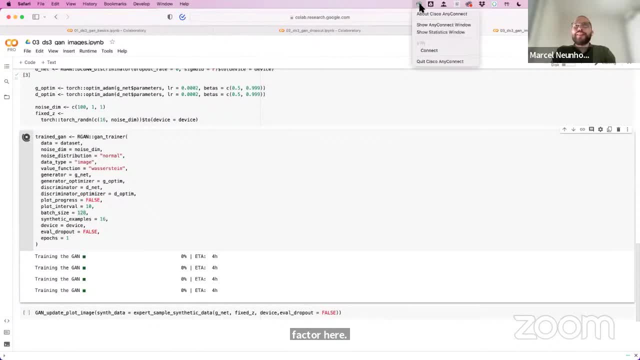 Nevertheless, I will let this run for a bit and in the meantime, show you like I pre-trained this on like my own GPU and connect to that Like I might lose the connection for a little bit, but I will be back, I promise. 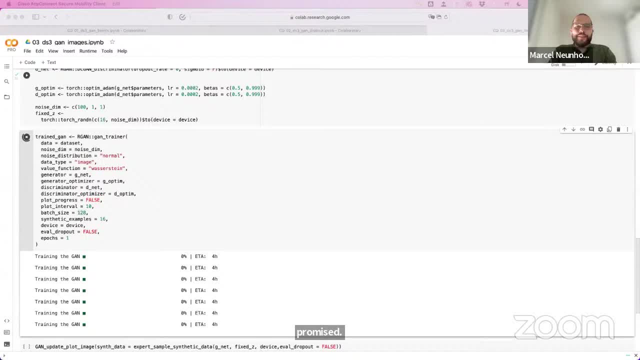 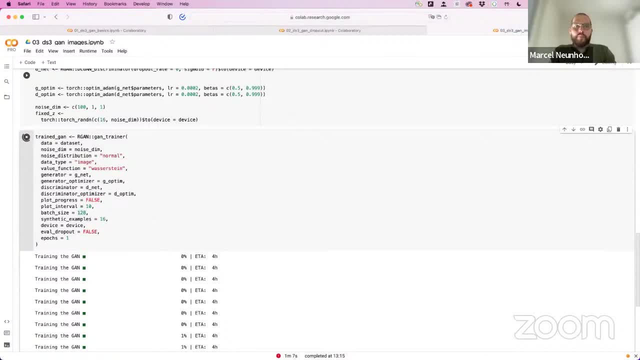 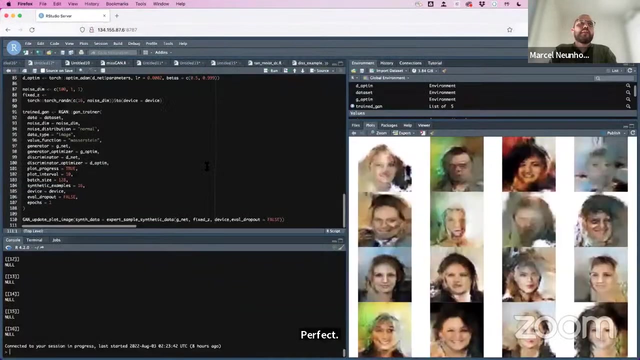 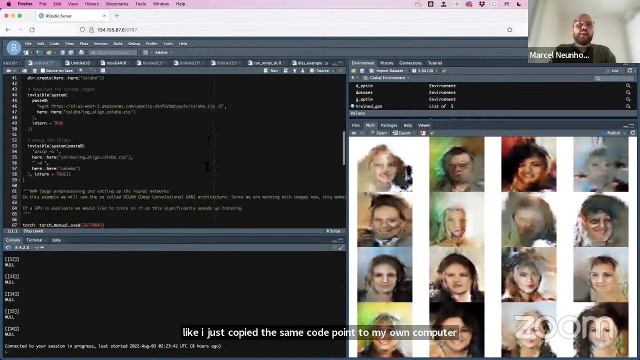 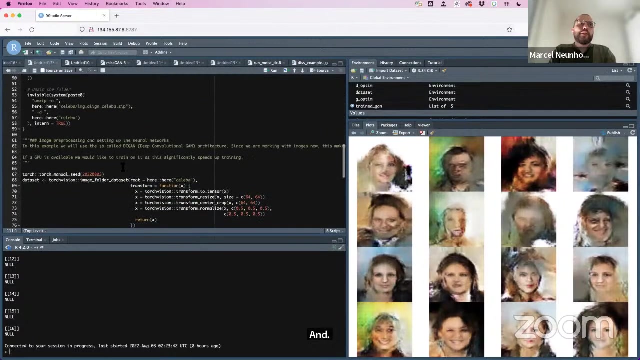 Okay, Okay, Okay, Okay, Okay, Okay. Can you hear and see me? Perfect, All right. So, like I just copied the same code like to my own GPU server here And I will actually also run it so that you can observe training during in real time here. 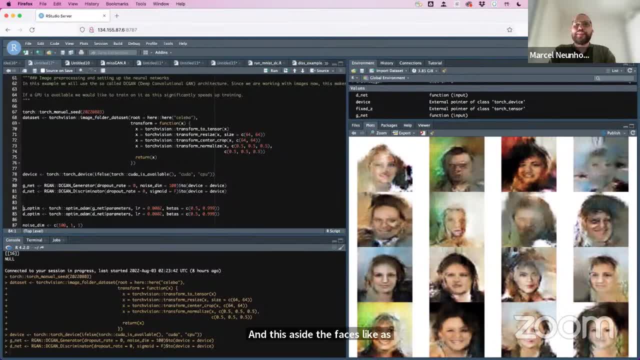 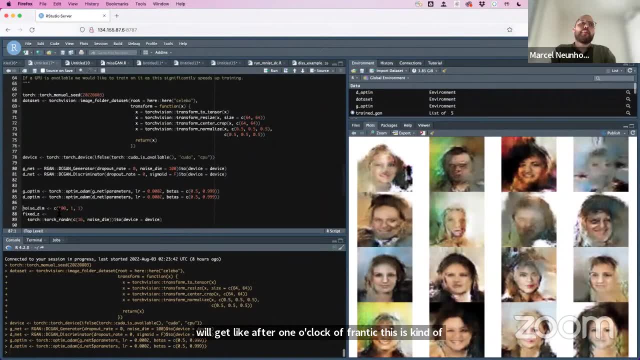 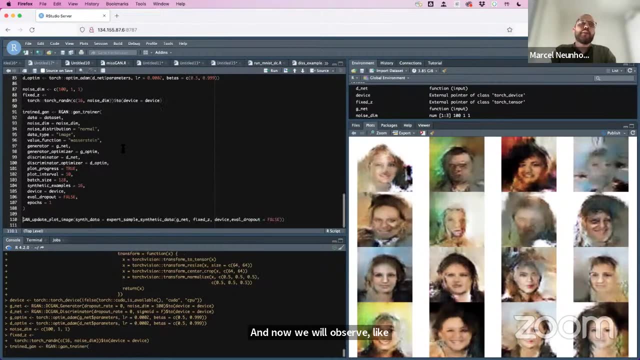 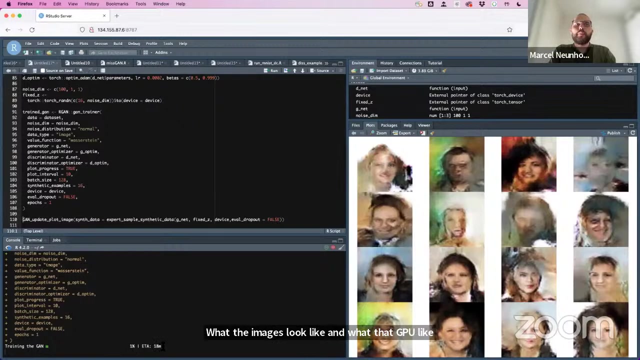 And this is like the faces, like as a like spoiler that you will get like after one epoch of running this, this kind of network. And now we will observe, like after every 10th step in this one epoch, what the images look like And with the GPU, like you can see, like this drastic speed up, like it's the same exact. 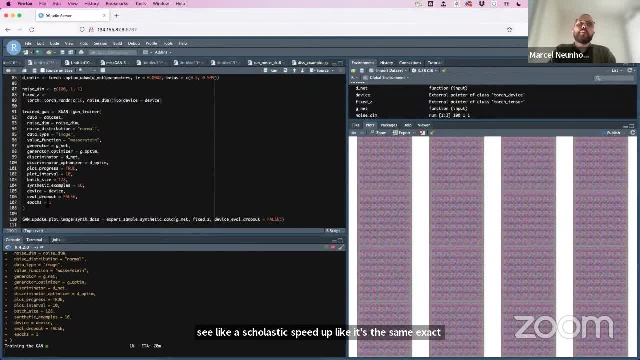 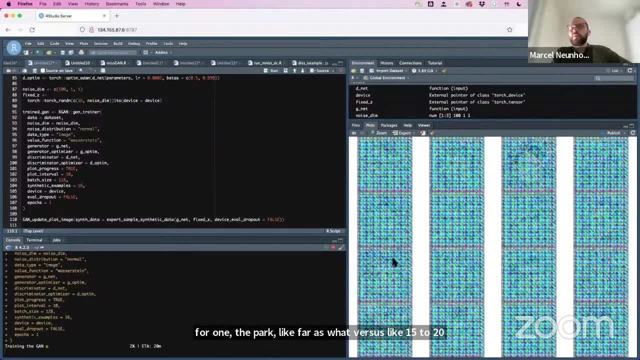 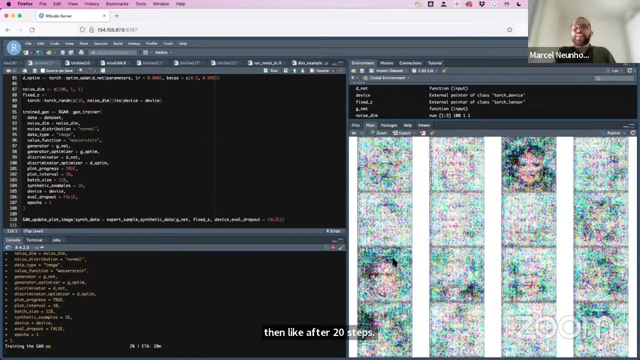 same configuration for one epoch, like four hours versus like 15 to 20 minutes. So this was after 10 steps like it was fairly random, And then, like after 20 steps, the colors changed And then, like after 30 steps, already you start to see like the outlines of faces, right. 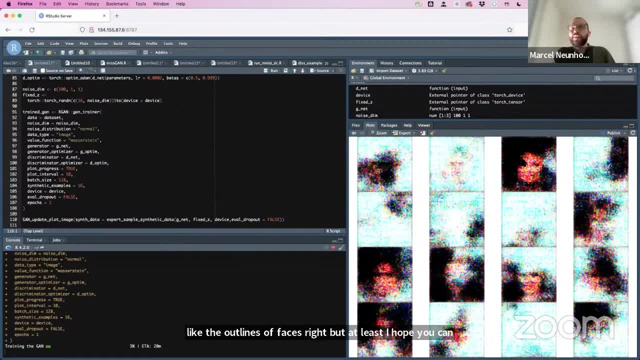 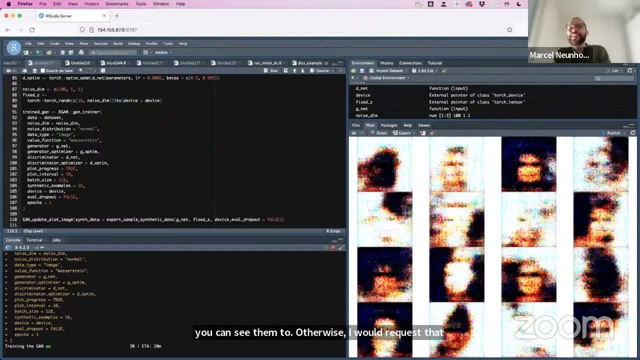 Or at least I hope you can see them too, Otherwise I would need to look less at such pictures and try to make sense of them. But now definitely, I hope, like that we can all kind of agree that we can make out faces And 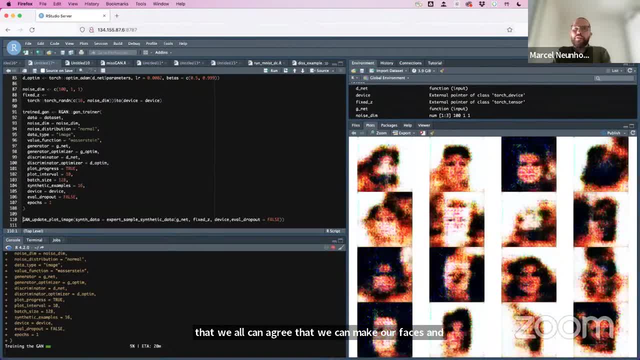 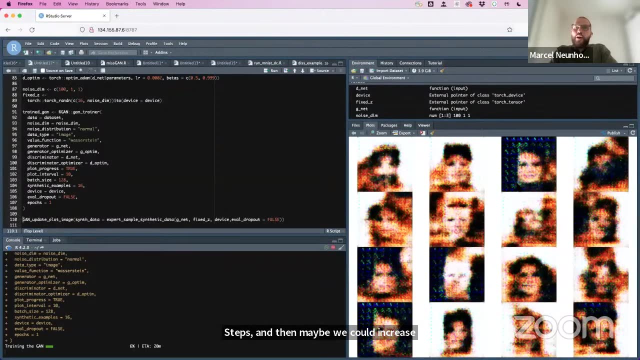 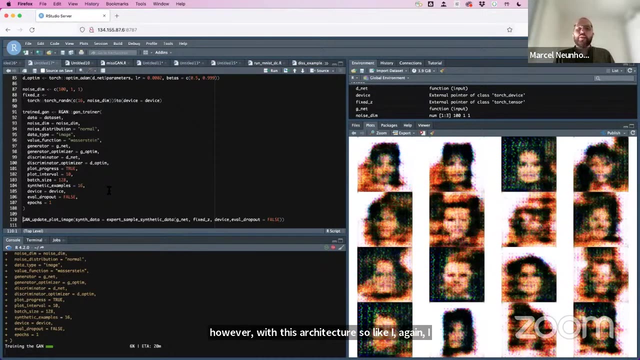 like after a couple of more epochs it will still look better and better, or steps, and then later we could increase the number of epochs. However, with this architecture, so like I again think it's really really cool that like we can on our own machines code something up that makes 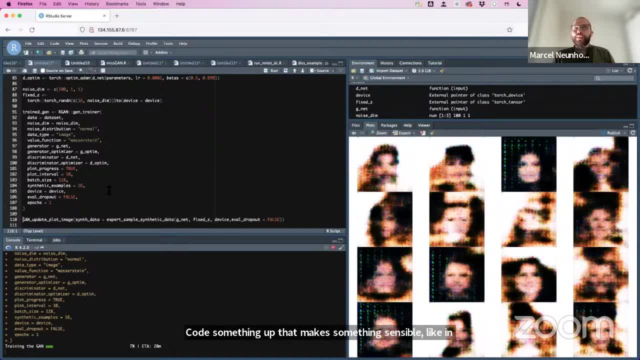 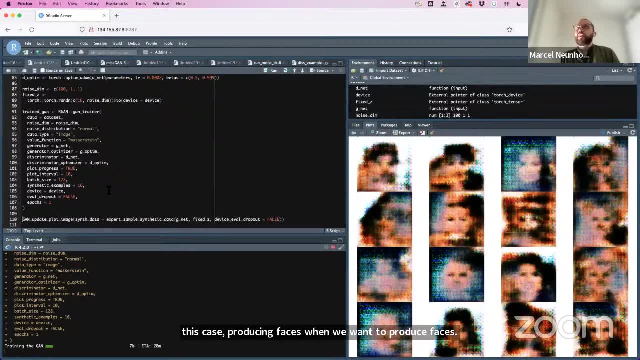 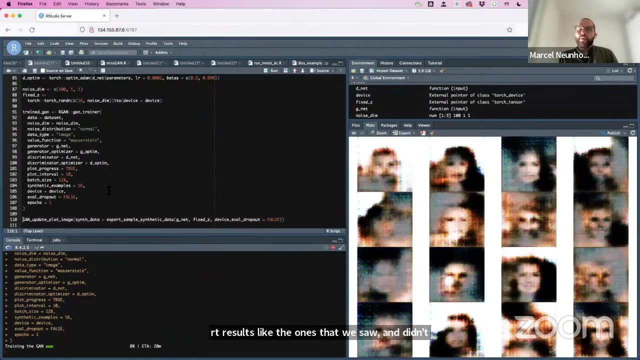 Like something sensible, like, in this case, producing faces when we want to produce faces. But you shouldn't expect to get like state of the art results like the ones that we saw in the intro, Like in the paper of StyleGaN 2, like those researchers at NVIDIA. they are very transparent. 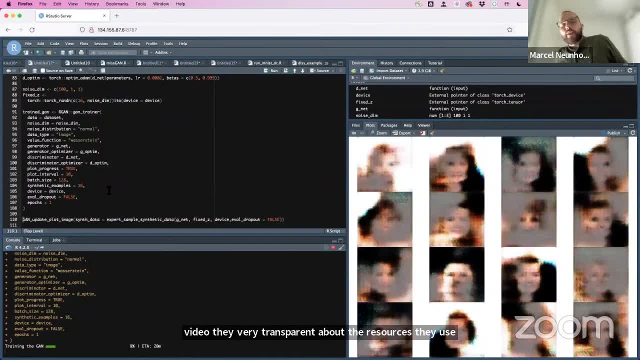 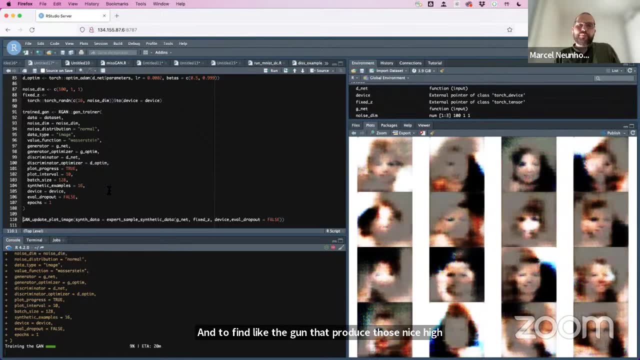 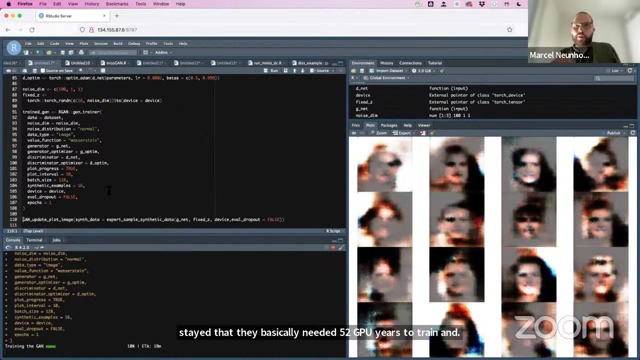 about the resources they used And to find, like the GaN that produces faces, Yeah, So when they produced those nice high definition, nice high definition pictures, they state that they basically needed 52 GPU years to train And as someone like me, like a junior researcher who has luckily access to one GPU, that would 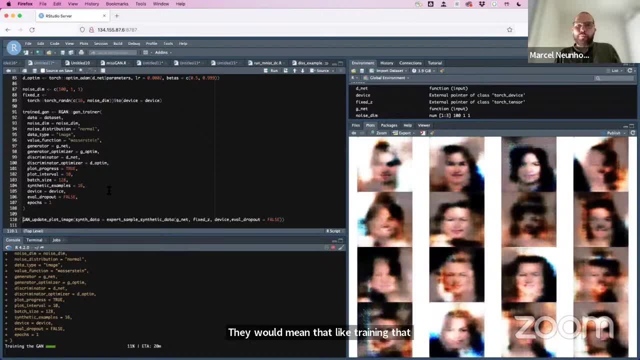 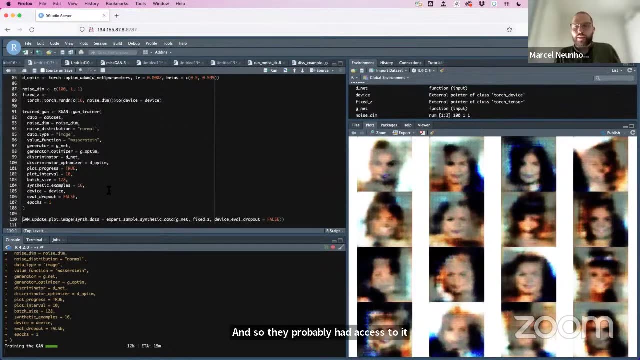 mean that, like training the same GaN would actually take 52 years, right? Like if I wouldn't spin up like some server with more GPUs, and so they probably had access to a hundred GPUs in parallel so they could do the same thing in half a year. 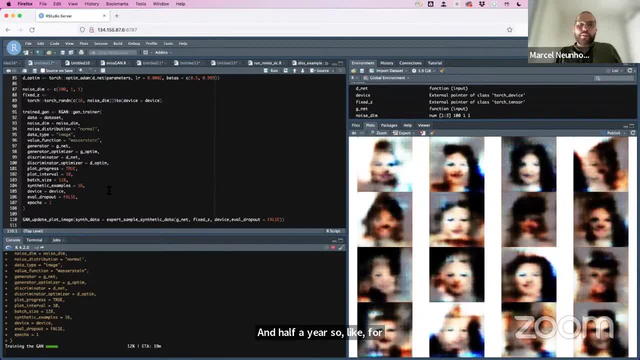 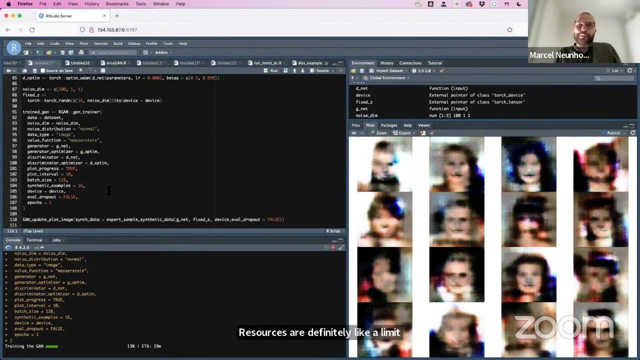 So, like for experimentation and getting to state-of-the-art images, in particular, resources are definitely important. Yeah, Like a limiting factor, And I would be happy to talk more about that, also the consequences of that, because it basically means that if you don't have the resources, you're locked out of doing like 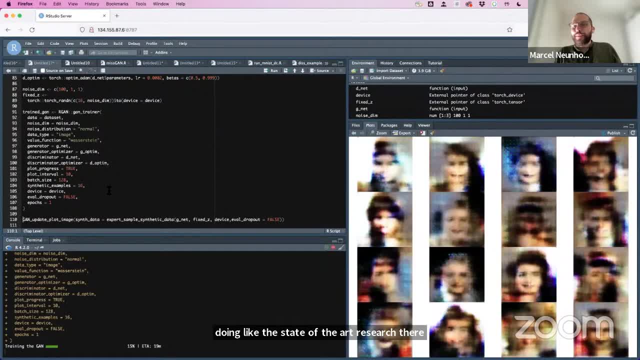 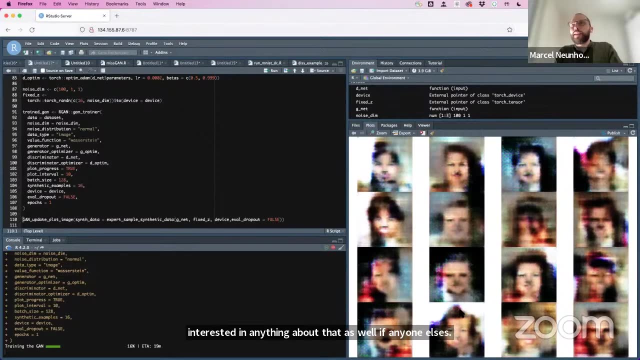 state-of-the-art research there. But let's pray for another time. But like I'm very interested in anything around that as well, if anyone else is All right. So now After training, like the first epoch for 15%, I hope now everyone agrees that we get to. 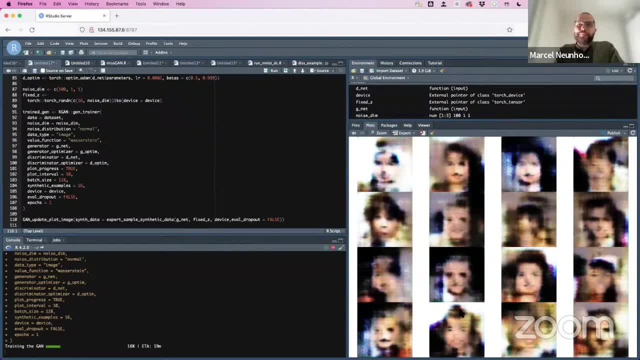 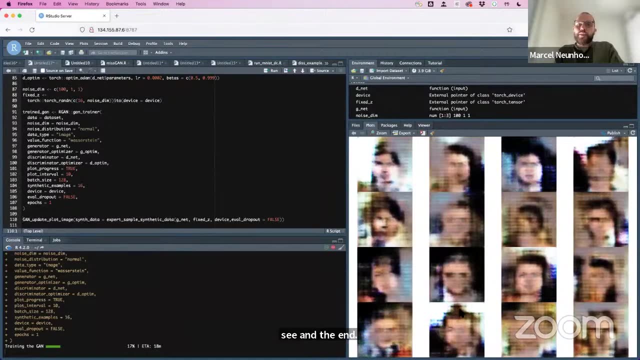 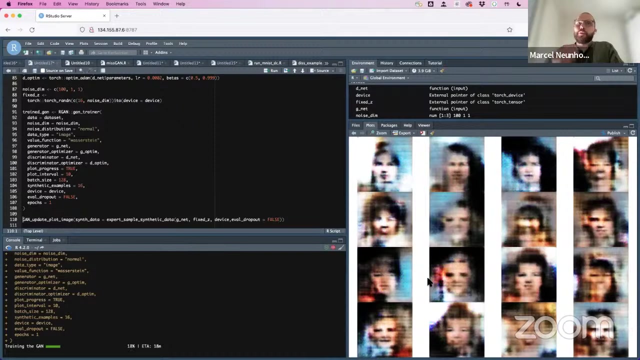 see faces And then like this, we'll just go on like that and you would see in the end, after one epoch, those pictures that I showed you in the beginning here, And then, If you would train it longer, they would get better and better. 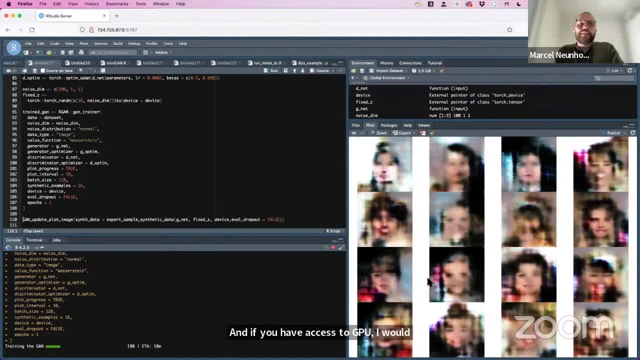 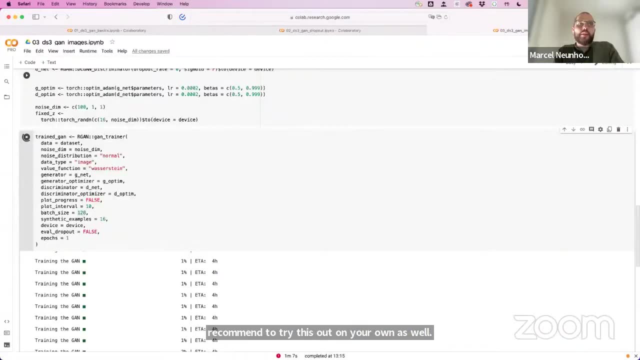 And if you have access to GPU, I would definitely recommend to try this out on your own as well. All right, So let's go back to our colab, where we, in the same time, didn't even like run longer. It didn't even train a few percent. 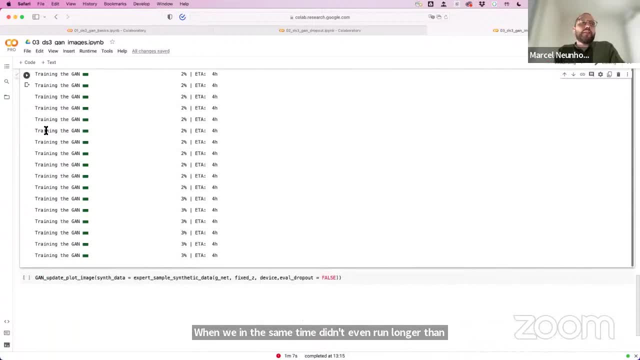 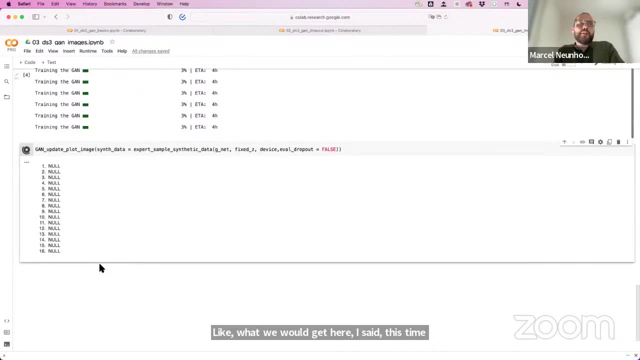 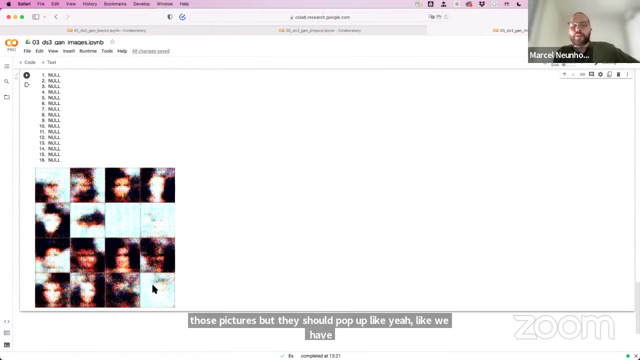 Yeah, But just to show you that, like what we would get here after this time. colab is a bit clunky when it comes to presenting those pictures, but they should pop up like: yeah, like we have seen a similar picture before. 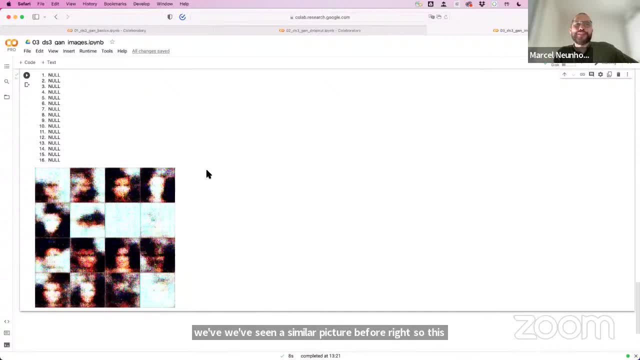 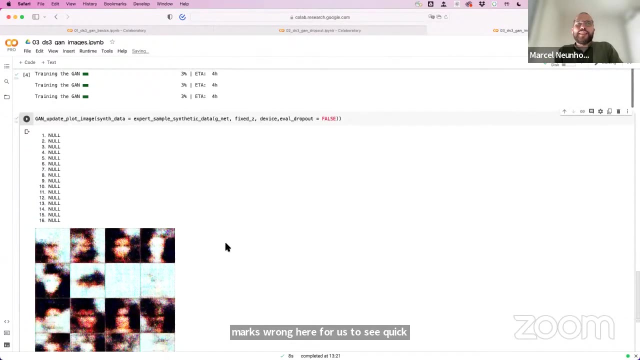 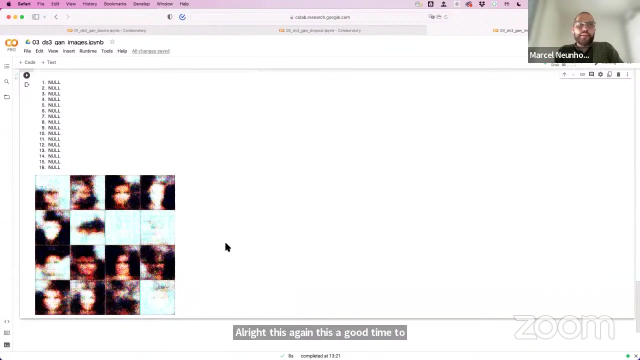 Right, So that's also. that's the right right thing, just as it, under quotation marks, wrong process are here for us to see quick results. All right, This again is a good time to ask questions And why we do that. 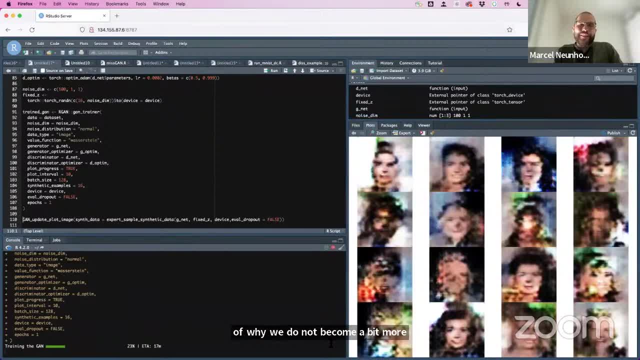 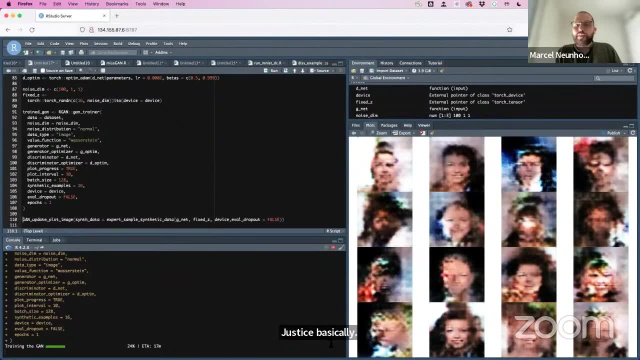 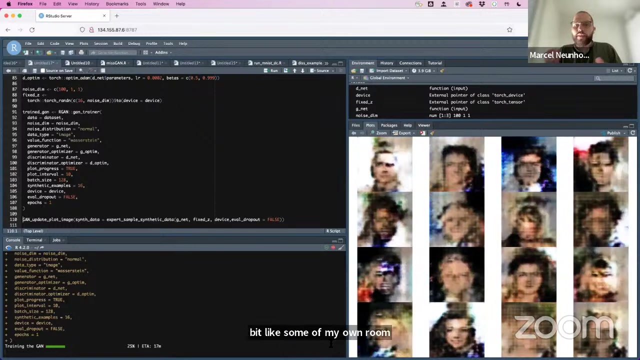 Because I'm not sure if training a bit more. because this basically Concludes the intro and coding part And I can the next section. I would like to show you a bit like some of my own research with guns and especially privacy preserving synthetic data. 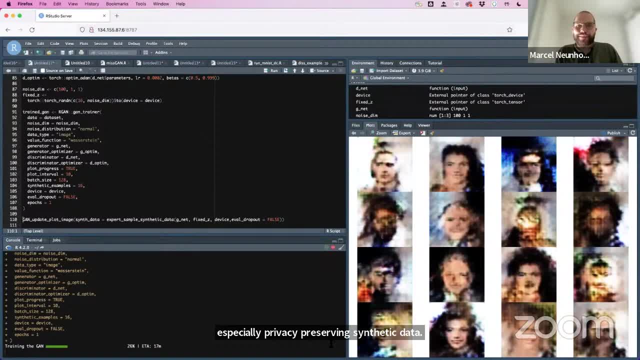 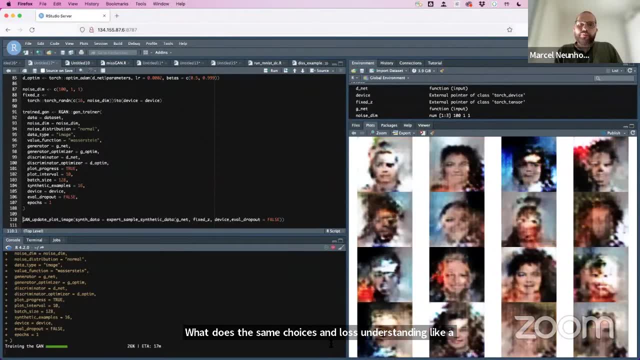 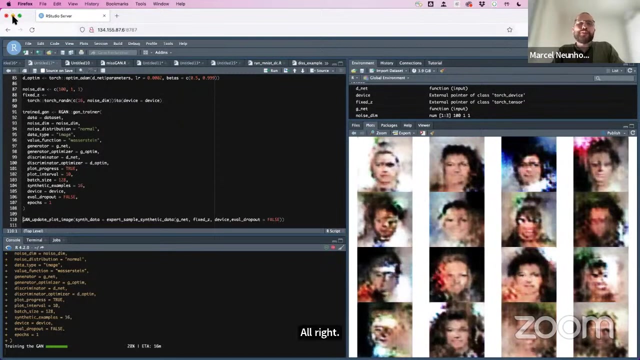 And how does That play into what we talked about with those design choices and also understanding like a basic gun? All right, If that's not the case, I'm sure questions will pop up. Feel free to ask them any time, And I'm also very happy to answer any any questions via email, like if something comes. 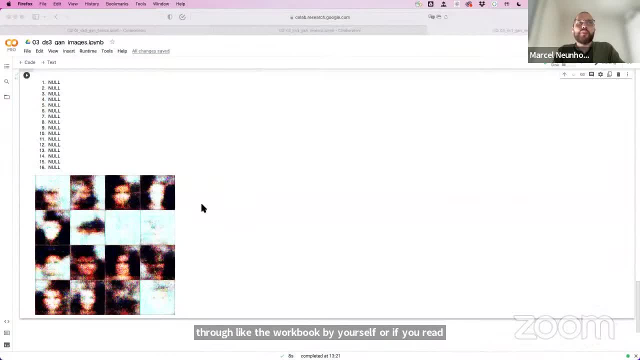 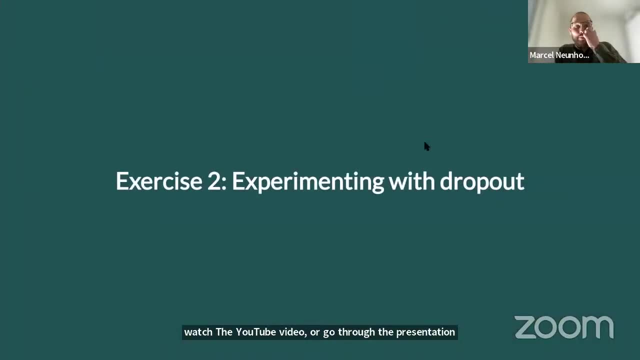 up when you work through, like the workbook by yourself, or if you rewatch the YouTube video or go through the presentation materials again. All right, We did like the experiment With dropout. Yeah, We did generate fake images, although like we're not quite there yet. 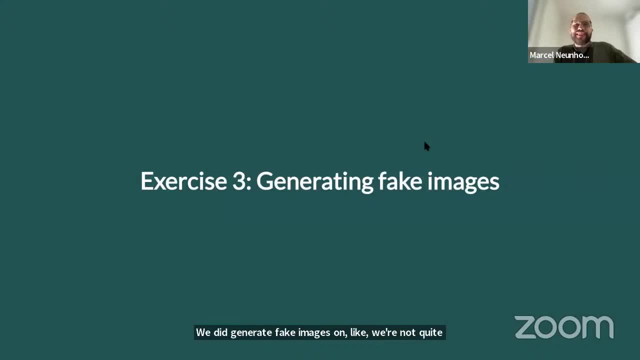 I can have another look like when, Like this next section is over And We can talk about those advanced topics that I teased at also in the intro for a bit now. So, basically, In one Research project that I Was participating in, like, our goal was to 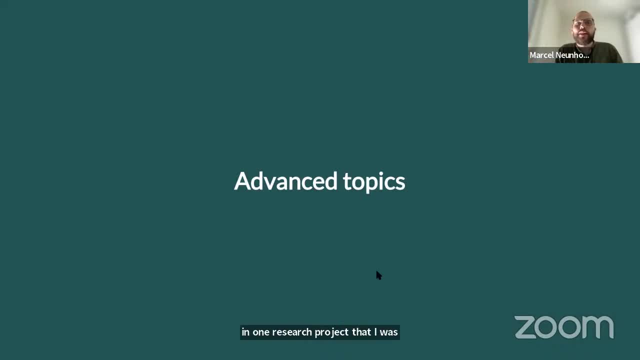 Generate my general purpose- Synthetic data for arbitrary tabular data sets That Preserves, Like The statistical Properties of the original data set as good as possible, whatever that means. This is also an open question, I think. I think 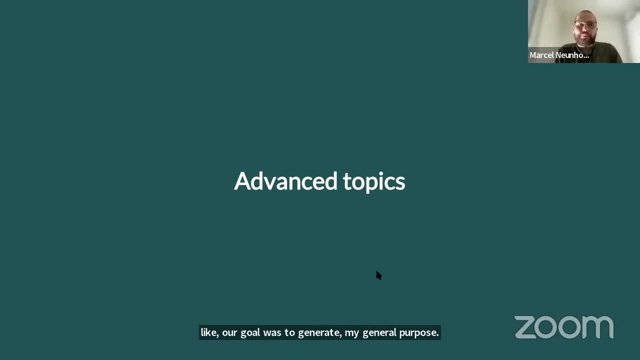 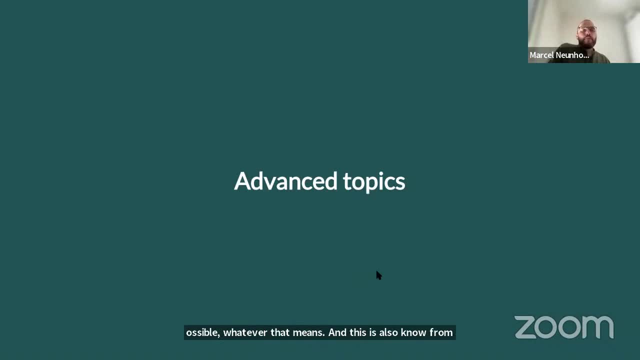 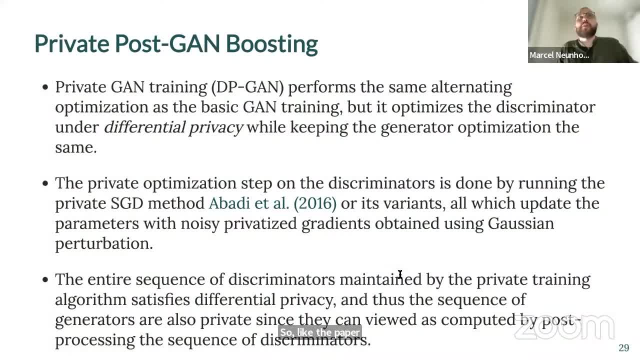 Those formal chefs can be proven. So like the, The paper or two, because it basically combines two ideas like private GAN training and also the post-processing of multiple GAN outputs. So in private GAN training and that's often abbreviated by DPGAN or like some other acronyms where DP is part of the name somewhere. 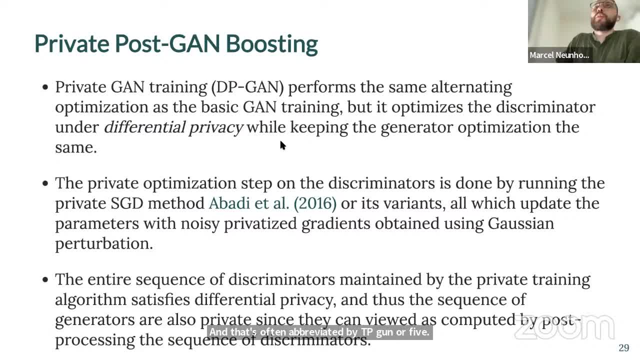 it basically performs the same alternating optimization as the basic GAN training that we looked at for the last three hours, But it optimizes the discriminator and the differential privacy while keeping the generator optimization the same. So why do we need to take care of the discriminator in the 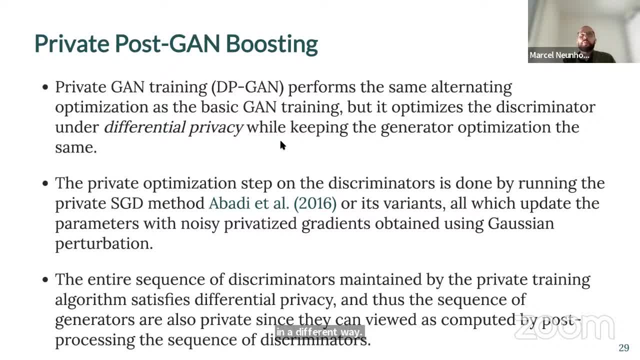 different way. If we want to have provable privacy guarantees- and one standard for that is differential privacy- we need to make sure that whenever we touch the original data, so our input training data set to randomize our algorithm that touches that data and randomize it in a way so that 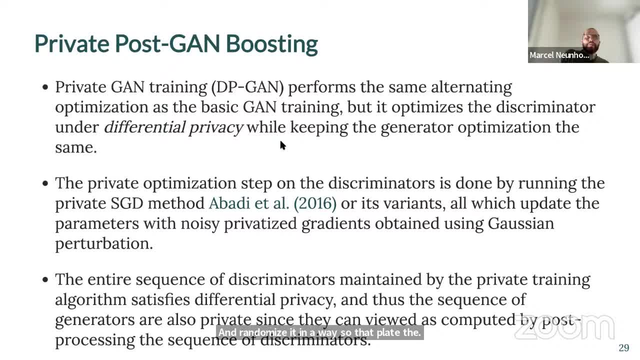 like the variance of that function basically is proportional to the privacy loss that we want to preserve. And where in a GAN do we actually touch the input data? That is only during updating the discriminator right, Like to update the generator. we just look at fake data and like at the feedback. 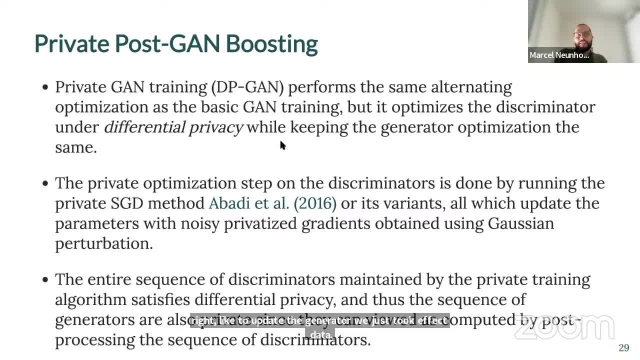 of the discriminator, of course. So indirectly we look at real data, but never directly. And during the discriminator training we actually look at real data. So if you think back to like the introductory example of like bandits and the police playing this game against each other. 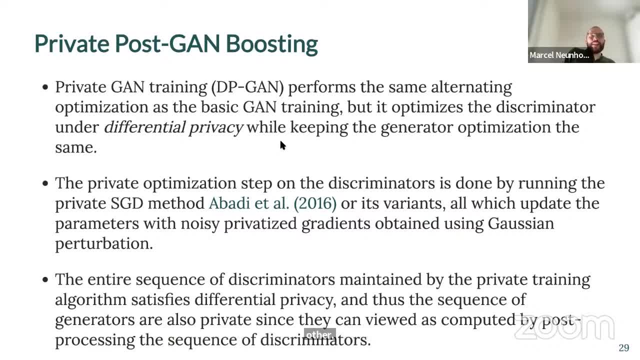 in this privacy-preserving training, training Afghans. we basically give the police like very, very strong eyeglasses that are not like what they need right, but that do the contrary, that they see worse than before, So that they can't actually look at the real money in high detail. 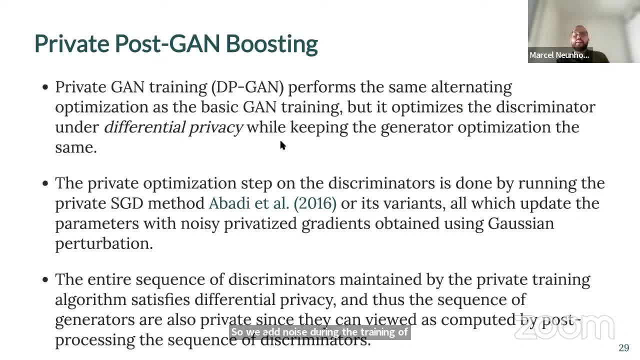 So we add noise during the training of the discriminator, so that we make sure that, like original training, data points cannot be leaked, or only with very small probability, Intuitively. this of course means that, like, the feedback that the police gives to the bandits is also noisier than before, which in turn also means that, like, we cannot achieve 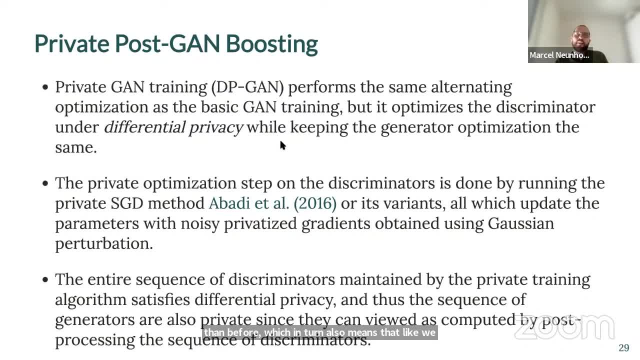 the same like utility or fidelity, quality of the synthetic data, because the feedback is just not as good. But this will achieve formal privacy guarantees And like. luckily there's a very cool method to like do private training for any machine learning model that uses some sort of stochastic gradient descent, and to keep track of like. 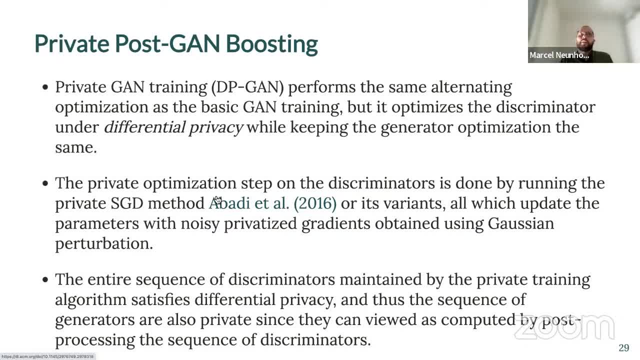 how much privacy budget one spent that was introduced by Aba. So, basically, to train a gun with privacy guarantees, the only thing we need to swap out is, like this optimizer for the discriminator And that's pretty cool, Like. that's like one very small change. 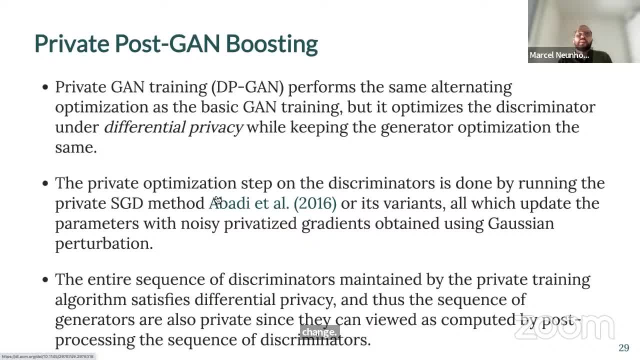 And then one problem, Okay, The problem is is that, like, reaching the equilibrium is very hard without noise during training of the discriminator and turns out to be even harder with noise right, Because the feedback is worse, and like we will maybe not even ever reach that equilibrium. 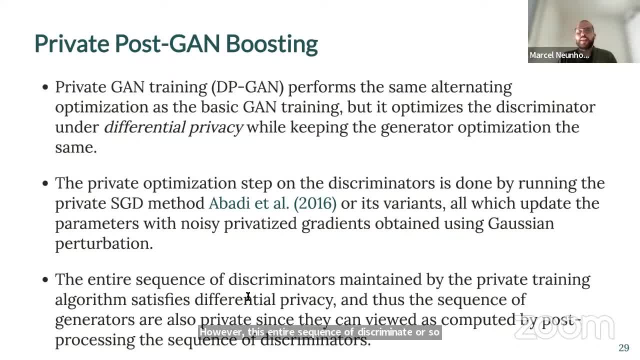 However, this entire sequence of discriminators that we can observe during training- right, Like each individual discriminator, like at each step we have a different, slightly different discriminator- is differentially private, And so the sequence of those generators is also private. And one cool property of differential privacy like this formal guarantee is that whenever 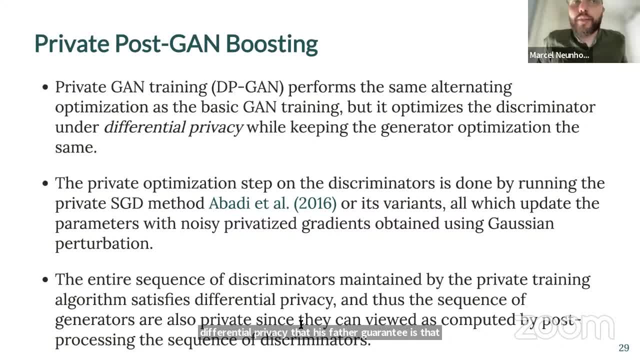 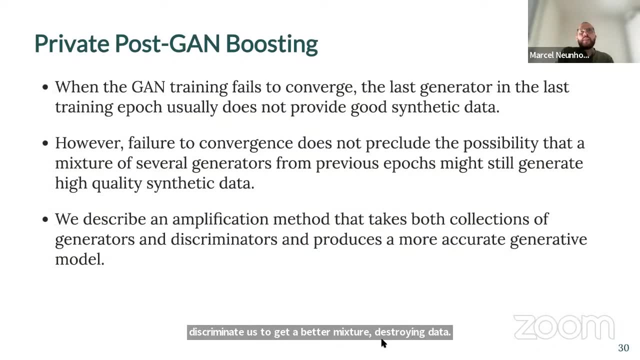 something is private, We can post-process as much as we want. So basically, we can post-process the sequence of discriminators to get a better mixture discriminator, And that's the goal here. So the issue is- and this will also be true for gun training without noise- is that when 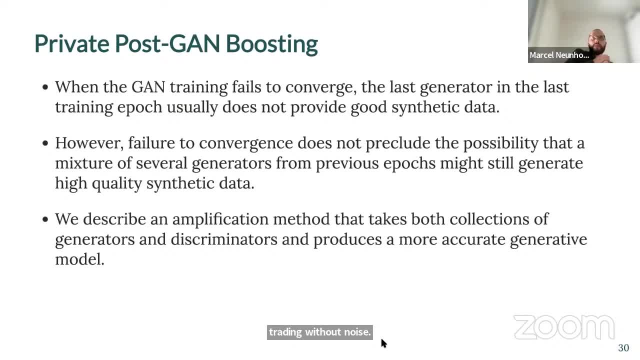 gun training fails to converge To the equilibrium. when it fails to find an equilibrium, the last generator, and that's what we use so far, to generate the synthetic data right, We just use the trained, the trained, fully trained, until this step, generator network. 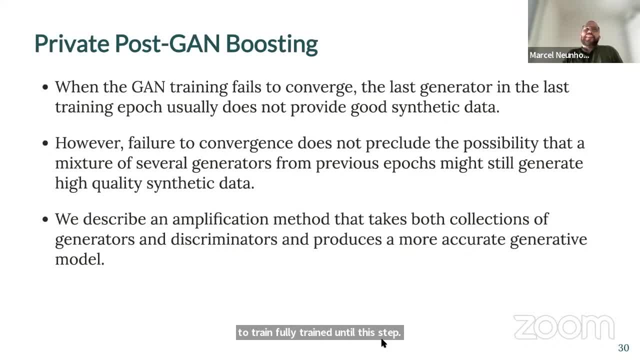 to generate data, But nothing guarantees us that the last is actually the best right, And We don't even know which one is the best. luckily, like the failure of convergence and the failure of the last generator does not mean that like a mixture of generators and 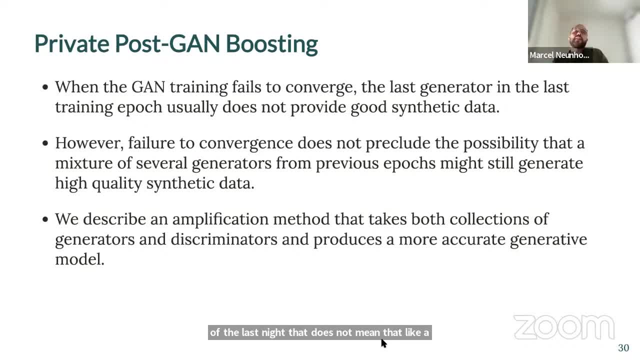 discriminators from the previous epochs can still generate like a high quality synthetic data, And so we basically came up with them, simple but very effective. So Okay, And where are we? Well, I think it's pretty simple. I think the first step is to come up with a more efficient method, right? 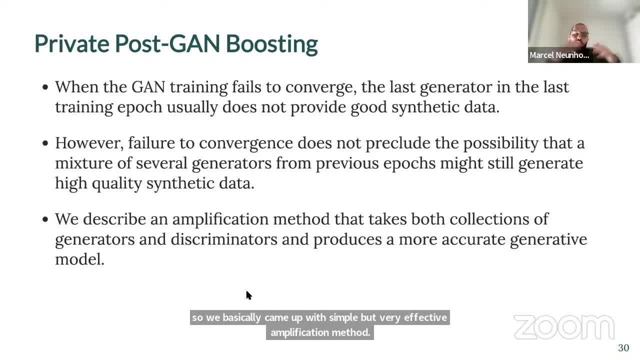 The second step is to come up with a more effective amplification method. that takes like a collection of generators and discriminators across All in parks, all update steps, So you need to store it. like those discriminators and generators make that's like a small overhead. 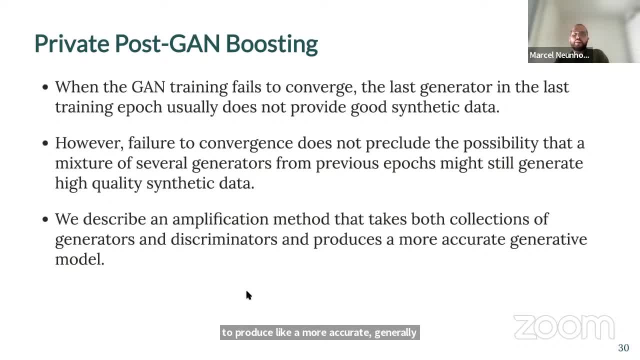 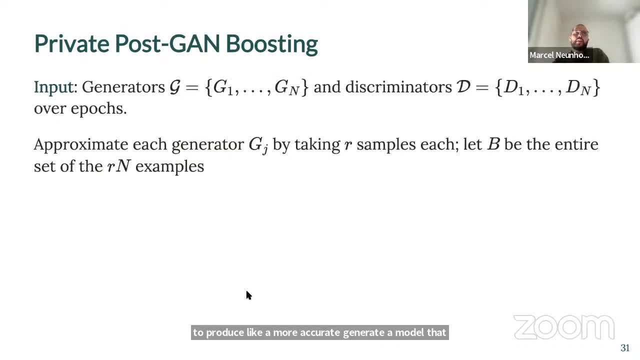 to produce like a more accurate generative model that takes into account like the whole sequence of generators and discriminating. So like this method takes us an input. So it doesn't really work on the GAN level, but like post-GAN right. 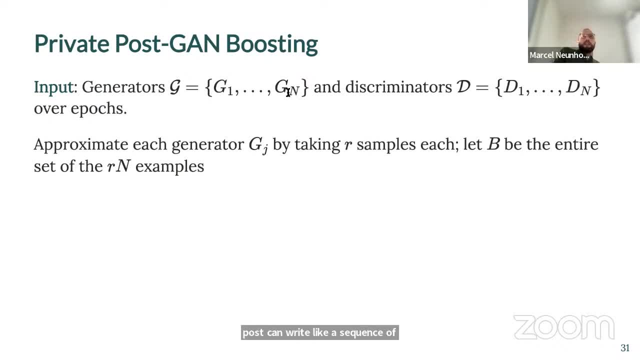 Like a sequence of generators from G1 to GN, like, and then can be like the last step. or it can also be like a different sequence, like where you only take like the 10th, every 10th or every 50th generator to save some space. 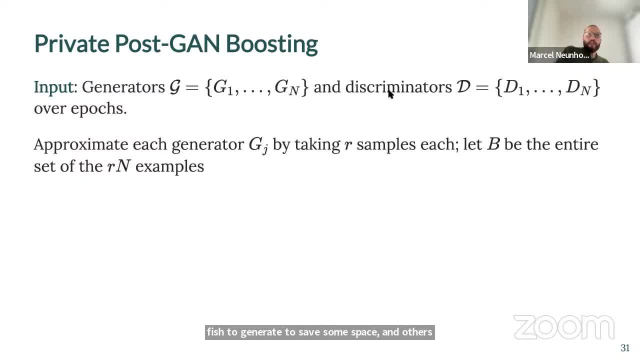 And a discriminator as well. I think those have to be the same, from the same epochs, And then we like each generator is actually like a generative model of the whole distribution that we try to model, but that's really hard to evaluate. 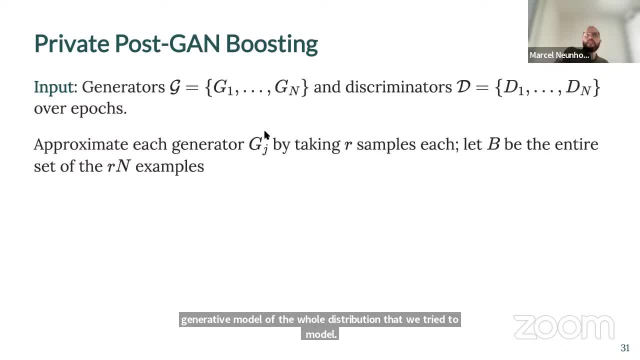 So one way to do this efficiently is to approximate each generator by taking some samples, like let's say a thousand, let's say a hundred thousand samples, And so we get like a number of B samples. that is R times N. So N is the number of generators here. 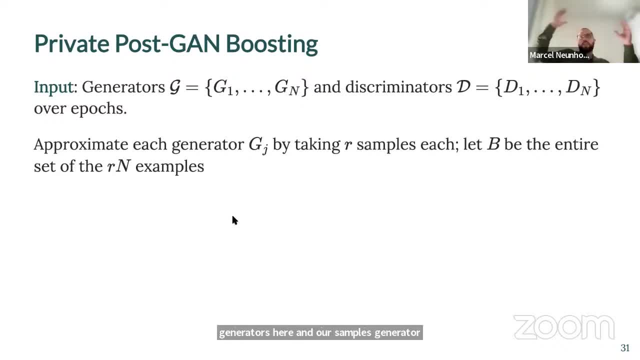 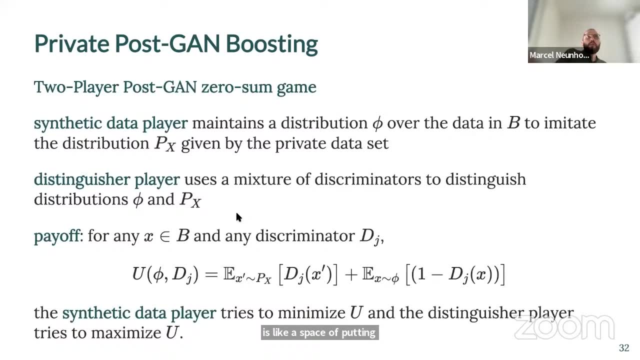 and R is the samples per generator samples. that is like a space of potential or good samples. And now we can continue like this zero sum game, adversarial game, like in the post-GAN where we have a two-generator world, where we again have two players. 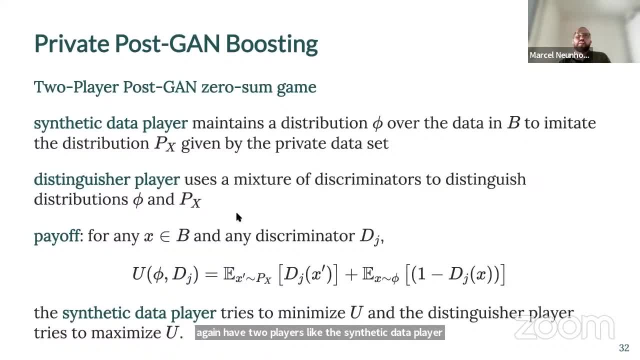 like the synthetic data player who has like a mixture distribution five over, like this whole collection of points that should approximate like the distribution of each generator, while B to imitate the distribution PX, and PX is our original data given by the private data set. 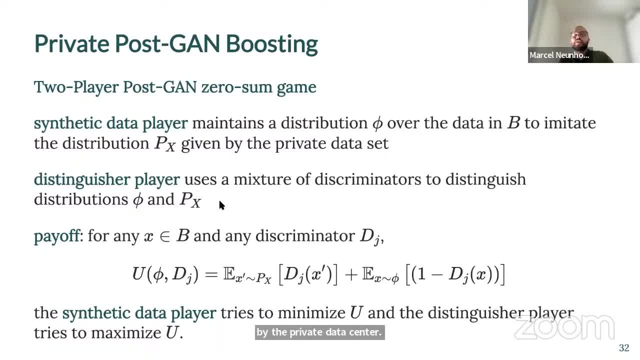 And the distinguisher player who uses a mixture of discriminators like that we also have stored to distinguish between, like this new mixture distribution and the original distribution. That means like here in this step, or rather here we have to access real data again. 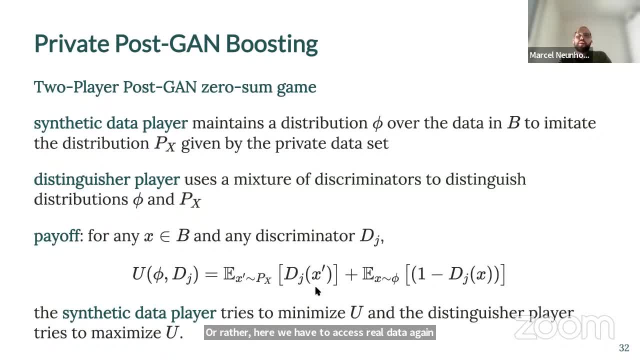 So we need to spend additional privacy budget here, but like that's not too much as compared to the training of the privacy preserving GAN actually. So we have like this utility function that like we want to minimize from the perspective of the synthetic data to the data player and to maximize 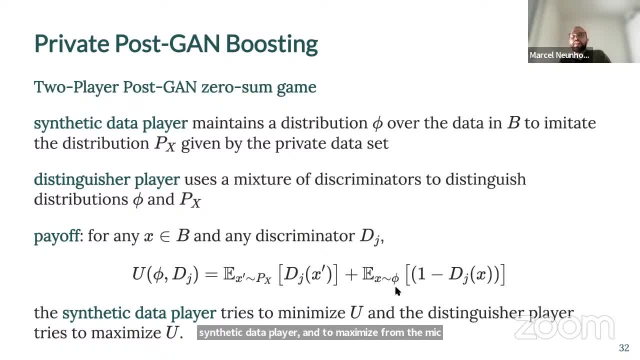 from the like perspective of the distinguisher player. And that's pretty much the same as, like, the original GAN function. right, And now we can use the multiplicative weights update rule, which is a nice algorithm, Like if you haven't heard of it. 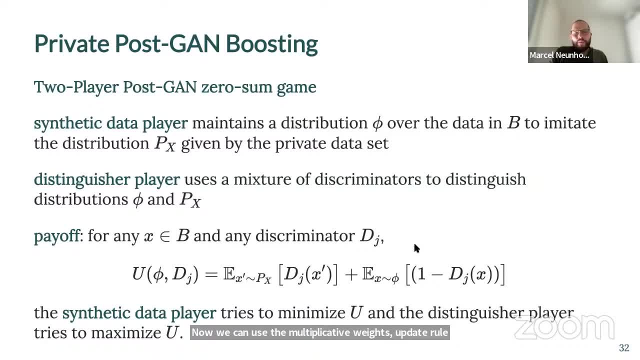 like. I would encourage everyone to read up on it. It's a very basic, cool algorithm for solving zero sum gains, very useful in lots of situations, and machine learning to like find an equilibrium here and find a good mixture distribution over all of those sample points. 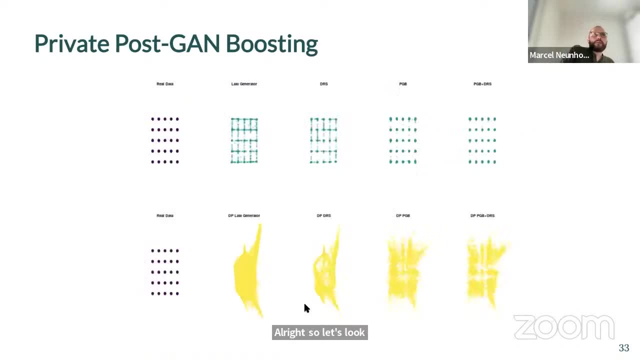 All right, so let's look at some results here. So here, like, the input, data is still just two-dimensional, but a bit harder than like, the parabola that we looked at. It is a mixture of 25 bivariate normal distributions. 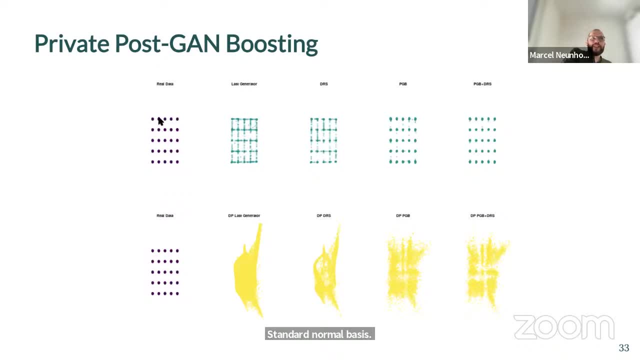 and standard novel basically rescaled for each center And that's the real data distribution that we tried to get at. So we just changed the vanishing point of the vanishing point. So that was all the information about if you get the word. 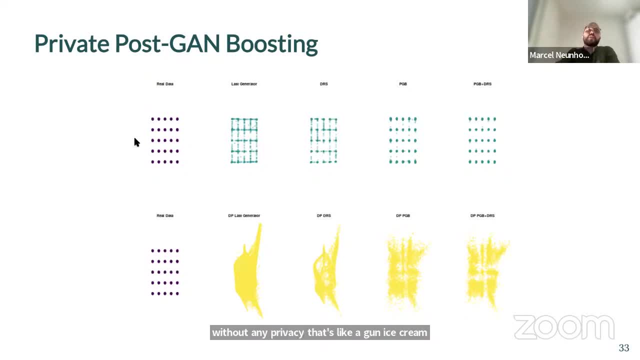 it's just going to be triple-digit. And now let's look at the difference between the two distributed GANs, like the one with the no one factor binary team that we're actually trying to figure out. So let's do that. So let's say, if we now would just 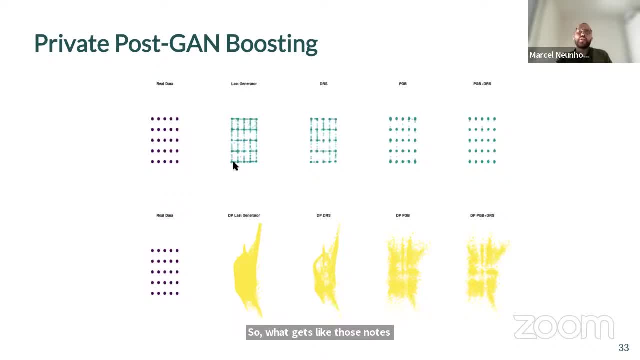 and like the first row here is without any privacy. That's like a GAN as we trained it before is due to like the noise distribution. So here, like if we would use a different noise distribution, that would have like a similar structure. 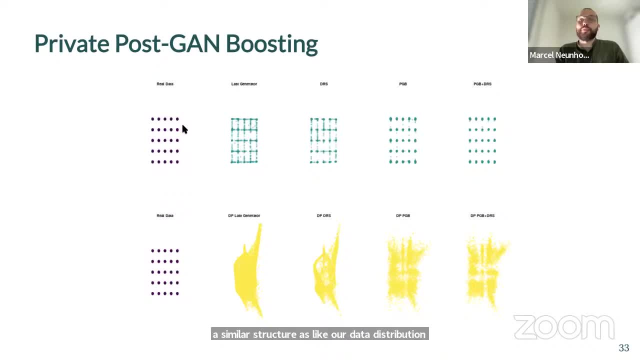 as like our true data distribution. this would also go a long way and help us to get rid of like those points in between here. But the noise distribution here is also just like a standard normal, So pretty much similar setup to what we looked at before. 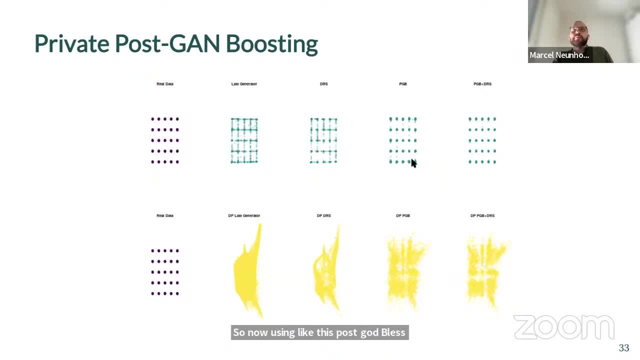 So now using like this post-GaN boosting method basically generates like a better mixture distribution that gets rid of like those weird points that shouldn't be there, because we use like this information, like we have like a bigger distribution to choose from and we use the information that is stored. 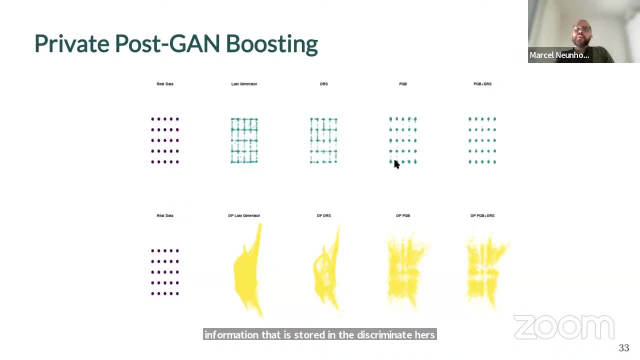 in the discriminators so that we can sample, like from a better generative model. And this can then even be combined with like another method that's called discriminator rejection sampling that uses a similar idea but without accessing training data again to improve those, So we can see those results even further. 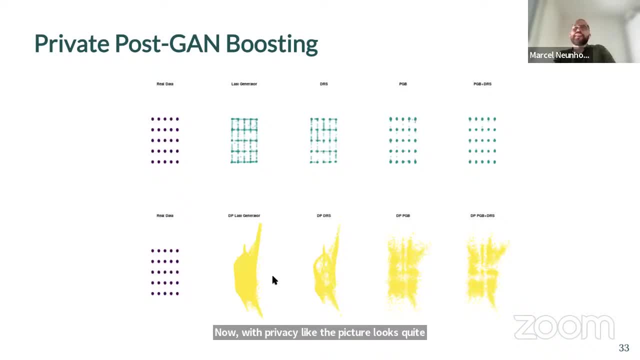 Now with privacy, like the picture looks quite different and like the last generator doesn't look, or hardly looks, like this grid or like those dots that we want to recover, And this is of course because, like we have like those glasses on that make it really really hard. 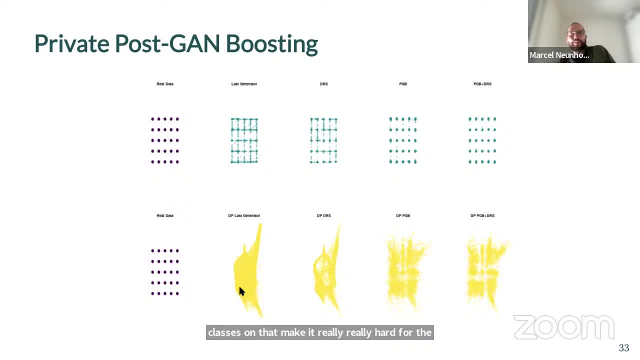 for the police to see, like to tell, to give useful feedback And with this post-gun boosting method, however, we can see that, like this, demand is recovered better, right, Like we can see the grid structure and like the demand is covered better, 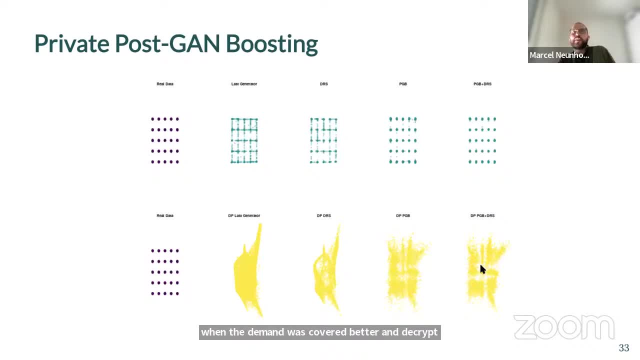 and the grid structure emerges And in the combination with, like this, DRS method, this also improves it a bit further, like by narrowing down a bit more, like those points like this center is preserved pretty well. Such toy examples are interesting, but like really useful right. 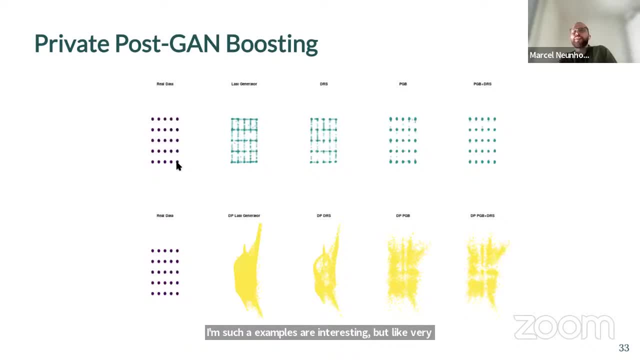 Like when would we ever want to sample from something like this? And like what would we do with data after we synthesized it? So what we also did is- and like there was a question to that before- like we ran some regression models and machine learning models, typical downstream tasks. 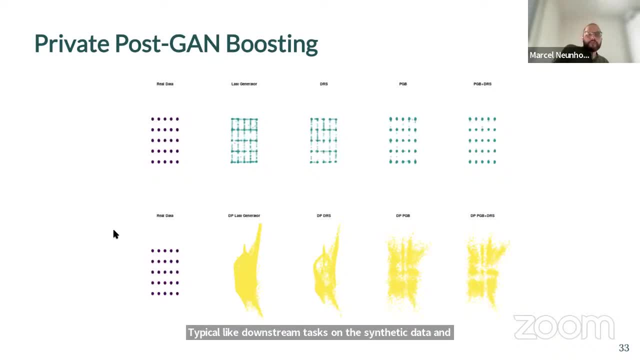 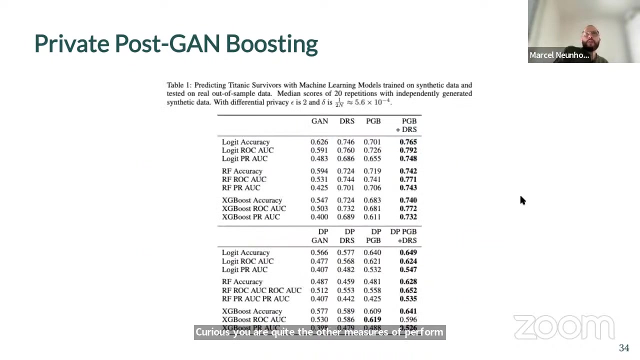 on the synthetic data And compared whether this improved, like this method improves, like this downstream task accuracy or like other measures of like performance for machine learning models. So, for example, we use the well-known Titanic survivor data set. I guess everyone who has ever been on Kaggle 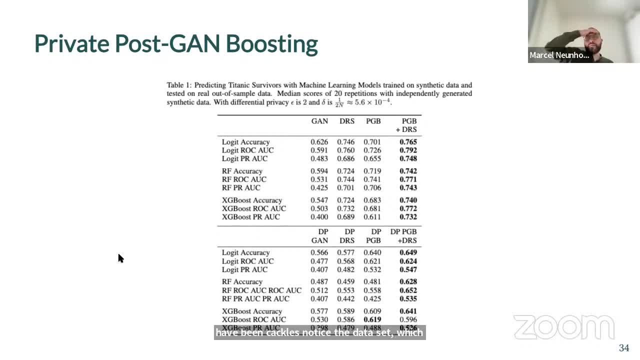 knows this data set which has just like a bunch of like variables on each like passenger on the Titanic and whether they survived or not, And like the prediction task is to predict whether someone survived or not And the first set of results here shows that. 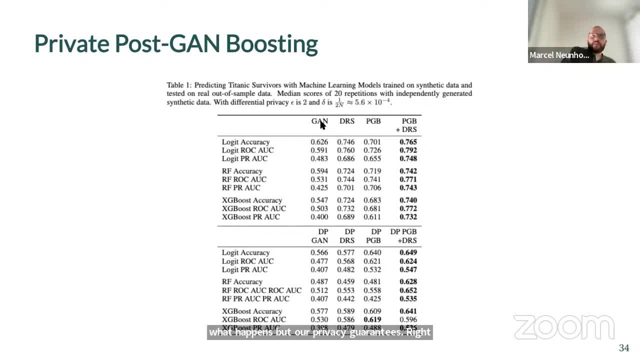 what happens without privacy guarantees? like we generate synthetic data, the model with a gun, then with those different post-processing methods and then train classifier on the synthetic data and tested on real out of sample data So that it was not part of the synthesization. 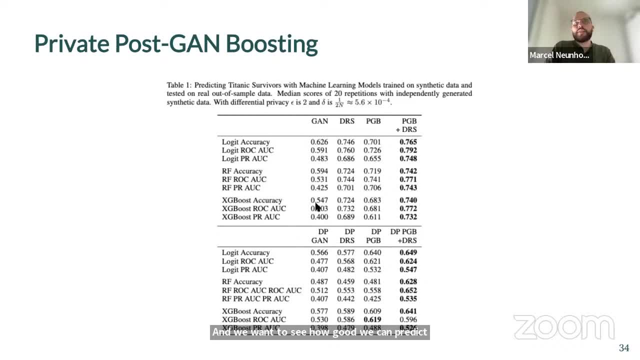 and we want to see how good we can like predict real Titanic survivorship based on those synthetic data example. And it turns out that there's not much extreme Armor data. turns out that this combination of post-scan boosting and DRS outperforms all other synthetic data sets by a lot. 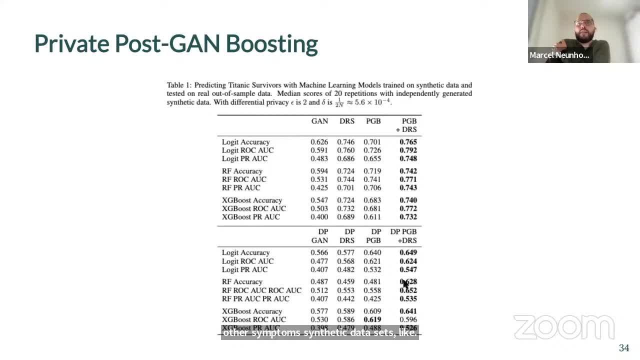 and even more so with privacy. And of course- again this is expected- The accuracy drops from the non-private synthetic data to the private data, since we again have the police, the discriminator, who only can give noisy feedback. All right, so that was a bit like the quick run through. 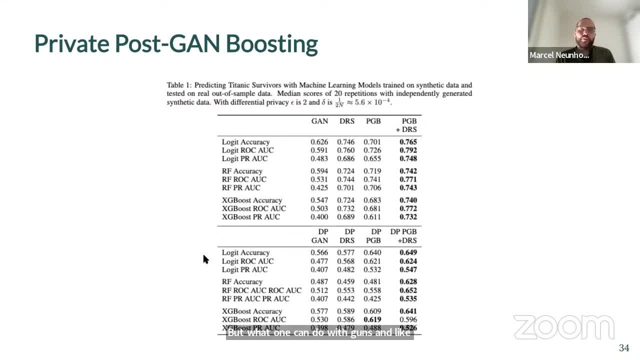 What, What, What, What One can do with guns and how they could be useful for classical data science, slash social science. And, to be honest, I was a bit quicker- maybe too quick- than I anticipated for this part, So we have plenty of time for Q&A. 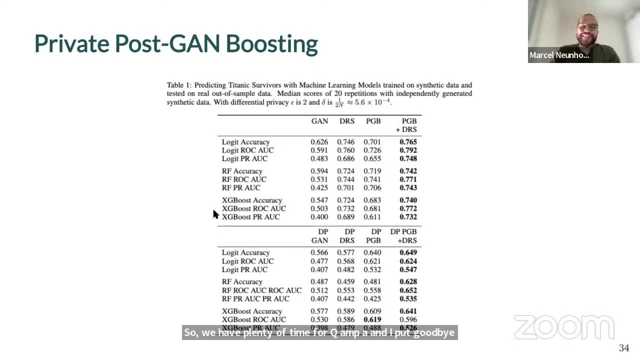 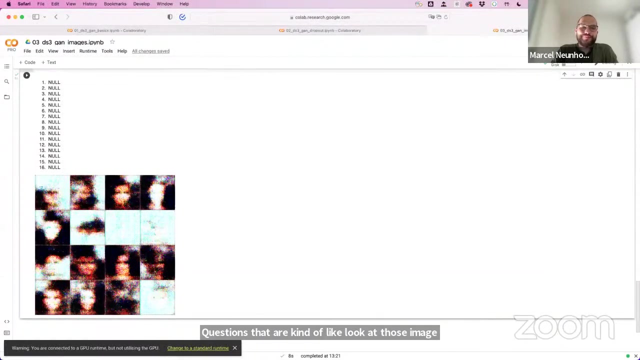 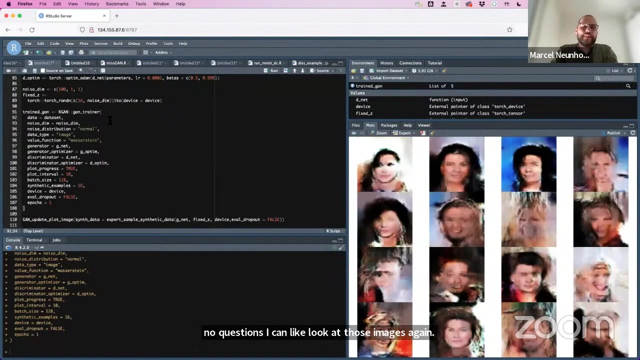 and I would be very happy to go through anything again that was too quick or that needs a bit more elaboration. If there's no questions, I can look at those images again. And there's one more question in the chat? OK, Yeah. 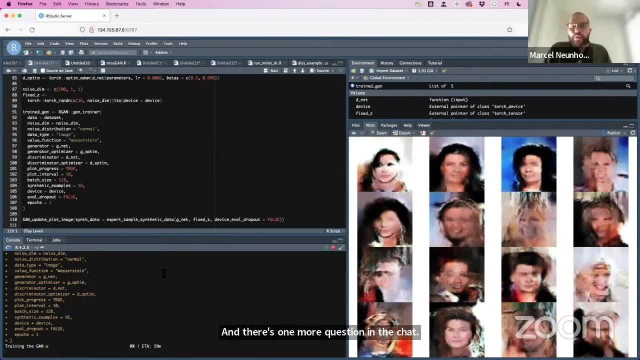 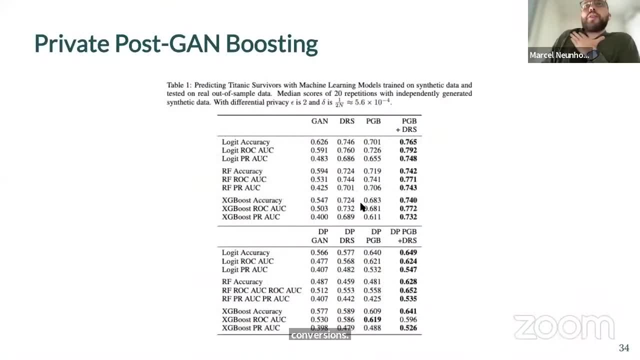 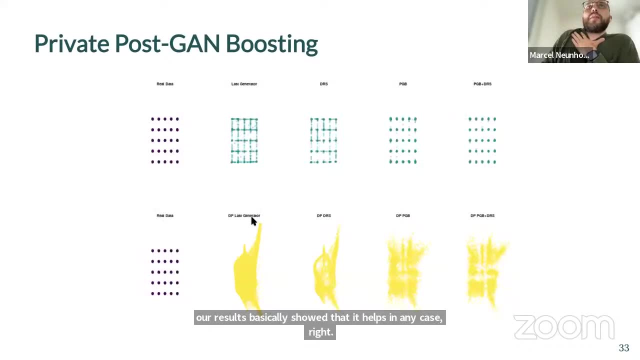 Yeah, Would you use the post-processing in any case or only if there is no convergence, Like? our results basically show that it helps in any case, right? Or like in the theoretical case of perfect convergence, you would probably not need it and it would probably not. 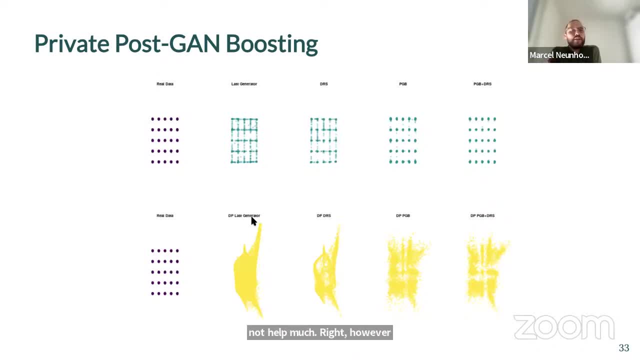 help much right. However, empirically, even without privacy and even training, a very good gun for the task. typically it doesn't get you close to convergence in finite time and you stop training at some point. And the cool thing really is that even then, 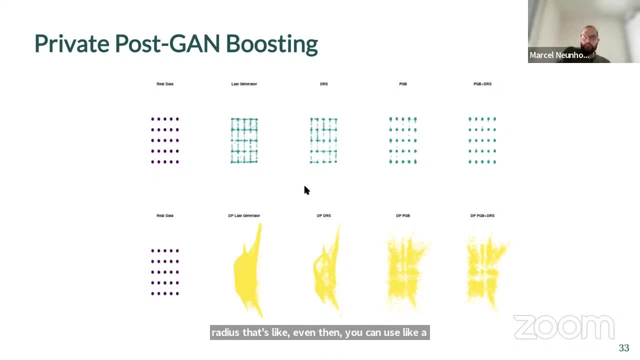 you can use the sequence of generators and discriminators to Yeah, Yeah, Come up with a better generative model, And in the case of non-private training, there's hardly any additional overhead to do that. The only thing really is that you 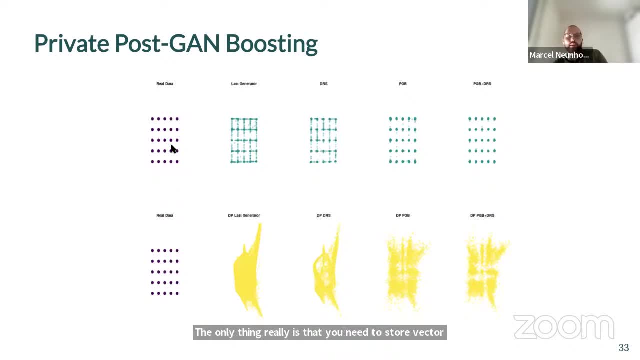 need to store the networks after each update step or after each update step that you want to use in the generation of the bigger model in the end. So that will take away some disk space but it won't necessarily slow training down or anything. 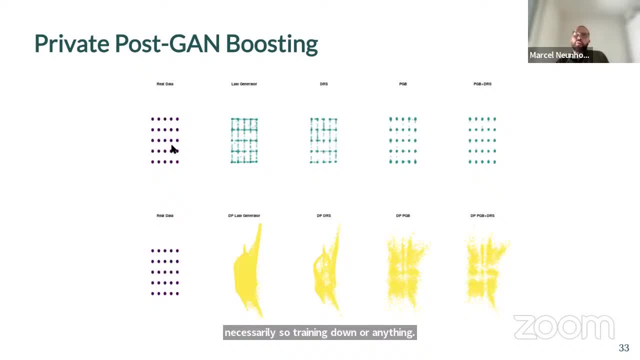 And then you just use that to run those multiplicative weight updates steps and come up with a nice generative distribution. OK, Yeah, That's a good question. In those examples we didn't use any dropout. It was pre-my dropout curiosity. 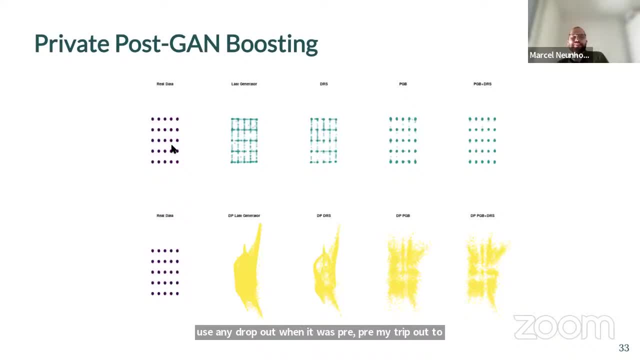 So that's the standard GAN set up. I just read the question again so that everyone who can't read it can also know what it's about. Might this not increase the risk of overfitting And this meaning like this post-GAN boosting method given? 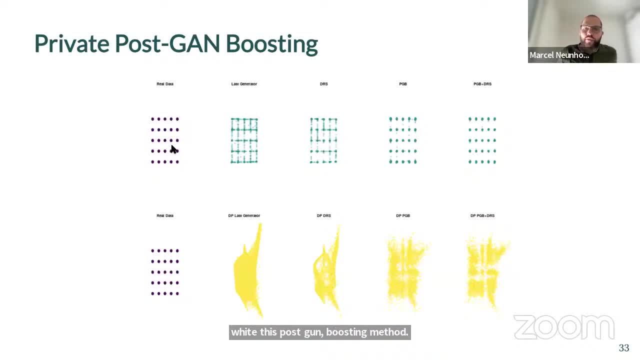 that we intentionally use it. We use the dropout to increase variance but then sort of average it out again in post-processing. So very good question. I have no idea. Yes, But intuitively yes, It would increase the risk of overfitting again. 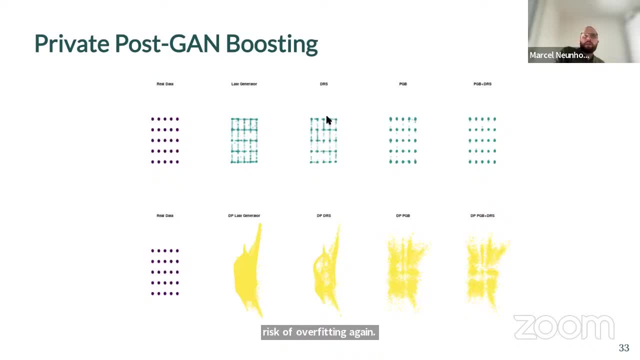 However, as we need to access the real data with the discriminator again here and also the generator, we probably should use dropout there as well, And then we should get a good mixture model that also gets the variance right. But I definitely have to try this out. 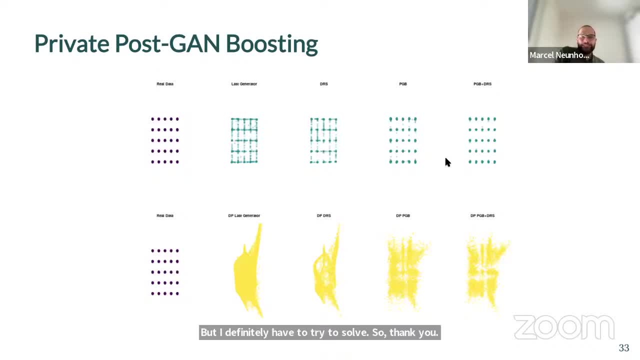 So thank you for the question. I have no idea. I have not done it And it's, by the way, is also a general and more interesting philosophical or procedural question in computer science, I think. But you know often the goal of synthetic data generation. 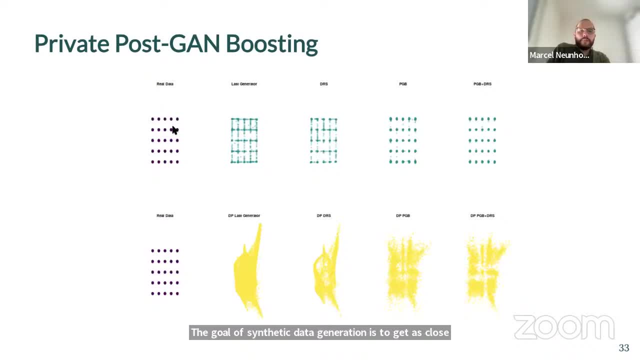 is to get as close as possible to the real data, So, in a way like even over fit to the real data sample that we had at hand. However, from a statistical perspective, that might not be the ideal goal, Like if we think that, like this is only a sample. 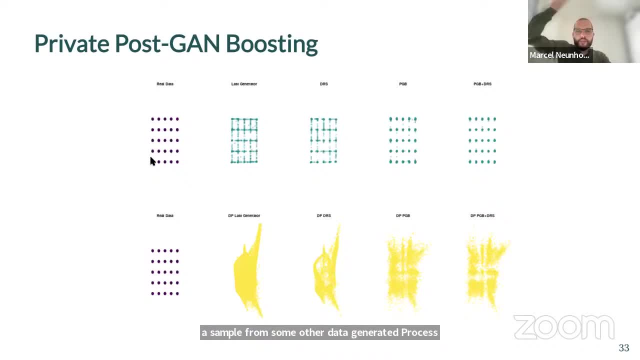 from some other data generating process and we want to make inferences about the other data generating process, then we would expect even more noise And like this would definitely be over fitting to the real data and probably not too helpful to make inference about, like the population. 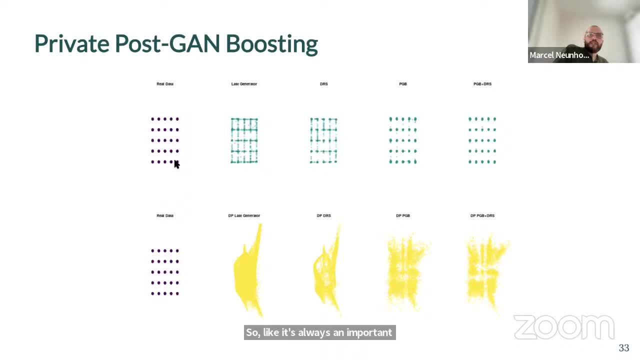 So, like it's always an important question, Like if you, using synthetic data, want to make inferences about, like the sample that you had at hand, then you want to be as close as possible, or do you want to make inferences about, like the population? 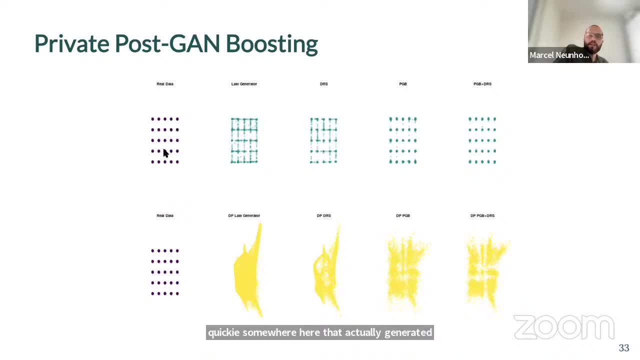 like that could be somewhere here that actually generated the sample at hand, And then you would want more variants to account like, especially to account for, like the sensitization uncertainty as well. So you can't just go into the data like, try to find like the most accurate. 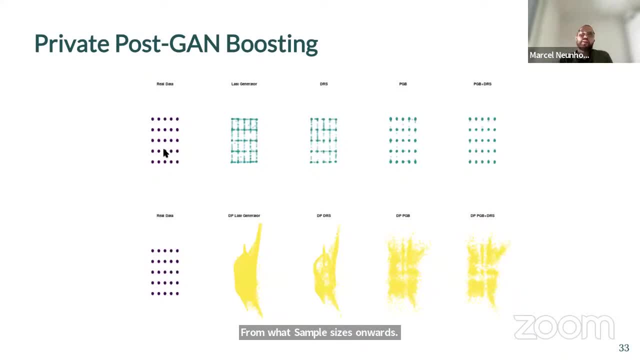 the most accurate, the most accurate data in the world. So that's, that's pretty much what we're trying to do, But it's, it's, it's, it's a, it's a. it's a really challenging question. 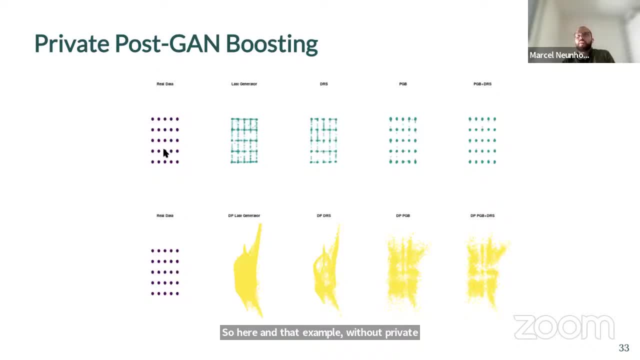 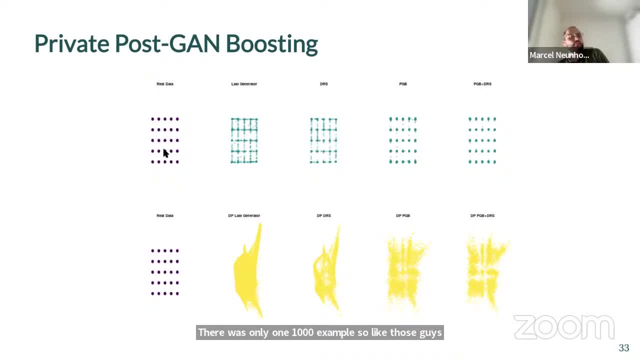 So like, uh, those guns work also pretty well with, like smaller samples, but of course, like, the more examples that actually sees from the distribution that you care about, like, the better it gets. and, um, like, if it's high dimensional distributions, like images, um, you would need more. 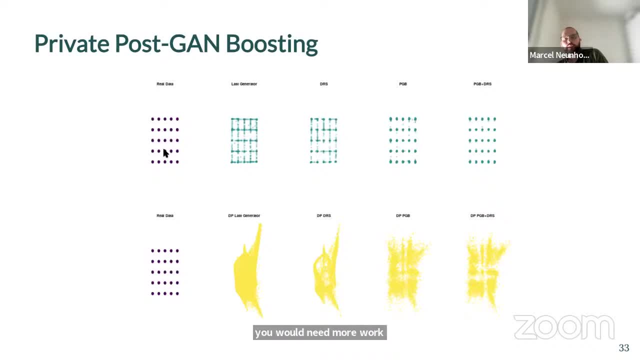 like more uh than than a thousand. Otherwise, um uh, this might not learn anything useful. So the the Celeb A with like I guess 40,000 images is like a good size there, Um, but of course it's it's harder um to collect and curate such such. 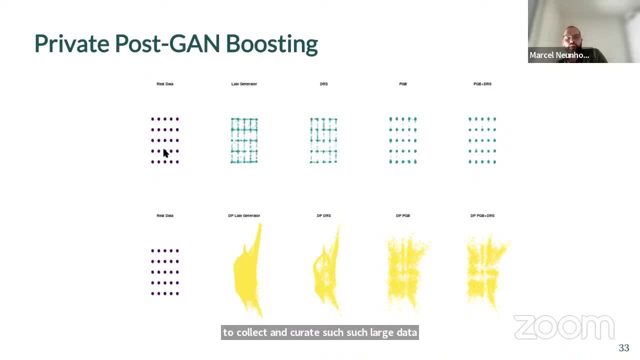 large um data sets of of images. So one of the, the, the, the main thing that we did is that we actually took a lot of images from the, from the, from the improvements that we made of our our the, the knowledge that we had got from the from the 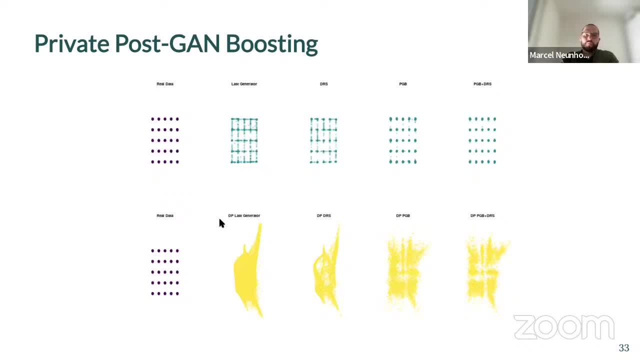 existing uh use of the information and the uh, the, the data set, um. and then we had a little talk with the, the, the uh, the, the uh the computer team, but there wasn't much that we thought we could do uh. 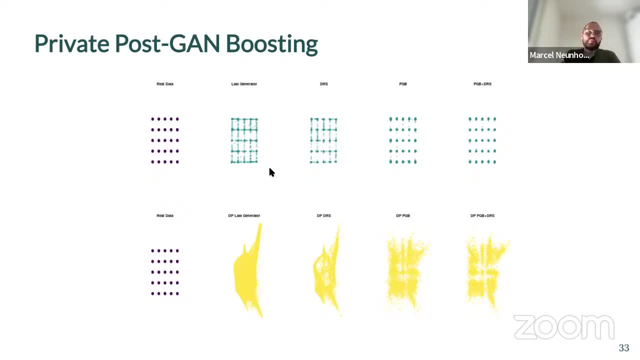 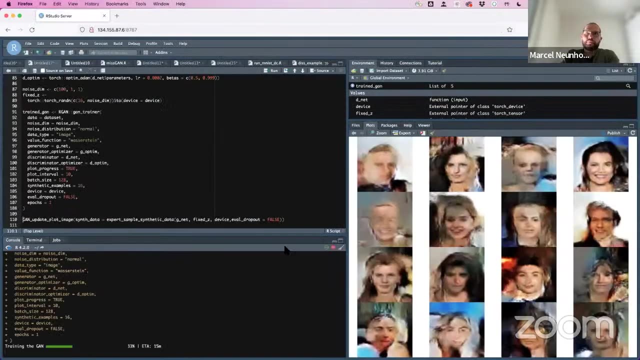 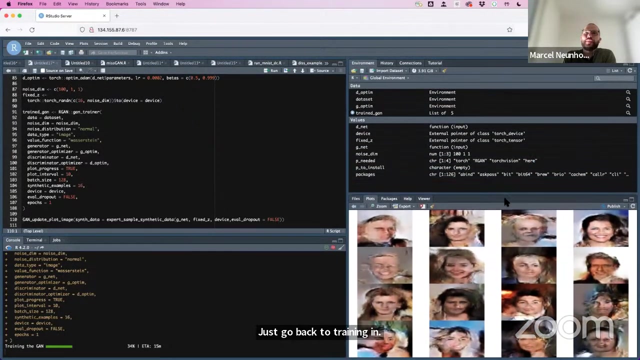 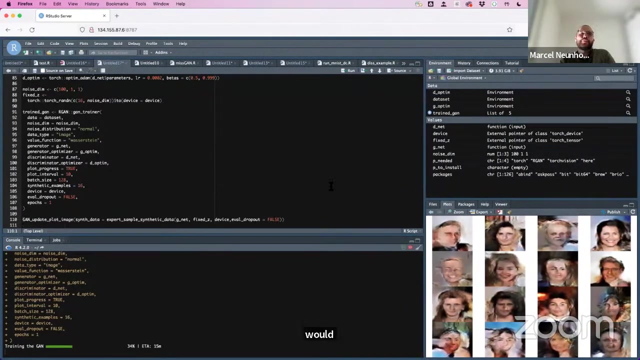 Just go back to training, and that's always the most fun part of like if we go smaller, that it actually gets closer to those 64 by 64 pixels. They're not too bad, like I would say. Look a bit like paintings maybe, But that's always the fun part, like of. 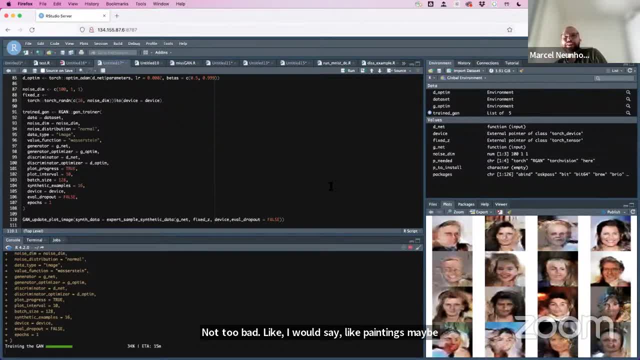 to be honest, of training generative adversarial networks, to wait and see if it works- And often it doesn't. And then it's also annoying, but sometimes it's as exciting as waiting for the next episode of your favorite series on TV. 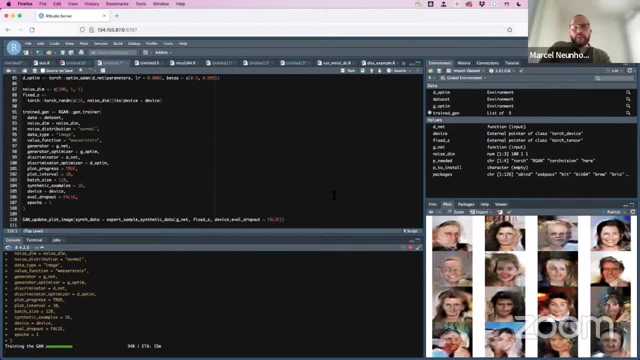 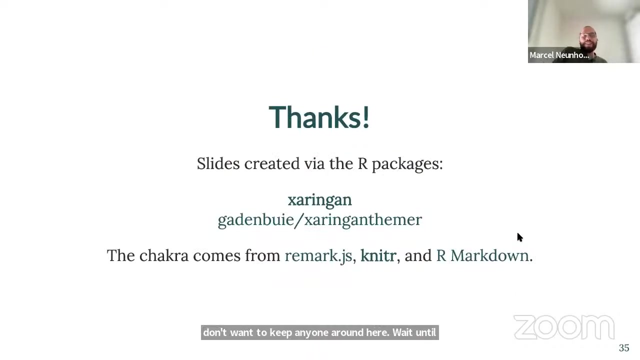 All right if there are no further questions. I don't want to keep anyone around here and wait until something exciting happens, So like thank you. Thank you very much for your attention And the excellent questions And it was a lot of fun And I hope it was a lot of fun for you too. 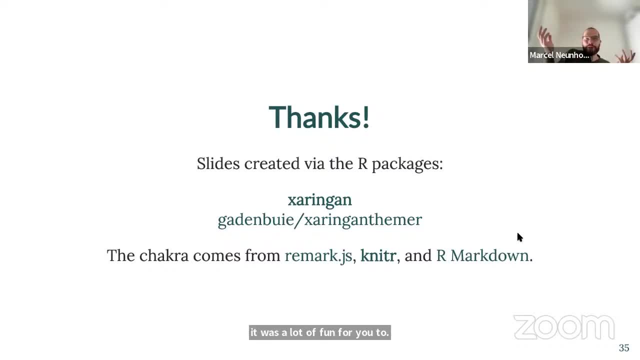 And I guess I will just hang around in the Zoom room for like a couple of minutes if any questions pop up. But on the GitHub page for this course you will also find my email address. if anything comes up, I'd be happy to read from you and 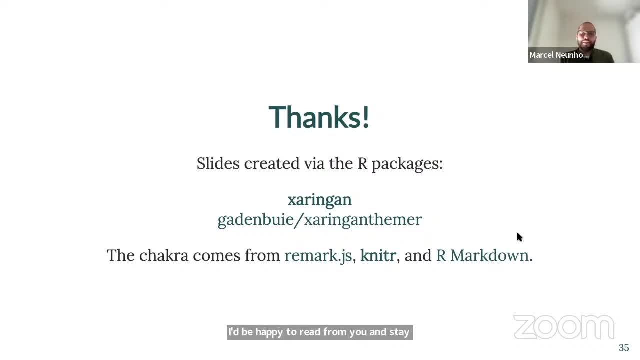 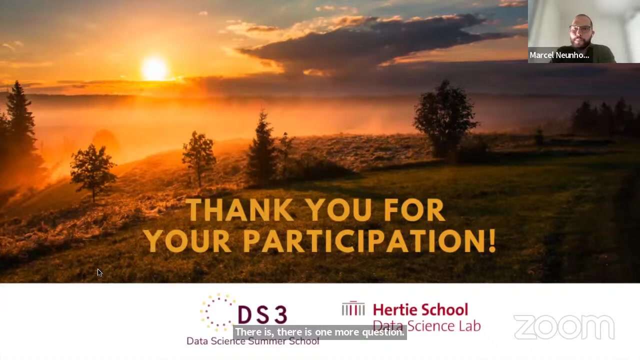 stay in touch with you. if you have cool ideas what to do with GANs, I would be very interested to hear about them. So thank you and, like, have a great Wednesday and a great like last couple of days after summer school. There is one more question in the chat. Would it make sense to pre-process the pictures? 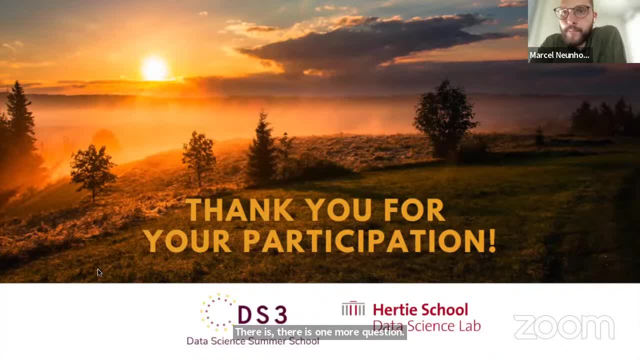 For example, align the faces and remove the background and train more. Yes, And like we kind of did that with the CELAB-A data set as well, right, We cropped them to the center, So like, in a way, to hope that we get the. 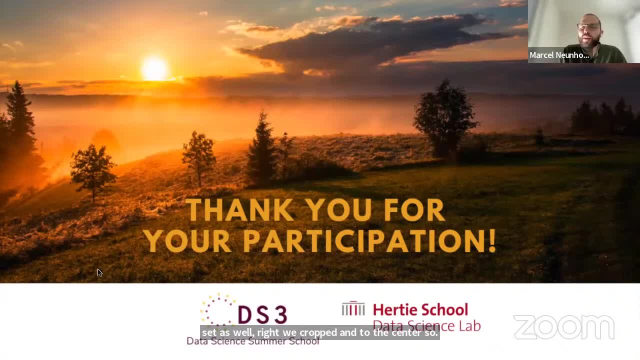 faces, Because, of course, like, the more similar the training images, the easier for the GANs to learn Like if you have, like, a very diverse set of images like, let's say, I don't know, landscape, animals, cars and faces. 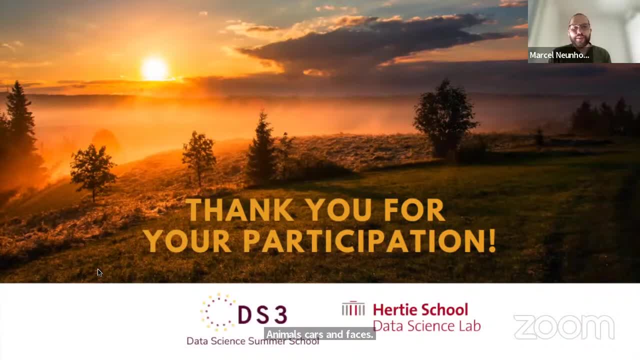 this would be very hard for the GAN to learn anything right. So the more similar the better. So I guess pre-processing the images is also one of the secrets from those high-definition GAN pictures that is not often talked about that much. 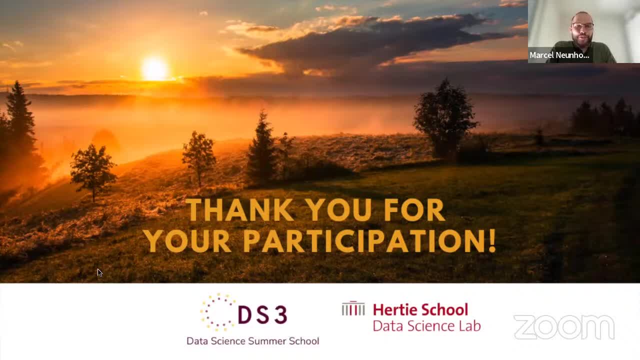 Because of course it's because the networks are so cool and not like the manual labor that has to go into it before Awesome. Thank you so much, Marcel. I don't see any more questions. There's a lot of thanks. 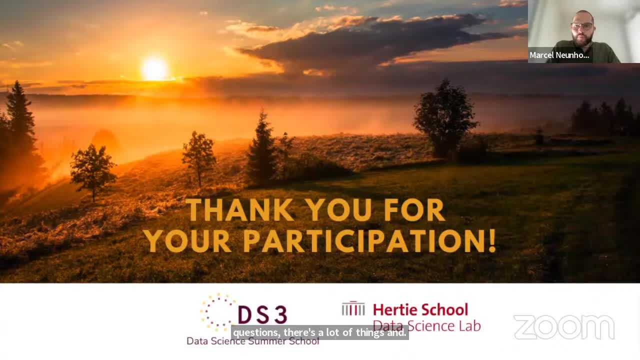 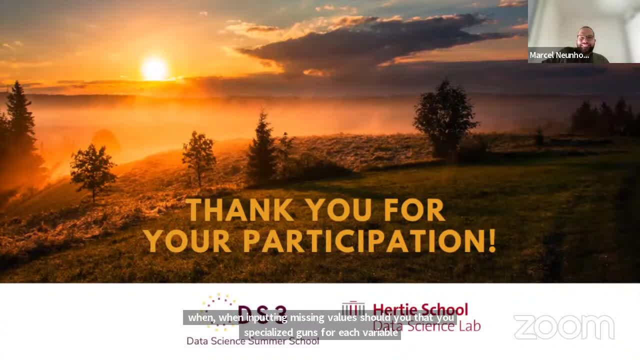 Again, I don't have a definitive answer for that. The way I would think about it and how I would think about how GANs in the context of imputation would make sense is to I would try to draw from the underlying joint distribution. 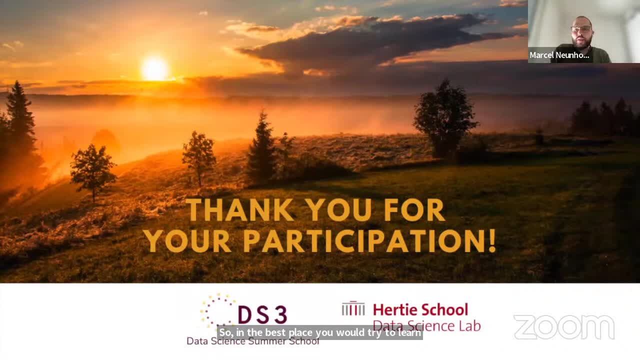 So in the best case, you would try to learn like the joint model for the data And like this can also entail making specialized choices for variables Like think of, like those mixed data types, Like if you have like real valued data and categorical values. 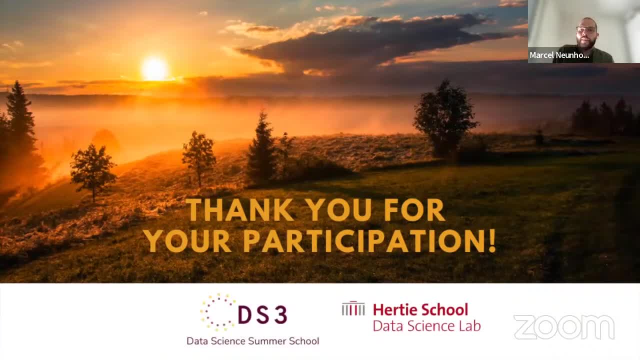 like you would need to make sure in the architecture that like you get the output that you expect for each variable. But I wouldn't use like a GAN for every variable separately. So I would try to learn like a joint model that tries to learn like the underlying distribution. 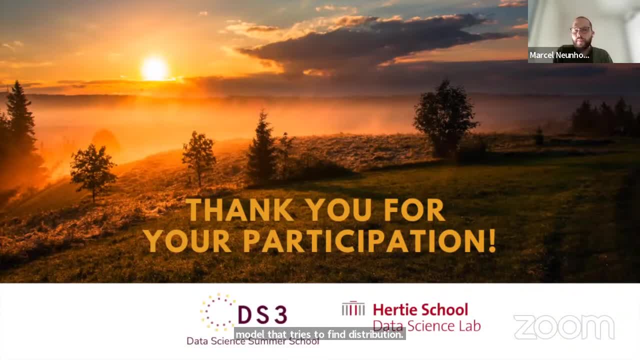 But that's how it makes sense. Otherwise, you could use, like the change equation, which is like you know. you could use like the change equation approach with, like I don't know, flexible neural networks as well, which would probably also yield very good results.